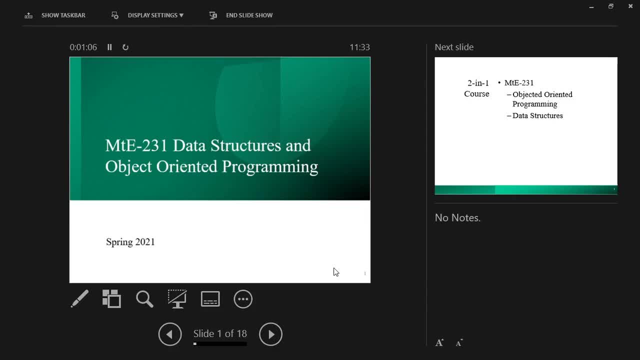 So, in the previous offerings of this course, usually I used to take, I used to give a quiz to the students, and that quiz involved, 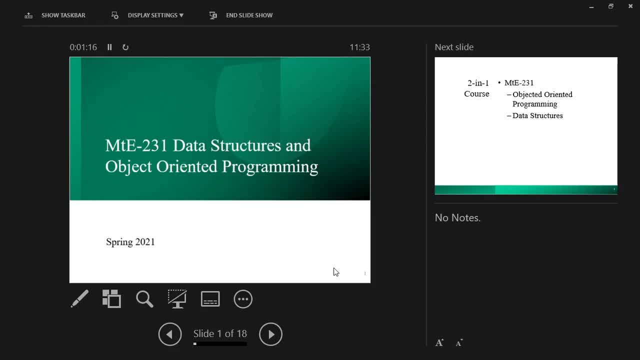 that quiz was meant to check your understanding. So, that quiz was meant to check your understanding of the concept of computer programming. 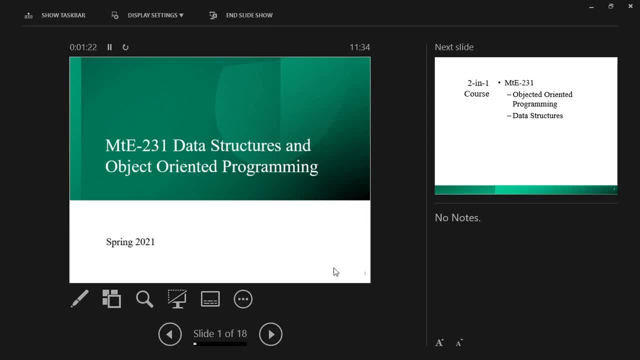 So, that, like we know that you will be comfortable in this course. So, let me give you a heads up. 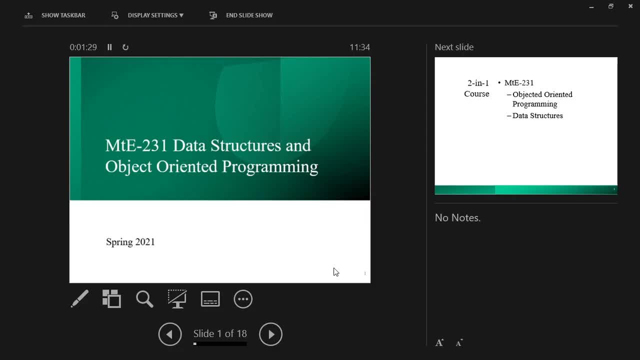 So, in this course, I guess in one of the lab sessions that we have had so far, if you have watched those video demonstrations, so, when we were creating objects, and we were talking about member access operators, okay, so, we talked about two types of member access operators, the dot member access operator and the arrow member access operator. 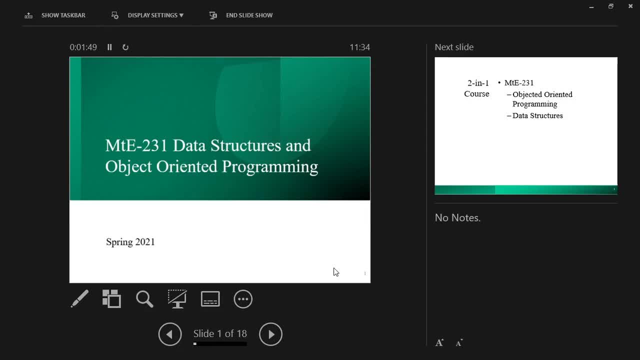 The dot you use with normal objects that you create by declaring variables, and the arrow member access operator you use with pointers. 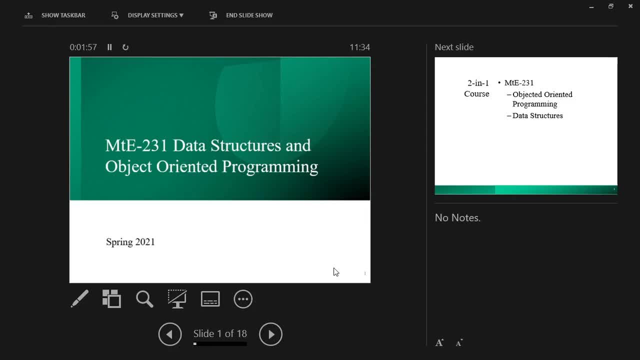 When you have pointer to an object, so, then you use the arrow member access operator. So, I hope like you have gone, you have watched that demonstration, and you know how to use pointers and all that. 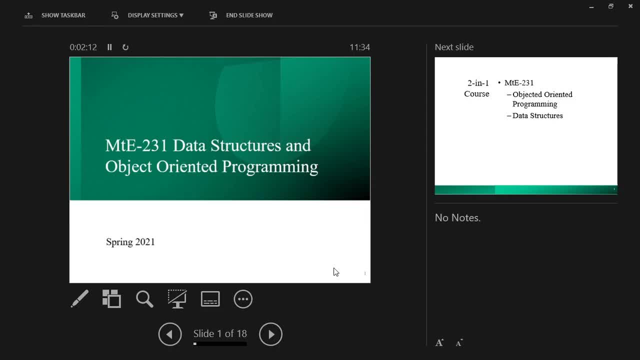 So, I expect that, that you have studied something about pointers in computer programming. 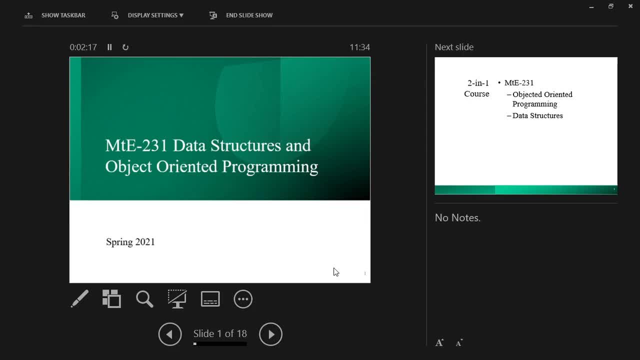 If you haven't, we will be using pointers extensively in different lab sessions, especially in the data structures part of this course, okay. 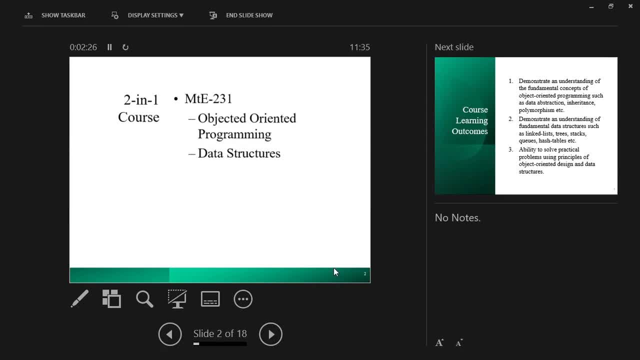 So, this is a combination of two courses, but we will squeeze it. So, that means like, 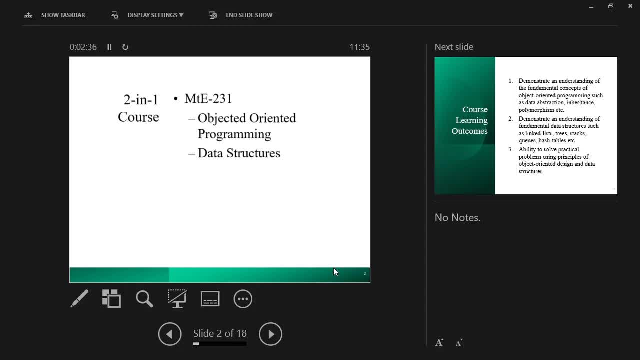 we will not like go into very extensive detail of object-oriented programming, and similarly, you won't be 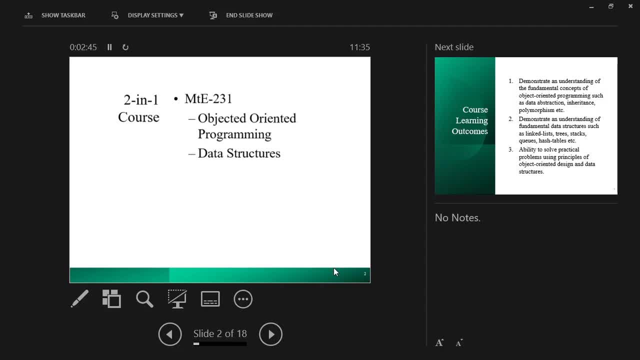 studying almost all the data structures. So, we will be studying only a few very important data structures. 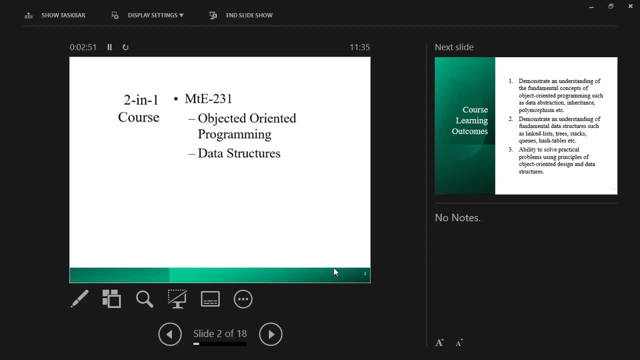 Now, object-oriented programming, as you might guess from the name, it is a type of programming. There are different ways of programming your computer. 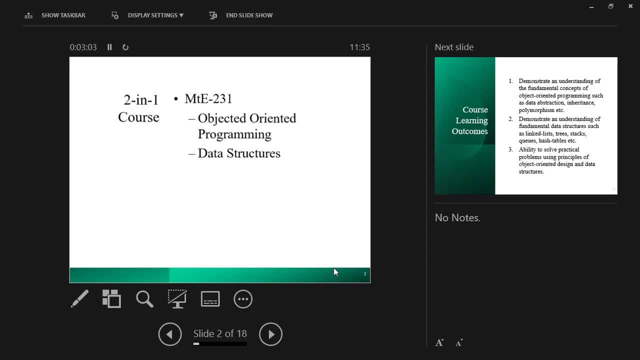 And whenever we say programming, so, we will talk about programming like, we will revisit the definition of programming, what is programming. So, programming is all about problem solving using computers. You solve problems using the computer. So, how do you solve problems using your computer? So, it has many aspects. One is how you can view the problem. How you can see the problem, how you can understand the problem, and then you have to recreate the same environment using a computer. 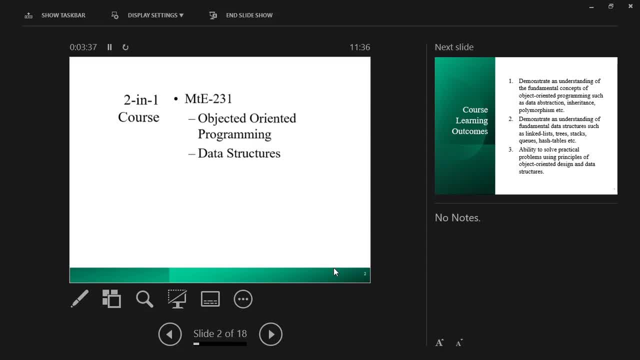 So, if you want to solve that problem on a computer, then the environment in which you are solving the problem, you have to recreate it on your computer. Now, this may be different. 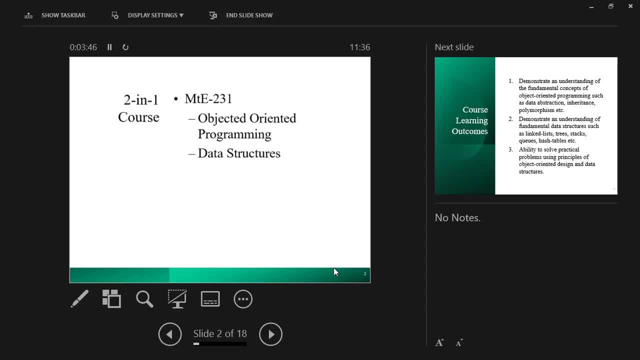 Okay. mapping is not always easy. It is not always clear. It is not always ideal. There can be many problems. So, in computer programming, you were doing something that we call structured programming or something that we call procedural programming. So, structured programming means that your programs have some structure. They can be divided into different modules and submodules like functions and subroutines. So, you had the main subroutine and from the main subroutine, you had other subroutines. You would call other subroutines from the main subroutine. This is how you must have done programming in the course computer programming. So, computer programming was all about writing blocks of code that we called functions. 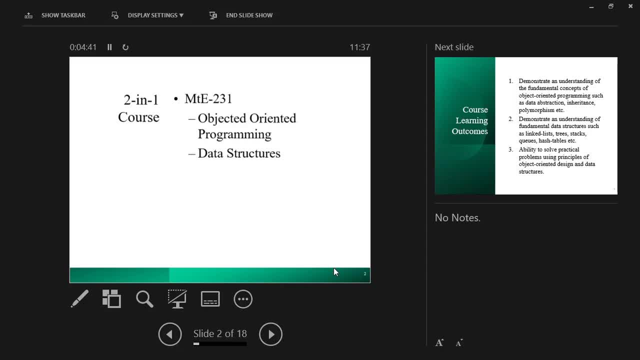 Each function or subroutine would do something specific. That is what computer programming is all about. Before that, like at the very beginning of computers, there was no concept of procedures or subroutines or functions. If you had to solve some problem, you just started writing code and it was basically a sequence of instructions. There was no structure or organization to those programs. It was just a sequence. Did you get that? did you actually get the track? No, I did not. 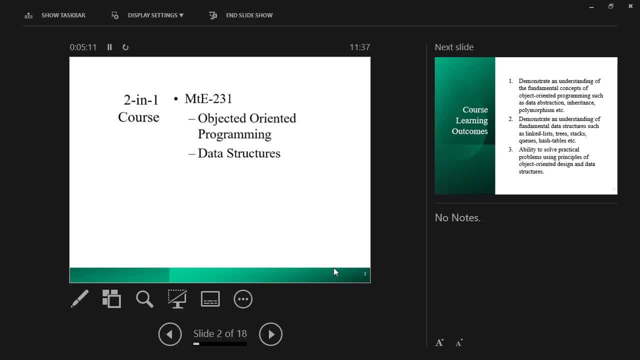 sequence of instructions. That was unstructured programming. That was in the beginning of computing when computers were just invented and people had very little idea about code organization and all those things and in fact the problems that people used to solve during those days they were not that they were important problems but they were this specific problem one problem a computer was a single tasking machine it was not a multitasking machine like right now we are multitasking right now we have a powerpoint slideshow going on in the background there is a recording going on so my voice is being recording the screen is being recorded so this was not the case in the early days of computing. Computing was very simple so you only had one program and the computer was running only that program so that was single tasking environment it was not multitasking so in a single tasking environment like usually in the very beginning some programs used to be unstructured so it was just a sequence of 1,000 or 2,000 or 3,000 instructions and that was executed like that the code was not divided into subroutines or functions and there was no organization like this function would call this one and this one with them or this one and something like that but we have come a long way from that the performance of hardware has 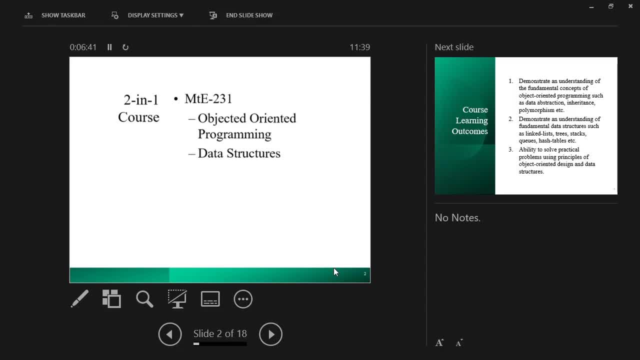 increased many many fold in fact Europe if you are aware of the Moore's law the code stated that every 18 months or two years the number of transistors on the microprocessor would double okay so it was not physical law or universal law it was a prediction made by someone Gordon Moore I guess and chip industry that prediction right for I guess 20 or 30 years or so. So if you have heard about the Apple M1 chip, the microprocessor that Apple has introduced for laptops and desktop computers and which is based on the same technology the ARM microprocessor technology that you use in your smartphones. So that processor has more than 1 billion transistors in a very small area. Okay, perhaps that is the highest number of transistors on a single chip and I guess it uses the 7 nanometer process technology that means that the smallest feature on that chip is 7 nanometer big. Okay, so that is a very small length and soon people like they predict that we will reach the quantum limit. Maybe the size of features or transistors or devices like it will reach that of a single atom and then beyond that we will not be 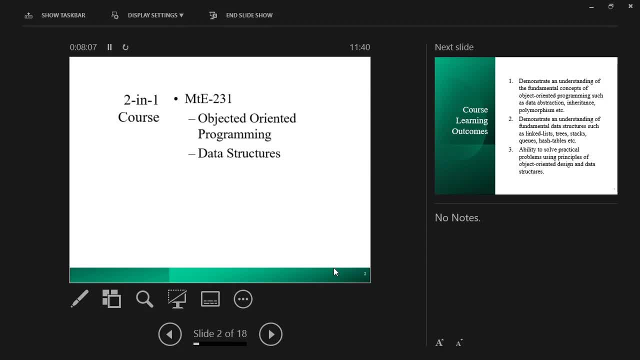 able to make transistors smaller on the microprocessor. So that would be the limit. So after that we would need to think of other ways of improving performance. So this is one way of improving chip performance and that is by making the transistor smaller and smaller so that more transistors can be fitted into the same area and you can get more computing power out of the same physical area. Okay, so that nowadays like we have pretty much reached that limit through which you cannot increase the computing power of a single chip. So that's why we have multi-core processors right now. So we want to do things in parallel and before we had multi-core processors we had single core processors and those processors did something that we call multitasking. They used to execute different programs and the execution appeared to happen at the same time. 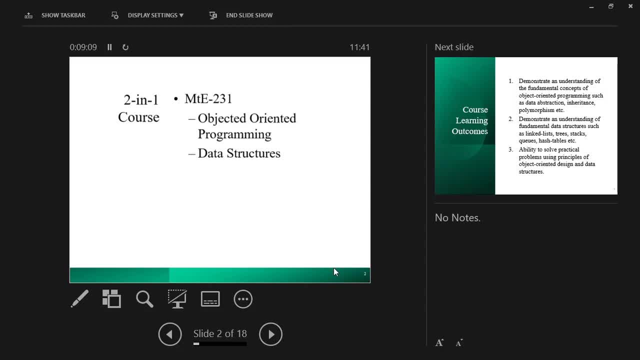 You used to feel like this is happening at the same time. But that was not possible like there was one microprocessor it can only execute one program. So the microprocessor since it operated at very high speed so it would switch between different tasks. So say for one microsecond it executes Microsoft Office for another microsecond it execute another process then another process. So in a round-robin fashion it would execute all the processes one by one for a very small amount of time one microsecond. So we would not feel one microsecond. Aara jo response time hai the way we work. Aara jo vision system hai se one tenth of a second se pehle justify kochi ho jaate hai so we don't feel going ahead with she's urge of each is we don't feel take it so that's why you see all the things there although there are only three wings but since our ajo vision system hey it's response like it needs one tenth of a second before it can process another image if the images keep on changing so it won't be able to process those images similarly sound which hearing system so you need one tenth of a second of a delay between two sounds in order to to detect otherwise you will hear a continuity of one sound reverberation 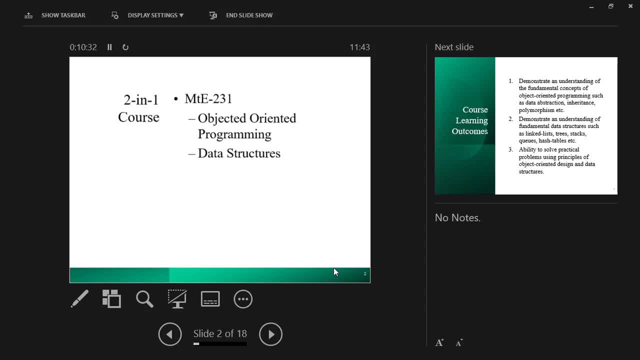 so this one tenth of a second interval this is critical so when 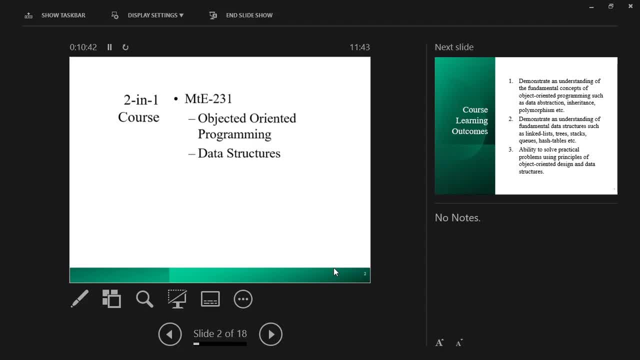 when the computer became complex and the problems that you wanted to solve using the computer those problems became more complex and complicated then you need needed to have tools that would allow you to solve those complex problems so the way we programmed computers that had to change 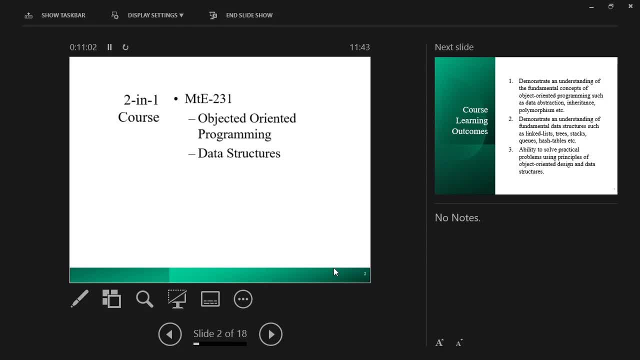 and one change that came was structured programming was introduced or procedural programming within procedure programming abhi it is very popular it is very useful and maybe uh 80 to 90 percent of the code this is just a rough guess 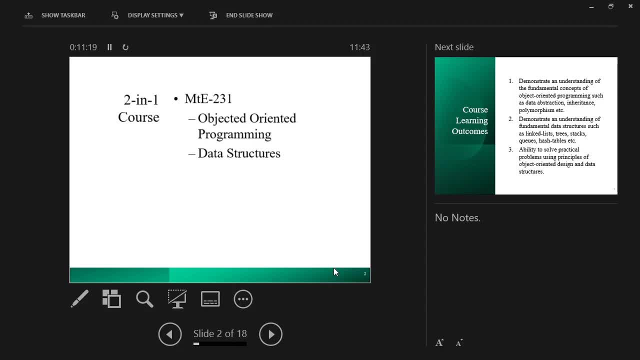 that you that you interact with on a daily basis it would be based on procedural programming okay although we learned in this course that object-oriented programming is 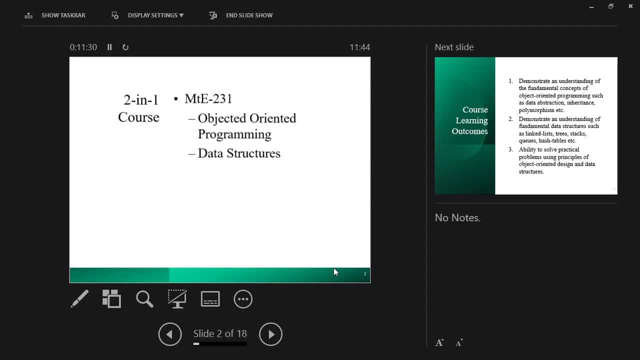 is also a very good way of programming computers but it is not the best way in in the view in the eyes of some it is not the 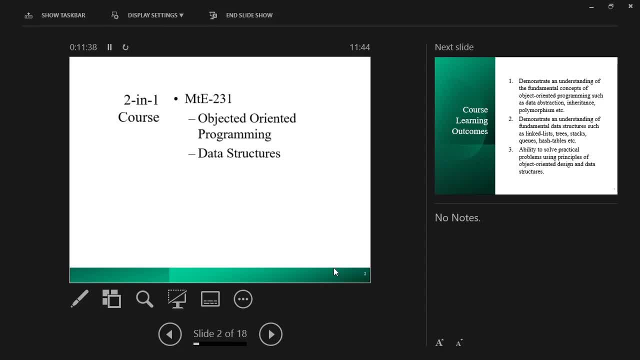 best way to program computers it may be best for some people under some circumstances but it is not always the best so many people still prefer to do procedural programming so we learn what procedural programming is but object-oriented programming is another way of looking at a problem and trying to 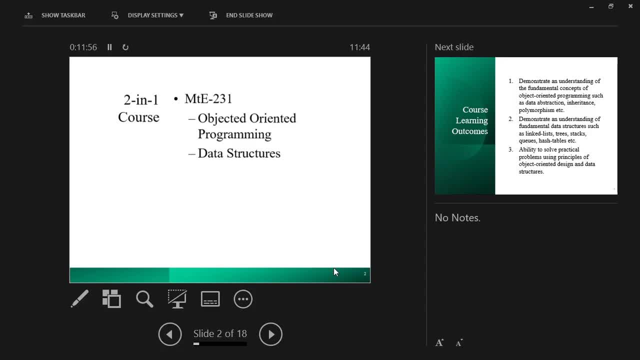 solve that problem and this way of problem solving is more more akin to what we do in the real world like in the real world if you see around you have different objects so we have this laptop and this laptop has an interface and i interact with this laptop through that interface this air conditioner this is an object it has its attributes and its behavior it can do certain things for you and it gives you an interface through which you can interact with this air conditioner similarly if you look at humans like we humans so we're also kind of objects and we interact with each other we have our own attributes and our own behavior and then we interact with each other through certain interface okay so if you look around the real world so all you can see is objects with some interface and those objects interacting with each other sending messages to each other requesting one one another to do things for themselves that is how things are in the real world so object oriented programming was was designed to model the world in this in this particular way now it may be appropriate in some situations it may not be that appropriate another situation for example if you are a game programmer then maybe object oriented 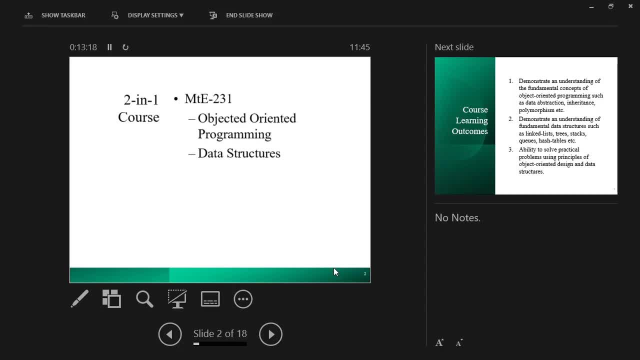 programming would be would sound very ideal to you because then you you have to simulate a complete real-world environment you have you need to have a concept have you have to have a concept you need to have the conversation have you need to have the conversation have cars running around, you need to have buildings and roads and all that. So, it would make more sense if you can think of those objects as objects in software as well. They are real world objects that you need to recreate or simulate on the computer. So, if you can think of those real world objects as software objects as well, then that would make more sense. So, in that situation, object-oriented programming would make more sense. It would be more appealing. 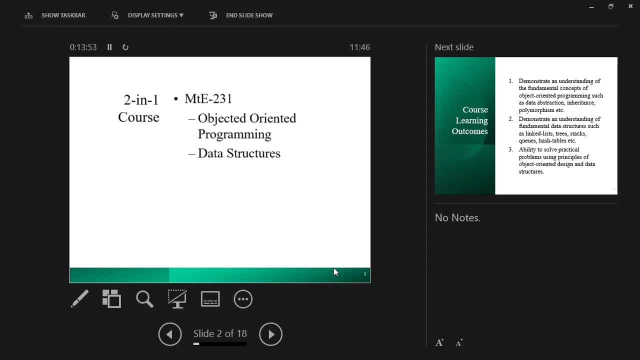 Similarly, those people who work on software and they work for software in organizations that are based on that, that basically whose sole purpose is to create software and sell it to other people. So, managers working in those organizations, software houses and say in Microsoft or maybe other organizations. So, they kind of prefer object-oriented programming. 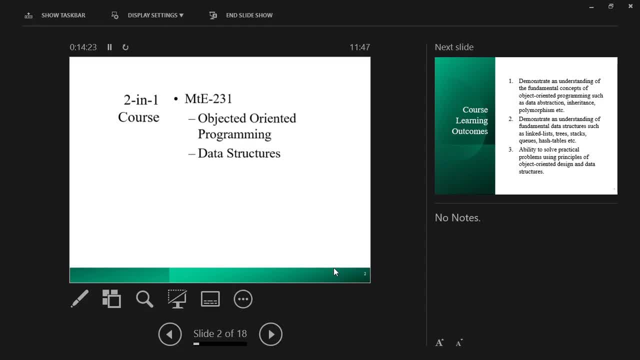 So, they kind of prefer object-oriented programming. So, they kind of prefer object-oriented programming. Why? Because object-oriented programming languages are relatively easier to maintain. If you write code in object-oriented programming, so it is a little easy to maintain that code. 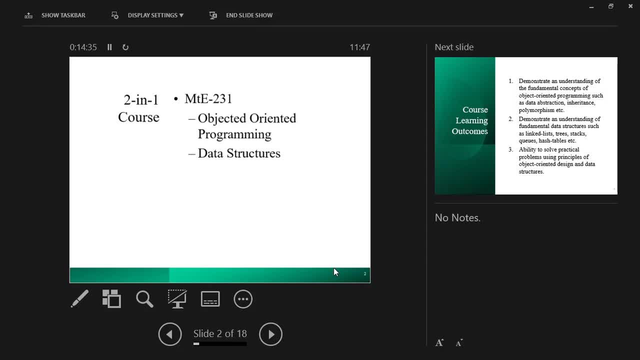 People may come and go from like they may join and new people may join the organization and old people may leave. But the new people may not find it that difficult to work on that code. 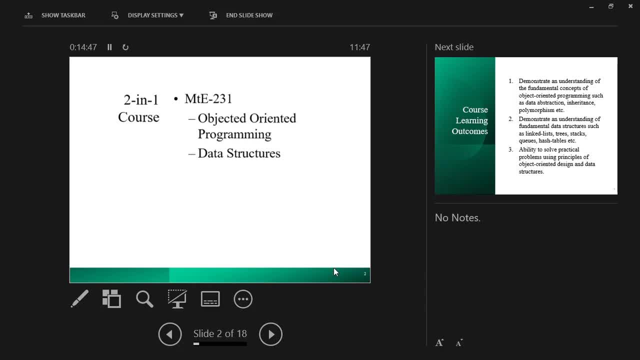 Okay. So, code maintenance and all these issues that are related to software engineering that becomes easy. So, even if you do not like object-oriented programming as a programmer, 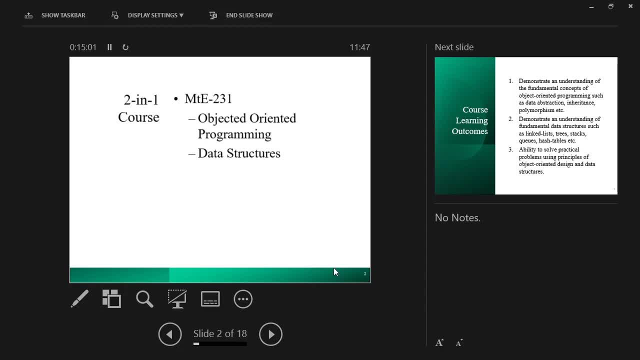 so you may not be programmers, but if somebody is working as a programmer, even if he or she does not like it as a programmer, maybe his or her boss would like this language. 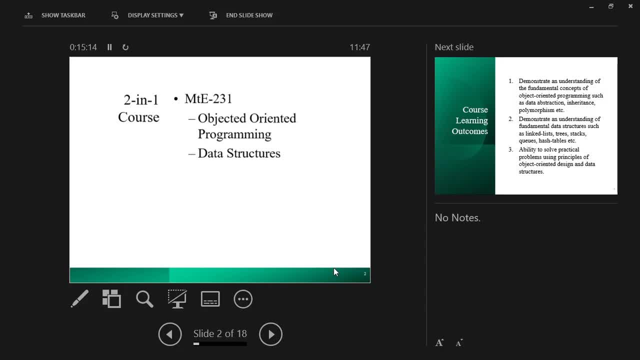 Why? Because the manager's job becomes easier. Because he or she has to ensure that the project goes on even if people come and move out of the project. Okay. So, object-oriented programming is a paradigm 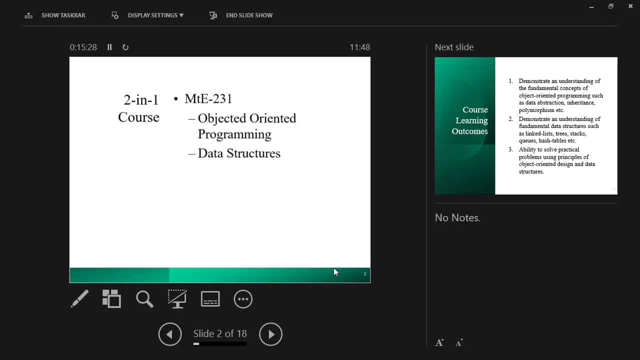 of programming, a way of programming computers, a way of thinking about problems, visualizing problems and then solving problems. And data structures, again, data structures are also 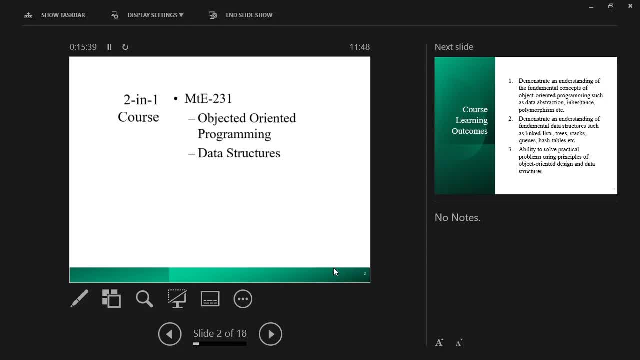 very important. There are plenty of data structures that we use behind the scene. For example, you must have used the undo feature in Word and PowerPoint, control plus Z, undo. You must have used undo. Now, how does undo work? If you undo something, the latest action 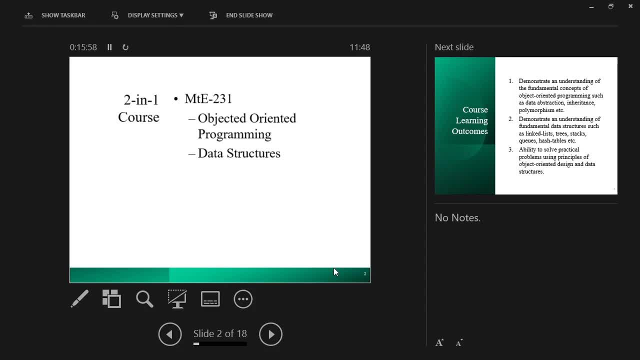 that you perform, the last action that you perform, that is undone. Okay. If you press undo again, so the second last is undone. If you press it again, the third last is undone. 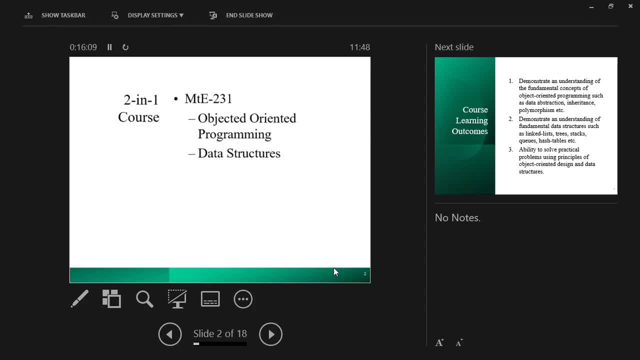 So, how does Microsoft Word or Microsoft Office or PowerPoint, how do they know like which action to perform, which action to undo? So, they maintain a data structure. That data structure is called a stack. 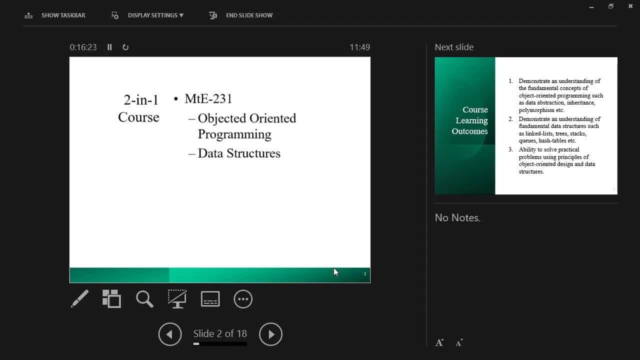 So, a stack is just like a stack of plates or a magazine in a, in a pistol. Okay. So, if you look at a stack of, if you, if you have gone to a restaurant and attended some buffet, so there is a stack of plate and from that stack, you can only take the plate from the top. So, when you take a plate from the top, the stack is spring-loaded. So, wo uspe vazan kam ho jata, wo thoda sa upar aa jaata. Thike, upar ek aur plate aa jaati hai. So, aap phir wahan se ek plate uthatdey, so upar ek aur plate aa jaati hai. So, on a stack, data comes in at the top and data is taken off from the top. Okay. So, this is a specific architecture. Now, this is a very useful way of storing data. Data ko store karne aur usko read karne ka yeh badaa, this is a very useful way of doing it. Ki aap sirf top pe data ko store kar sakhein aur wahan se retrieve kar sakhein. 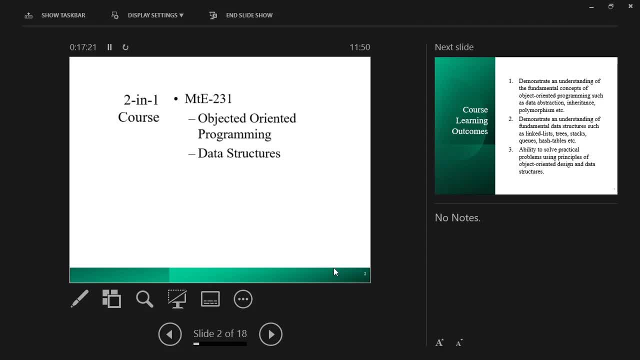 How, why is it useful? So one situation is this undo thing. Jo bhi aap action perform karte hain, to Microsoft Word takes that information about that action and pushes it onto a stack, wo ek stack pe rakh deta. Phir aap ek kuch aur kaam karte hain, to wo ek stack pe wo karta jaata. So you are typing in Microsoft Word and you are formatting and doing all things and behind the scenes, Microsoft Word is recording each and every action that you perform. Aur wo saare actions jo hain, wo stack pe wo dalta rehta hai. 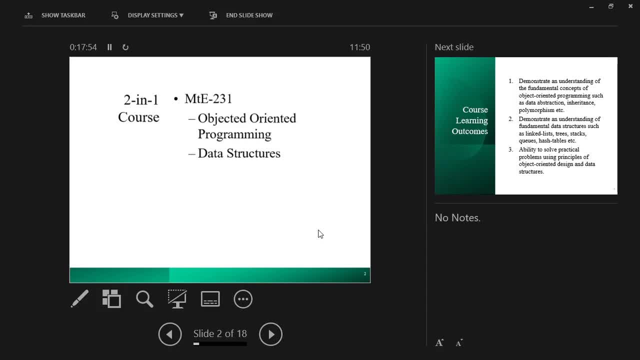 And if you decide that, if you find out that I have done something wrong and I want to undo the last action, then you press ctrl to z, so how would Microsoft Word know which action to undo? So it would go to that stack, it would pick up the action from the top. And it would undo the effect of that action. How does it do it? That is again complicated. 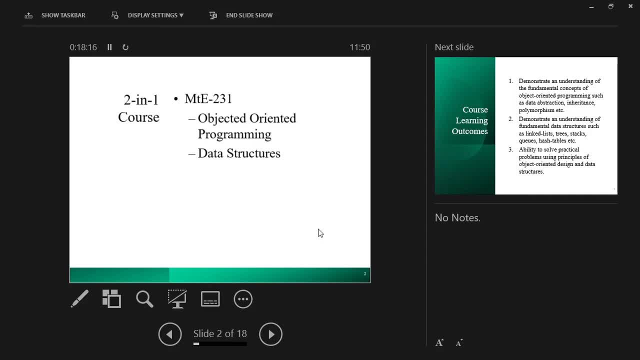 So it's not that complicated, it cannot be figured out, but it is complicated enough ke mai yahaan explain neekar sakta. 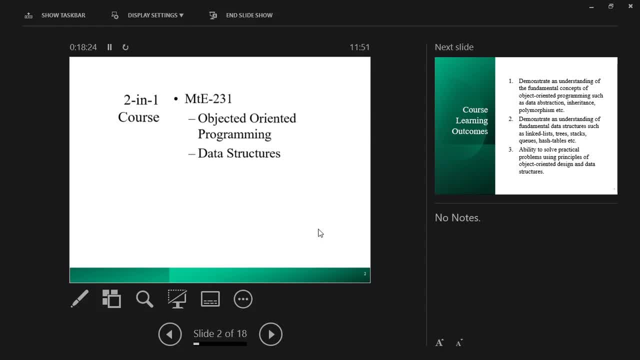 The other example, you all use browsers, internet browsers to browse the internet. So if you are visiting browsers and then you have this back button on the browser, if you want to visit the last page, you press the back button. The second. Last page, you press it again and again. 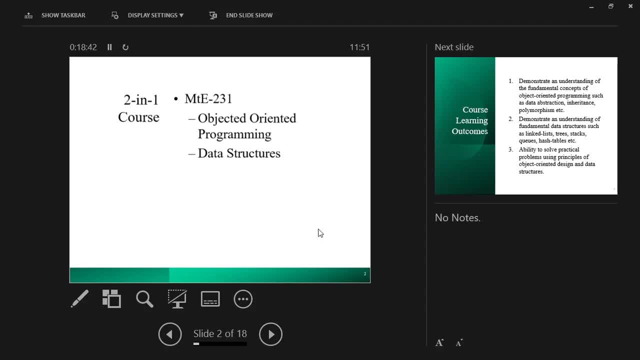 So your browser also maintains the list of web pages that you are visiting. And it maintains a stack aur stack pe un pages ki urls wo dalta rehta jisko aap visit karte jaate hain. If you click a link, you visit, you are basically opening a new page, the url of that page goes on to the stack. Wahaan pe you click another link, so you open a new page. The url of that page. Then it goes on to the stack. So when you decide to go back, so the browser accesses that stack and picks up the top entry. Aur aapko page pe le jaata hai. 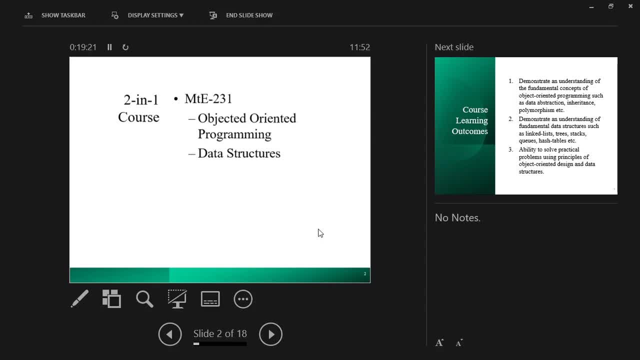 If you want to go further, back, so it picks up another url from the top. 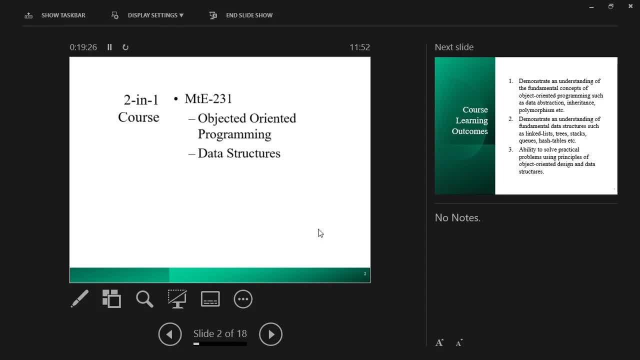 Similarly, queues. Queue is another data structure. 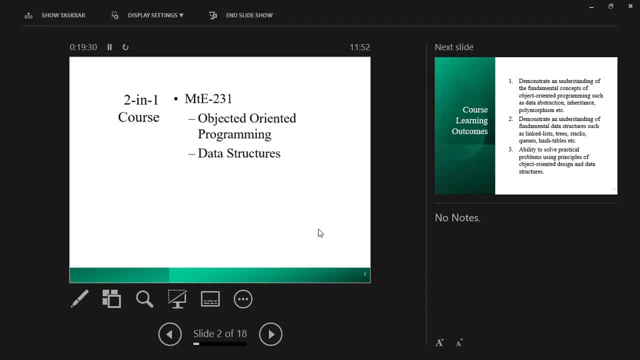 And like we are aware of queues. Aap kahin pe pe jaate hain, so queues are basically first in first out structures. Jee, please. 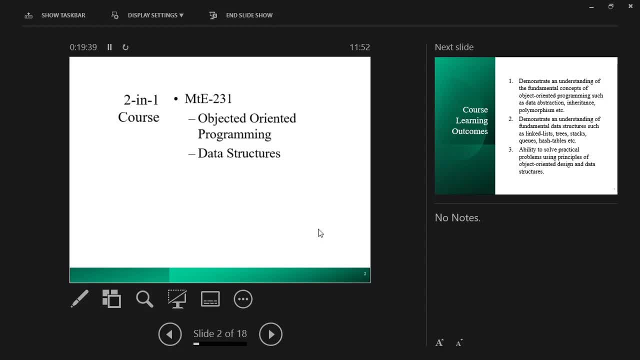 So in a queue like, queue katar, queue means katar. So if you go to any place where there is one service provider, and there are many people who need that service, for example, if you go to a bank, there is one person who can handle cash, and you all need to draw money using your checks. 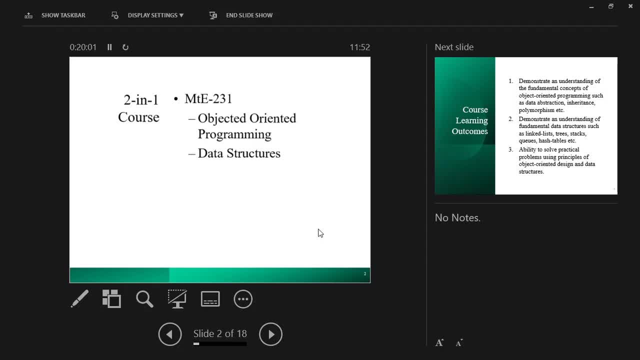 So there are five people of those five people need to make a queue. Okay. The. Pressure line is extremely big. Because the one person who has come first, he or she deserved to be served first as well. So that's why a queue is called a first in first out data structure. A queue is called first in first out data structure. 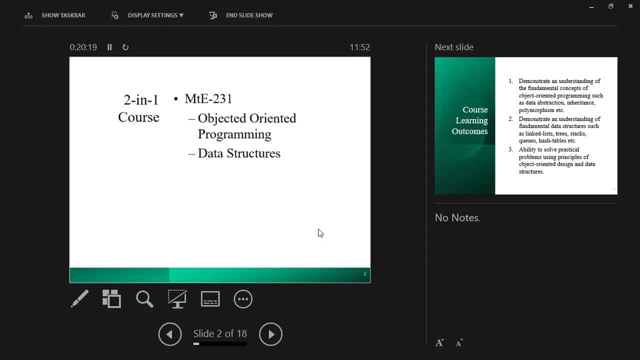 Those of you who have joined late, so I'm recording the session, you can watch it. 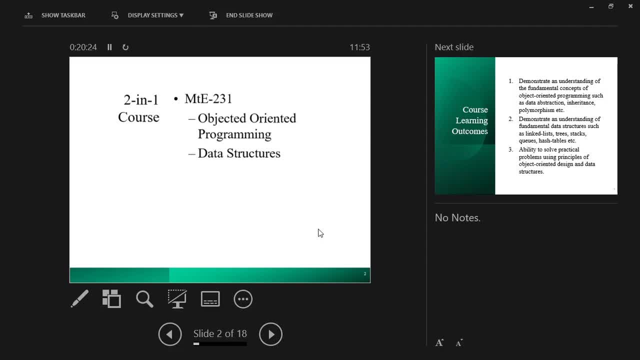 Don't worry this focus on whatever we are discussing right now. 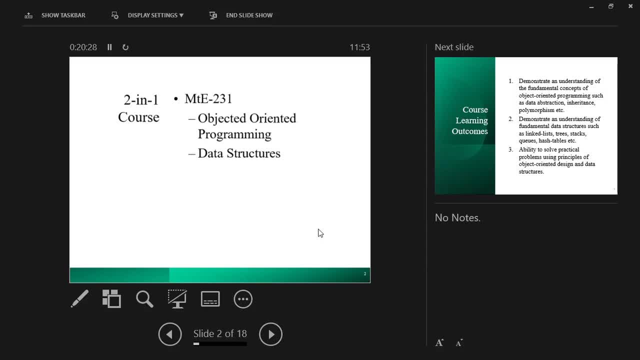 So a queue is the first in first out data structures. Now a queue is a data structure . Okay. Thank you. 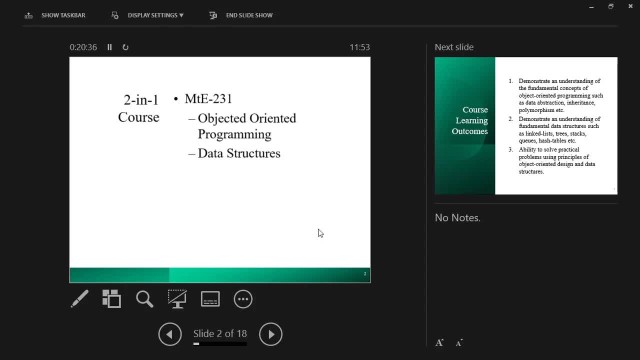 Let me continue my question's going, okay. our daily lives like wherever we go if we are disciplined and good people well-mannered so 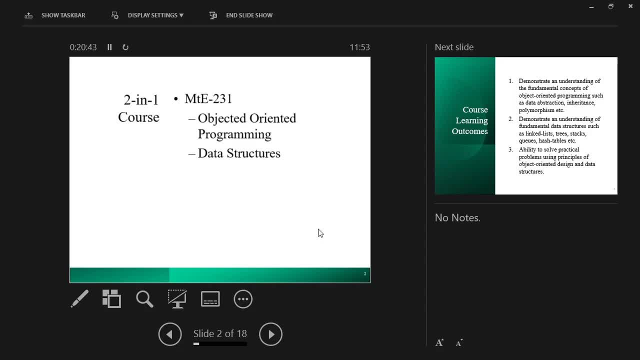 we make cues and then uh we are served uh as per our position in those cubes 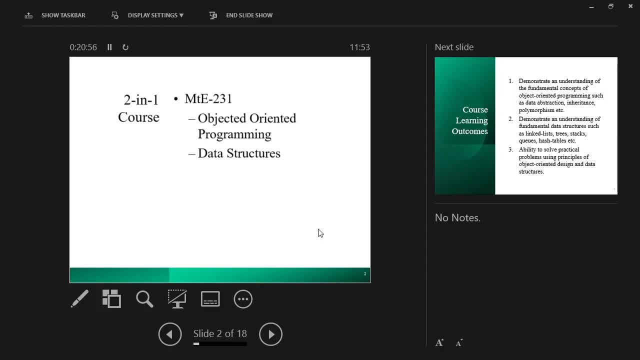 now all these communication networks communication networks means all the uh all the computers that are connected via the internet these mobile phones and everything so all these devices they are connected through a network okay so if i send a message that message goes through plenty of computers and finally it reaches its destination so if i type a whatsapp message so my whatsapp message would go from my smartphone to the jazz networks computer the nearest bts it would like it would go there then it would go to the jazz network from that if the other it would go to whatsapp servers 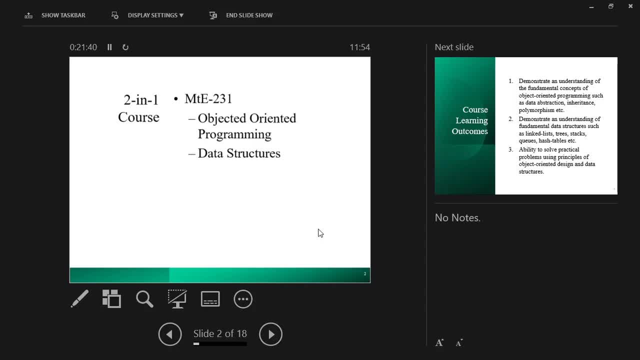 from whatsapp servers it would go to ultimately if the person i'm trying to communicate with if that person happens to be on telenor's network from whatsapp network it will go it will come to telenor's network and from there it will go to that person's smartphone okay 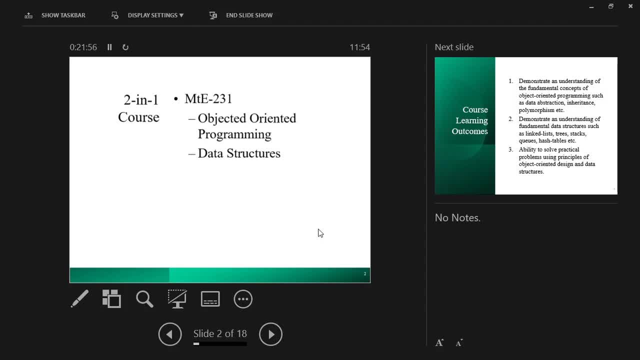 so this is a long way through which one message has to go through and it is not just one message there are billions of messages like millions of people they are constantly sending those messages and the network it is not always free to forward these messages the network can be busy the bandwidth is always limited okay and there are peak times and there are not so much peak times so sometimes the messages can go through quickly sometimes they cannot go through quick okay so every network knows that so the network has lots of memory they maintain a lot of memory and in that memory they maintain a queue of messages okay so you send those messages that message is queued somewhere in the network and then that queue is forwarded 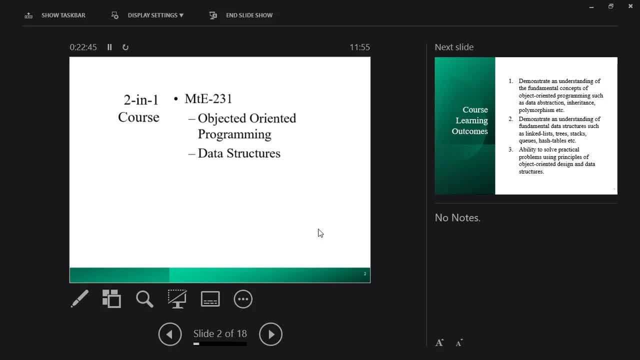 to the next destination the next destination may also maintain a queue depending upon its traffic if it is getting a lot of traffic it will have a queue if it is not getting that much traffic it will have very small queue and that queue will like vanish in a very small amount of time 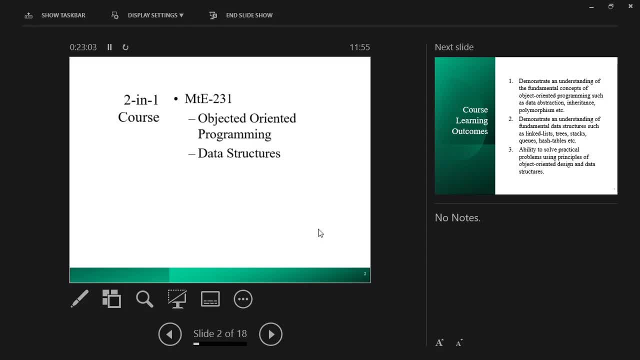 so data structures are also like important things and like virtually anything that you might come across for example databases you guys even if you don't know about databases databases are very 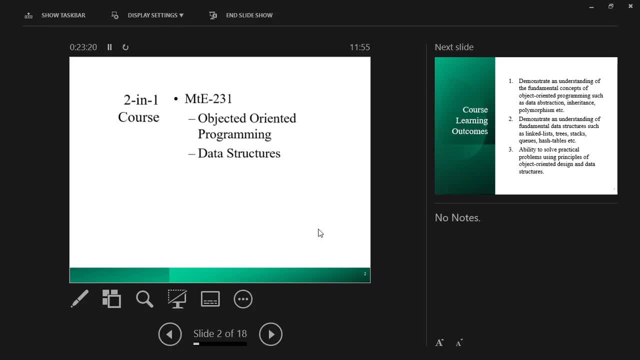 important and very extensively used for example the national database and registration authority nadra so it uses a huge database that maintains records of all the citizens in pakistan maintains the records of all the arms licenses issued to the citizens of pakistan maintains information about 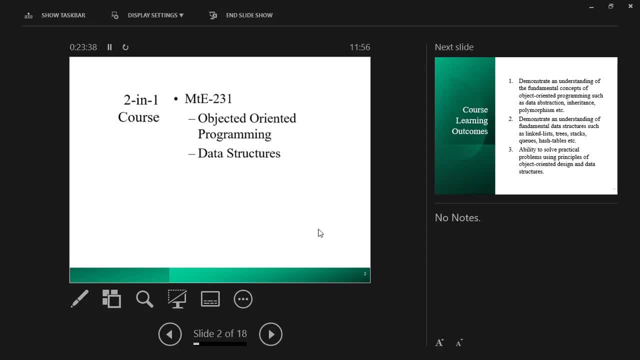 maybe passports of different uh all the citizens of pakistan okay so that is a huge database so once upon a time databases were created using data structures a specific type of data structure called trees okay but then somebody found out that it is not that it is not the best way of creating databases okay so it is a huge database and it is not the best way of creating databases okay so 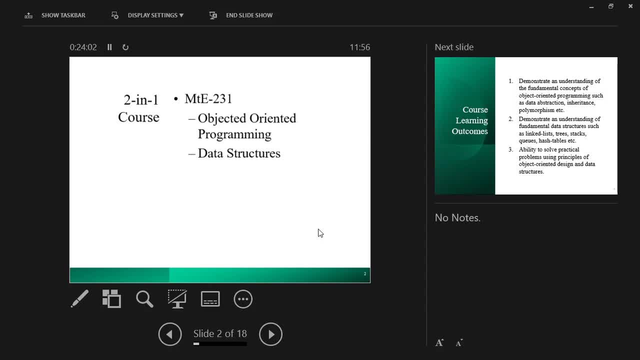 now databases are mostly relational databases so they are basically tables of data tables of data are two-dimensional arrays rows and columns and those tables are linked with each other okay so nevertheless they are also a form of data structures data structure is anything that 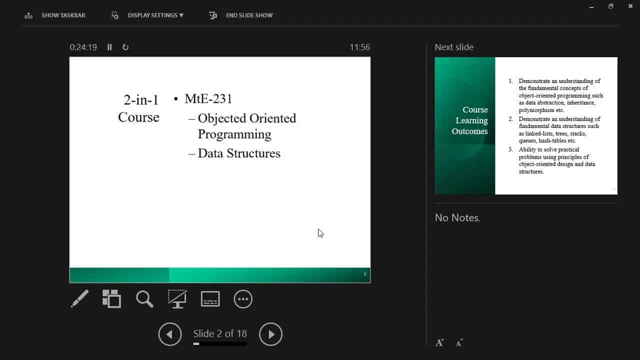 stores data anything that is used to store data so your files they are also data structure any file that you use to store data you can also think of it as a data structure it is a way of storing data so this course basically involves talking about or studying those data structures 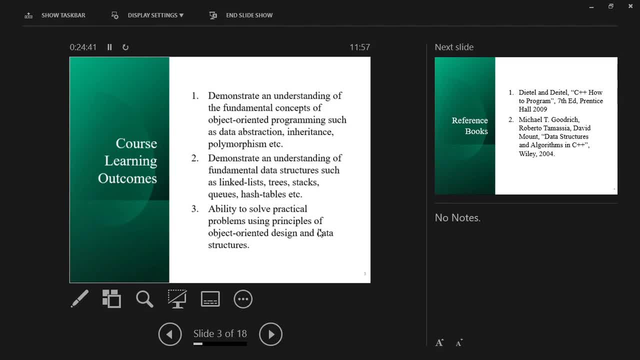 next uh we haven't talked about these uh the learning outcomes for this course like what do we want to get out of this course is number one as we said that this course is a combo course first we need to understand what is object oriented programming so you need to understand and you need to demonstrate that understanding 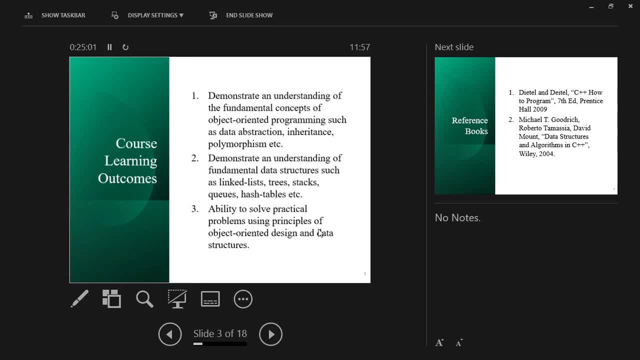 object-oriented programming has some very important characteristics one data extraction so you need to know what data extraction is and i guess like maybe i i'm not sure whether i've talked about data abstraction in those videos or not but if you have like in the first lab you were required to create structures structure is also a data structure struct you created struct you want to create a new data type that and your requirements cannot be fulfilled by the default or built-in data type so you can create you can use structures to create a new data type and i guess in the first lab session we did we created complex data type and fraction data type and similarly you can go on like you can create any type of data for example if i need to 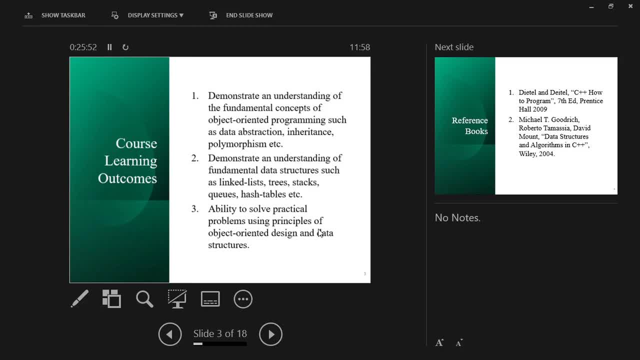 store information about students so i can create a student data type using structures so a student will have a name a registration number a date of birth and uh current semester and and things like that so we can decide about that so first is we need to understand 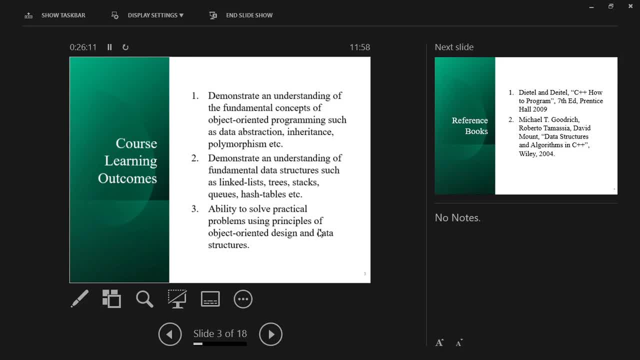 object-oriented programming so we'll talk about this we'll start from this particular lecture and we'll talk about all these things and hopefully you'll have a very clear idea about 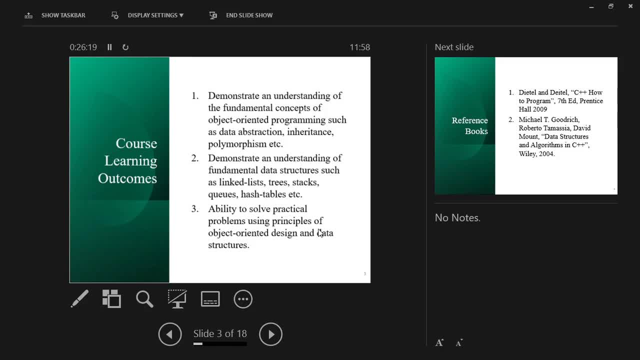 what these things are second is you need to demonstrate an understanding of the fundamental fundamental 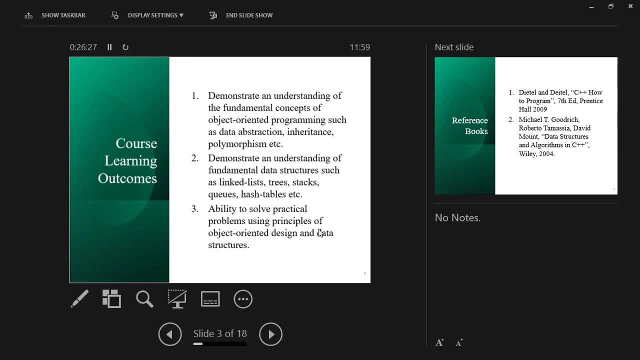 data structures like linked lists stacks cues trees hash tables etc so these are not like they may sound uh i don't know whether they sound difficult or not but definitely they are new 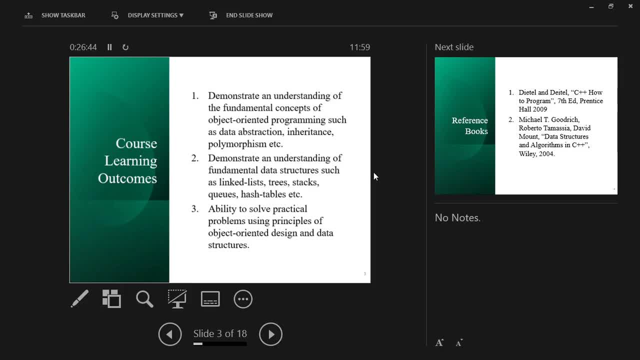 and anything new may sound a little difficult but if you have a very clear if you if you have a reasonably a decent idea of what pointers are and what references are we'll visit those things 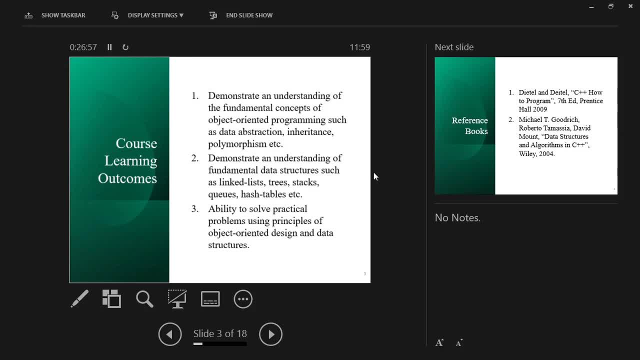 again you will find it very easy okay so these are all 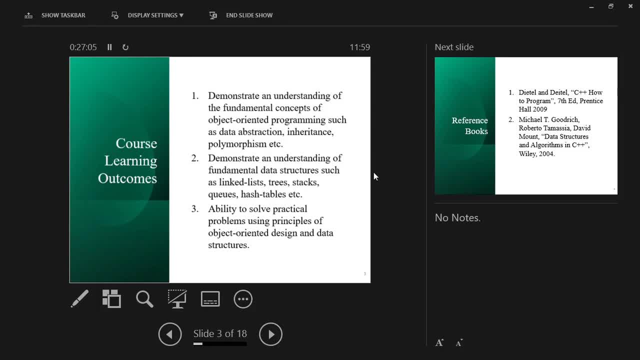 abstract data types okay a tree a stack a cube a linked list these are abstract data types these are abstractions that we create on a computer abstraction something that like does not exist in reality but uh 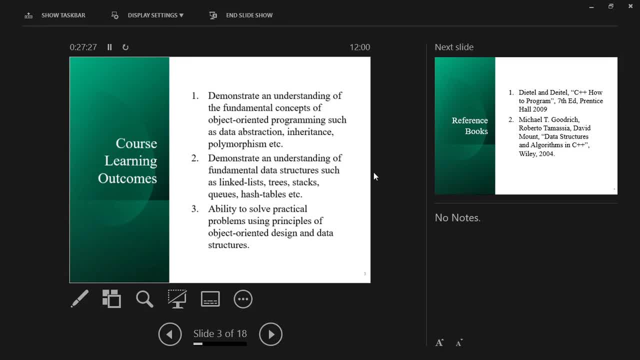 like you can create an idea of that thing you can think of other things in that term but say let me give you this as an example 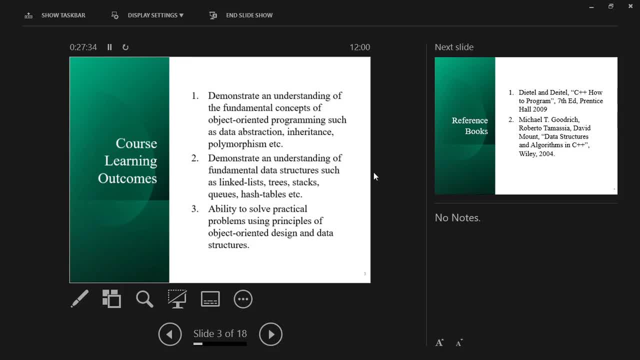 so so if you have a microprocessor for example so a microprocessor has so the basic structural unit of a 1000.000.000 microprocessor is 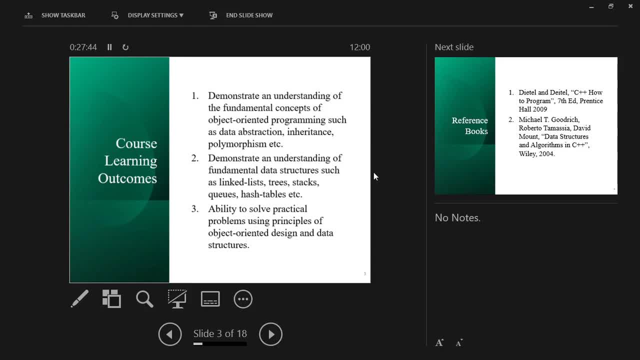 transistors so it has say 1 billion transistors 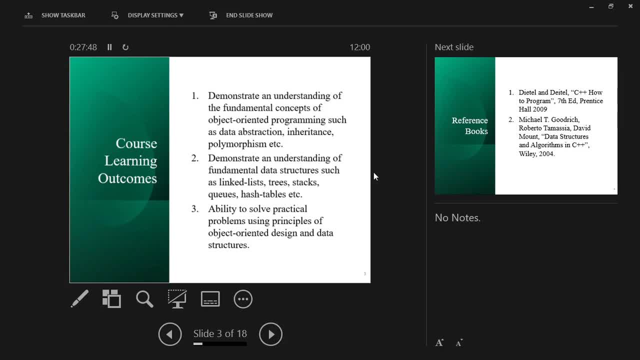 but when you have a microprocessor you do not think about think in terms of microprocessors ES 봐 ES hard to controlledily think but this also has more micro processors than rub guys i mean there are lots of micro processors there are Burma A 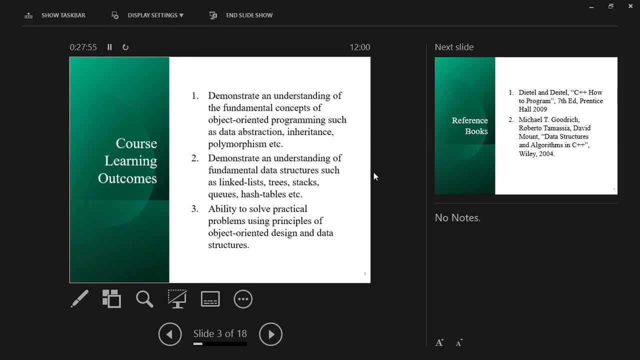 arabs is the other microprocessors you do you do not think in those terms okay we use those mic those transistors to construct gates or combinational logic devices okay so we think 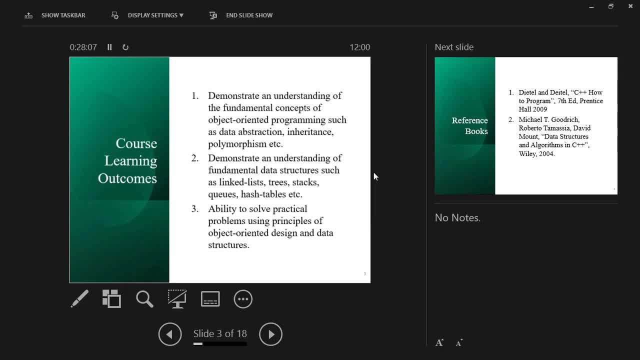 in terms of those devices okay this is an adder this is a subtractor this is a multiplier okay 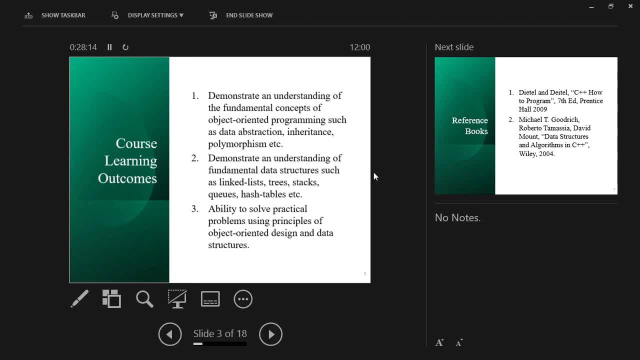 what is an adder an adder in essence is basically transistors okay what is a subtractor it is basically transistor because it is created out of transistors similarly if you look at this this building so what is the structural unit of this building okay so if we like simplify for the purpose of our discussion so maybe it is bricks okay so if you break apart this building so all you'll get is bricks okay but you we do not talk in terms of bricks or talk in terms think in terms 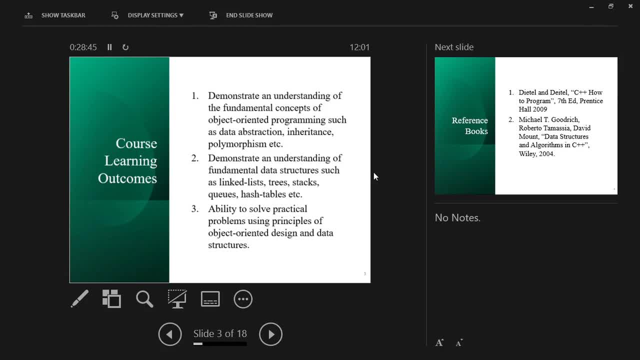 of breaks we talk in terms of rooms this is classroom one classroom two this is a lab this is an 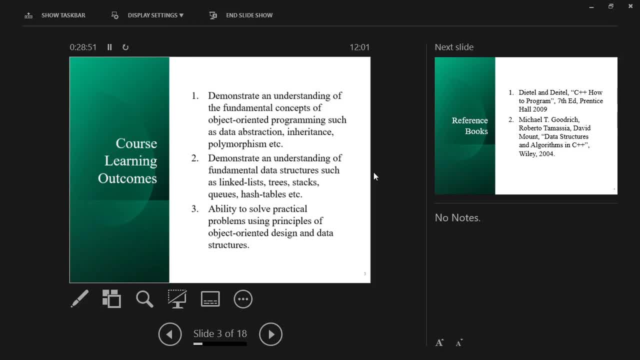 office this is a gallery this is a hall this is that this is that ticket so these are abstractions like we use those breaks and we create these abstract abstractions although like you can physically see this room as well but in the case of software engineering you will not be able to see 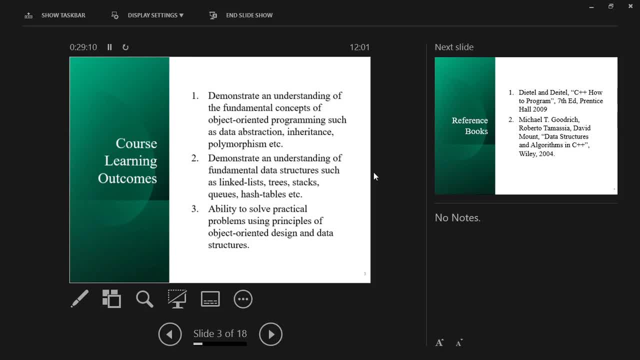 those data structures that you will create okay so we'll create an impression using push which techniques use that they will create an impression as if this thing is behaving like this particular data structure so you'll understand it hopefully inshallah third is 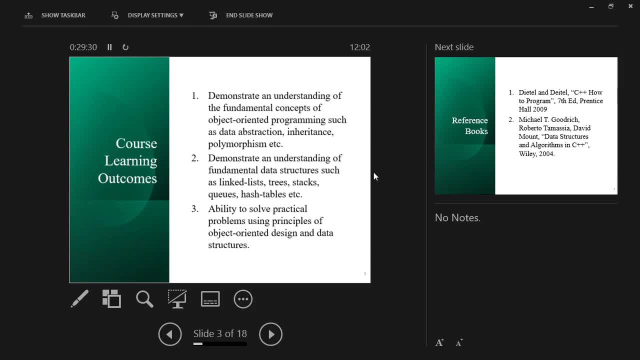 object oriented programming and data structures we we study these things for solving practical 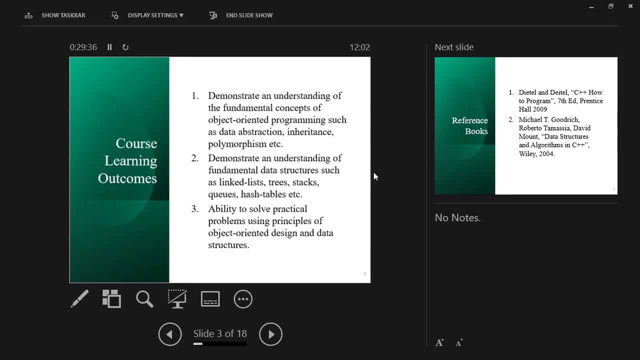 problems okay so we should also we should also be able to solve these use these techniques to solve practical useful problems 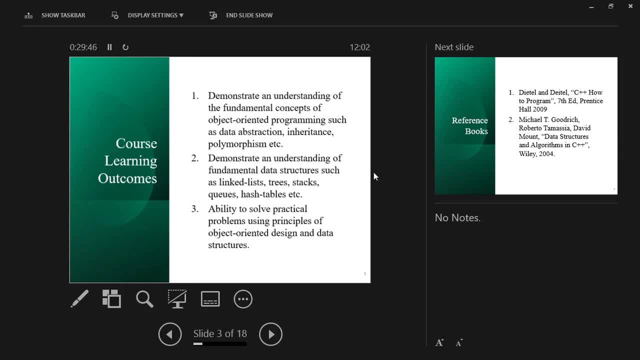 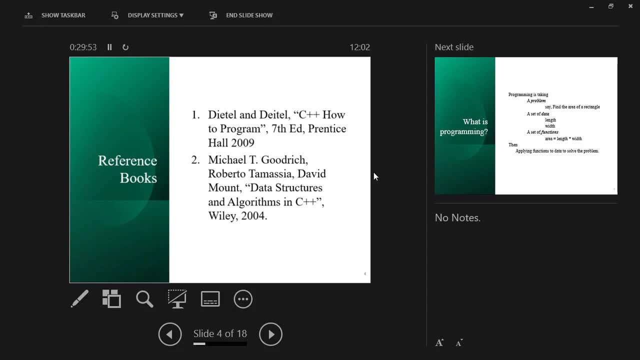 so that is the third learning outcome that we want to achieve now the books that we want to have we would refer to in this particular course is one the same book that you had for programming 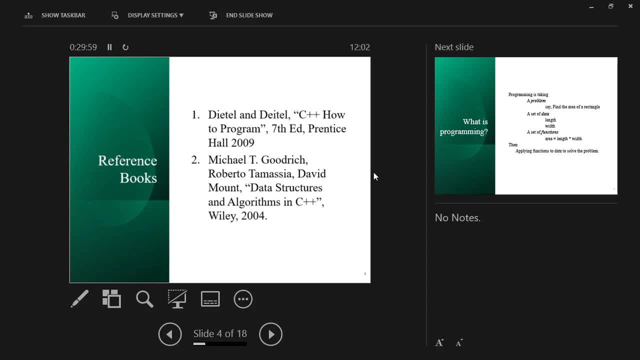 and if you have gone through that book so it basically starts in the initial chapters there's a chapter about classes and objects so it starts with classes and objects in the very 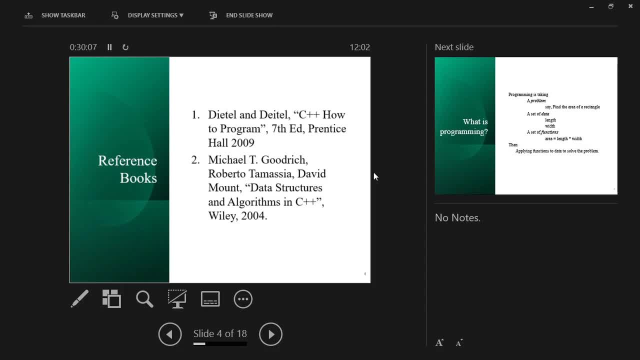 beginning so c plus plus how to program you can have any you can use any edition of it 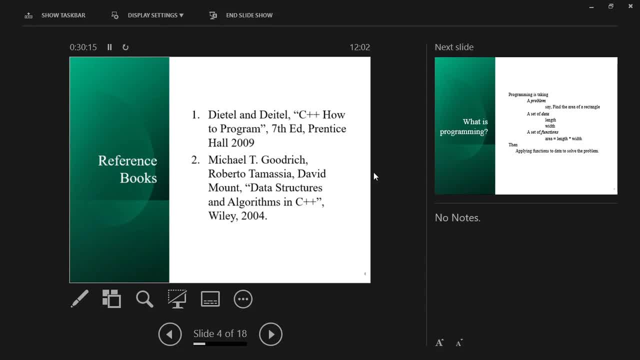 i i i i have a soft copy of it as well i'll try to share that that with you as well in fact i have soft copies of both these books okay so this one is for the 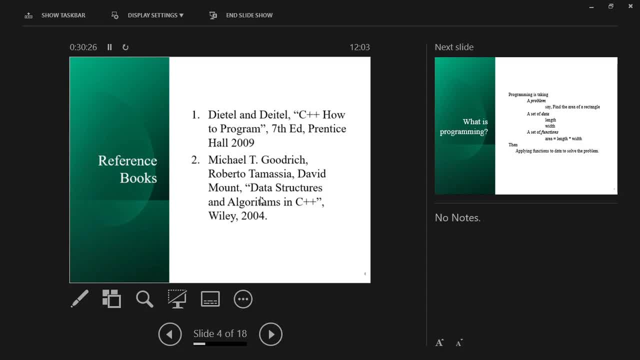 data structures part you can also like refer to it for object oriented programming as well because the first chapter of this book it deals with object oriented programming very briefly because you need to understand object oriented programming for in order to understand data structures because 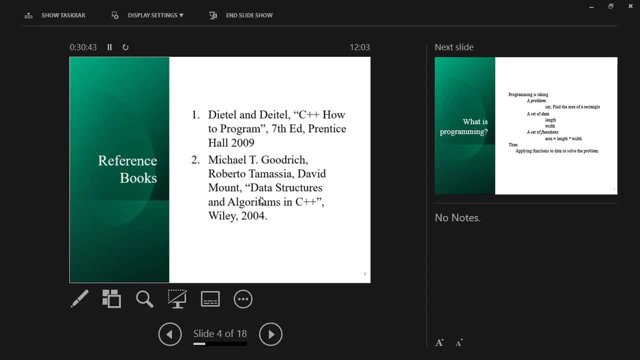 data structures are created using uh object oriented programming now if you remember when we talked about classes and objects we said that you classes and objects basically they are a means of creating new types new user defined types you can create new types and you can define behavior for 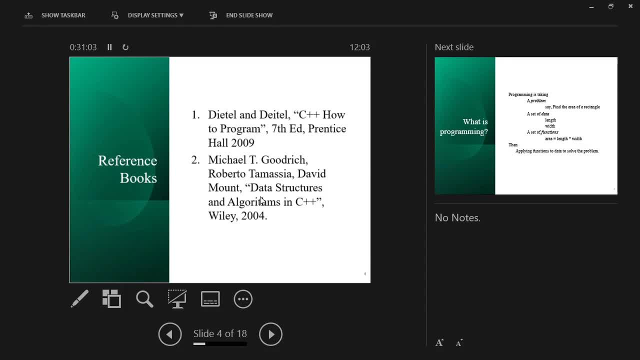 those types using object oriented programming so data structures are also new data types they are kind of new data types so that's why they are closely connected hoop and data structures they are closely connected so i'll share these two books with you and you can refer to it 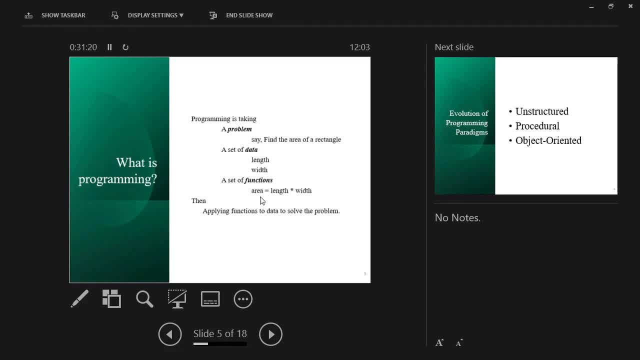 these things now we'll start with programming so i hope like you know what programming is so programming usually is you have a problem that you need to solve and say for example the problem is you need to find this is a very simple problem you need to find the area of a triangle now how do you we look at this simple problem and we'll see how do you solve this problem using procedural programming and how can you solve this problem using object oriented programming so we'll write the code in both cases as limited by this it may be decided so we will start with programming so we'll start 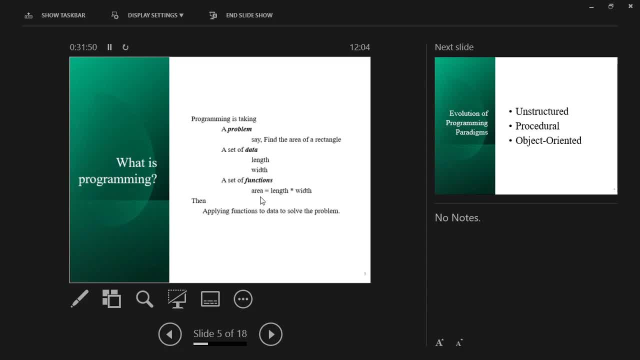 then we see like what is the difference between the two so you start with the problem the problem in this case is to find the area of rectangle and in order to solve this problem you need a set of data so what do you need to find out the area per rectangle you need the length of the rectangle and the width of the rectangle and then you use a formula or a function to find the area so how do you find the area you just multiply the length with the width in this that's how you get the area so in programming what you do is you start with the problem and data you first 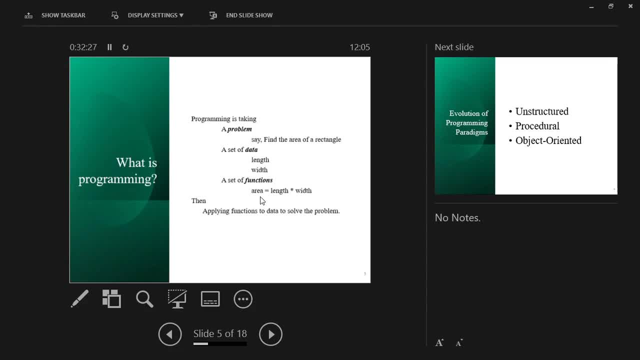 devise an algorithm for solving that problem and then you solve that problem you write code for it you code those functions in order to solve this problem this is what programming is 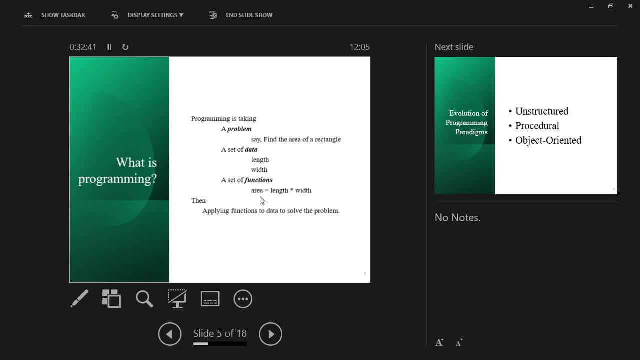 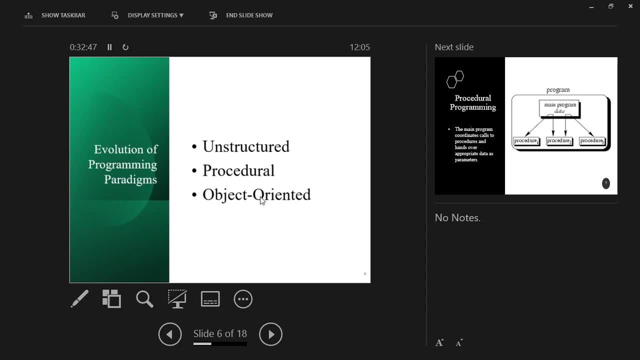 now programming this is what it is but over the years as we discussed it has evolved in the beginning people used an unstructured approach towards programming okay so they only thought of a single problem and they would solve that problem just that problem they would not they would think as if all the resources are available 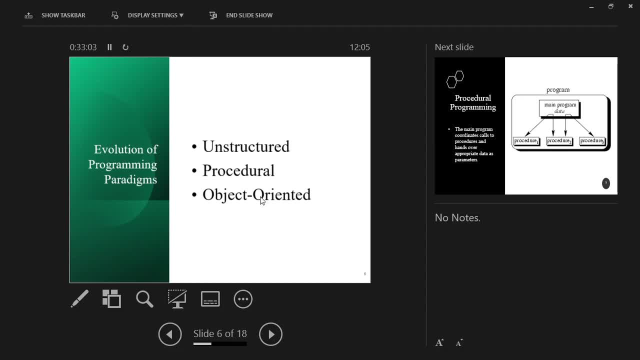 to them in order to solve that problem by the way one like limitation of single tasking was 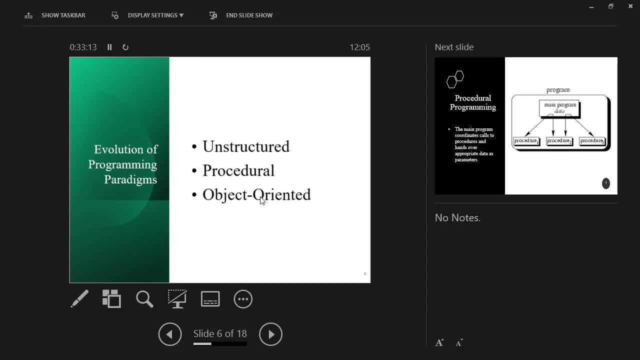 it cannot do something else for example if your computer is printing a document so while it is printing that document it can not do anything else so you have to wait for that printing to finish and then you would be able to do something else that that is how single tasking environments used to be and in those days like 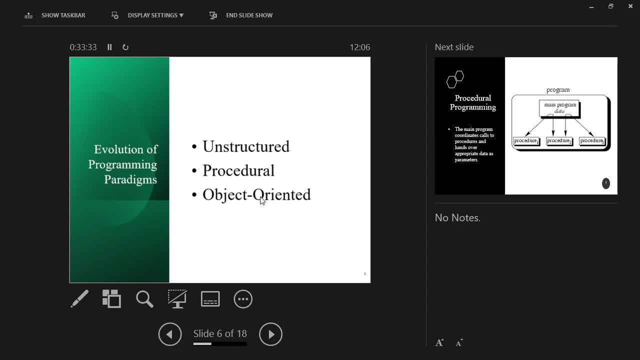 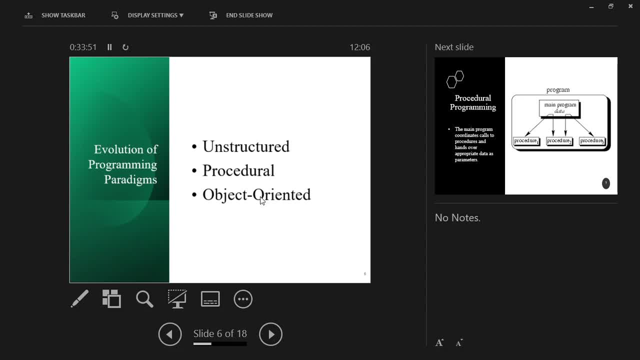 day so people used to reserve computers for themselves and then during that time they would they were 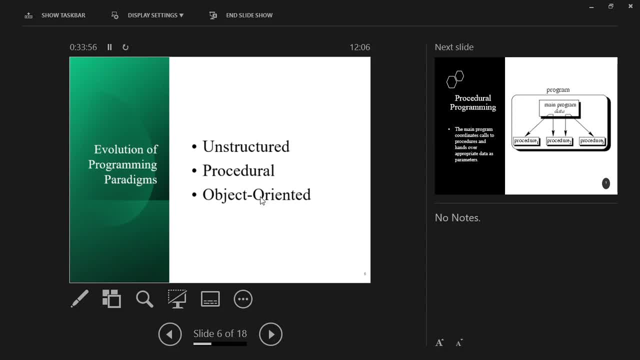 supposed to finish their task and all that so in those days programming was unstructured there was no structure to it but after a file may yeah file be named say so initially like if you if you have 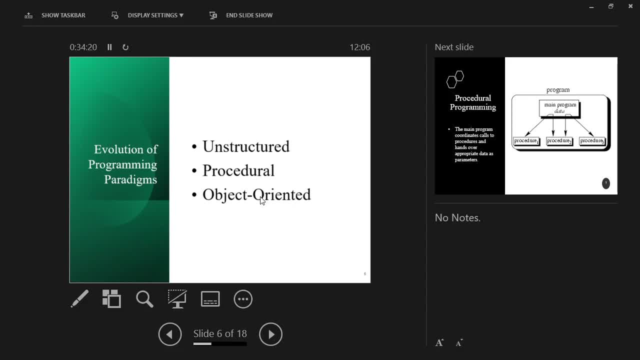 read a about the history of computing so initially programming to have a keyboard or in jesus 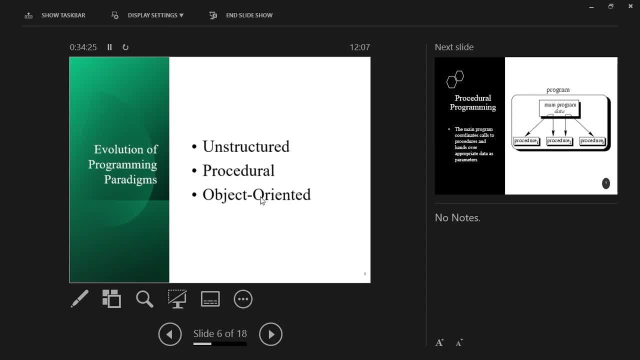 reasoning so they're initially people used to do punch card programmers programming so people would take cardboards small small cardboards and punch holes on them so the holes or the absence of a hole would represent one or zero because those machines were kind of electromechanical machines so holes or a no hole as one or zero interpret that that would be one instruction for programming so that was the history of computing so that was the history of programming 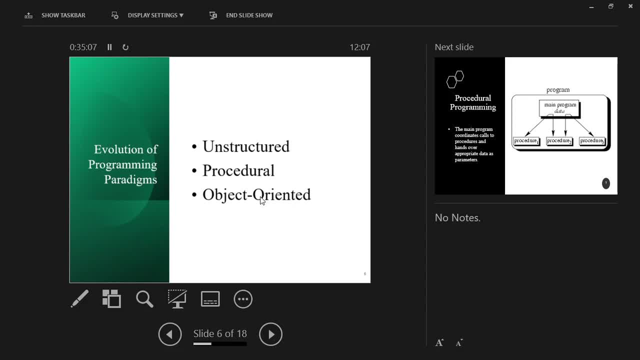 right now like nowadays we are used to uh electronic computers so jesus brother dad man jesus jesus 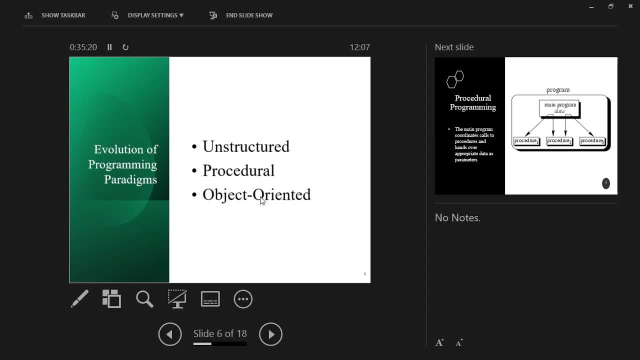 touch that program and it used to be in the form of punch cards so they can that was those days so in those days things were unstructured then procedural programming the idea of procedural programming was introduced programs should have some organization we should have blocks of code that should that can do something specific and then we should be able to call different blocks of codes or execute them we should give some we should be able to give some input or arguments to a block of code or we should calculate some output or result and then we have object oriented 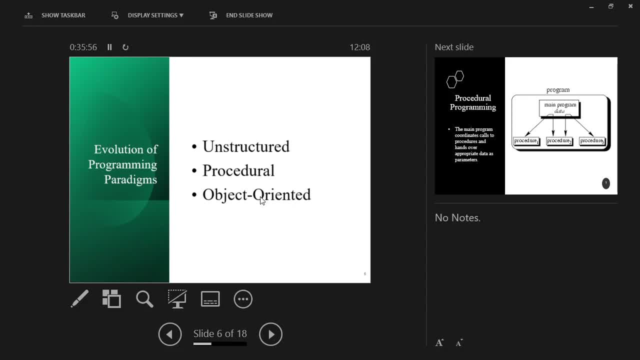 programming okay now these are not all the possible programming paradigms programming paradigms means different ways of programming so unstructured is no longer here so right now we use procedural programming then we have object oriented programming then we have functional programming functional programming is a little different okay functual programming idea is that all your programs should be just functions a function to call another call third call fourth call fifth call and then you will say what is the difference 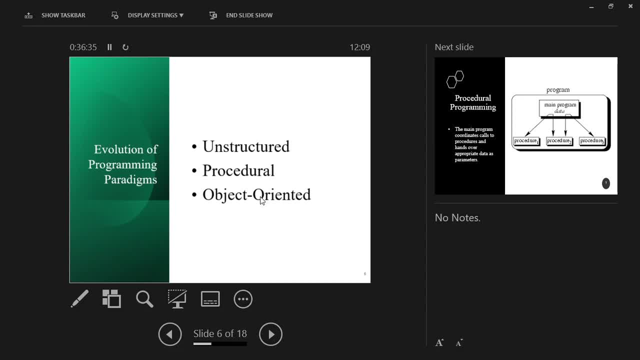 between procedural programming and functional programming so in functional programming like all programs just function and function work is that they should not mutate the data they should 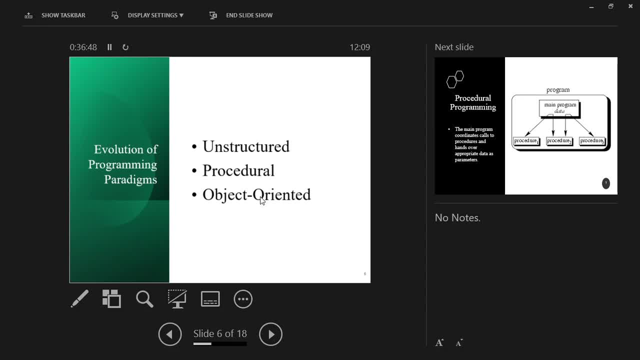 The data you are transferring to the functions, they should not affect that data. 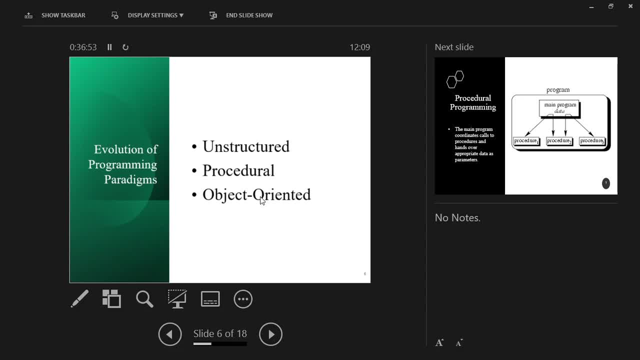 By using that simple data, they should calculate some output, but they should not modify that data. 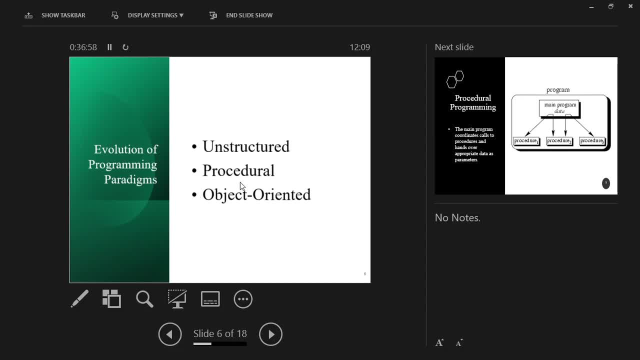 In procedural programming, when you write a procedure or a function, you give it some arguments. The function can return its output value as a return value. Or the function can give you the output by modifying the arguments you are giving to it. So if you remember, in programming, you may have read the concept of pass-by-value or pass-by-reference. That you can pass the arguments to any function in either of the two ways. 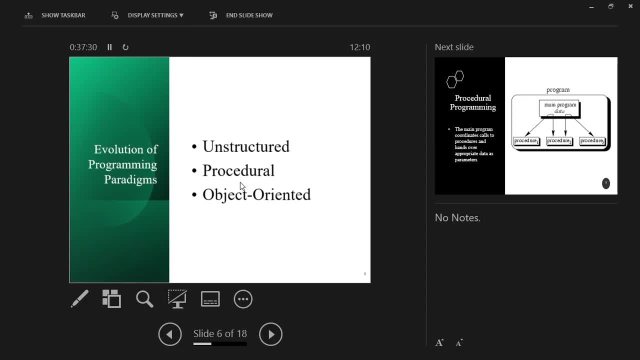 One, pass-by-value. What happens to that is, the copy of the data you are passing to it goes to that function. The other is, that you pass data by reference. 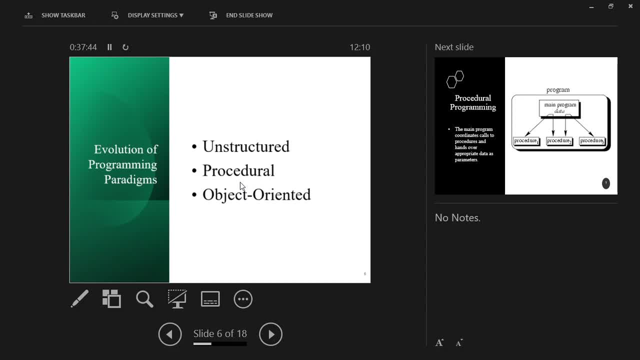 That you are giving the address of the argument to the function you are calling. Now, this is useful as well as it can be problematic. 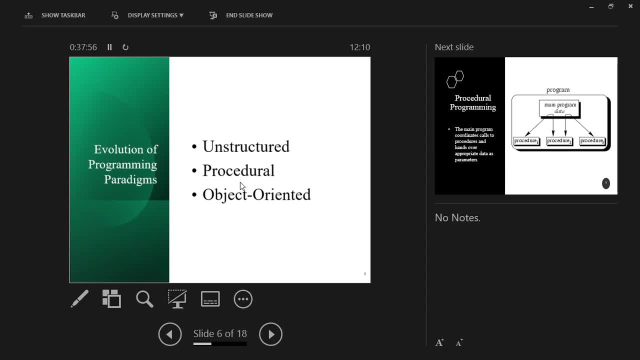 Useful in the sense that you can pass huge amounts of data very efficiently. You don't have to make a copy of it. 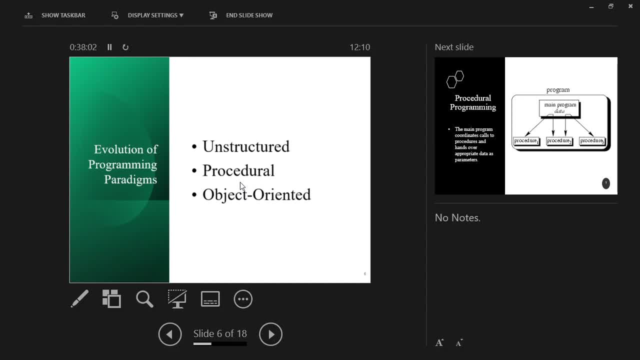 Copying is a slow process. And the dangerous thing about this is, 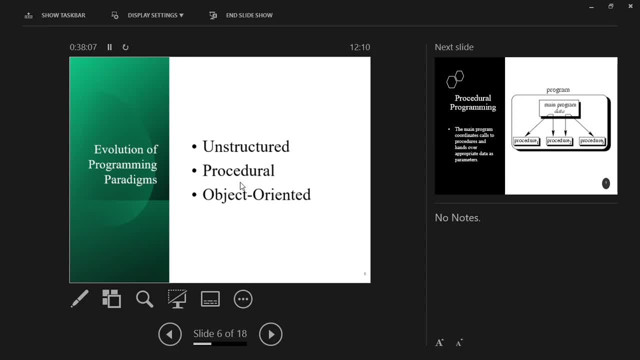 the callee function, the one you have called, it can change the data. The original data. 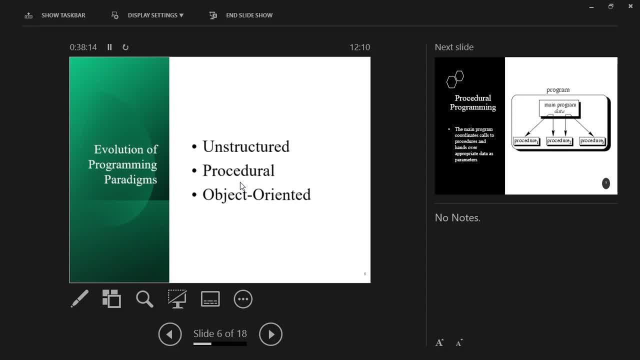 So sometimes you do it deliberately. You want to get the output in such a way, that you just give the address of the data, and the function that has to operate on it, it modifies that original data and gives it back to you. Okay? 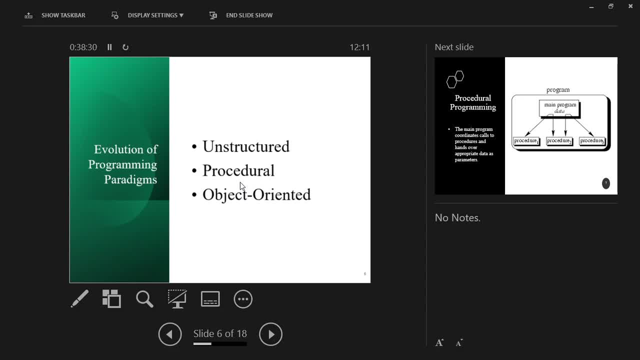 So sometimes you do, you transfer data or you pass data by reference on purpose. Okay? You want the function to change your data. 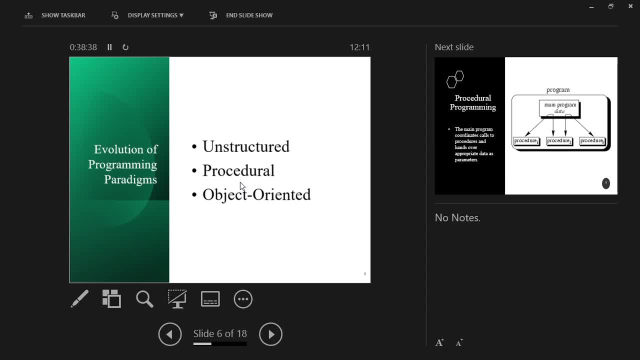 The output, if you, uh, if, uh, if you return it, then the return can do only one value. Okay? It can't do more than that. 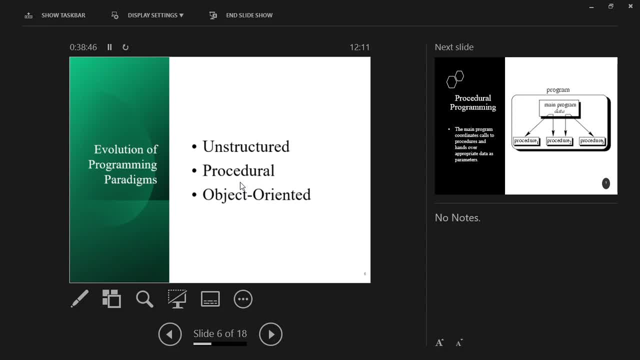 But if your output is more than one value, then you use the method of pass by reference. Okay? 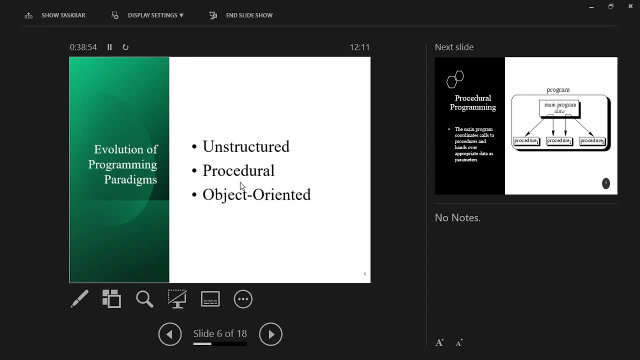 Now this is, this is one, this is, this is the, you, you can say this is the distinguishing feature of say, procedural programming and functional programming. 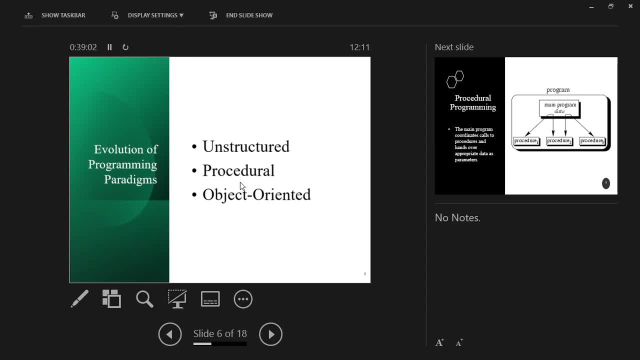 Both have functions. But in procedural programming, functions can mutate the data. 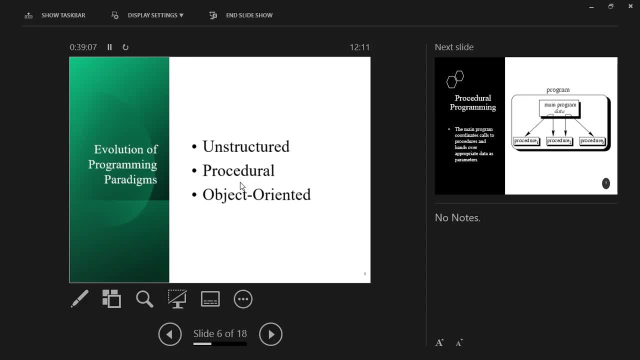 In functional programming, functions do not mutate the data. They, they cannot change the arguments. They cannot change it. 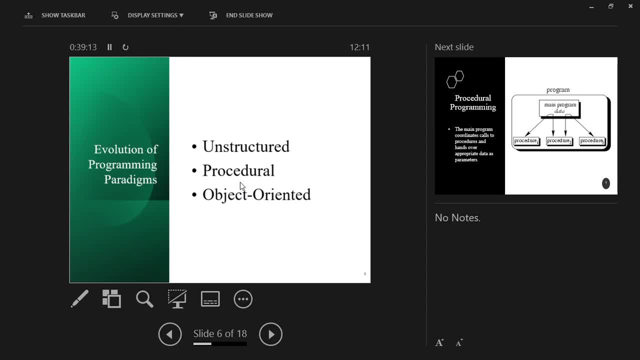 They only use it to calculate, uh, to, to, sorry, to calculate the output, to determine the output. Okay? 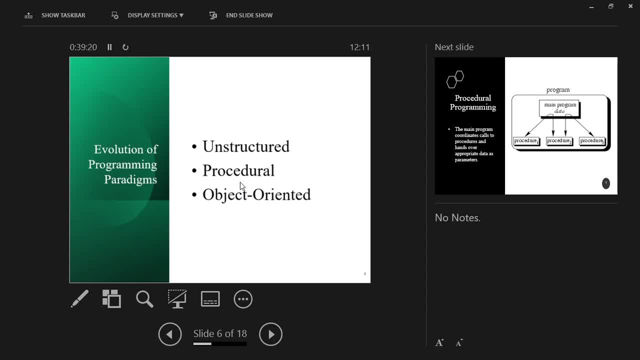 The second is that in functional programming, ideally, you should, it is, it is, this is, the aim is that you should have just function calls. 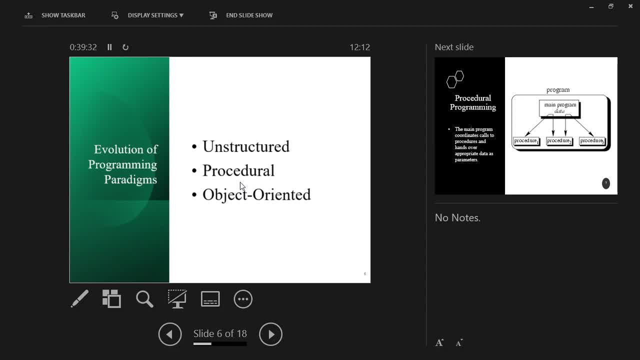 You should not have loops and if else, and this kind of things. The less you have, the better it is. You should only have function calls. Okay? 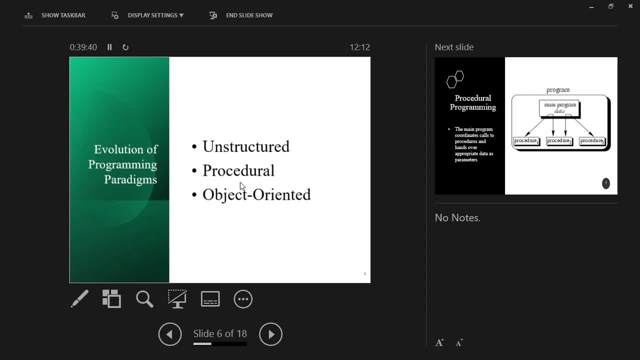 Through a sequence of function calls, you should be able to solve any problem. So that is what the, the, the, the role of functional programming is. 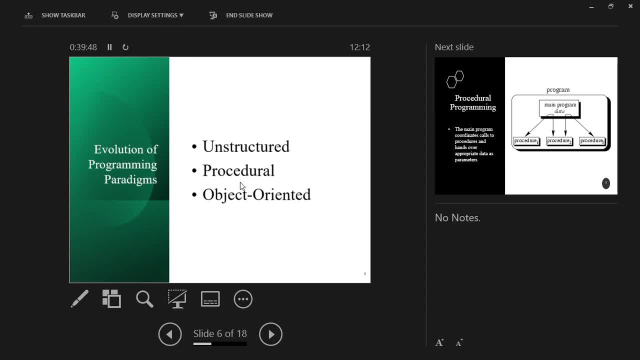 But we are not talking about functional programming. But this is the way of functional programming that since we are talking about programming paradigms, this is not an exhaustive list of programming paradigms. Okay? 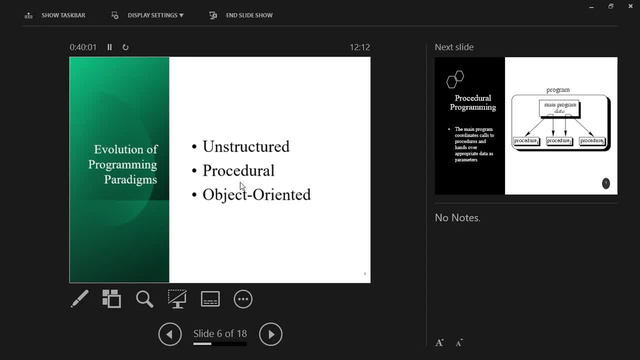 There are more programming paradigms and some are also evolving. 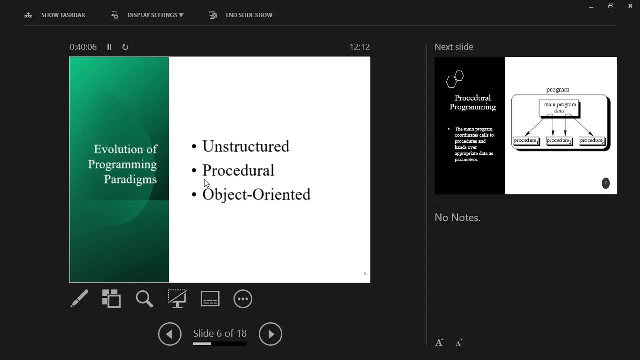 So there are many ways, but we will only be, like, using, 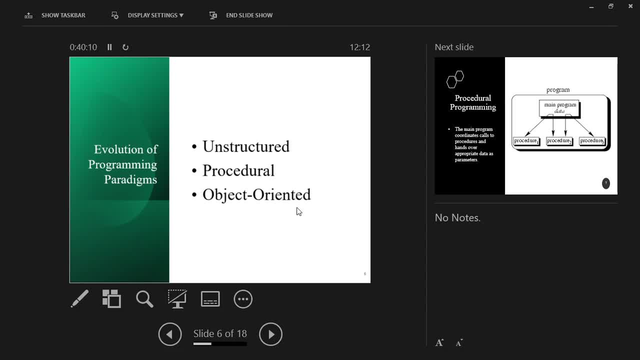 we will predominantly be using object-oriented programming in this course. 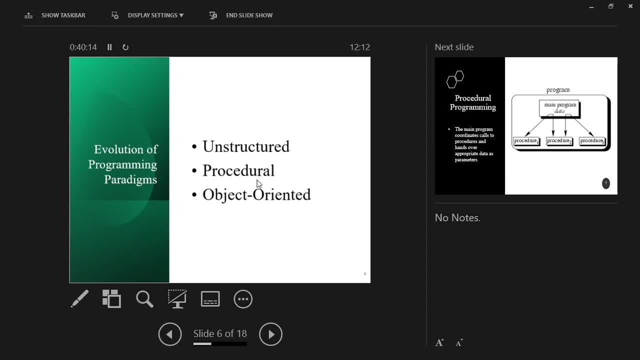 Procedural computer programming, we use Karchakin, but you can also use that here as well. Okay. What is procedural programming? So you have this idea. 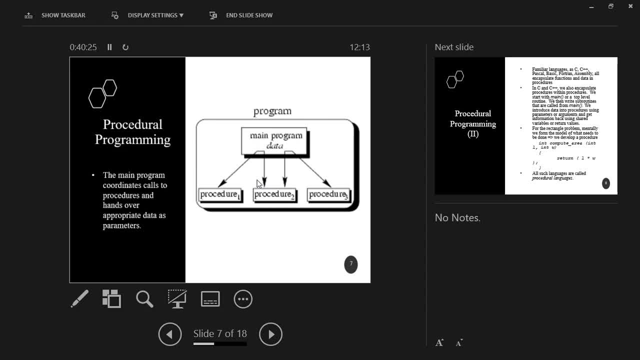 In procedural programming, your goal is to write as many procedures as required. You have a problem, you divide that problem into sub-problems. For each sub-problem, you write a procedure or function. And then from the main function, you just call those things. Okay? 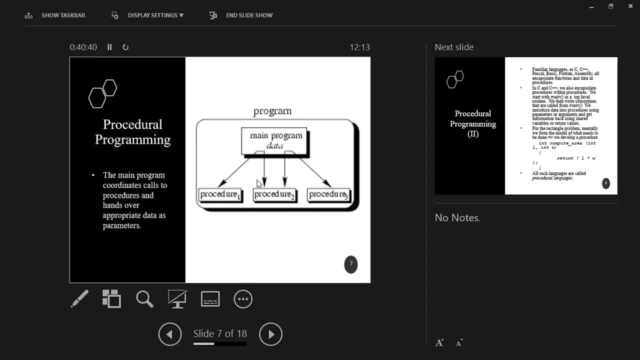 You call those different procedures in a sequence so that you can solve the big problem. Okay? That is how it works. 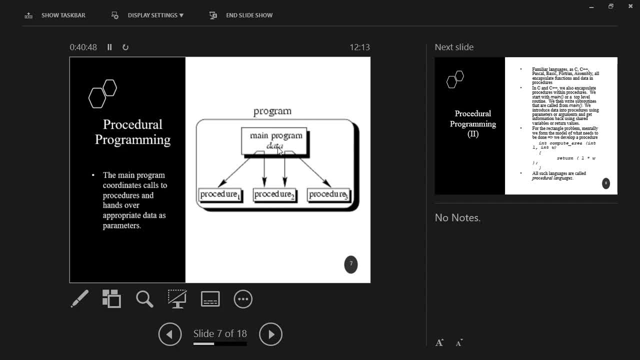 Procedural programming or functional programming is the same. No, it is not the same. There is a slight difference. There is a similarity as well. 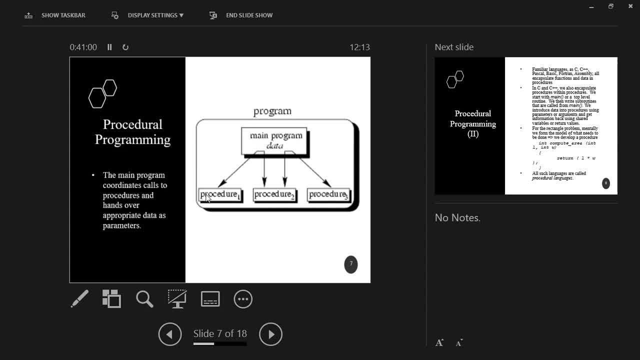 The similarity is that in both, we have procedures or functions. And different functions can call different functions. That is the similarity. 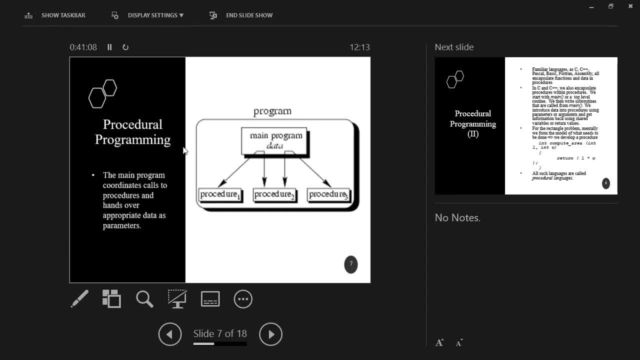 But there are differences as well. So one difference was that in procedural programming, when your main program passes data to procedure 1, procedure 1 can change this data. In functional programming, procedure 1 cannot change this data. Okay? So those are the subtle differences. 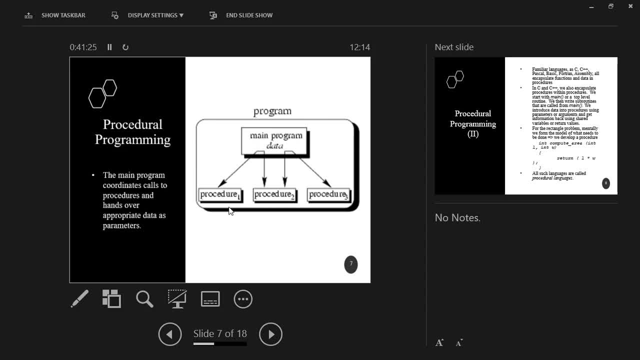 The other difference is that in functional programming, the aim is that you should solve the problem by only making function calls. So the other code is if-else or if-else-if or switch-or-butt-else. So ideally, you should not have that code. Okay? You should only have function calls. That is the idea. That you just have to call one function, then the other, the third, the fourth, the fifth, the sixth and your problem will be solved. Okay? Just by function calls. Yes? Yes? 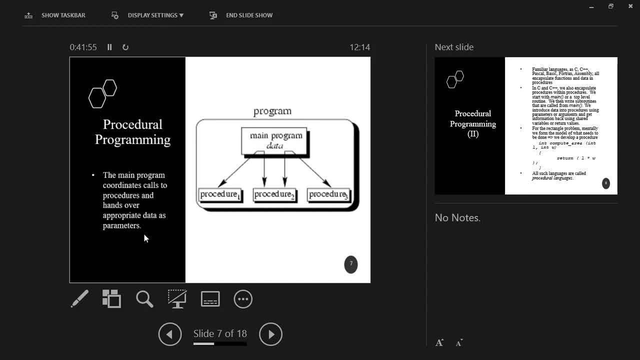 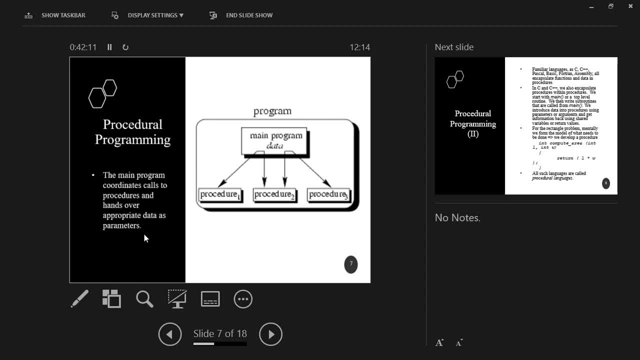 Google form is different. It is different. 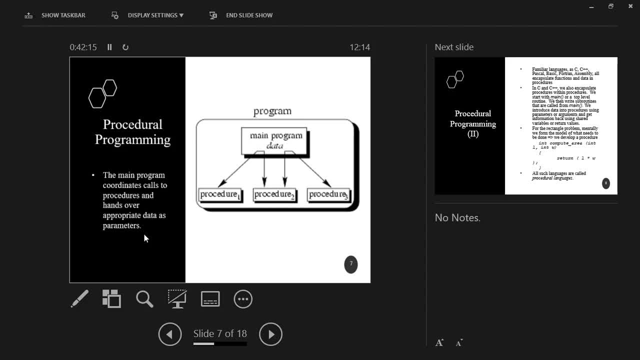 Maybe you cannot understand what kind of analogy you are trying to give. But that is different. 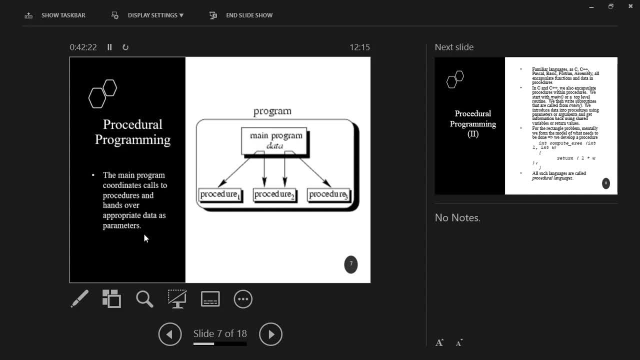 Functional programming is more, is closer to mathematics. For example, in mathematics, if you have to calculate the sine of an angle, you just call the sine function. Okay? 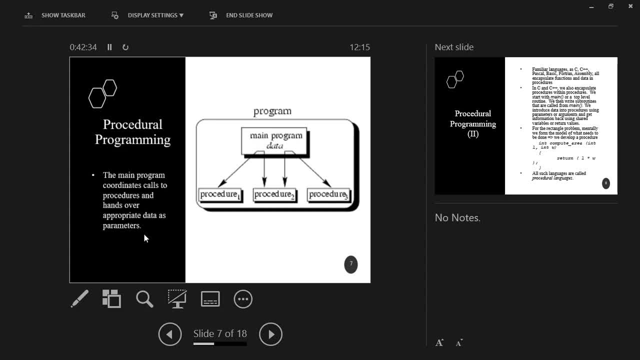 If you have to calculate the tangent, you take the ratio of sine and cosine. So, tangent will be known. Okay? 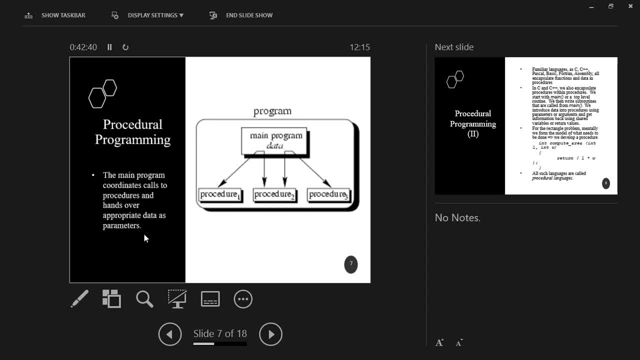 The idea is that you should be able to solve any problem using a sequence of mathematical functions. And then you code those mathematical functions. Okay? That is, function calls only. So, functional programming is more close to mathematics. Okay? That is, it is inspired from mathematics. In mathematics, we can solve any problem by defining different functions and then calling those functions. Okay? Okay. For now, do not confuse this. Okay? 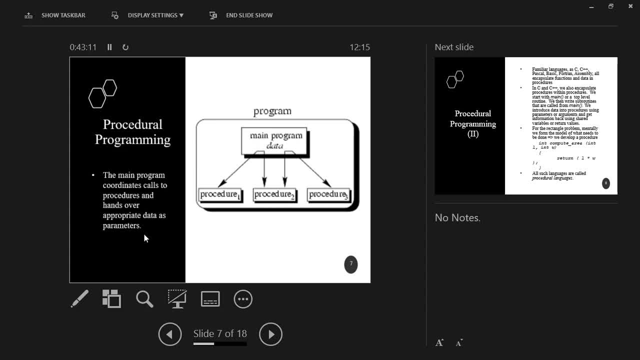 Let us say, forget about, you just remember functional programming. Listen to the name, yes, this is also a programming paradigm and it is different from procedural programming. And one difference is, one important difference is that in procedural programming, procedures can modify the data, the input data that they get. In functional programming, they are not allowed to. Okay? This is what procedural programming is. Now, in this. Some. There are some losses. One. 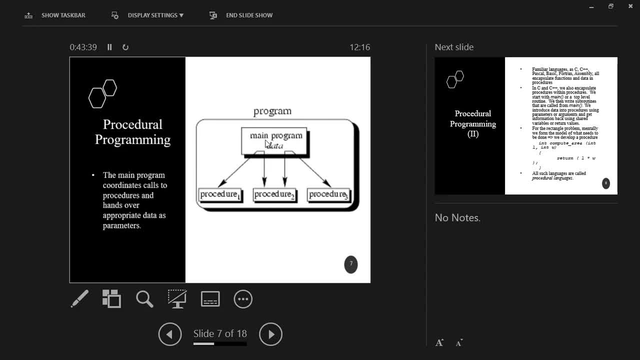 One problem is like, I do not know whether you have talked about global variables in programming or not. Global variable, do you know what a global variable is? So, one. There are local variables and there are global variables. 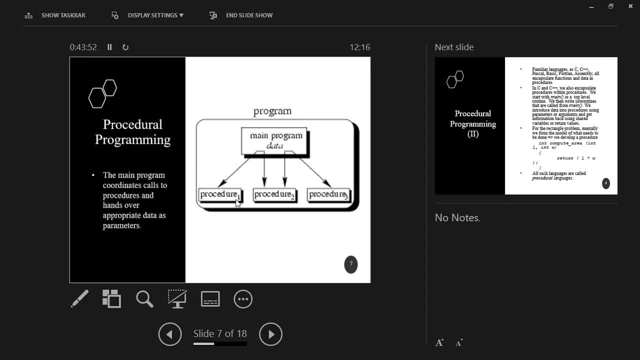 Local variables are visible only in a particular procedure or on a particular block of code. So, if you declare a local, a variable inside a for loop, that variable is a local variable to that for loop. You cannot access that variable. Similarly, if you declare a variable inside a procedure at the procedure level, function level, so that variable becomes a local variable to that procedure. You cannot access it in procedure 2, you cannot do it in procedure 3, you cannot do it in the main program. Okay? 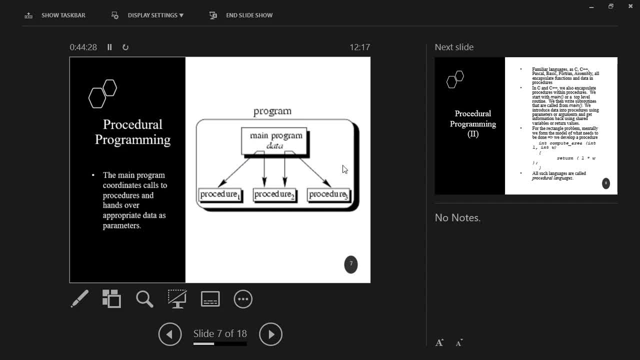 Global variable. What is global? A global variable is accessible to all procedures. 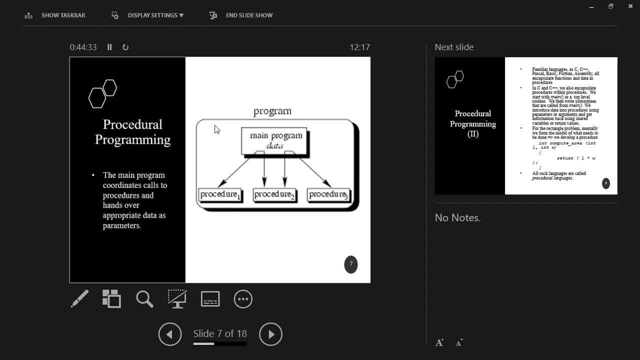 If we declare a variable at the file level, i.e. above the main program, we declare that variable. Okay? 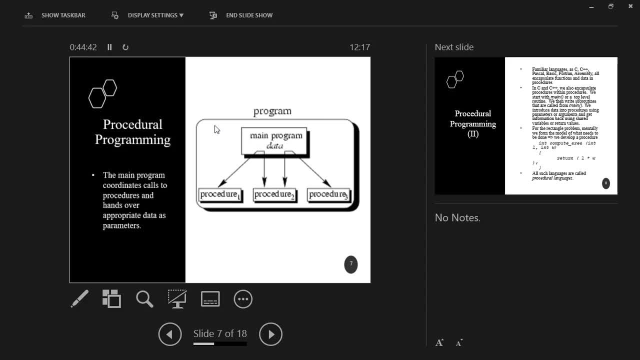 Do not declare it inside any function. Declare a variable outside all functions. That variable becomes a global variable. Now, that variable is accessible to all these procedures or functions. Okay? 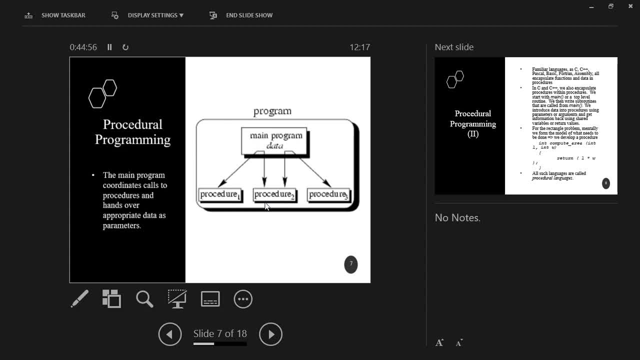 Why do we have global variables? So, global variable is one way of sharing data among functions. 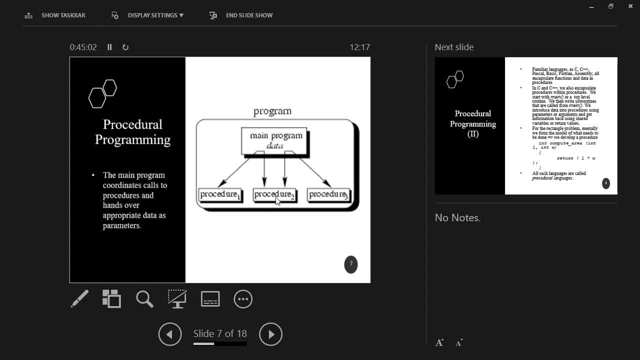 If you want. All procedures can share data among functions. So, you can use global variables for that. Okay? You can use global variables for that. 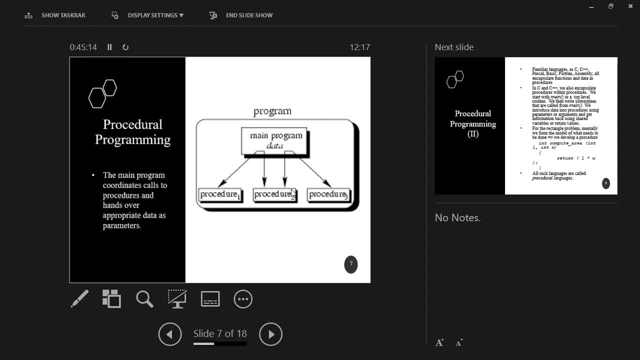 Global variables are useful, but they can be problematic as well. Okay? 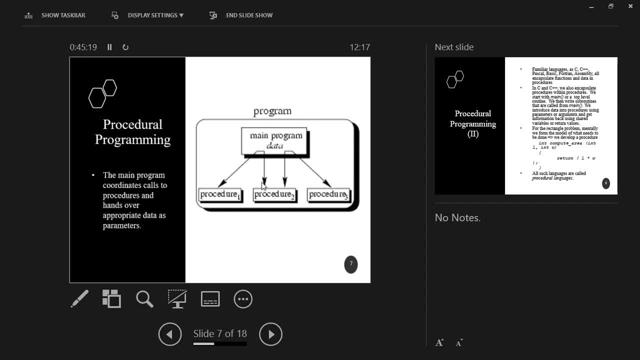 Useful in the sense that sharing data with all procedures becomes easy. Problematic in the sense that any procedure can change the global variable. 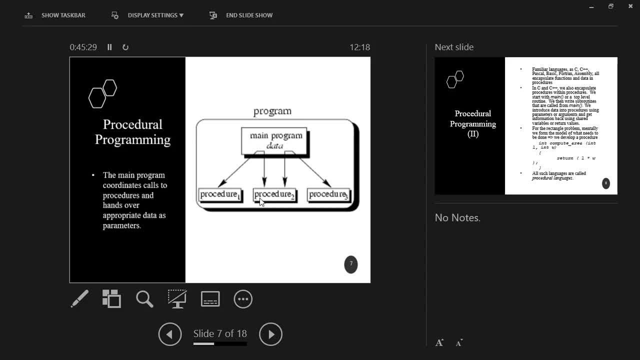 And if you run into a problem. If you have some bug in your system. In the program. 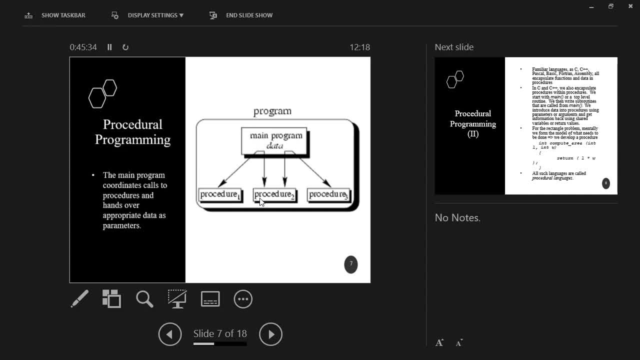 So, the most problematic bugs involve global variables. Because it is very difficult to track that which function is modifying the global variable. And how it is modifying it. So, to locate one problem, you have to look at all the functions. This is not modifying it. This is not modifying it. This is not modifying it. Okay? 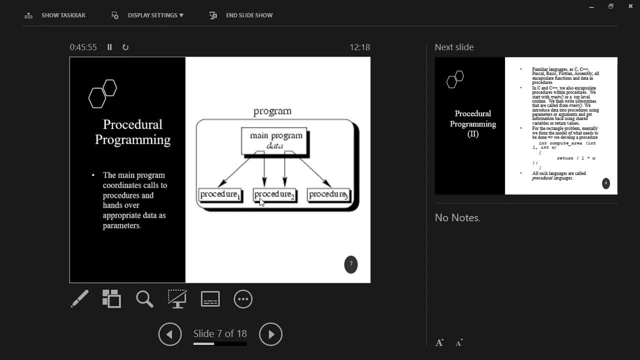 So, global variables have their benefit. And they have their problems. Okay? 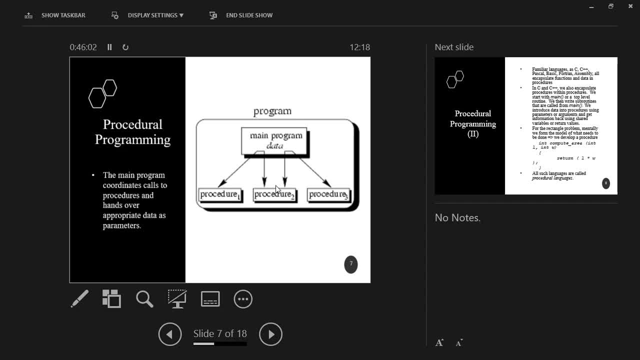 So, now issues like these. They prompted that in this main program. Data and procedures or functions that operate on that data. 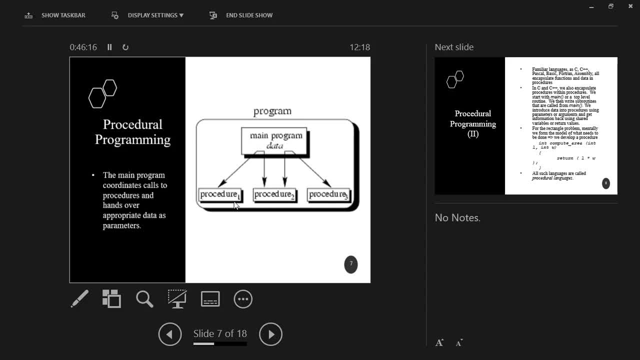 So, function is separate. And for that function, data is coming separately from somewhere else. They are not close together. Okay? 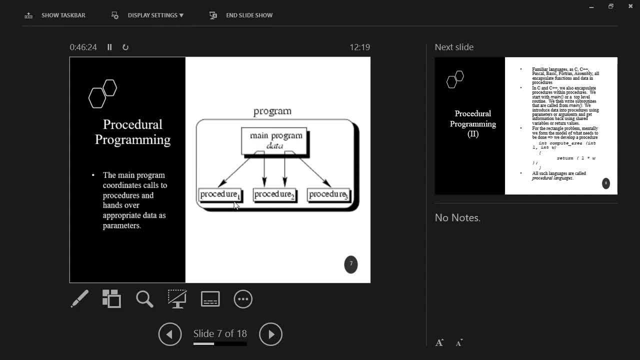 There is no relation or connection between them. Now, this is good in some sense, in some ways. And this is not so good in some ways. Okay? 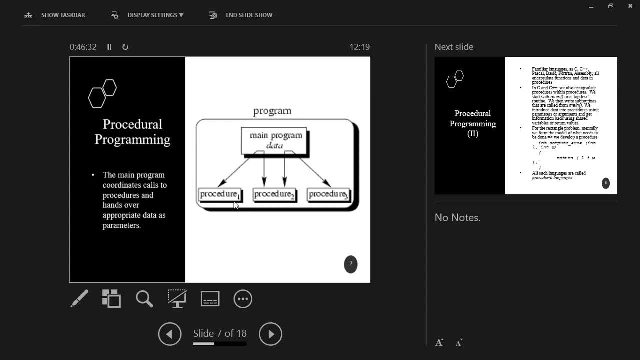 When there is no relation between the data and the functions modifying the data. 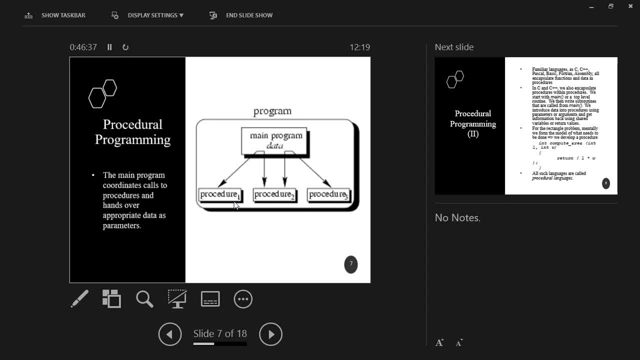 Then it is at times it becomes very difficult to track which function is modifying which data. Okay? 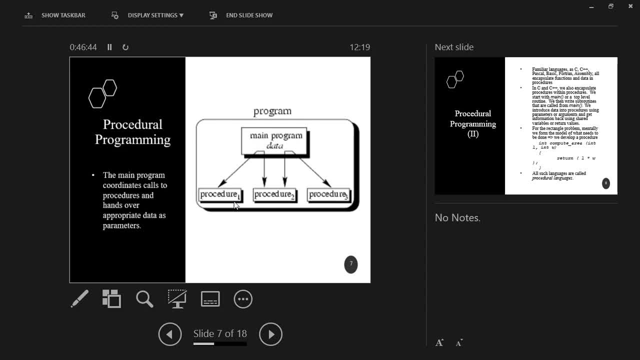 And if you have a bug that involves such functions and such data. So, those bugs are very difficult to remove. 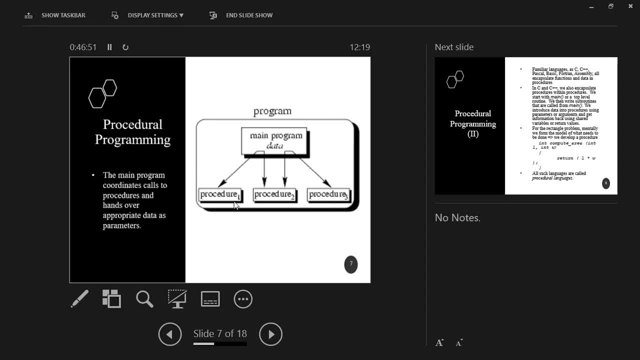 Now, what object oriented programming did was they brought the two of them together. Data and the functions that operate on that data. They should be close together. They should be encapsulated. They should be in one place. Okay? 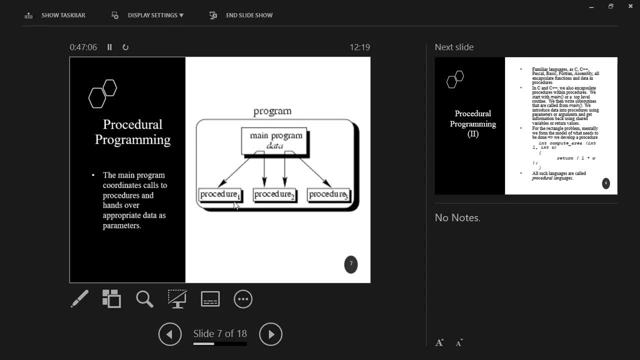 Data and the functions operating on that data. They should be in one place. They should be enclosed in one package. That is called data encapsulation. What does data encapsulation mean? That data and the functions that operate on that data. You encapsulate those two things together in a single module. In a single class. Okay? 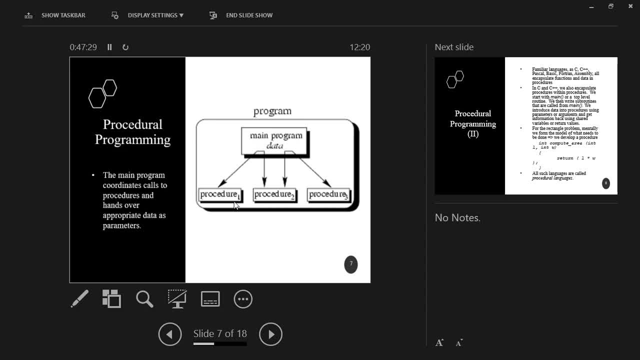 So, that happens in object oriented programming. But in procedural programming again by studying or discussing object oriented programming. We are not dismissing altogether procedural programming. That it is very bad. Do not use it. It is not like that. You will continue to use procedural programming in different languages and in different situations. In some places maybe object oriented programming would be more suitable. 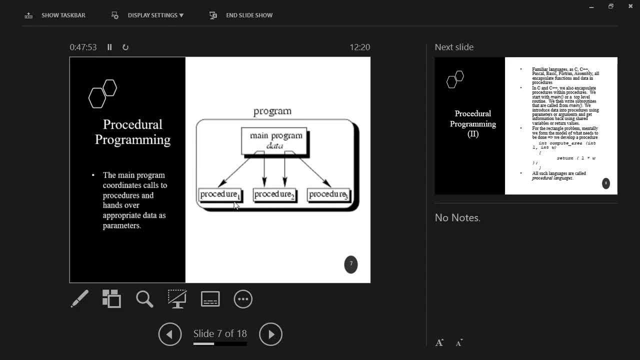 There you can go the object oriented programming way. Okay? 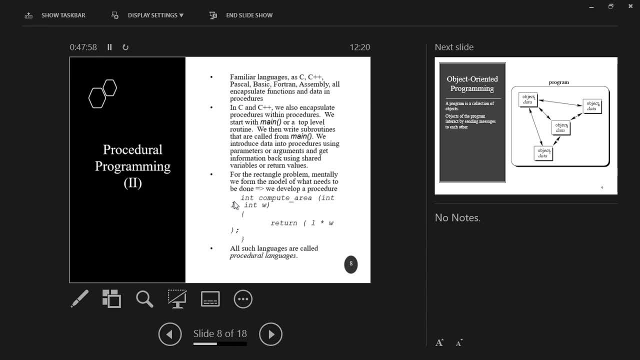 Many languages. C, C++, Pascal, Basic, Fortran, Assembly, C sharp. You can use object oriented programming. 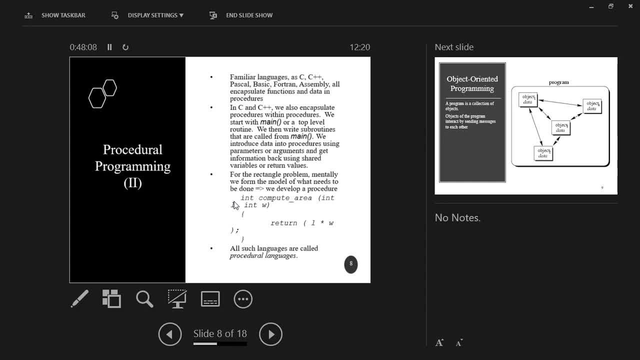 Java is a purely object oriented programming language. You cannot do procedural programming in that. Python supports both object oriented programming and procedural programming. 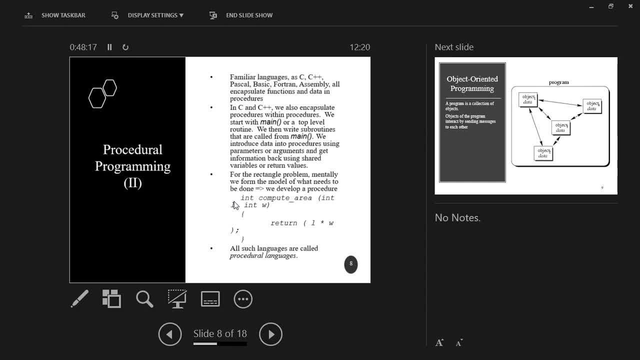 In MATLAB you can do both procedural programming and object oriented programming. 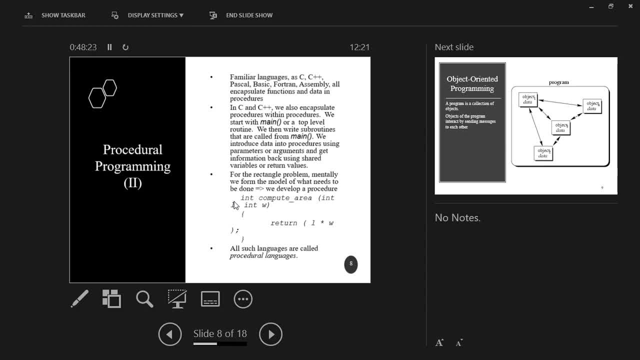 Linux is an operating system. And it is, it is, it is built, it was built using C. So, in Linux you only use C programming language. That means, Linux is an operating system like Windows. Linux is just like Windows. So, it is not a programming language. But Linux was predominantly built using C. And the people who build Linux they do not like object oriented programming. Okay? 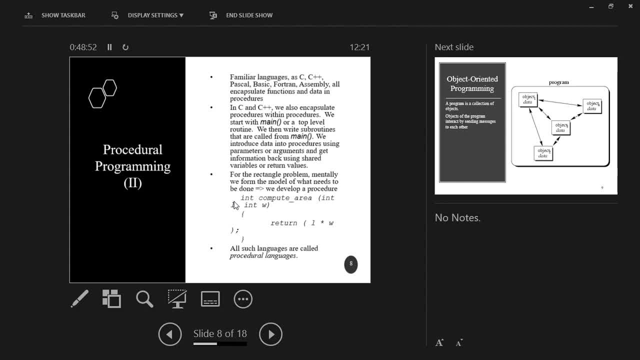 They neither like C++. They like non-object oriented programming. 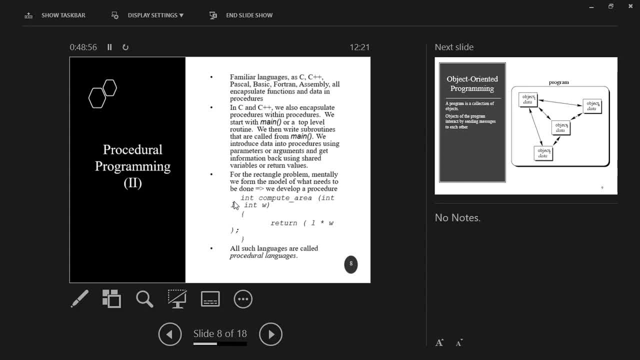 So, the creator of Linux, Linus Torvalds, I guess. You can see him on YouTube. You will find him. 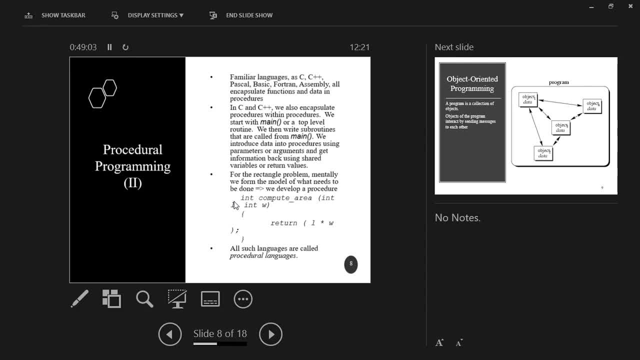 He is not, and he has a community. There is a community which develops, which maintains the Linux kernel. Okay? The kernel of the Linux operating system. 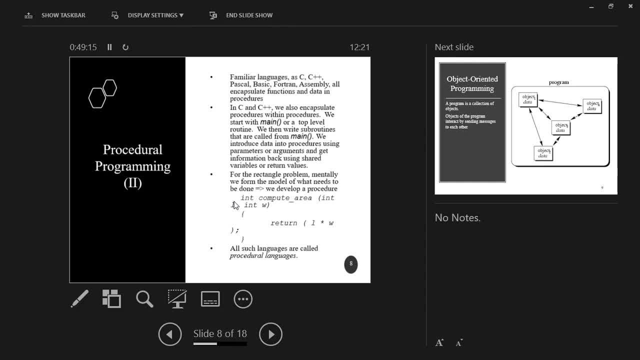 The permanent memory resident portion of an operating system. So, a community is maintaining it. 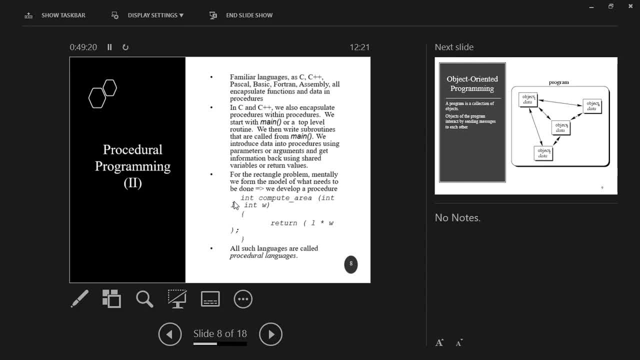 And that community is not a fan of C++ or object oriented programming. So, they are hard core procedural programming fans. Okay? So, again, the point that I initially made. A OOP does not mean that procedural programming is bad. This is just another way of programming computers. And it is useful to learn about this way to program computers. Okay? Okay. 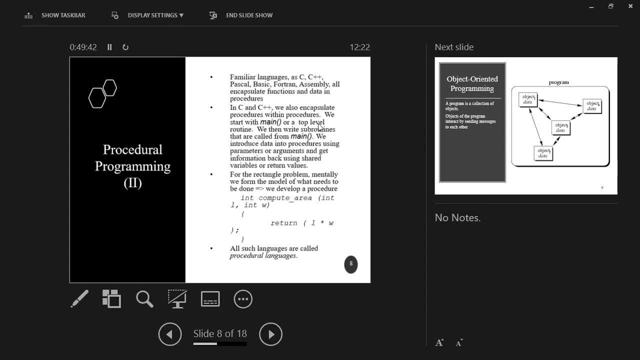 Now, we have discussed it. That C, C++, whatever languages, procedural programming languages. 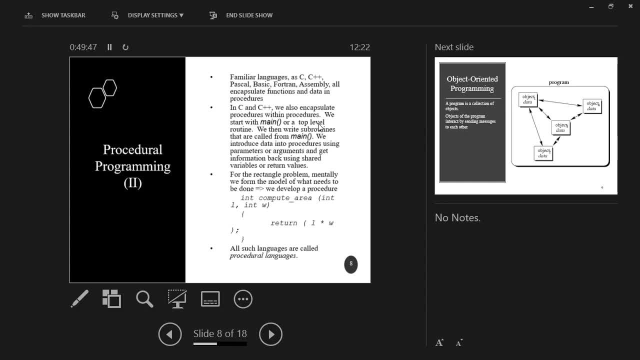 In these languages, you have the main program. And the main program then calls others. Other. You have the main function. And the main function then calls other functions or procedures. Okay? You call it from there. 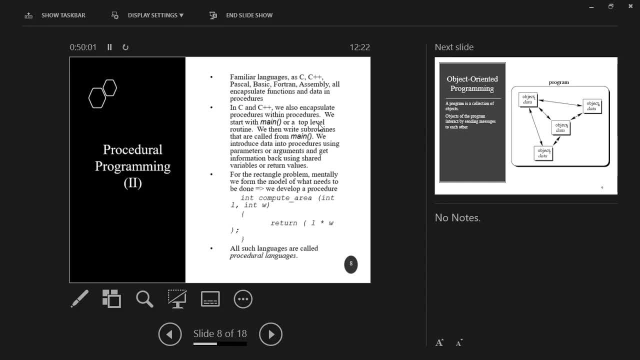 So, you can think that the main function encapsulates the other functions. Whatever functions are present in your program. The main program encapsulates all the functions. Okay? 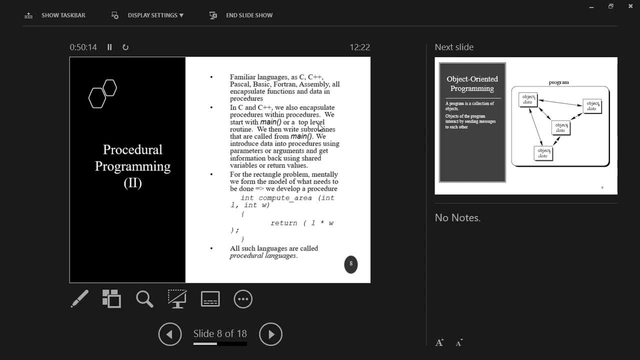 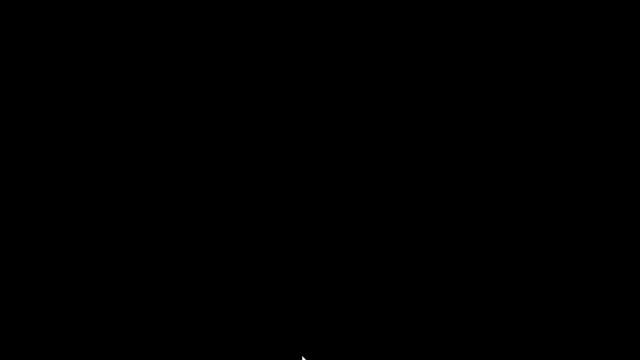 So, how would you solve the problem of calculating the area of a rectangle. Using procedural programming. Okay? So, how would we do that? Again, this is very simple. 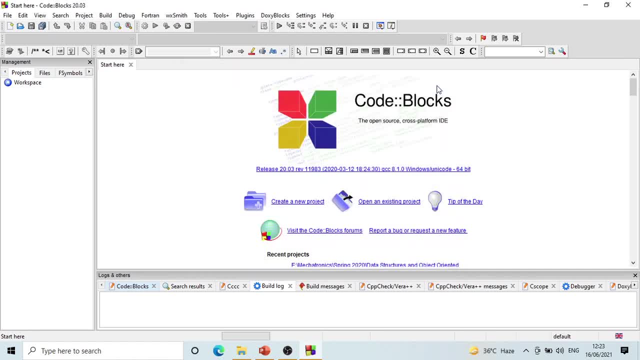 Okay? But I want to demonstrate the object oriented way as well. So, let us write that code. Okay? 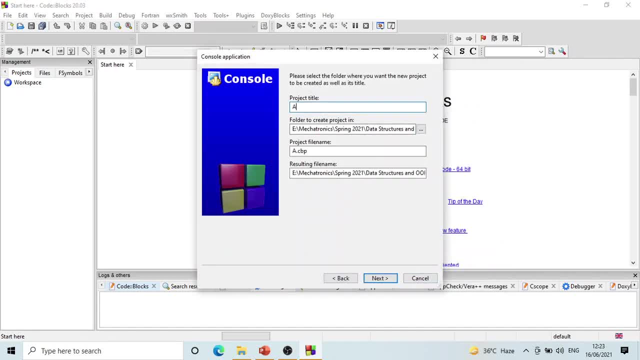 So, let us create this project. Say, this is rectangle area. Rectangle area. Okay? Okay. See it. 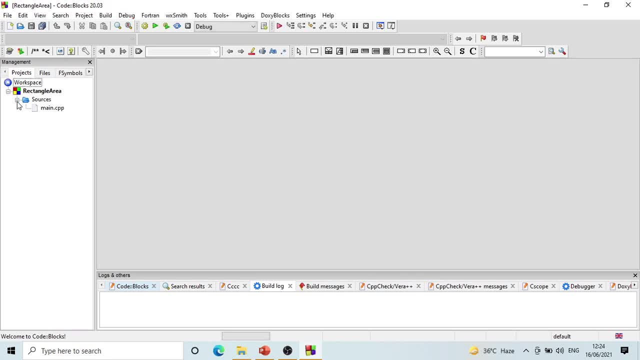 Okay? See it? See it? Yeah. 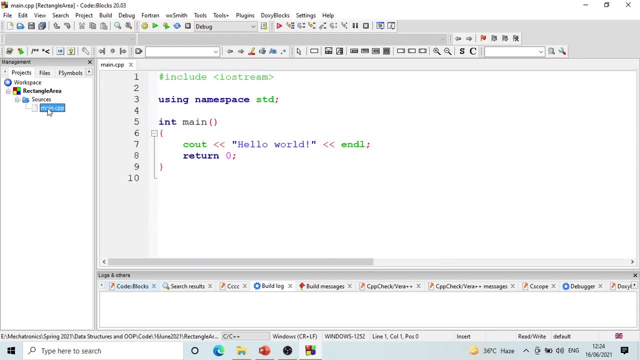 So, the was out in the nature room in that no object. the word is. As you can see. You don't have to write this. You don't have to write this. I see. You do not have to write these too. increase the font size just a little bit okay he already sized 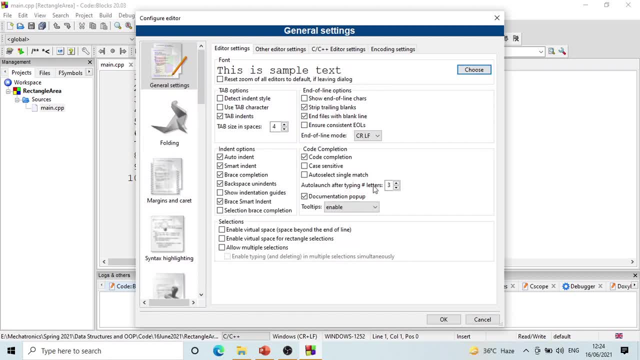 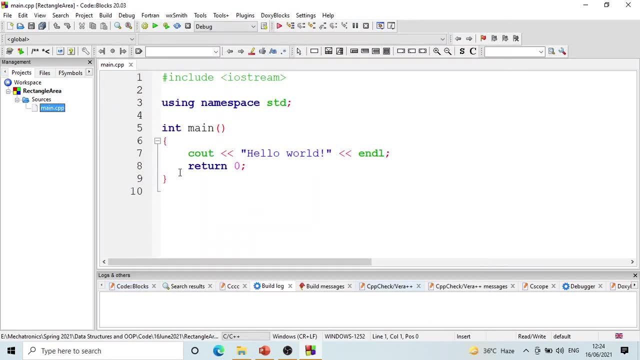 okay so let us make it 18. so if you if you want to find the area of a rectangle using the procedural programming way to you need to write a function in order to write the function you need to write a function prototype in order to inform the compiler that i am going to write the function of this name so let us find the area of rectangle so we need to write a function that would return as a double value double find area 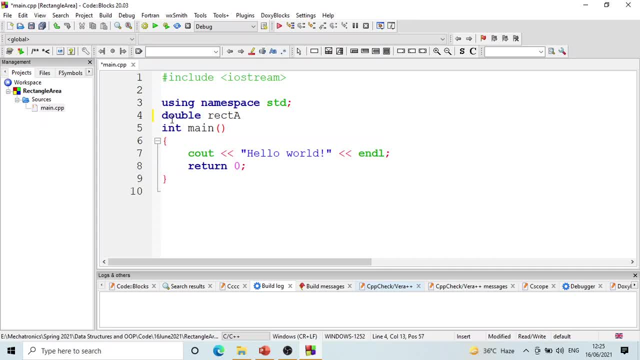 so rectangle yeah rect area okay and it would receive two arguments two double values this is a convention asha these are conventions 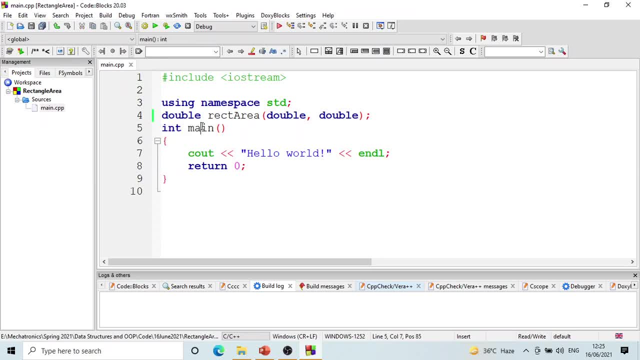 usually other if your if your function name has a single syllable so you just write it in all small caps either main for example this small caps but if your function has two syllables so usually this is a convention it is not a requirement 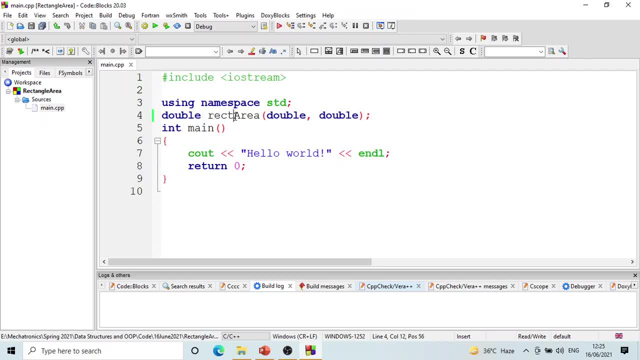 that the first letter is in small caps and the second letter is in uppercase letters right 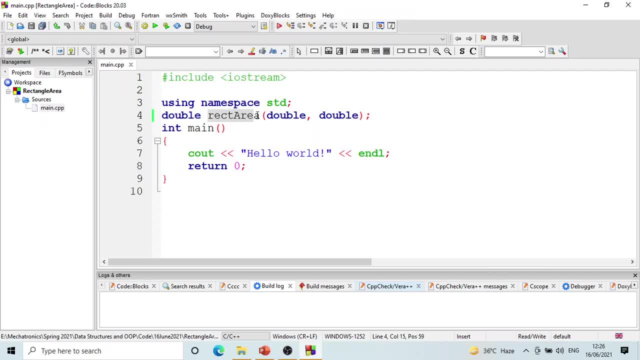 the question was that why did you name this function like this that the first one has r small and this is a capital 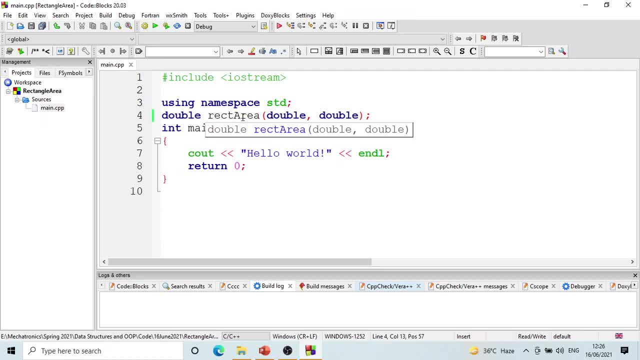 this is not a requirement from the compiler this is just a convention it is a tradition 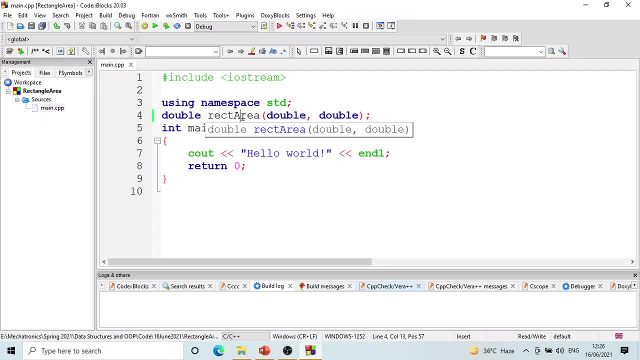 those people who program in c and c plus plural in other languages as well so the preparation is that if your function name has a single syllable 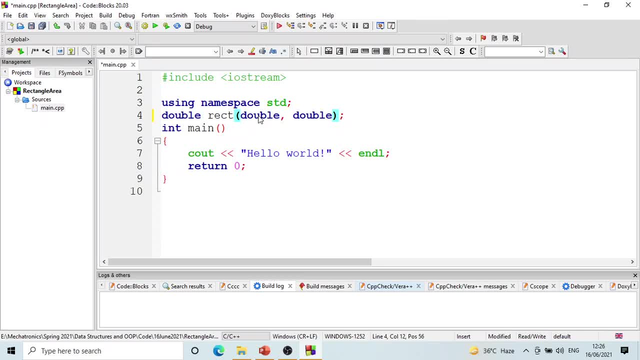 so keep it small letter lower case if it has two syllables the album also is it the word called ic 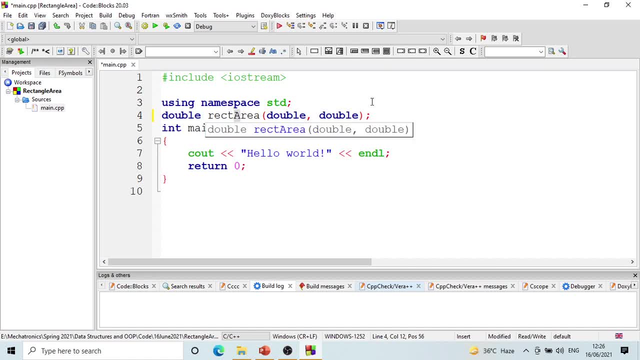 should start with a capital letter that's the convention otherwise you enter as you like it increases the readability okay so you know that these two different words these two words have been made together so that the game code readability is also very useful concept so in the computer or something anderen word something else is identified which is called each other its notHow it might not be so called that way you can call it word of a type of Default this creative word in in interacting with this and you create specific variants for nodeutz this code readability is is also made to check uses their constance because you know that 이름 of the Ughar this is also the 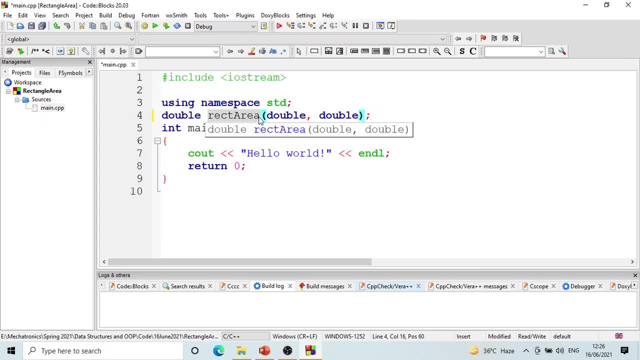 readability is is also a very important attribute of your code that your code is easy to read and easy to understand 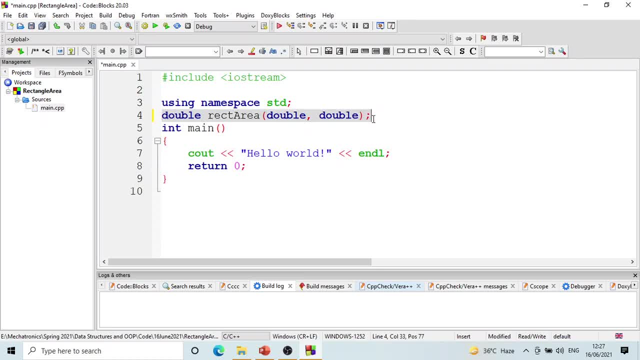 ok this is the function prototype ok I hope you remember function prototype so this is the function prototype now let's implement this function let us write the body ok so now we need to provide names here as well length and 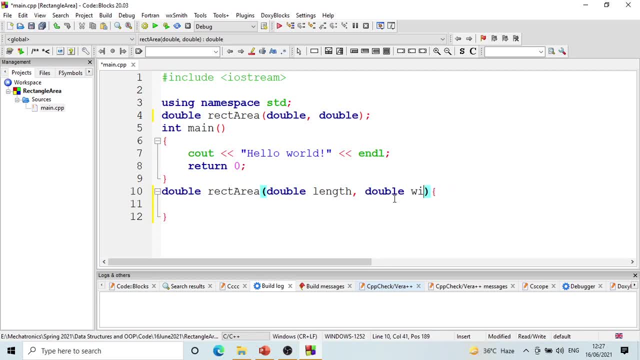 width ok or you can use this simple word double w and l say l for length and w for width so how you have to calculate the area return l multiplied by w that is how you find out the area 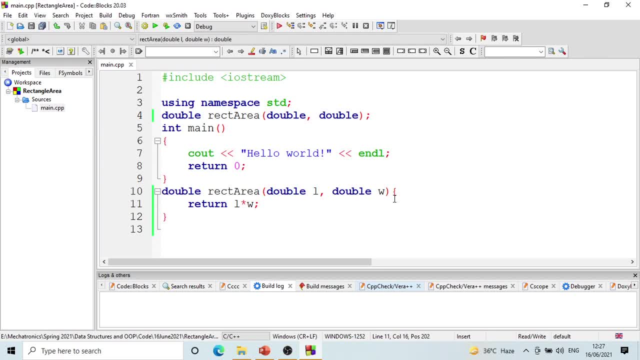 this is the procedural programming way of finding out the area of a rectangle now how to use this 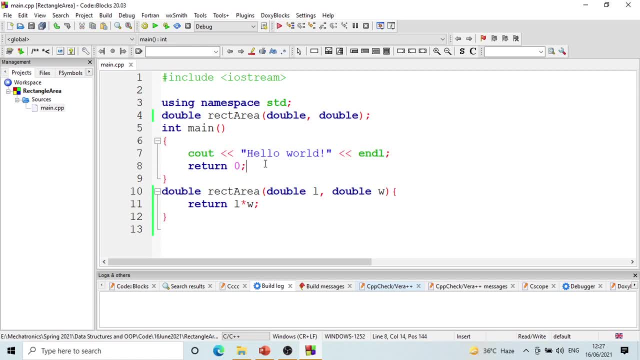 ok say v say cout ok enter the length of the rectangle 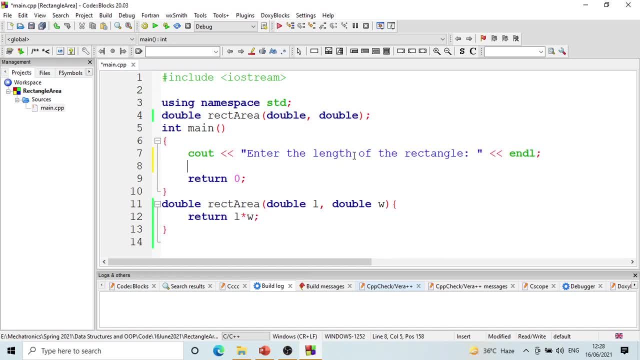 in fact let us simplify enter the length and width of the rectangle and then we say cin l w ok so in one go we will 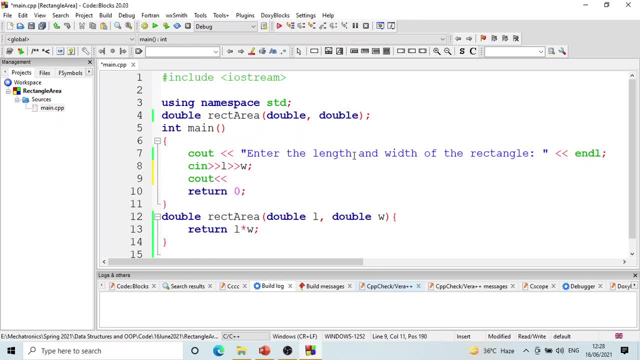 and then we want to yes yes we have to declare sorry double l w 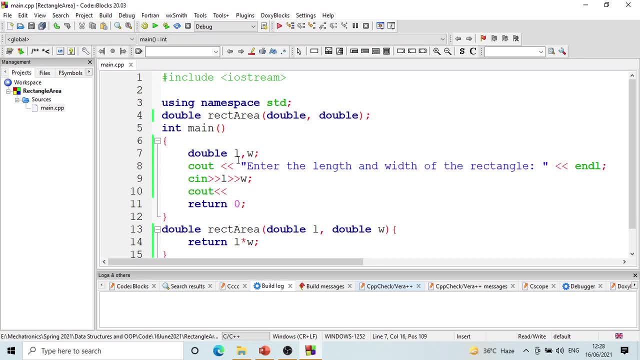 ok now see here these two variables l and w these are local variables to the function 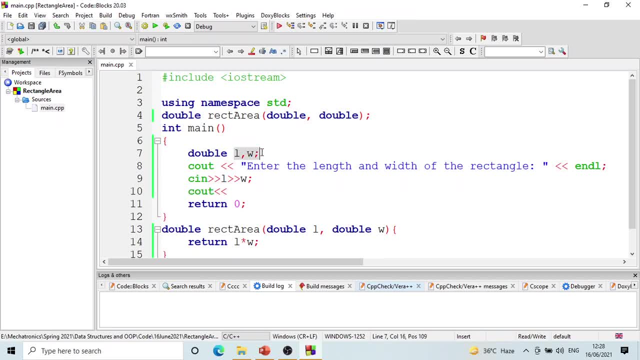 main outside this function these two variables are not visible 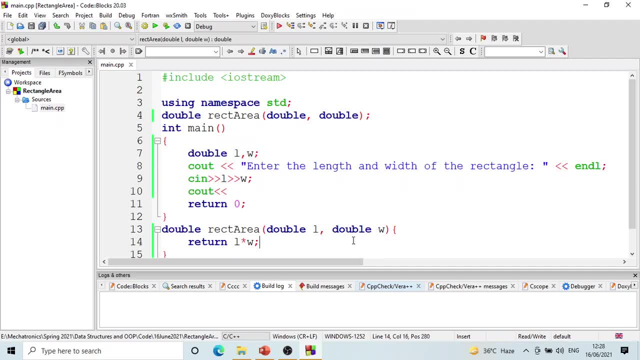 we have these two variables l and w these are local variables to the function rectangle 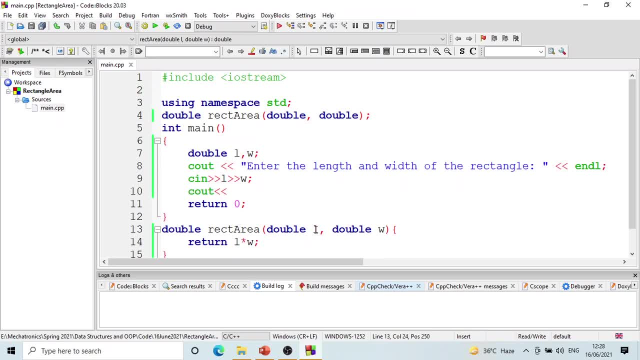 rect area ok these variables are not visible outside 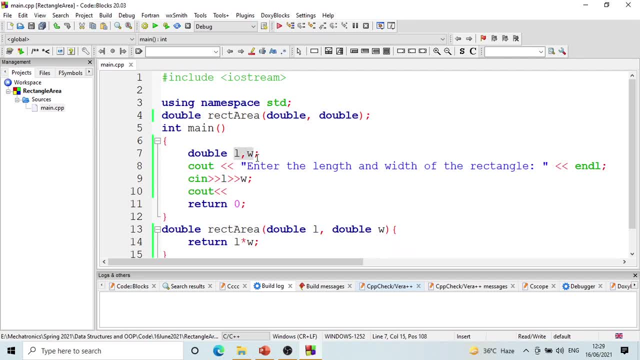 this function so these two are separate variables this is not one this l is a separate variable this l is a separate variable 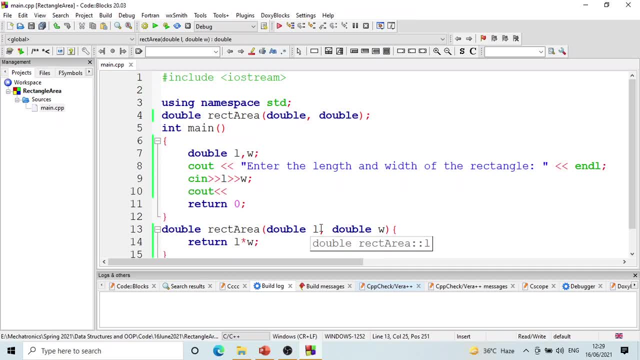 ok you can verify it by printing their addresses if you print their addresses so you can verify that these two are separate variables ok 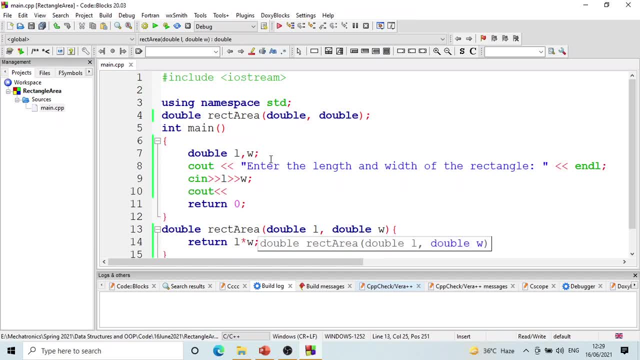 you are getting the concept of local variable so l and this l and w although their names are the same ok but they are in different scopes their scope is different 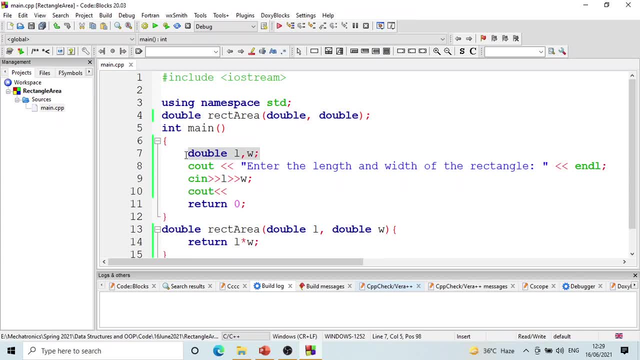 one is in the main function the other is in the rect area function so they have different scopes they can have we can have similar identifiers in different scopes there is no problem in this these are two separate variables there are four variables the names of both are l w and l w but the scopes of both are different this is one variable although you should know it from your computer programming background ok so now we need to find out 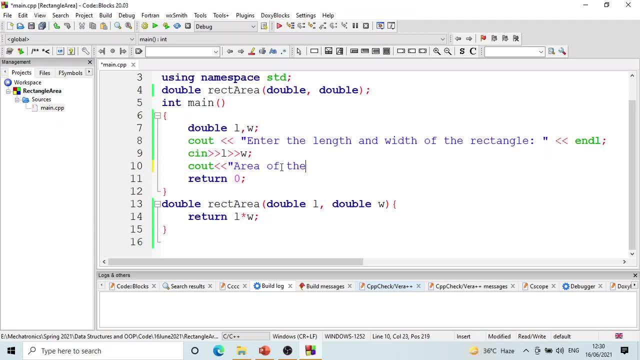 what is the area area of the rectangle 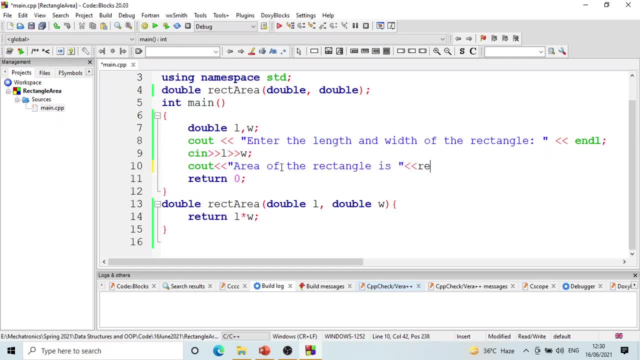 is and then we just call the rect area function and pass these two values to it l and w ok ok 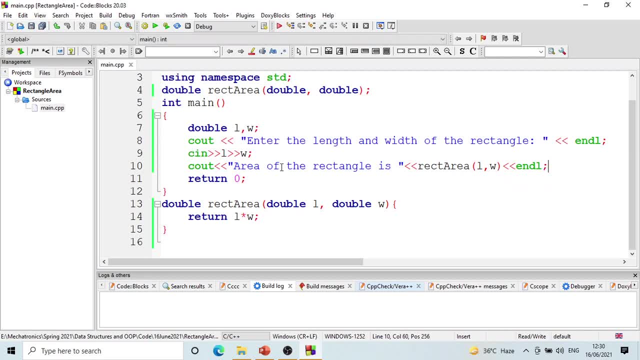 so this is how you basically find out the area of the rectangle build and run this so so enter the length 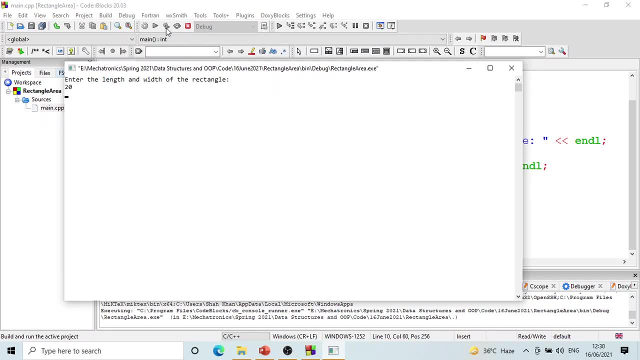 and width of width so say 20 and then 30 so area of rectangle is 600 ok fine 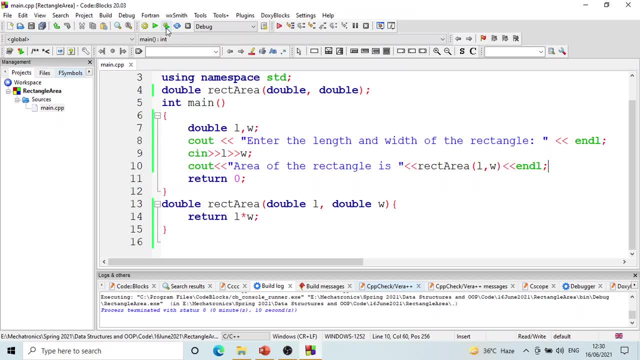 so if you are aware of solving problems like this if we have to solve the same problem using object oriented programming 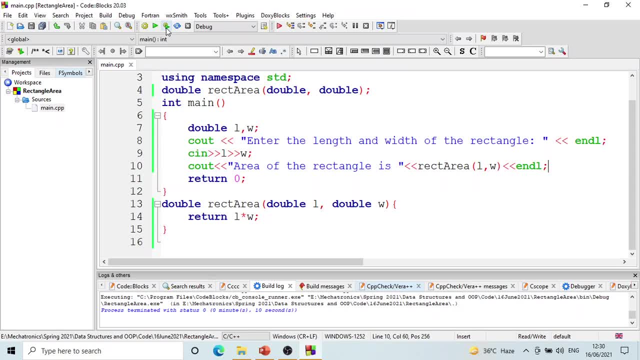 ok so that would be a little different you will have to write more code so maybe you will say what is the benefit of this 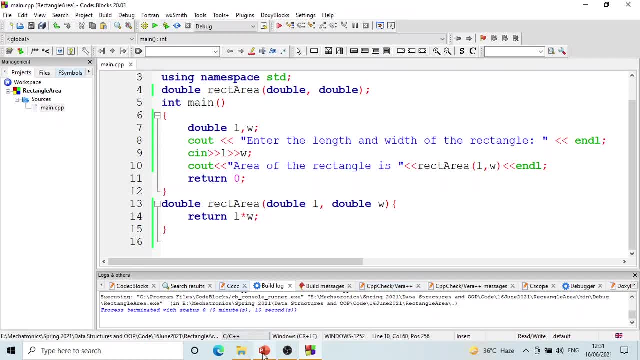 so let's do that but before we do that let us do some background reading ok 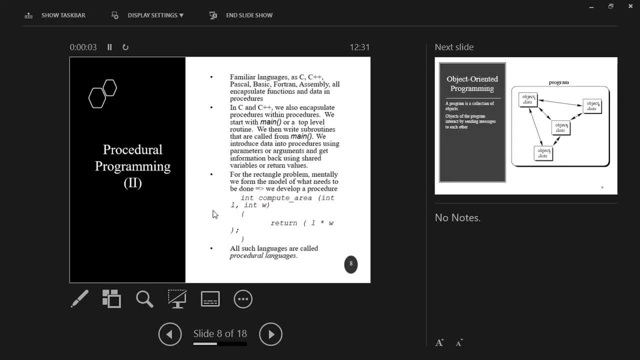 ok so in procedural programming languages this is what you do you have a problem 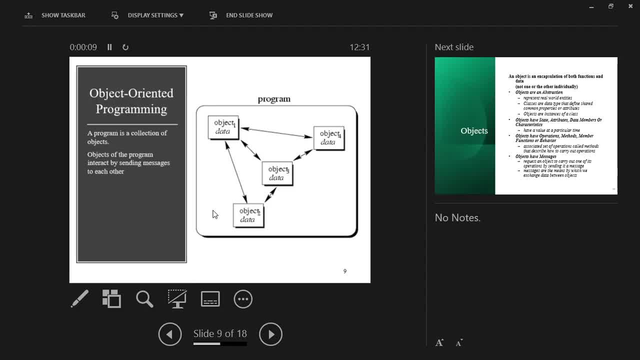 you have a procedure for that problem ok that is what you do 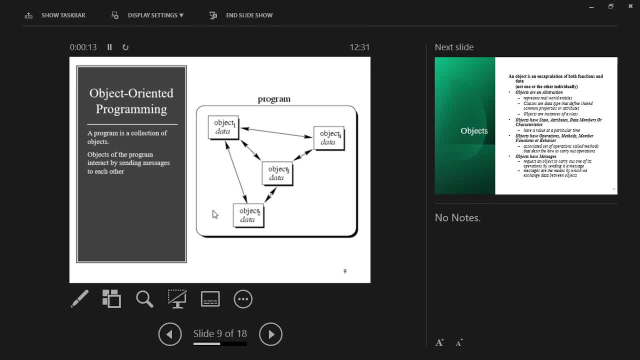 now in object oriented programming ok ok ok ok ok 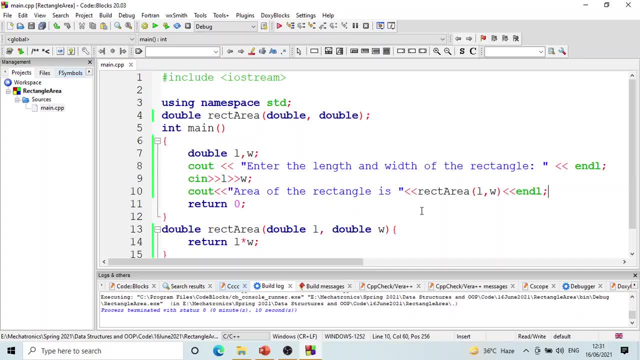 ok so the question is from here we have called this function so we have passed this function these arguments by value or by reference who would answer that by reference by reference yes by reference by value ok those who say by reference how 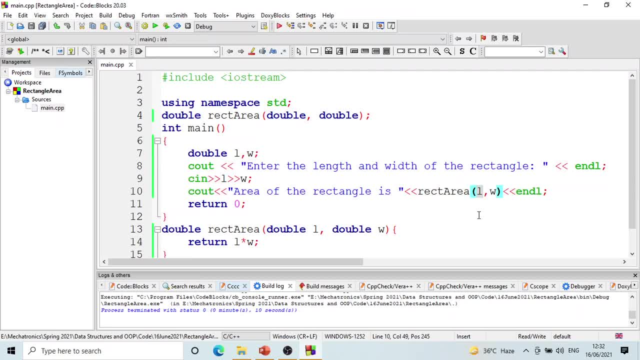 by value ok see by value you have defined this function 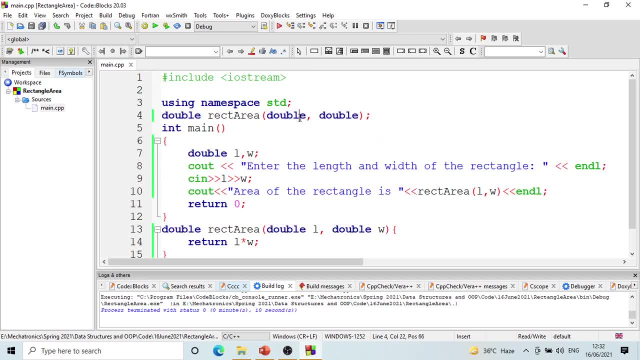 here in a function prototype so the function prototype says it is receiving a double value ok 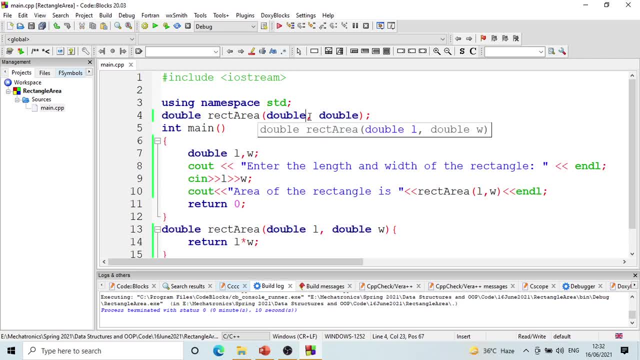 if the declaration was like this ok ok 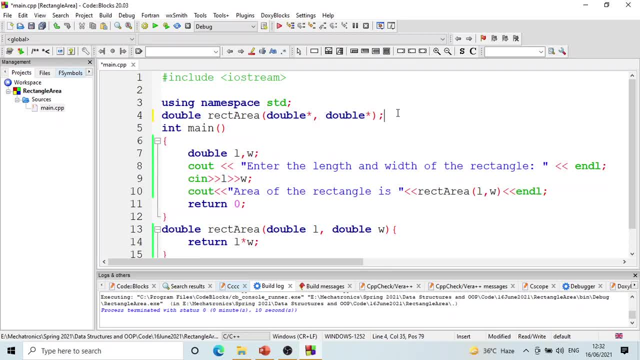 so now you are saying it is receiving a double pointer ok 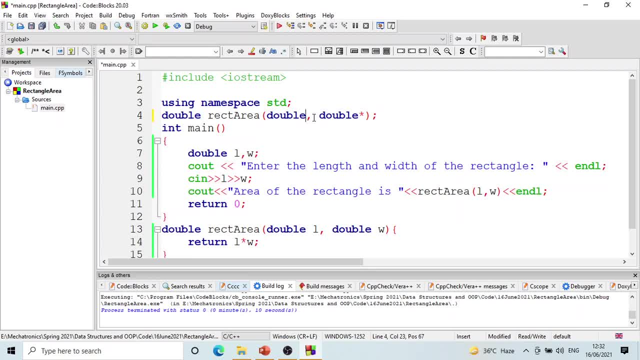 yes if it was something like this 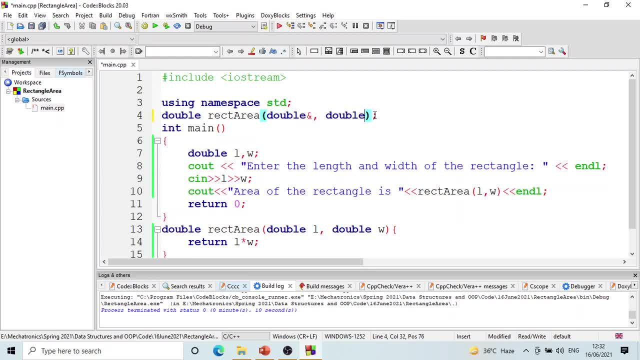 ok ok so now you are saying that you you are basically expecting a reference of type double pointer reference value there are three different things keep these in mind when the time comes I will demonstrate what is a reference reference is nothing but an alias which we call in urdu so this is the second name of the same variable 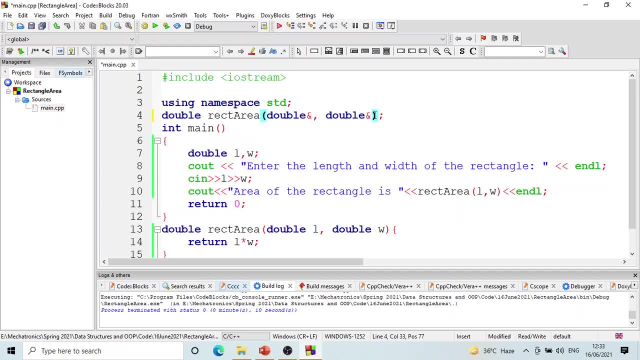 ok the variable is the same but you can create multiple references of it like there is no urf ghulam urf gamma ok ghulam mahmood soor there are multiple names or there can be two or three so references work that way references work that way so if your if your function specifies that I am receiving arguments like this 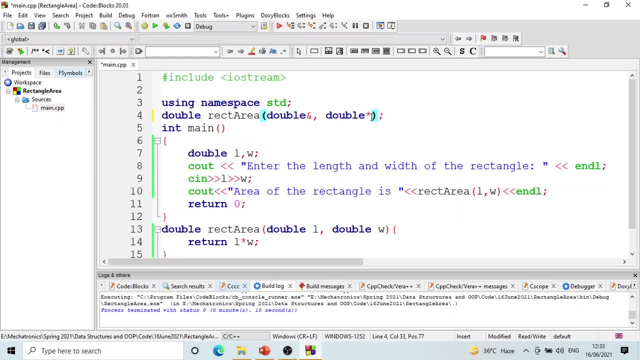 or like this so then pass by reference is happening but since we did not specify anything like this 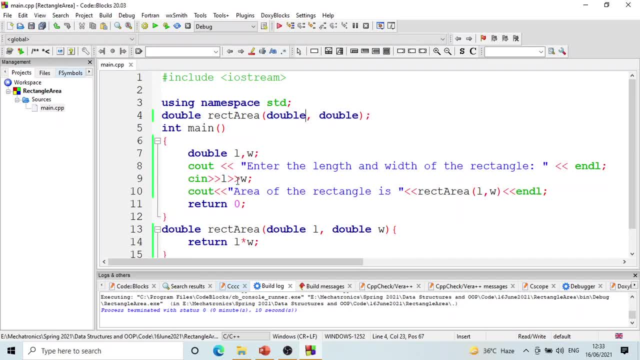 so that means we are passing by value we are sending values forward so we are sending a copy of l in this variable and a copy of w in this variable so we are sending a copy 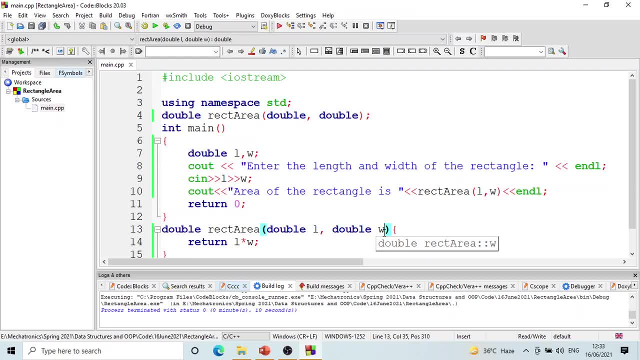 ok you can also reference ok you may not feel the effect 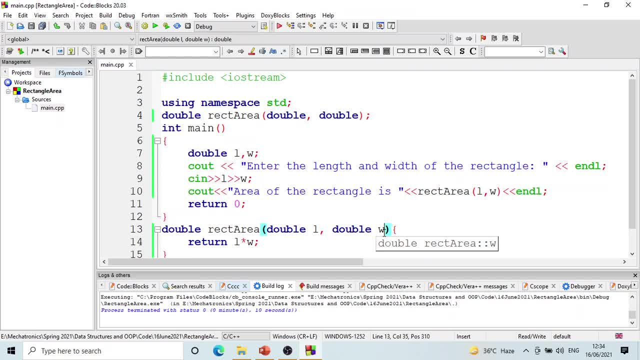 is it working or not let me demonstrate first see this ok ok ok it depends ok I have done here 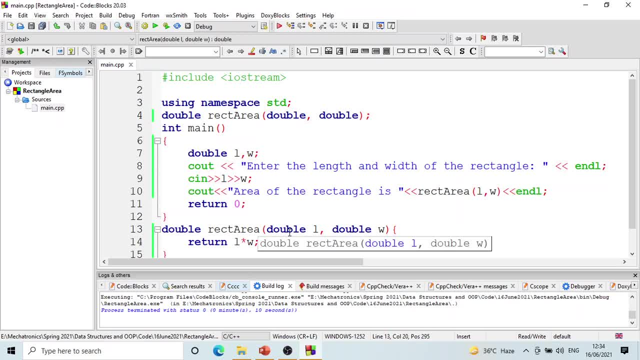 you are doing here this is a declaration 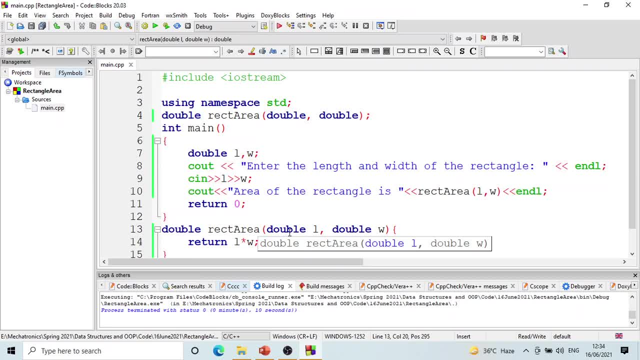 where are you talking about are you talking about main function or rectarea function ok ok 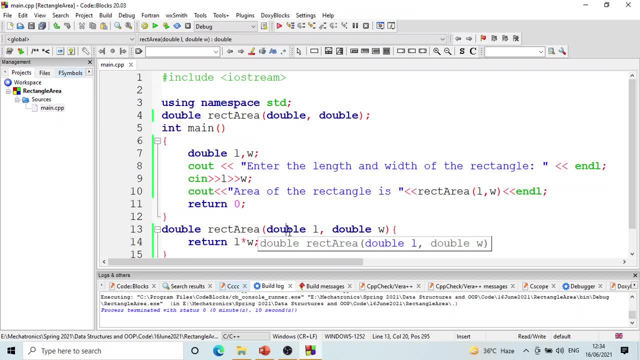 no talking please ok so here we will finish the reference story before we proceed 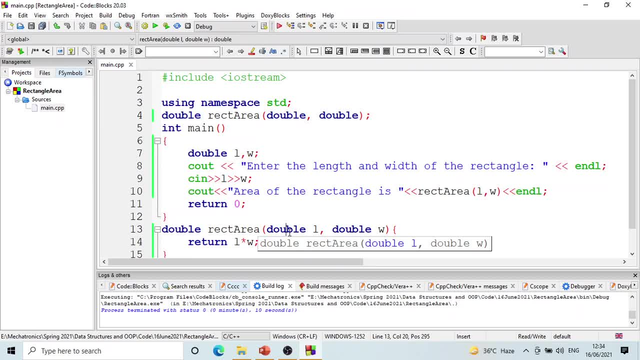 now say for example defer it to later or we already already talked about pointers as well chicken they can let us differ pointers to later reference could be somebody this is also important say for example we say that this is a reference 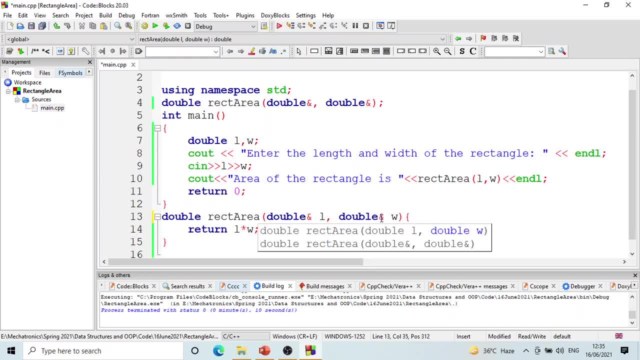 of type reference okay before i do that 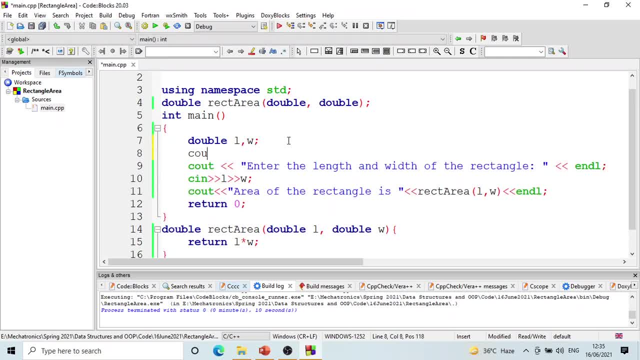 so i want to say print the address of l and w so i want to make a point these variables are different variables 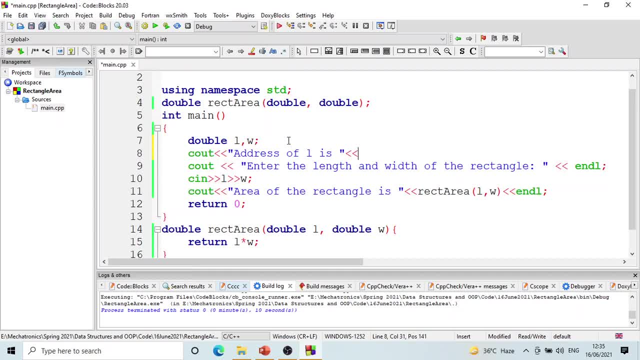 address of l is and then uh address of operator and l okay similarly address of w 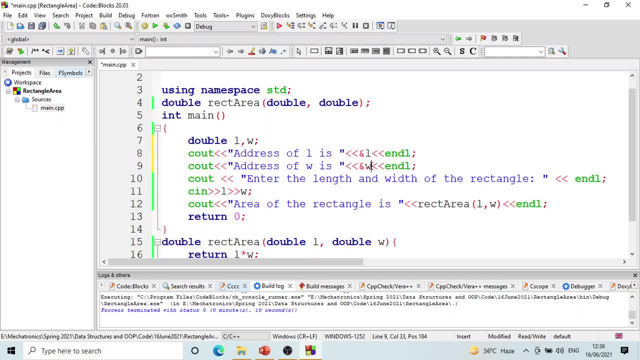 address of w is and then address of w this is important okay 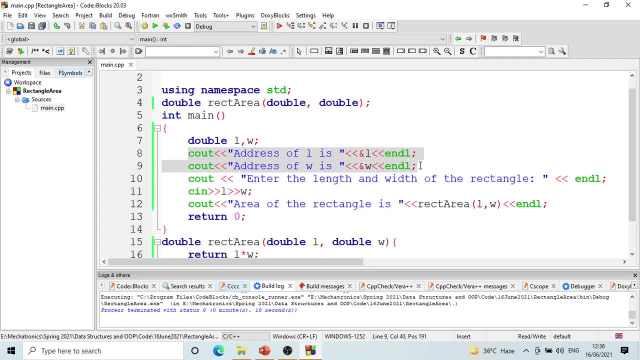 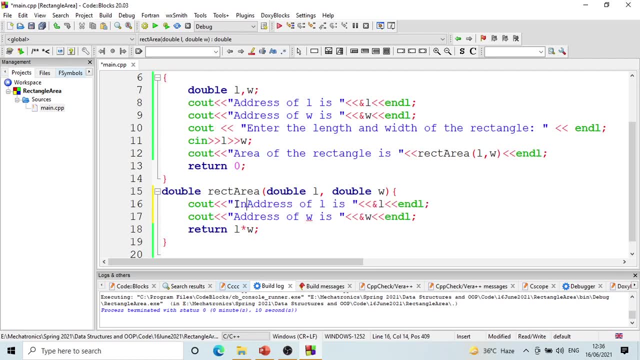 okay now we take these things inside the rect area function and here i add another text inside 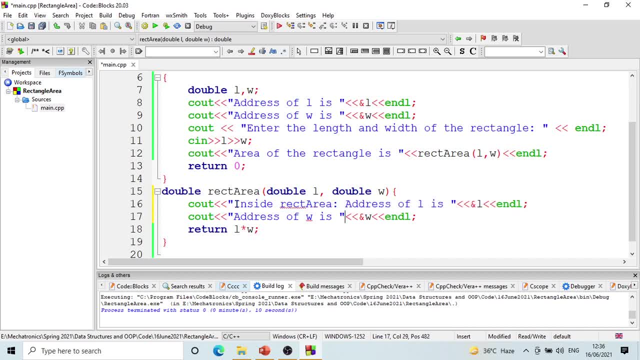 the rect area function and here i am printing the address of l and address of w 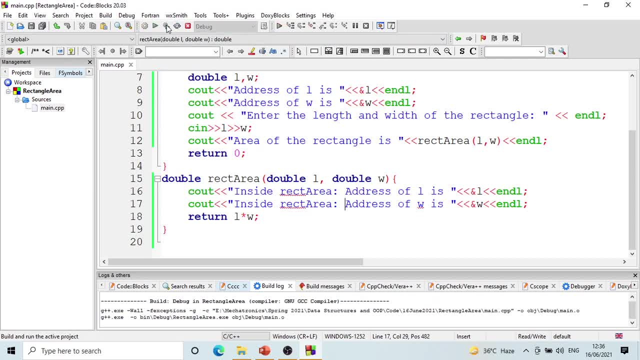 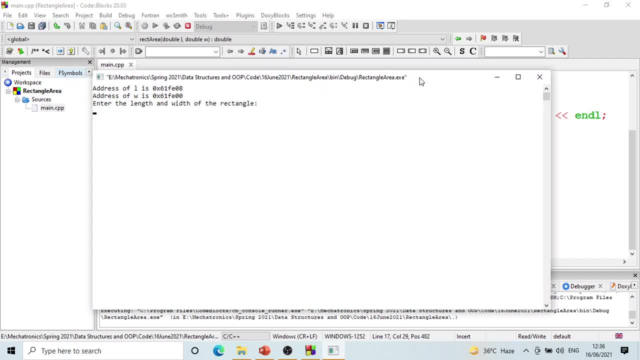 actually let us build and run this code okay address of l you can see if there is any value of it okay the value is not important but you should know that it is different from the other one 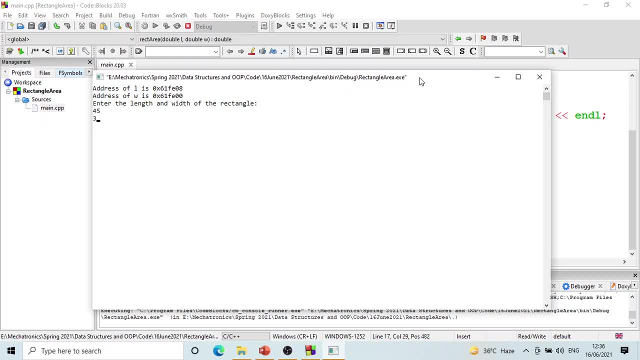 okay so here we have entered 45 or 32 area of rectangle is okay it is being printed here but before that these messages are being printed inside rect area address of l is six one f d e zero which one is this six one f e zero eight which value is this yes which value is this which value is this address yes no address garbage 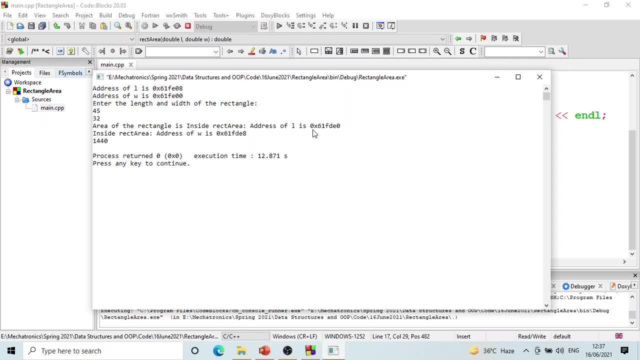 there is no garbage value any value that starts with 0x that is a hexadecimal value that is an address okay garbage value that is printed in decimal and this is an address this is Sebastian's hexadecimal value of zero x so this is a hexadecimal value and this is a hexadecimal value okay so it is an address the point is that l and this is l 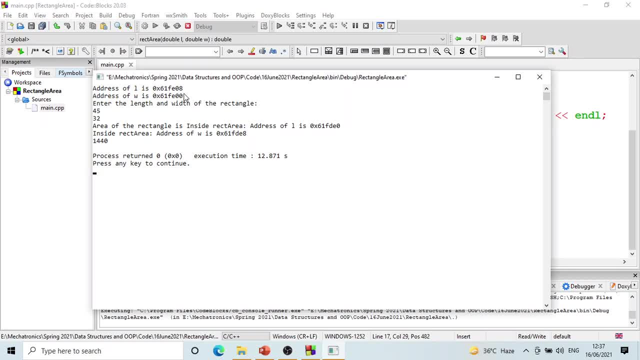 And this L, their two addresses are different. W and this W, their addresses are different. That means these are different variables. These are different variables. Okay. 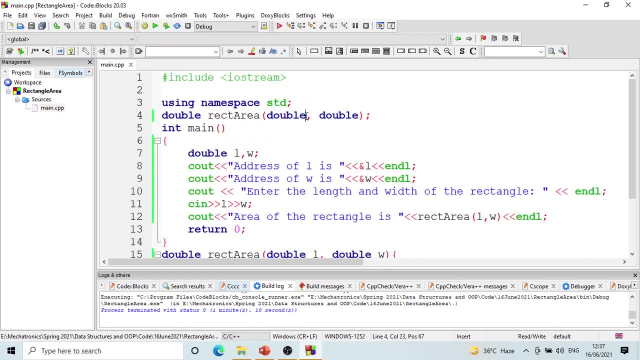 Now, we will change this code a little bit. Now, let us make it a reference. Okay. Let us pass these values by reference. Okay. 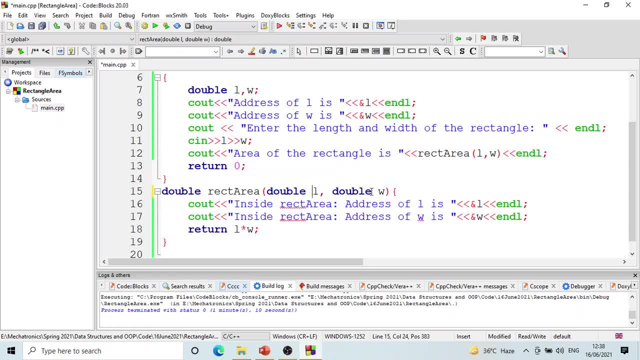 Okay, this ampersand symbol, you can put it here as well as there. Okay. Doesn't matter. Okay. 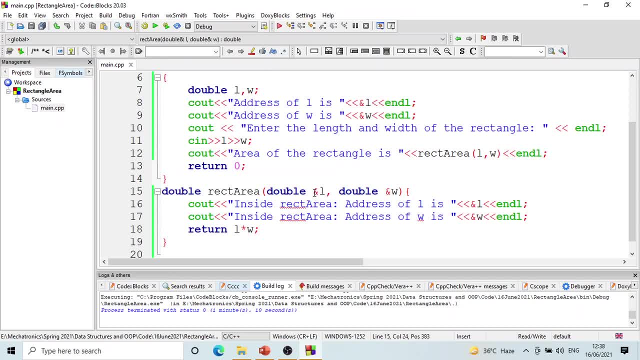 Now, when you use reference, now L is a reference. W is a reference. What is a reference? Reference, very simply it means an address. Pointer is also an address. But pointer is a variable. That is so. 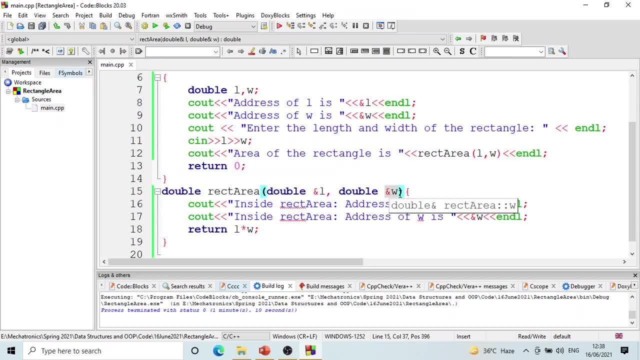 Pointer also stores an address. And reference means an address. Okay. And you can also understand it as an alias. Okay. Reference is usable. 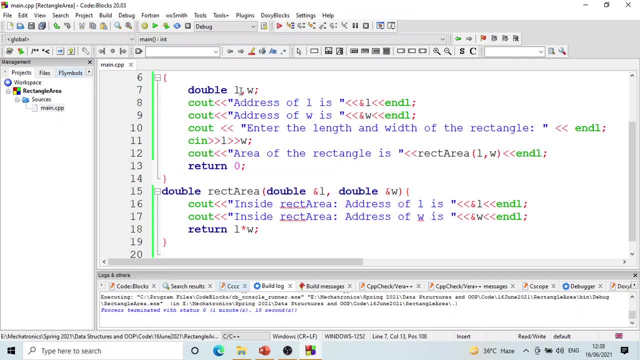 This L is the second name of this L. Although it is not so different. But still. 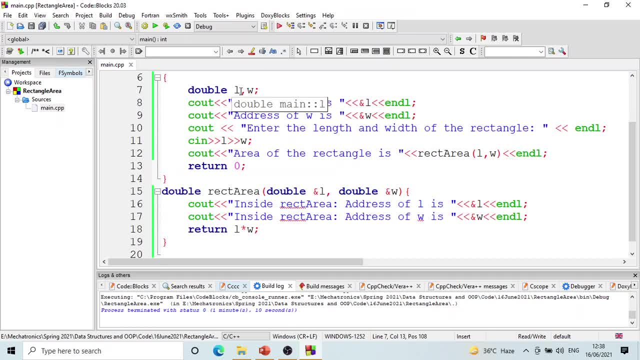 Now, I will demonstrate you a little point in this. Okay. 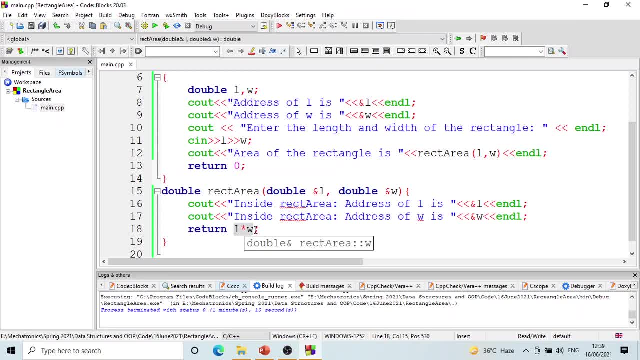 When you use it, you do not need to use it differently. You use it as normal variables. 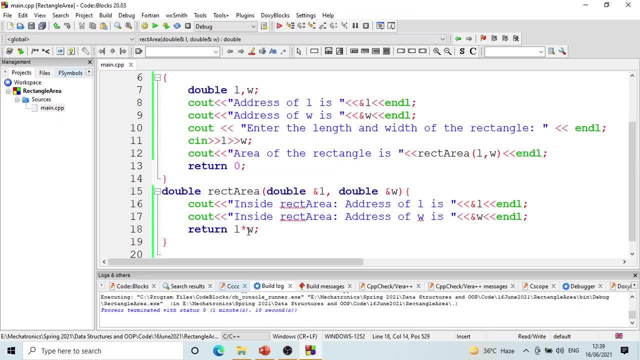 Like here we have ampersand. You do not need to use that. 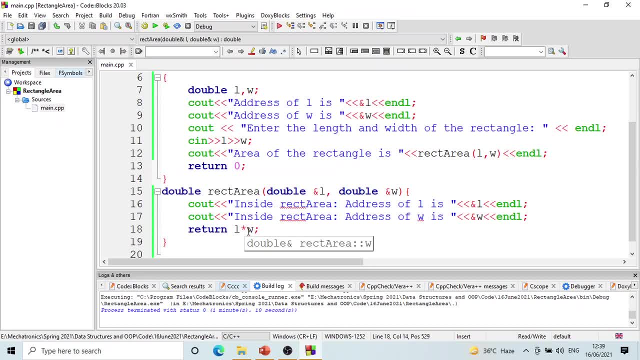 In the case of pointer, this is not the case. If you are using pointers, if you want to access the value of a pointer, then you have to use a dereferencing operator. 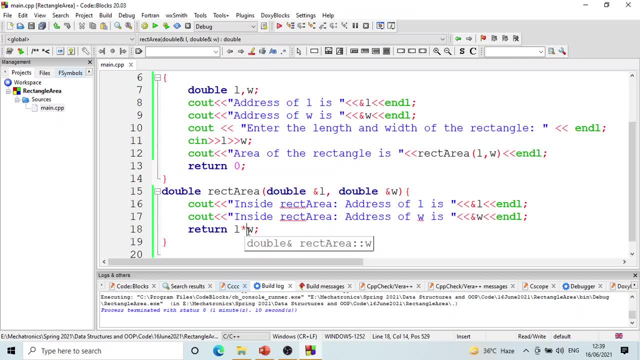 But in the case of references, you can access the value of the reference without using any special operator. Understand? Do you understand this? 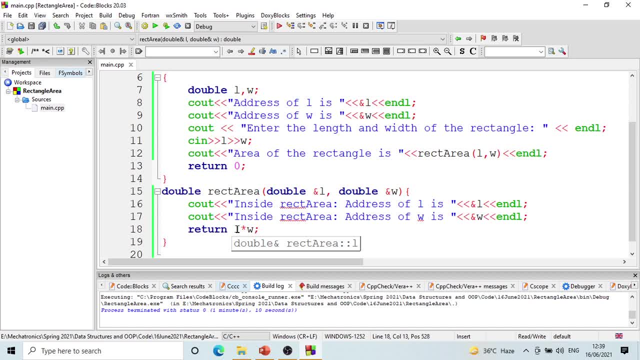 You use the reference as a normal variable. You cannot use the pointer as it is. 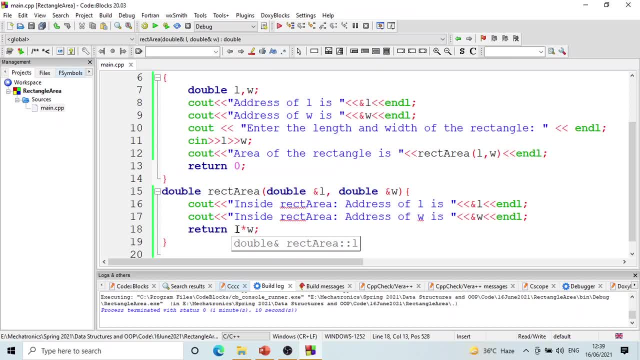 If you want to access the value of the pointer, then you would need to use the dereferencing operator. Okay. 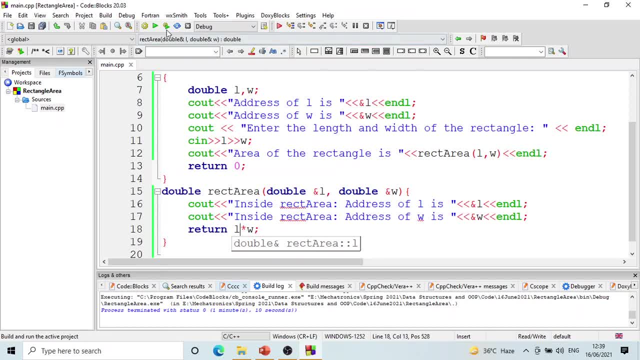 Now, let us see this code. Okay. So, let us enter these values. What is the address of L? 61FE08. 61FE08. 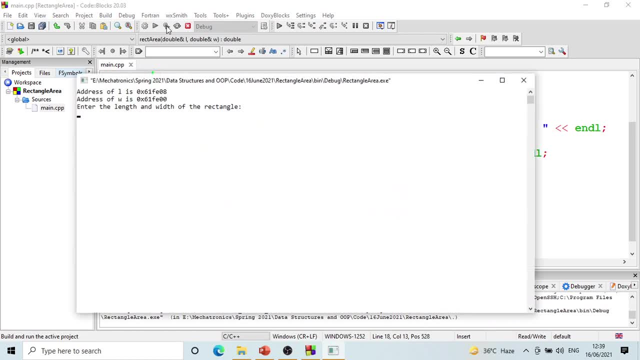 The same address. 61FE00. The same address. W. The same address. W. W. W. W. 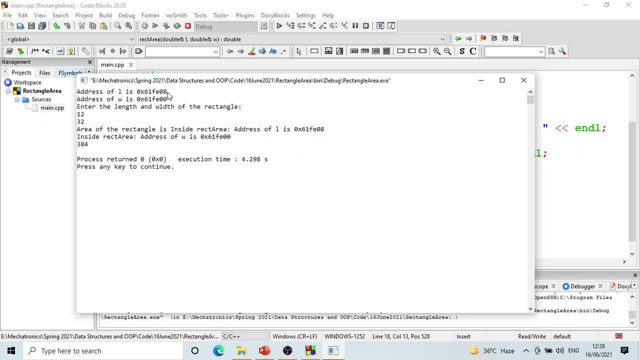 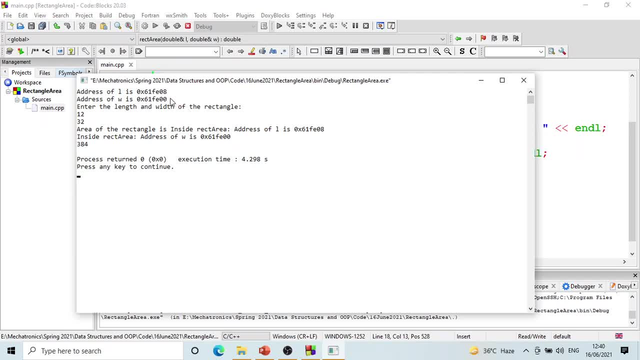 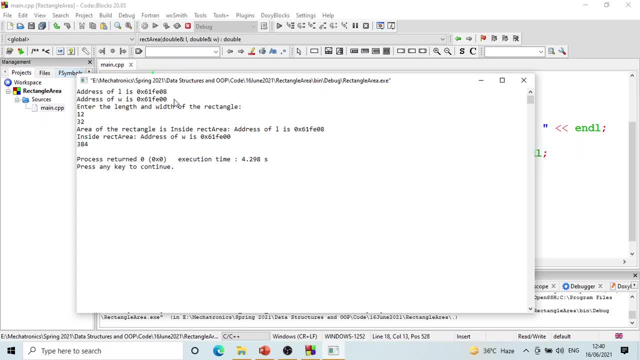 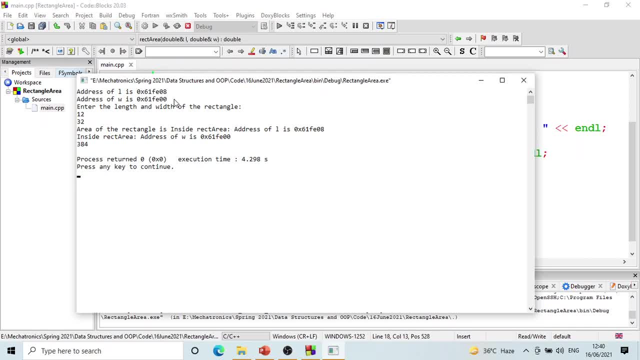 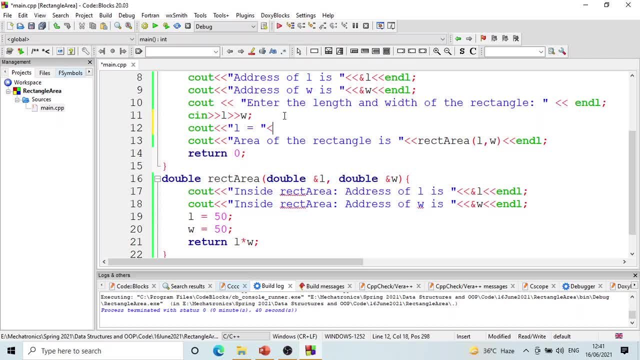 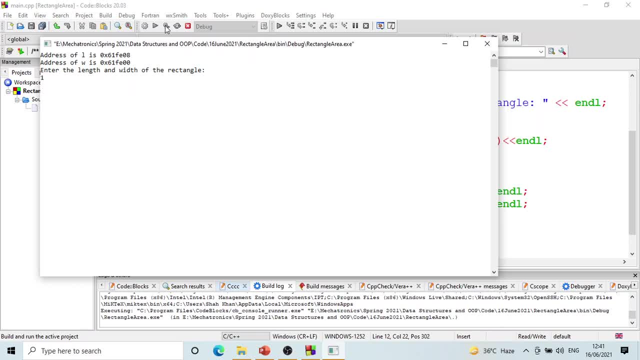 Let us enter values. Let us say I enter 10 for one and 15 for the other. 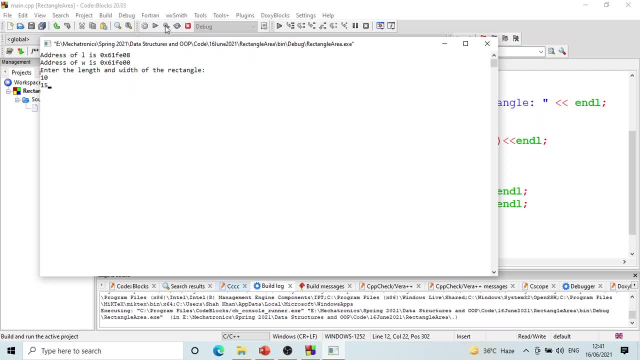 So I am expecting that I would get 150 as the area. Okay, before calculating the area, I am changing it. L is equal to 10, W is equal to 15. 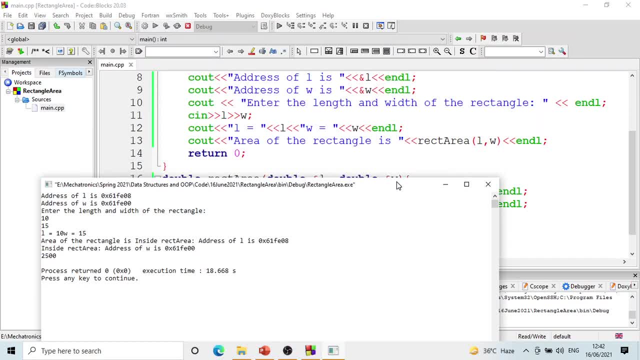 Where am I printing this? Okay, before call. Before call. Look at this. 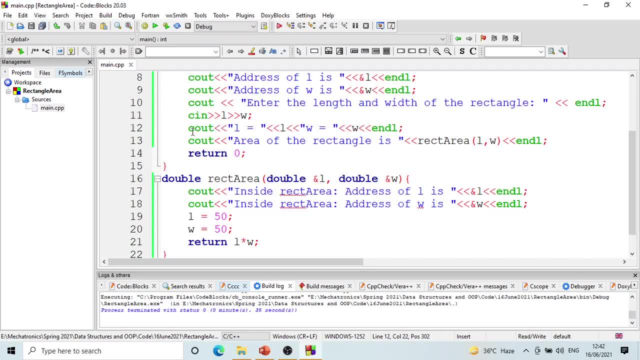 See, the area has changed, right? But that does not make it a point. 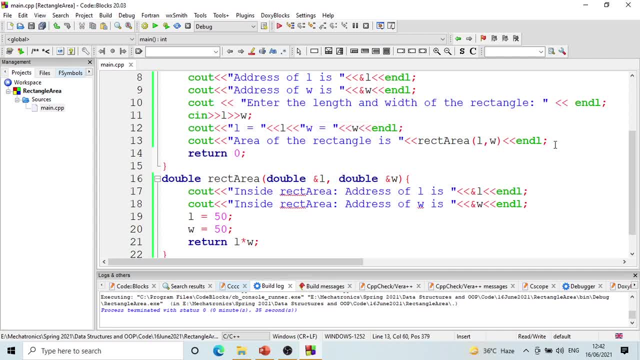 These are the values that you entered and after coming back, these values change. I will write before here. Okay? Before. These are after. After calling the function, its values change. 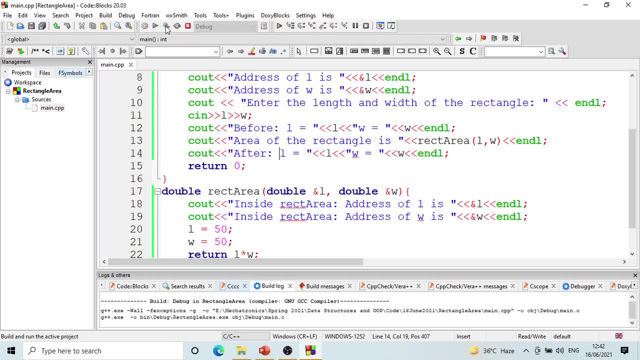 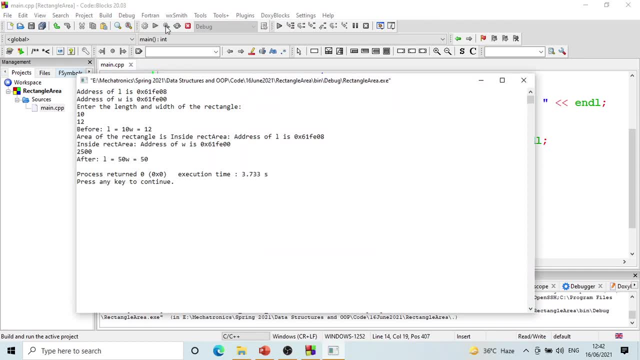 So, before we call the rect area function, the value of L is 10 and the value of W is 12, okay, which we entered. Once we call the rect area function, it calculated the area, i.e., first it changed the value of L, then it changed the value of W, so it calculated the wrong area. It did not calculate the values that we sent. Okay. 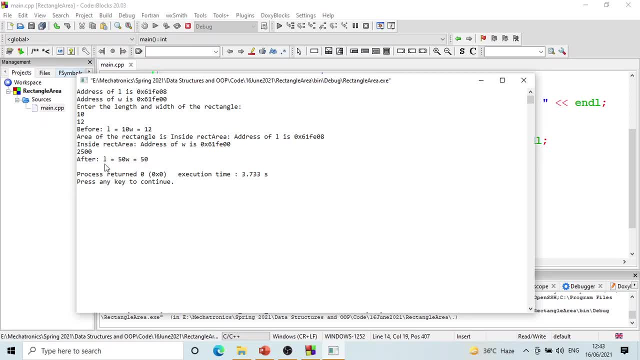 Okay, the changes that we did in the rect area function have been reflected in the main function as well. See, after we return from the rect area function, the value of L is 50 and the value of W is 50. Can you see? 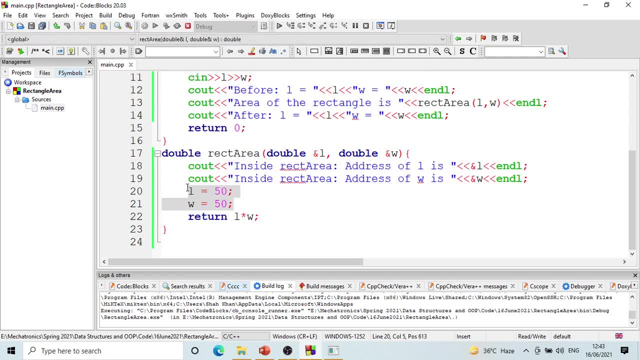 Why are these values being reflected there? Because we passed the variables by reference, we sent their address. 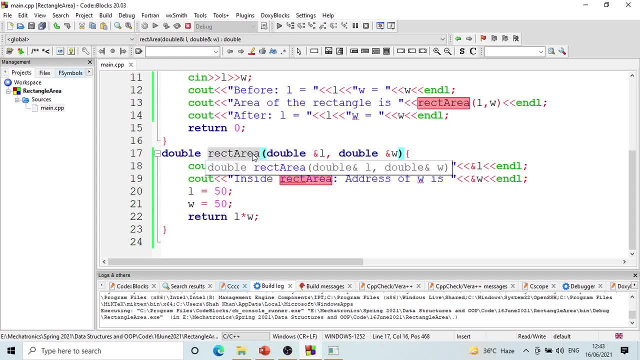 So, this function is not reflected in the main function. This function has got access to the original variable. So, it can change its value. This is a powerful feature as well as a problematic feature. 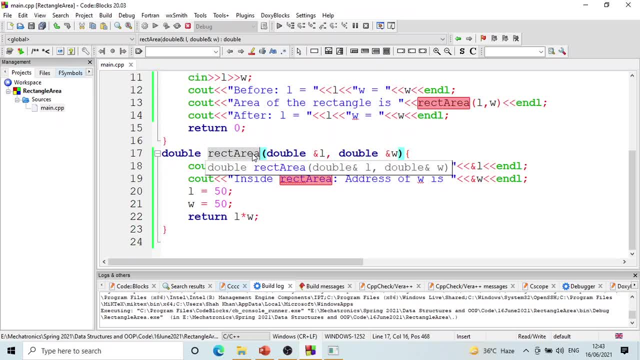 Okay, if you make a mistake, there is a chance of making a mistake. So, you can make mistakes as well. Yes. Yes. Yes. 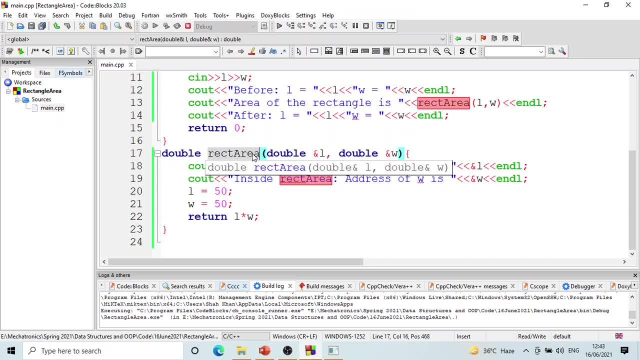 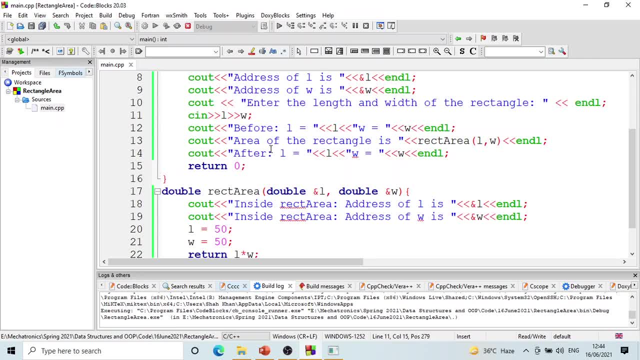 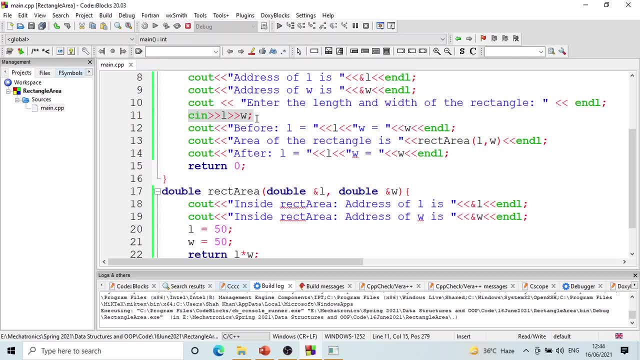 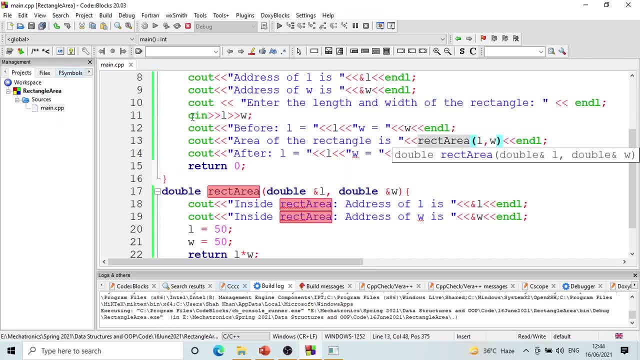 Yes. Yes. Yes. Yes. after calling the rectangular area function? Okay. 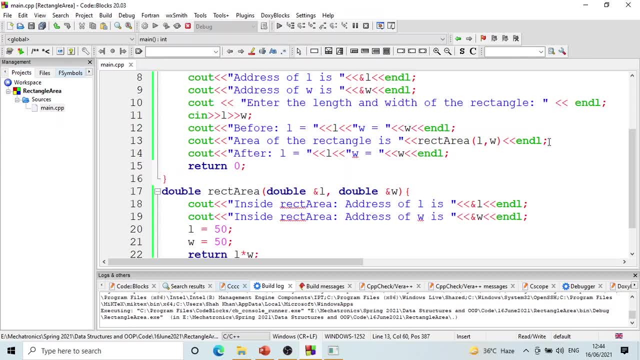 There will be two prominent effects. One, L and W contain garbage values because we just declared them and we didn't initialize them. 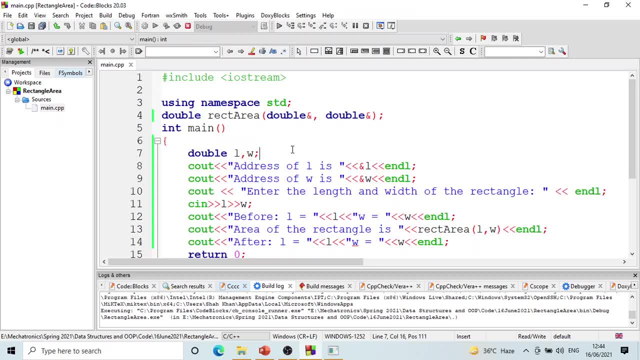 So, the area you are calculating that would also be a garbage value. Okay. 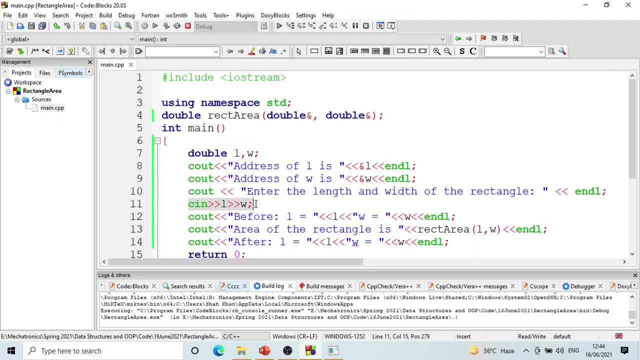 We are initializing L and W through this statement. We are assigning initial values. We are assigning initial values to this CN statement. Okay. 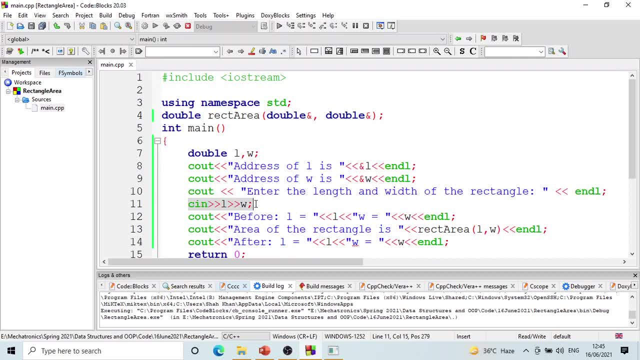 The second purpose of the program is that we take the length and width values from the user and calculate the area from them. 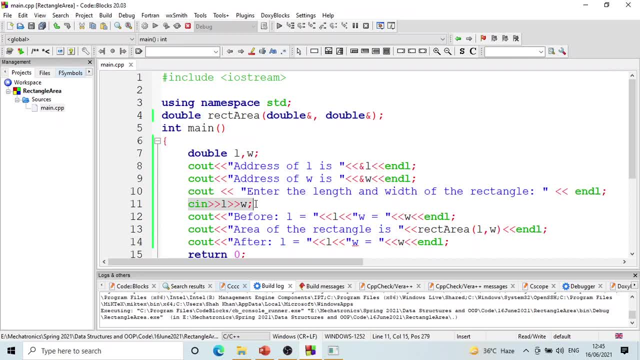 If we calculate the area first and take the values later, then it doesn't make any sense. Okay. No. I will correct this point. Okay. 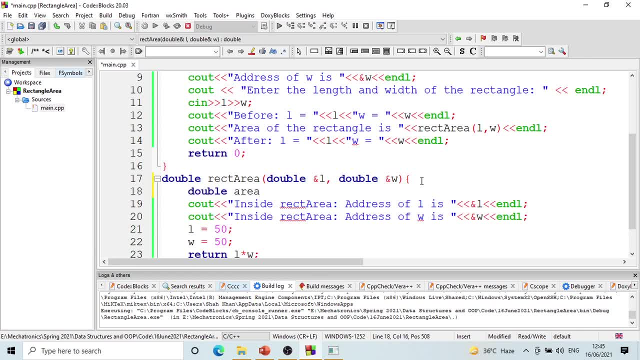 Here, I, I declare a variable double area and double area is equal to L multiplied by W. 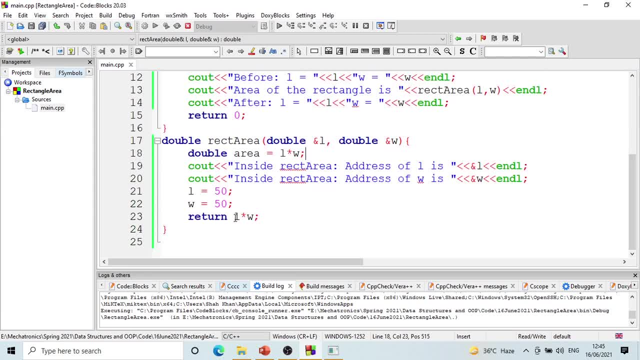 So, we have calculated the area and now we are returning this area. So, the area will be calculated correctly. Okay. 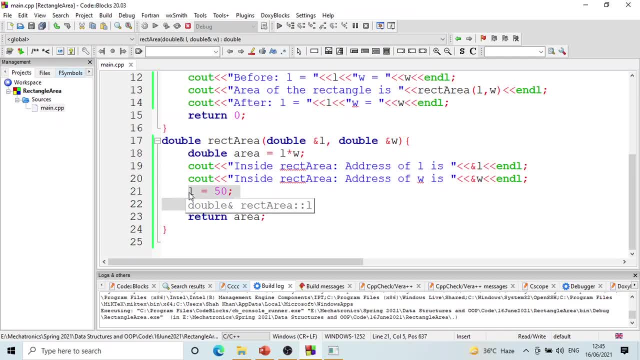 Why did I do this work? Why did I change L and W? Because I want to change that if I change the value of L and W in this function, 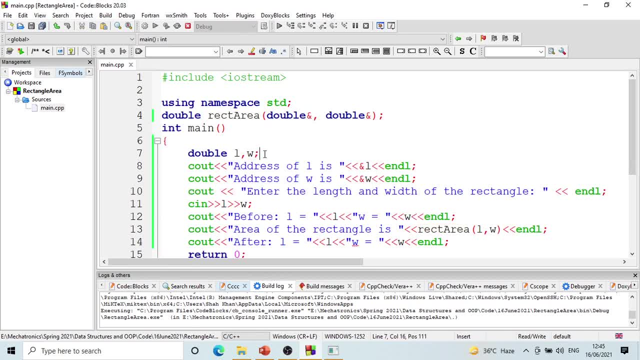 then will it have an effect on the main, does it happens at the L and W variables in this function or not? 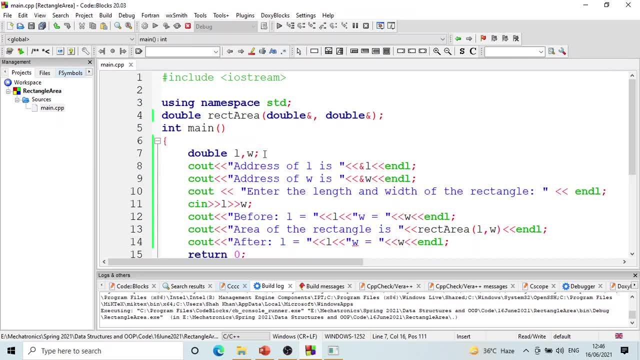 It happens in this case, when you pass variables by reference, then it happens. 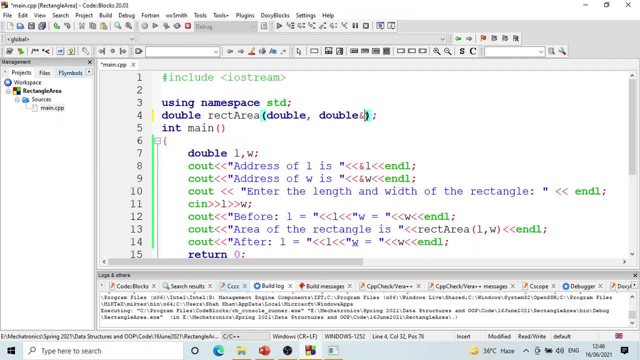 If you pass by value, remove this, Okay, then you will not find any difference. Then, there will be no difference in these changes. 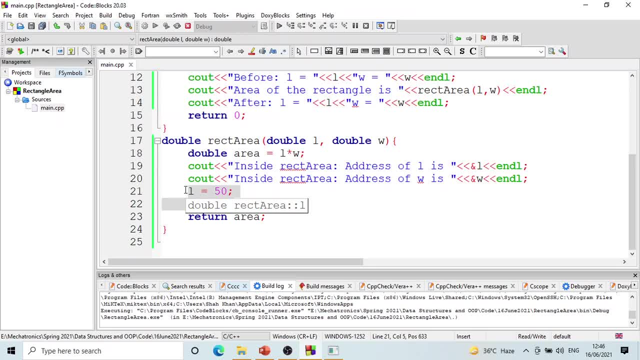 What does that mean? That is, Are you going to calculate? No, that will be calculated, 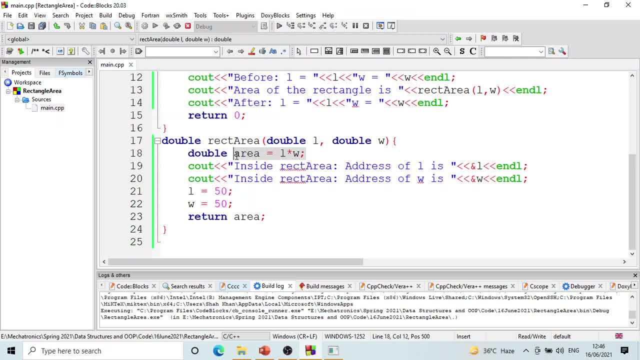 We have fixed the problem of calculating area from the values that we have passed here. 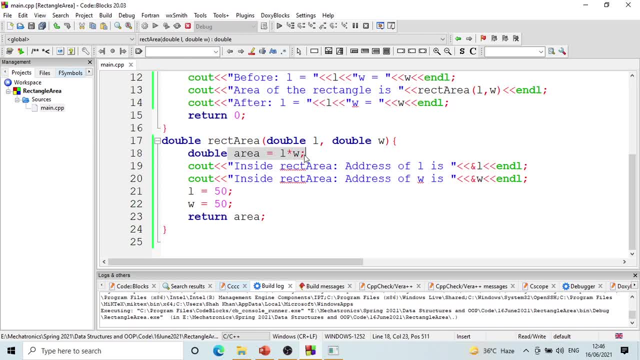 Because we calculate area before changing the values of L and W. See here. 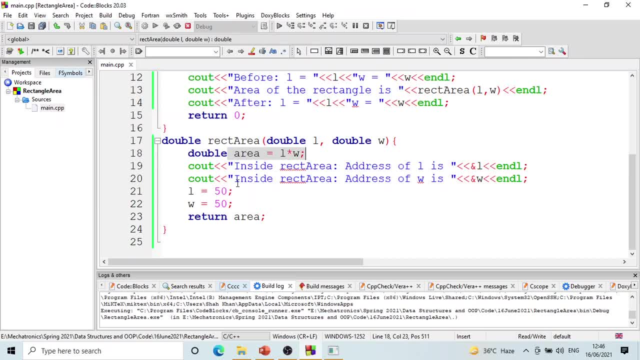 We use L and W first for finding out the area. We change it later. And here we return the area whose value is calculated here. 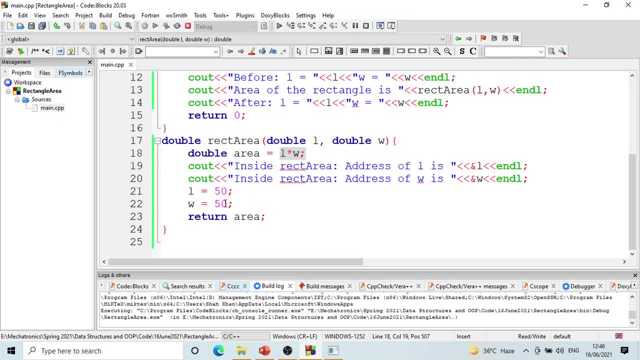 If we change L and W, it doesn't affect the value of area. We have fixed that problem. 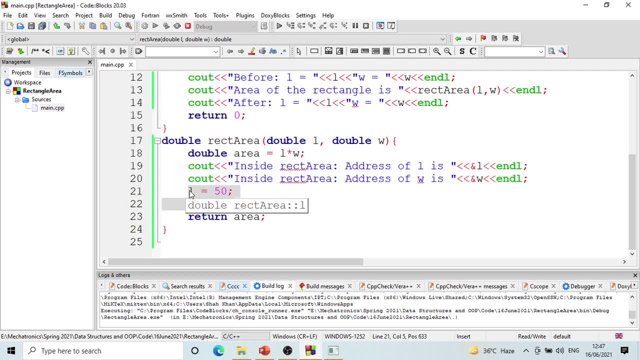 The second problem is that we are changing L and W in the RectArea function. Does this change reflect here or not in the main function? This change reflects in the first run. 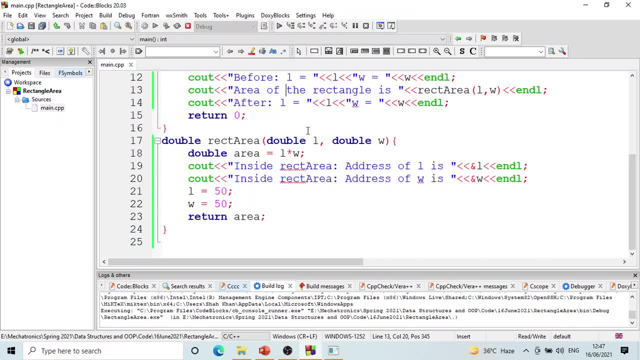 If we change the value here, it will be there. Why? Because we were passing L and W by reference. It will be in reference. It will not be in value. Okay. 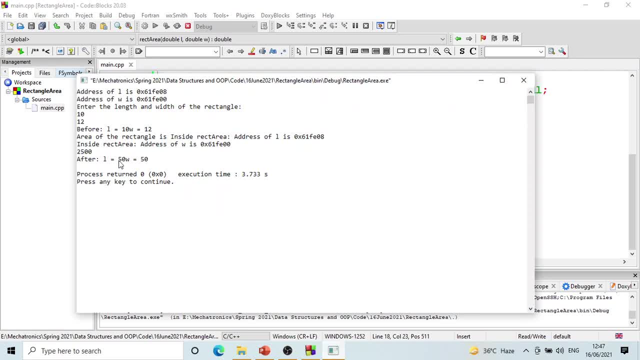 We want to verify it. See, it changed in reference. 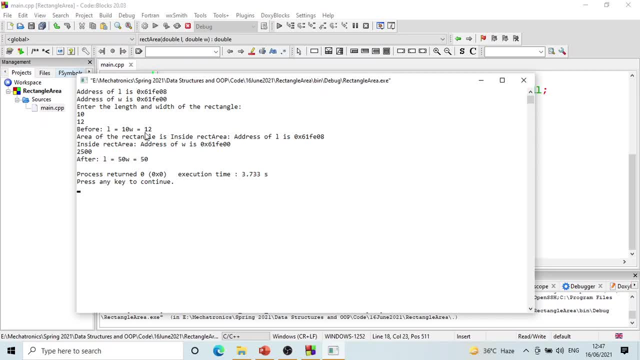 Before 50-50, it was 10-W. 10 and 12, sorry. 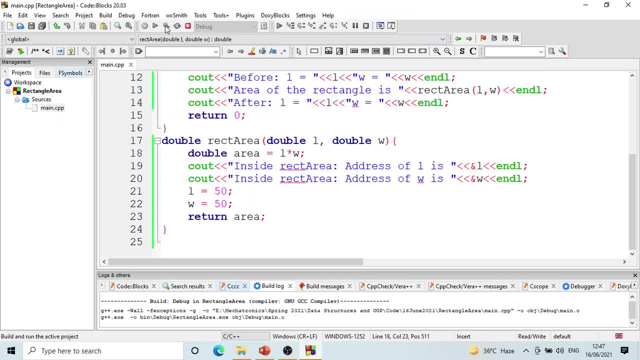 If you do it by value, there will be no difference. 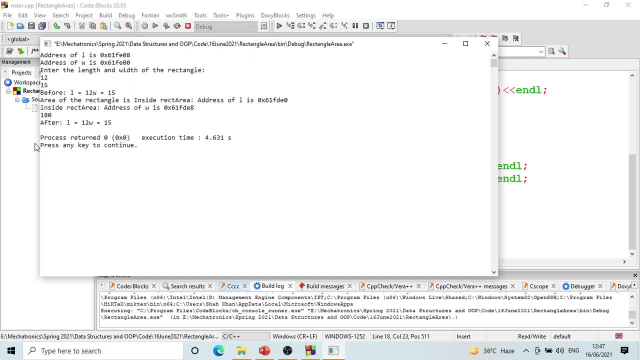 Say, 12, 15. So, before calling the RectArea function, L's value is 12, W is 15. 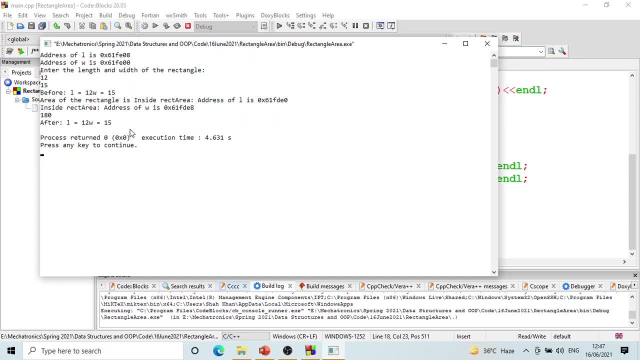 After calling, it is 12 and 15. There is no difference. So, this is the difference between pass by reference and pass by value. Okay. 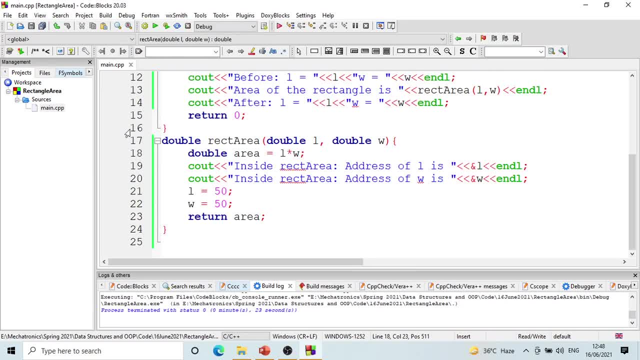 So, you should know about it and you should be using it carefully. 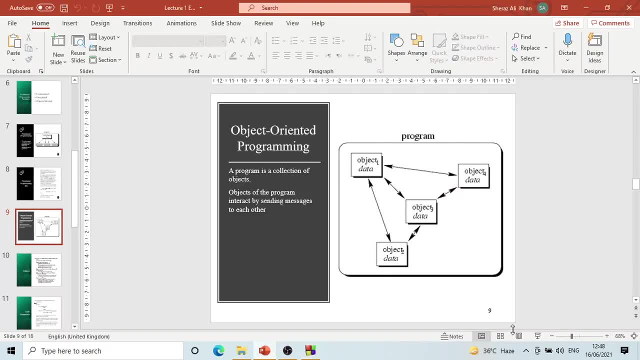 Okay. Now, let's get back to the slide. 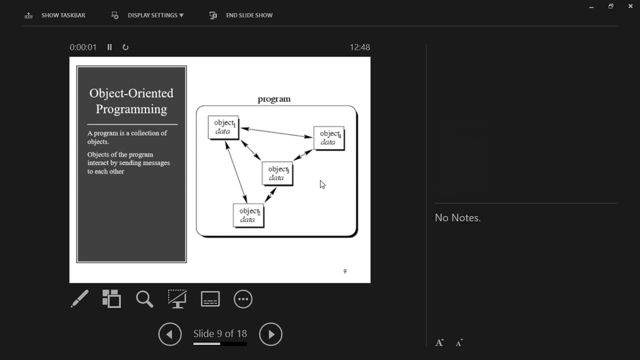 So, in object-oriented programming, a program is nothing but a collection of objects. A program is nothing but a collection of objects. Okay. Virtual objects. They are not real objects. But we model real objects as software objects. Okay. 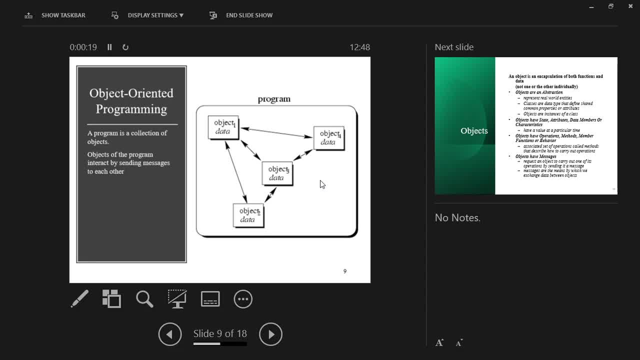 And objects are two very, and these objects are constantly communicating with each other. Like, they talk to each other. Like, in the real world, we have objects, different objects and those objects interact 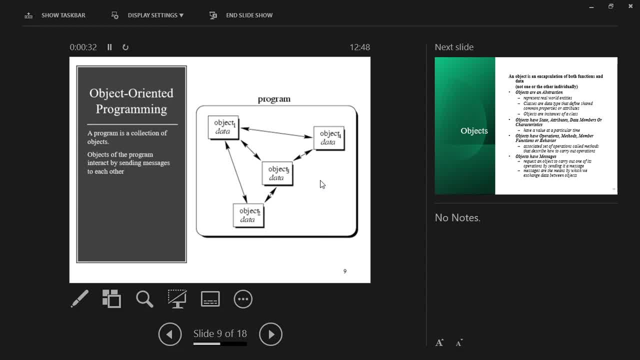 with each other through their interfaces. If I want to say something, I am saying it. If you want to receive something, you are watching me and you are listening to me. Okay. So, this is how we are communicating. Okay. 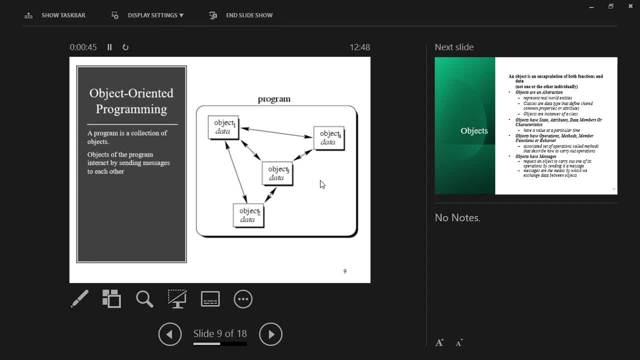 If you want to turn on the fan, it has an interface. Here, you have a regulator and a button for on-off. That is the interface. You can turn it on and off with the on-off button. 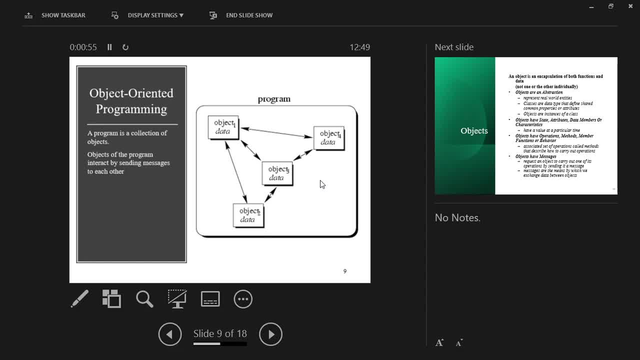 You can control its speed with the regulator. This is an air conditioner. 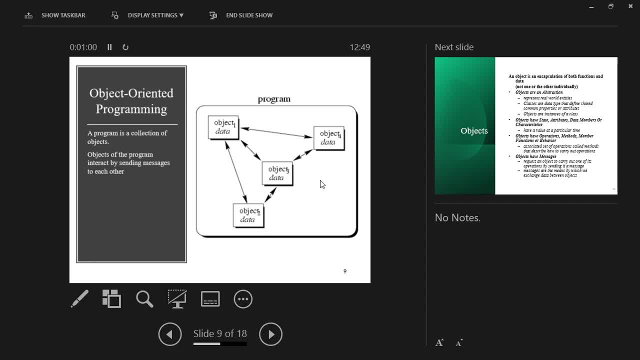 This is an object. If you want to interact with this object, you have two interfaces. One is the power plug and the other is the remote control. So, using that remote control, you can change its set temperature, humidity, mode and other things. you can change different things 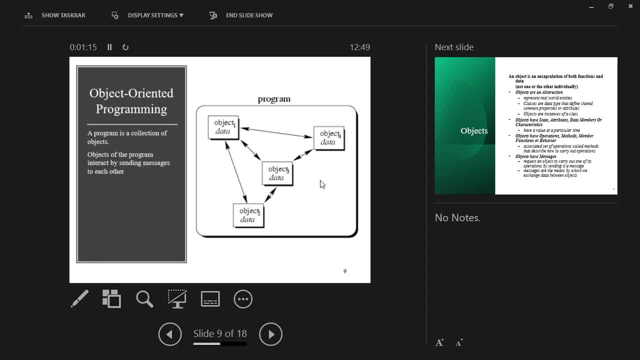 now whatever goes inside the air conditioner 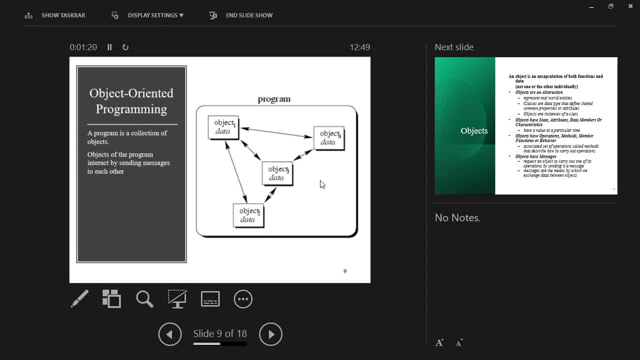 usually we are not bothered by that we are not concerned about that you are driving the car 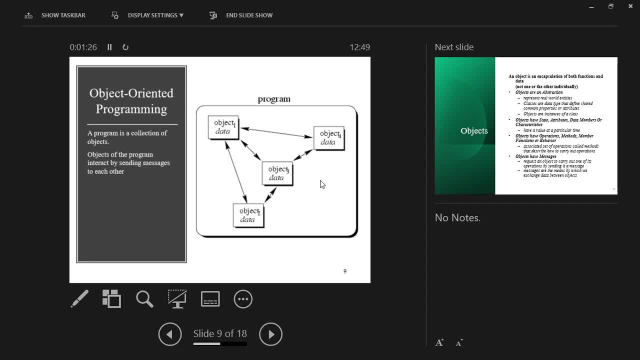 so all you are interested in is the interface steering wheel, clutch, accelerator, brake pedal, handbrake 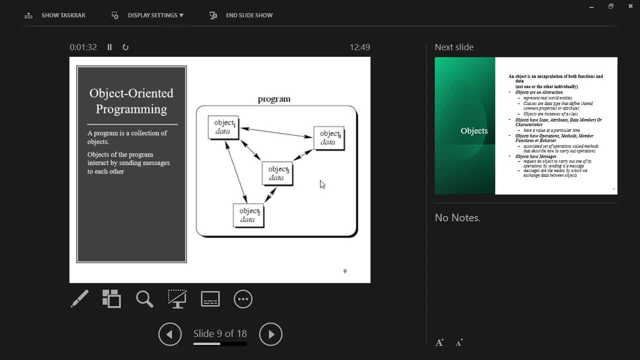 that is your interface with that you are controlling the movement of the car 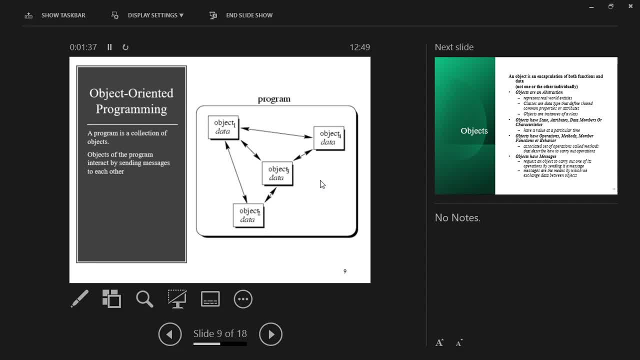 now what is happening inside the engine that is usually hidden from you 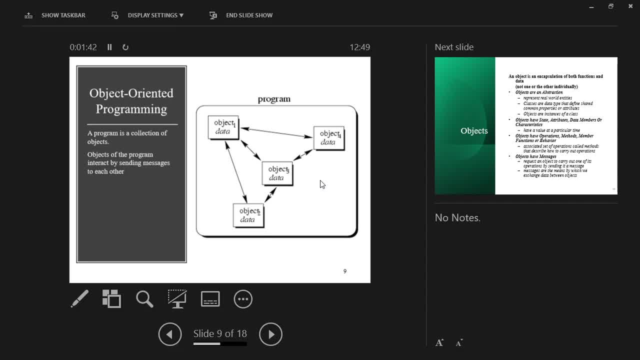 you are not opening it what is going on inside the engine 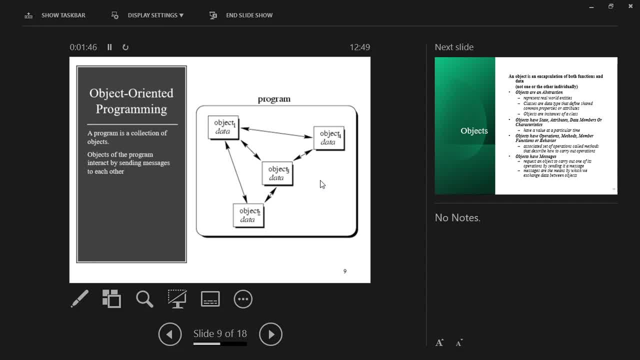 so that is the idea of object oriented programming as well that we create software objects those software objects should have public interfaces and through those interfaces they will be communicating with each other 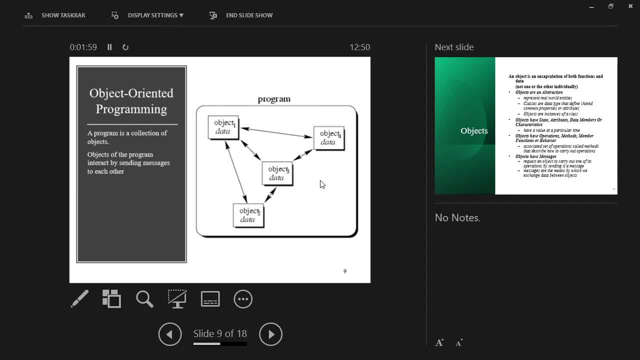 they will communicate with each other and in that way we will try to solve the problem 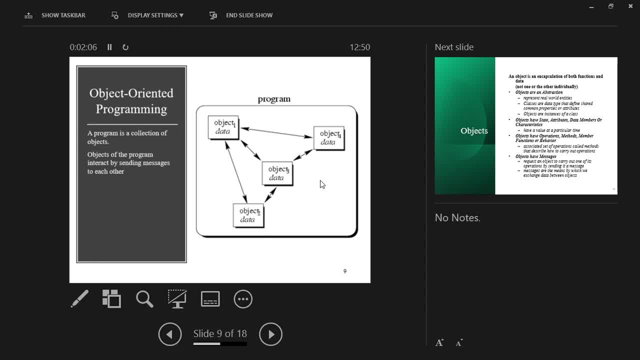 so in some situations this would be an ideal way to solve problems 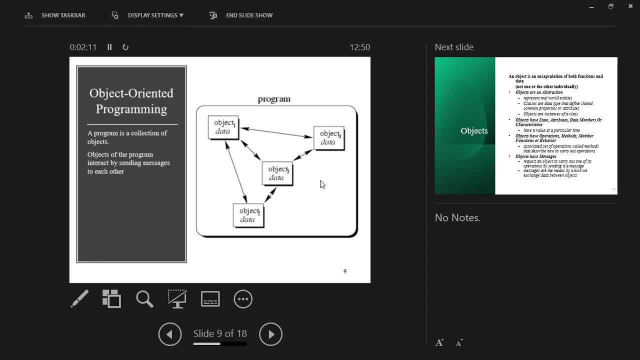 in some situations this would be an ideal way to solve problems in some situations this would be an ideal way to solve problems 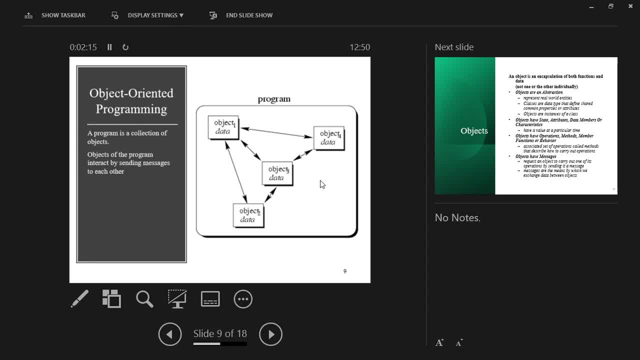 it may make things more difficult but in any cases we have our own provisions 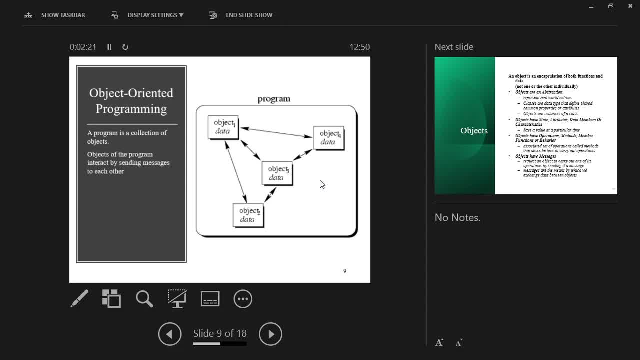 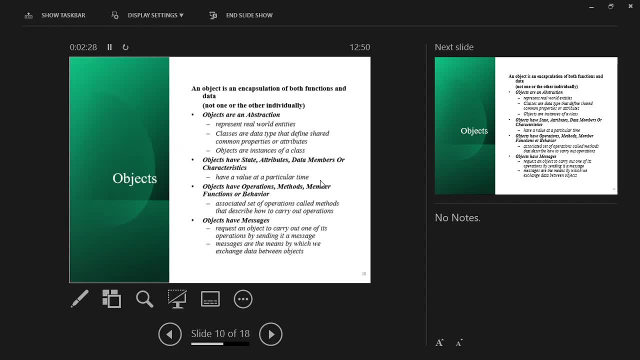 so in object oriented programming this is how your program would look like you will have different objects and those objects will be communicating with each other we will basically differentiate between 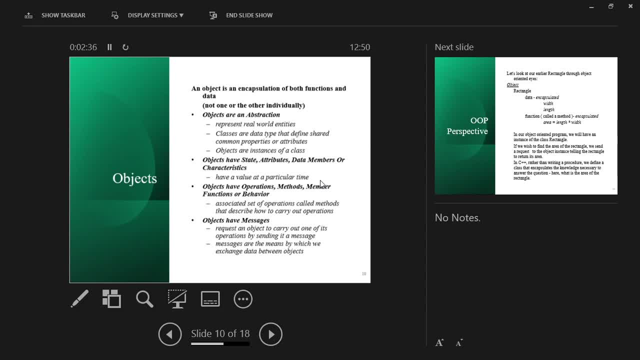 the term of the object we will define it 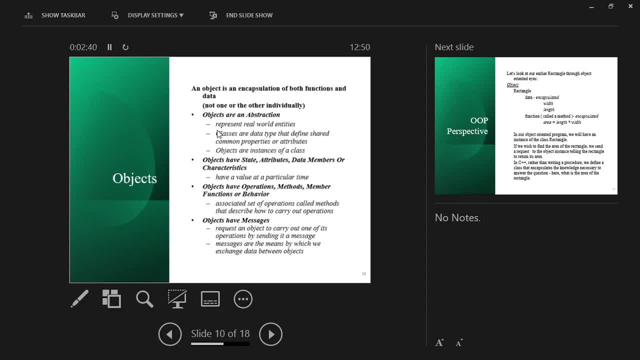 but here you can see the basic concepts of object oriented programming 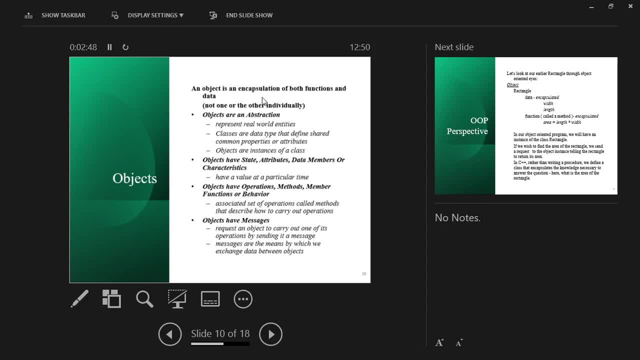 an object is an encapsulation of both functions and data just like we said before 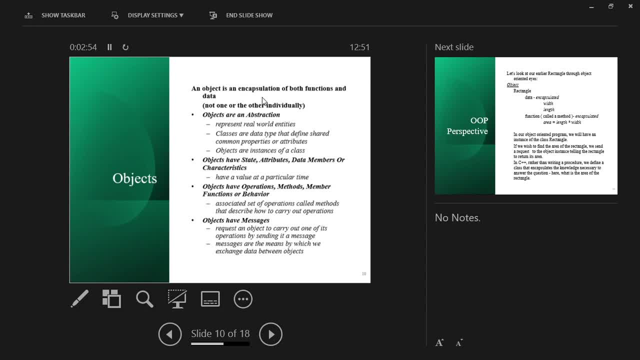 objects combine both data and functions into one the functions which operate on the data they are put together into one package 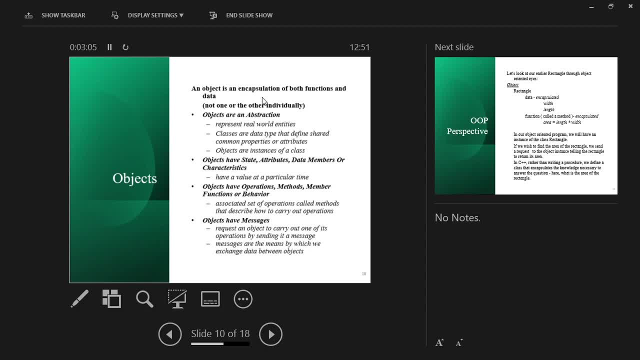 the object can receive a message from outside the message that comes from outside is basically in the form of data but we don't call it data we call it message 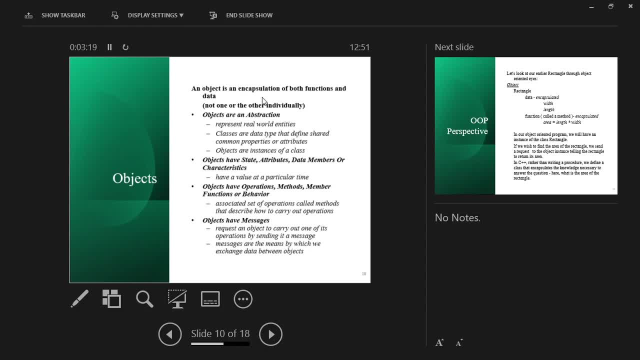 usually the objects which have to operate on the data are present in the same package 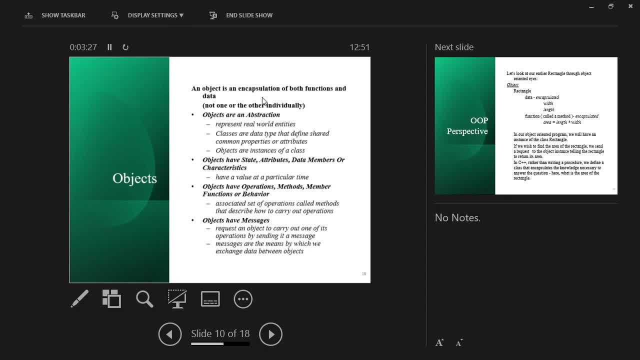 say for example I hope like you have created those you have done the first lab in this my complex class object infection class object which we have created now my complex object it has two attributes it has a real part and it has an imaginary part the real and imaginary part all those functions which can modify it or it should be accessible all those functions are accessible and they are part of one package 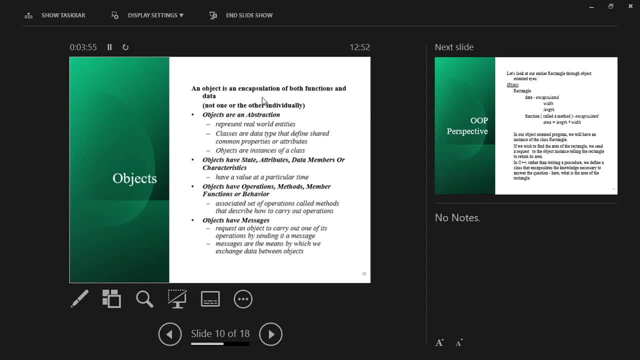 they are part of one package other than that that means 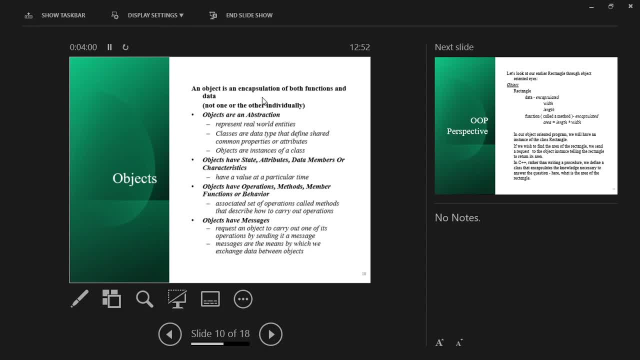 my complex object does not need to work on any other data we can have situation in which we can say 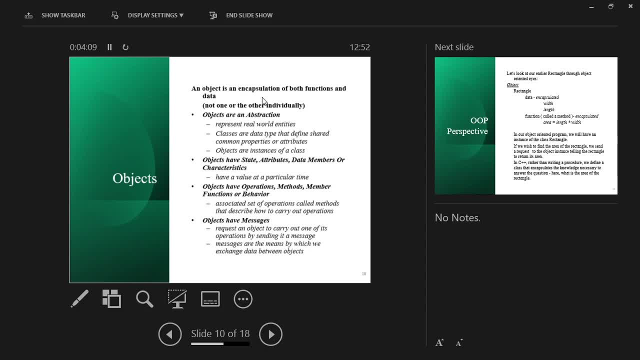 we would like to add to my complex object so in that case in that particular case then we need the messaging and in the message we can have one more copy of my complex object and we can add it ok 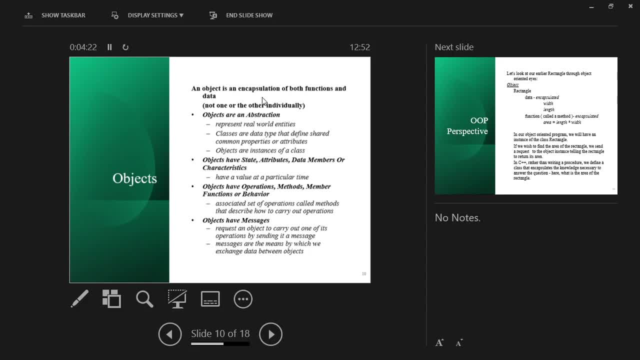 but other than that whatever object you will create 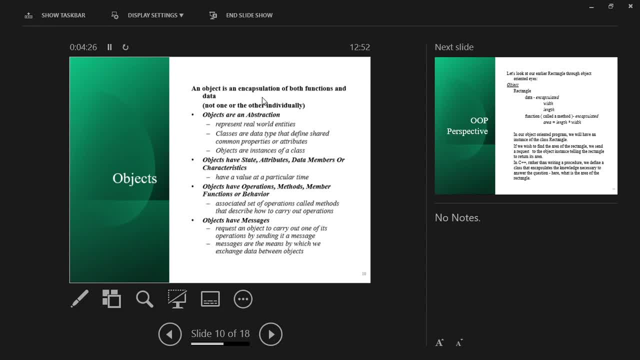 all the member functions of that object the data on which it has to operate that data and the member functions they would be part of one whole they would be part of one package 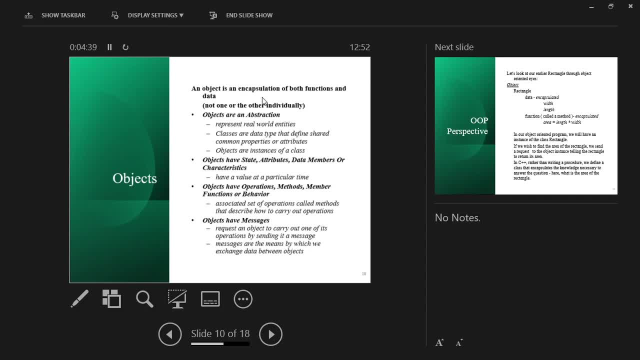 so we will create it in this particular case the problem of finding the area of the rectangle 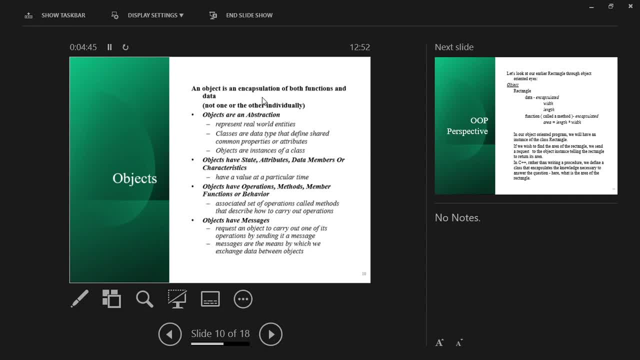 so we will solve that in the using the object oriented way and then we will see 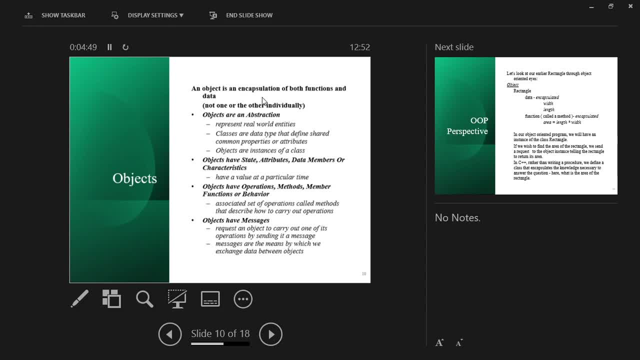 what is the difference between the two objects are an abstraction ok 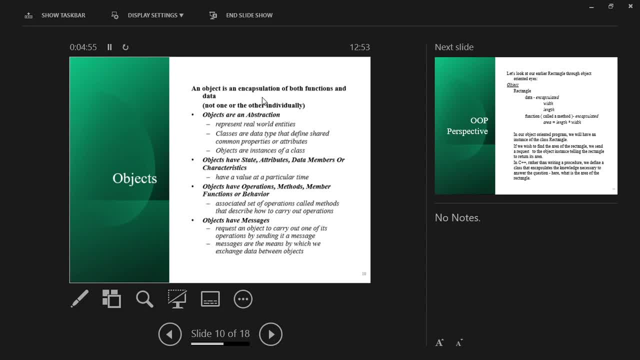 abstraction means they are not physical objects that we create so we may have an air condition this is a physical object that we can see if I have to model this thing here 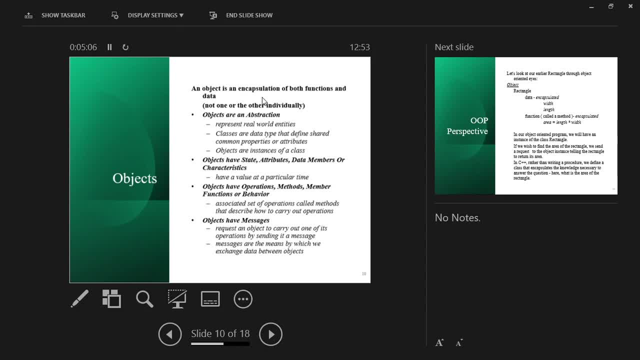 on a computer we create an abstraction of an air condition that is not a real air condition this is an abstraction of an air condition 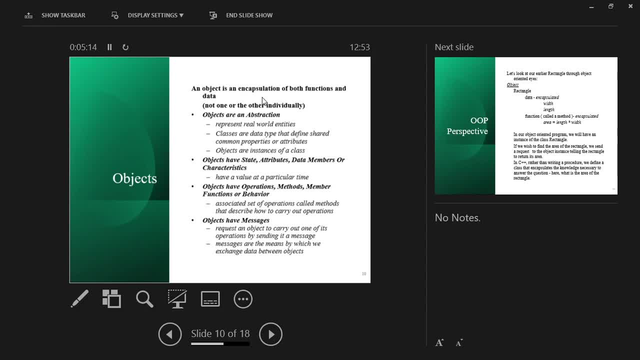 and usually like object oriented programming is used in situations where we want to model real world problems 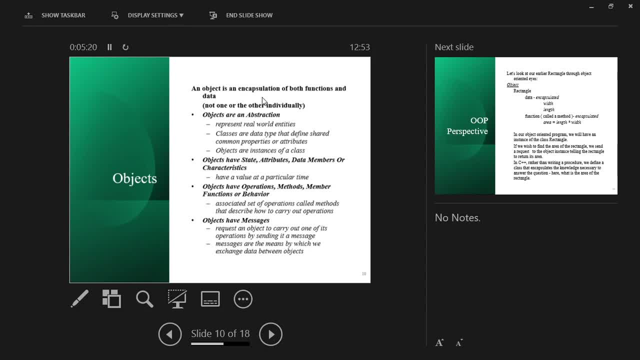 and we want to represent those those entities in the real world inside a software ok 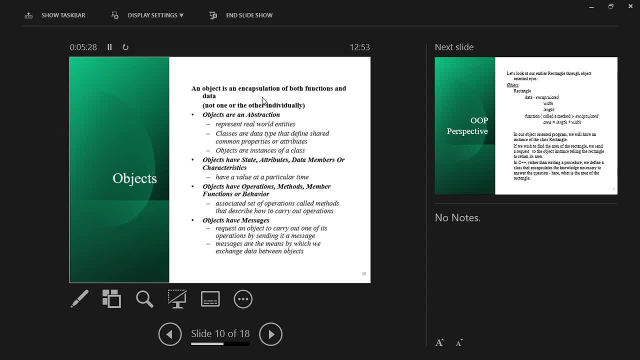 so for example all your games and simulations which are very popular nowadays so there 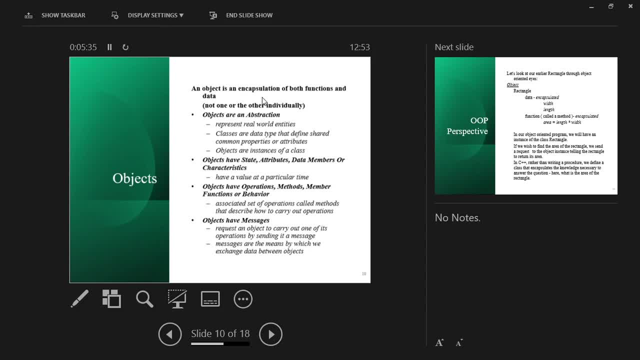 these object oriented programming concepts they are very useful ok 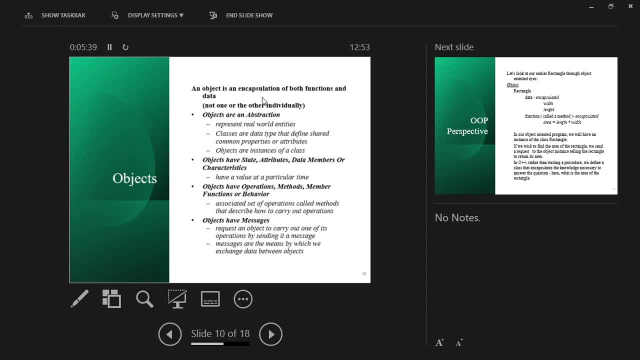 so for example if you are playing FIFA World Cup Football 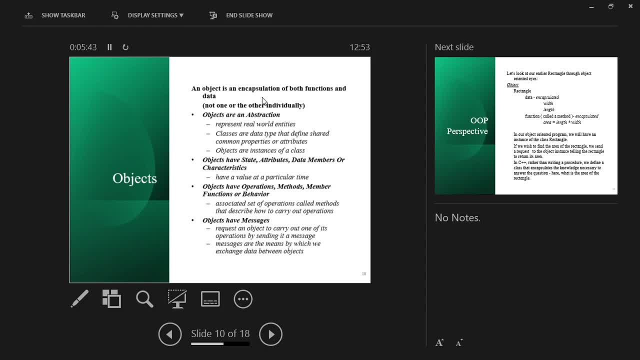 EA sports etc the game or if you play a game on a game console 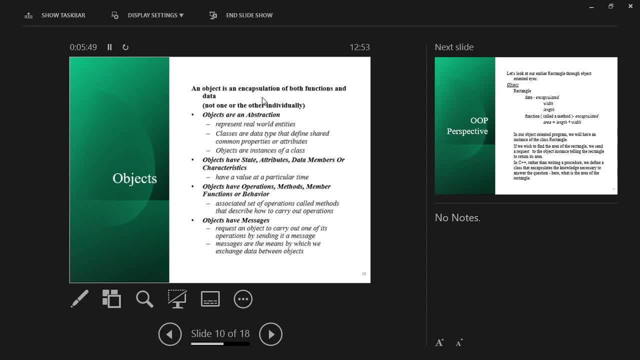 so there those games they have virtual objects so there are football players say for example 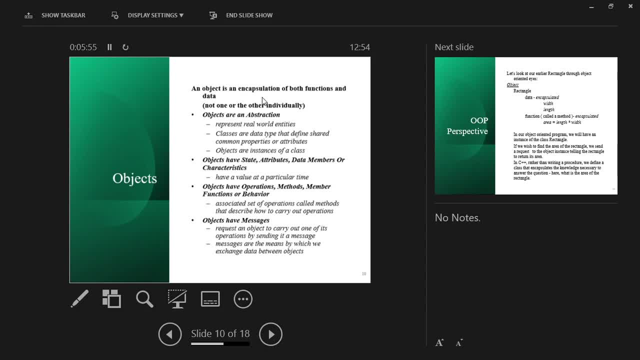 now a football player would have different attributes ok he will have a uniform he will have particular moves 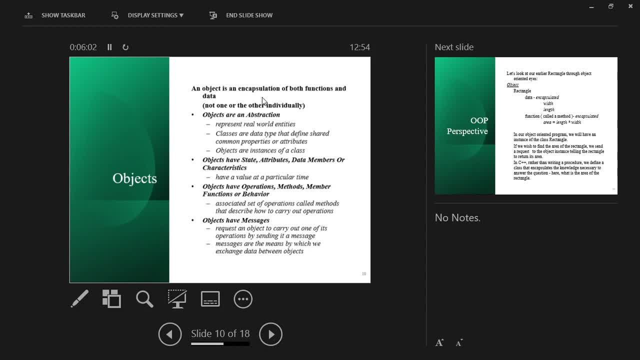 a side kick or a penalty or a shoot etc every player will have his characteristics so 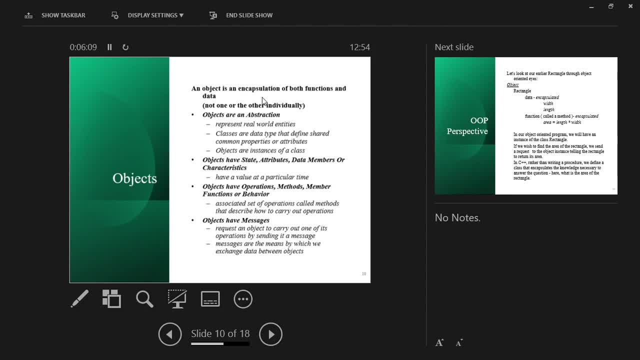 in that game you will have those virtual objects and then those virtual objects would be interacting with each other the players would be interacting with the ball ok with the field and they would be communicating 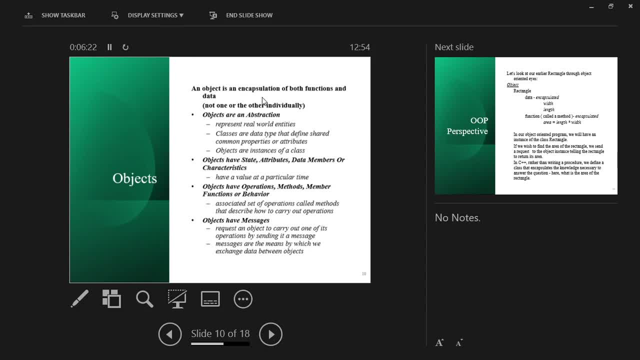 with each other so there is a virtual environment inside that thing very heavy computation is going on 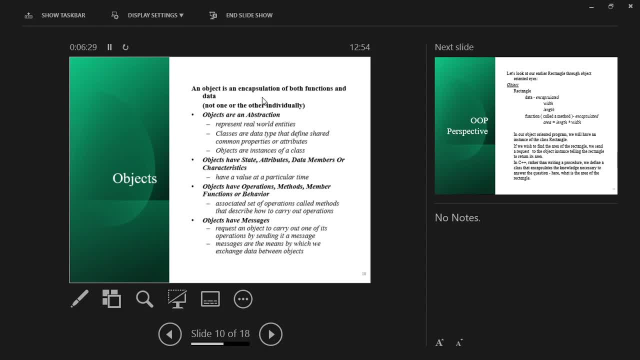 in games and they try to mimic the behaviour of real world objects 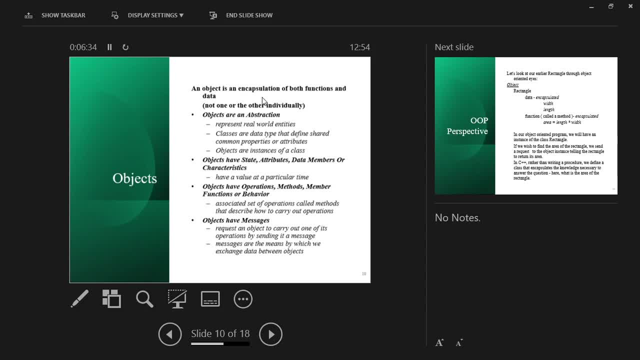 ok in that particular those particular problems object oriented programming is very useful in that thinking and processing of things 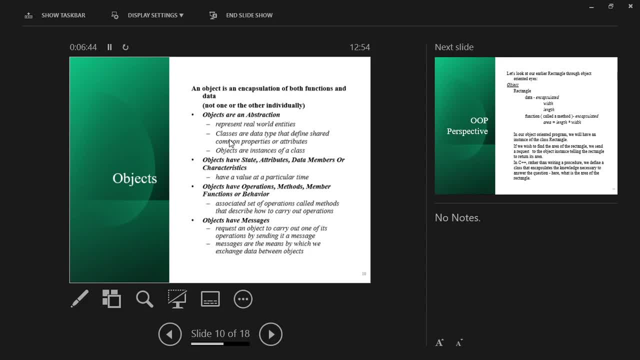 ok now when we talk about objects 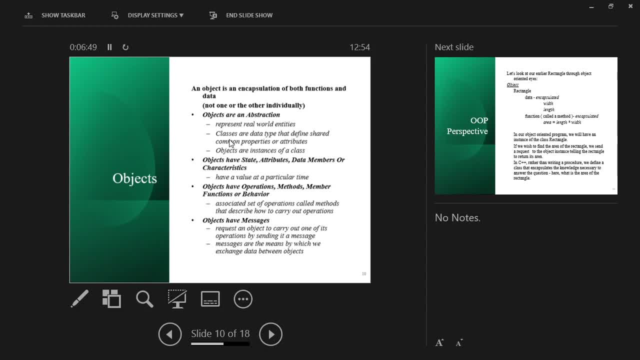 with objects there is another concept that is tied to objects and that is the concept of classes ok 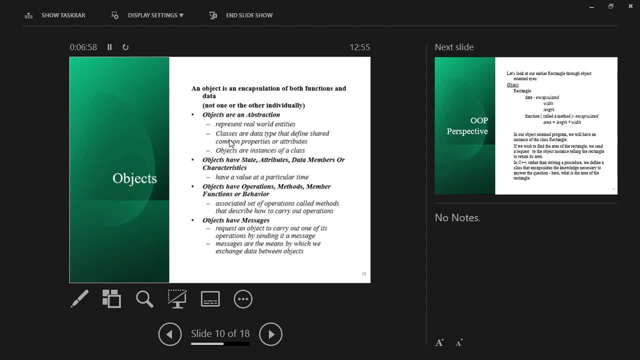 so classes are basically on the next slide we have defined that classes are basically 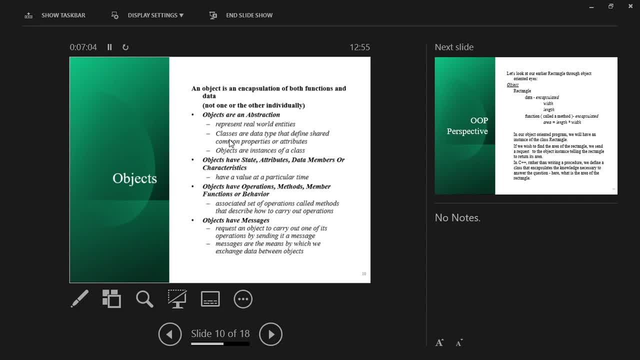 maps or specifications or blueprints ok and objects are physical beings like you have a map 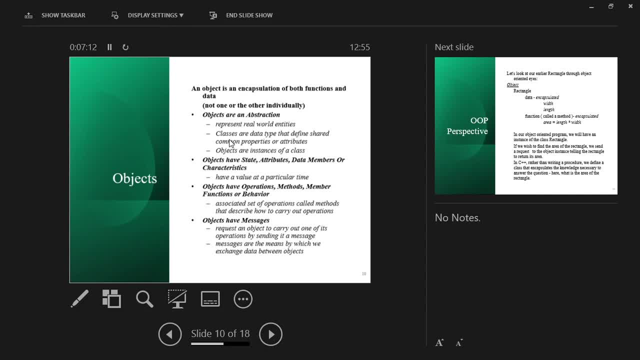 the map of this building so whenever you need to create a building first you construct you construct that building you create a map for that building first you make a map ok 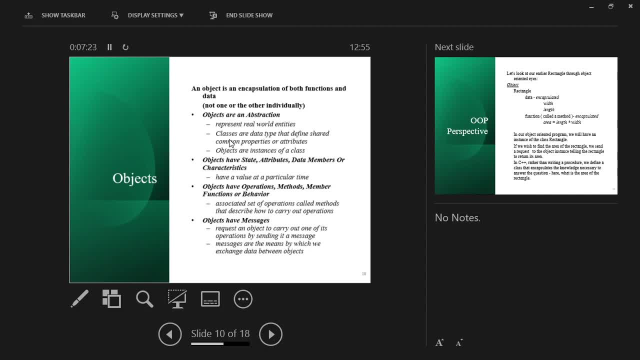 how many rooms will there be what will be the dimensions of the rooms where will be the beams what will be the dimensions of beams 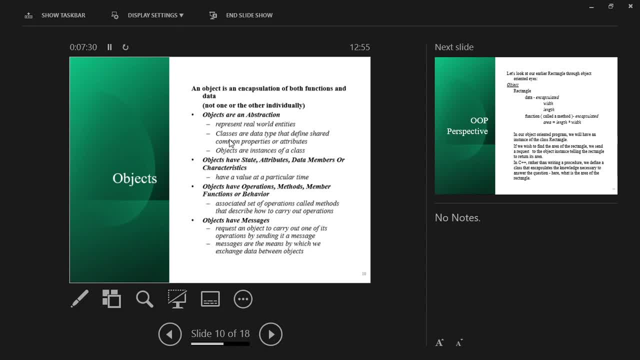 what will be the specifications so a map is a complete specification but it is a map 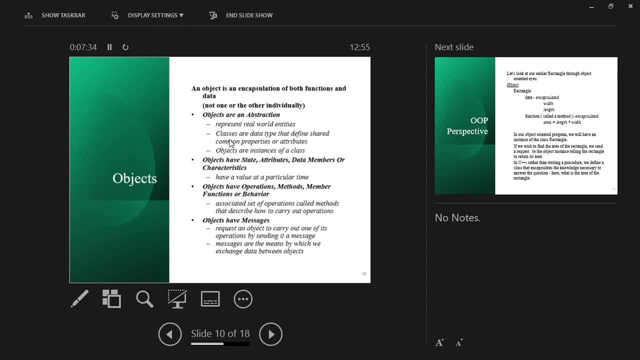 you cannot live in that map you cannot go to classes in that map it is still a map using that map then you create a physical object so this particular building is a physical instance of the map ok 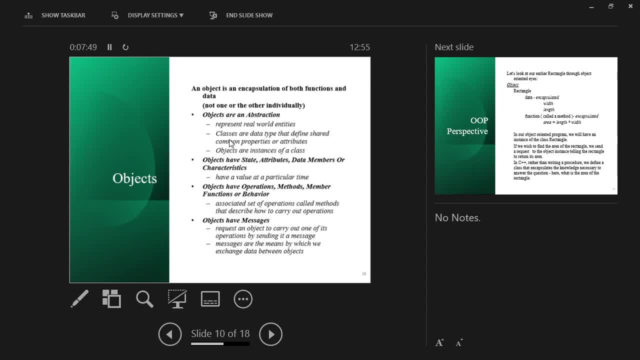 similarly when you are programming so first you you write the class first you write the class definition you specify that what will be the characteristics of the objects of this class and what will be 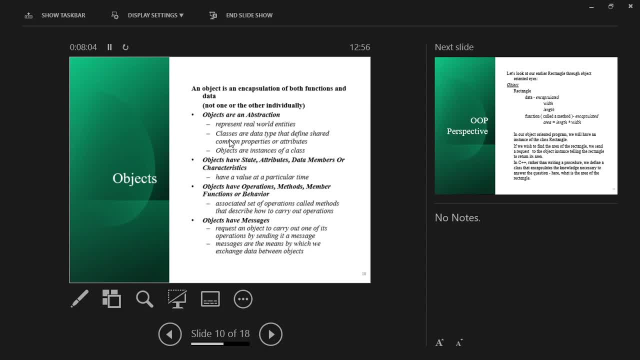 their behaviour so in a class you specify two things the attributes or properties and the behaviour or methods 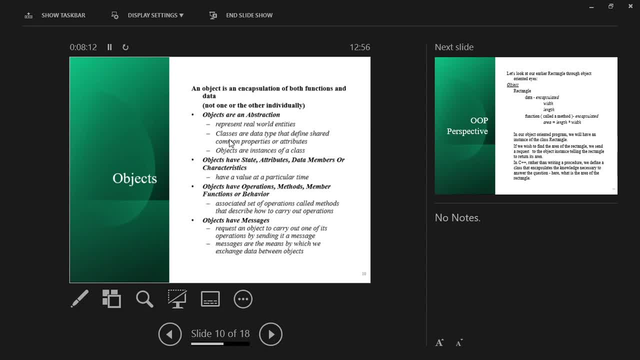 so we use these different terms for that ok so first of all we will be writing a class 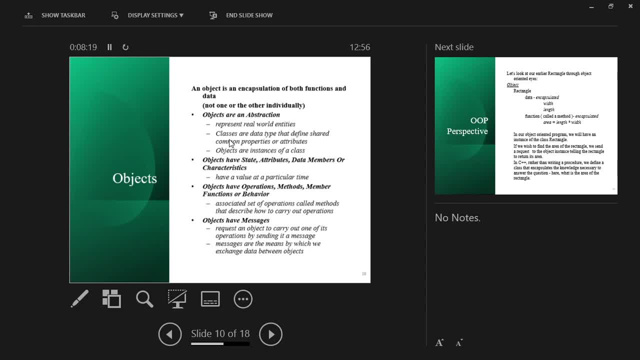 but after writing the class automatically nothing will happen 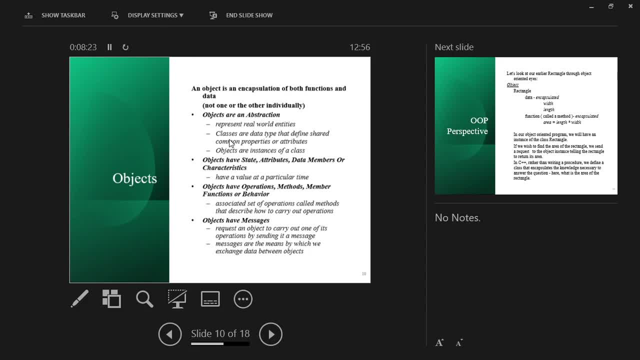 in order to use that class you have to create objects of that class like this map of the building 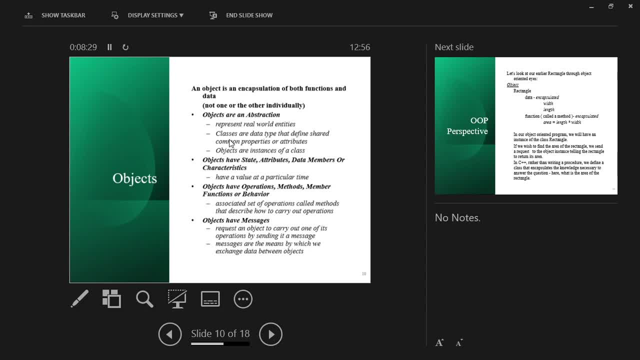 so we cannot live in the map to live we have to build an actual 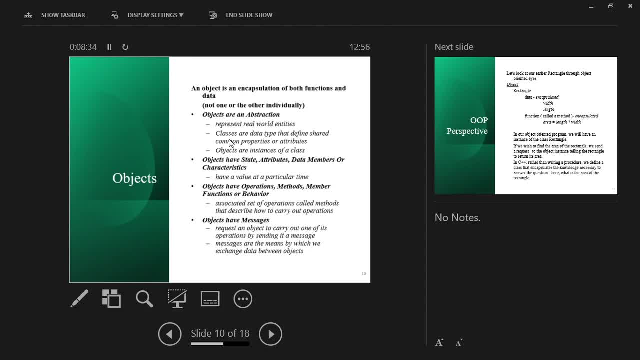 building then we can use it ok so objects are an abstraction but you create these abstractions by first writing classes or specifications for these objects you first do that and objects are then basically instances 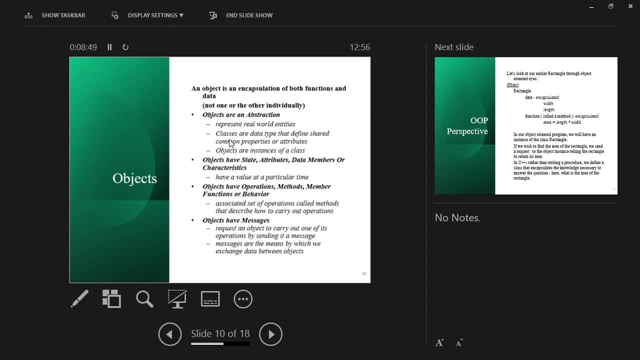 or examples of that class it has a physical entity or instance in the context of programming and computing whenever we use the term physical object physical object means that 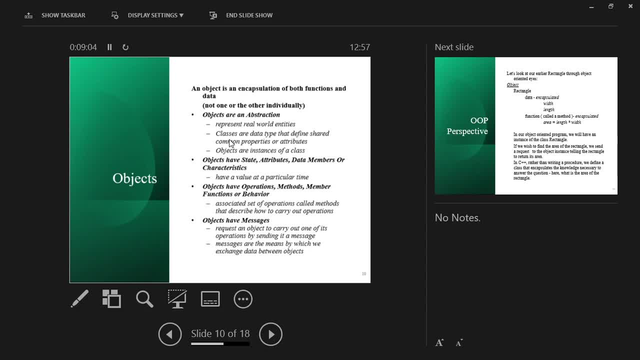 it is allocated in random access memory so that object then exists in your random access memory computer's random access memory ok so objects are physical beings in the sense 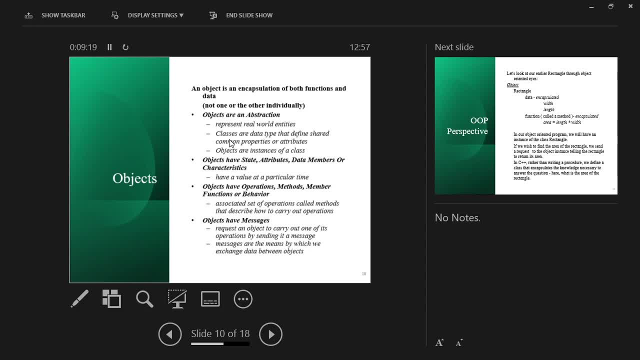 that they exist in your RAM computer's RAM and classes they do not like exist in RAM classes are like in your hard drive 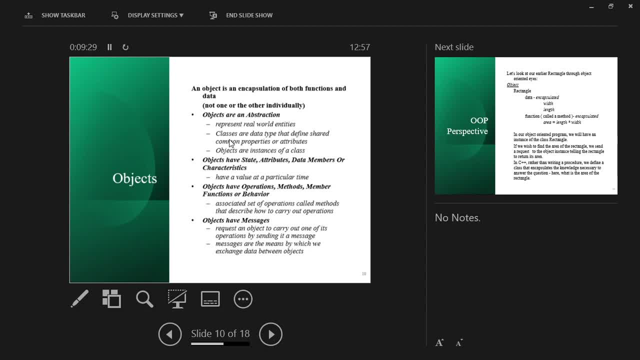 the file in which you saved them something is there ok 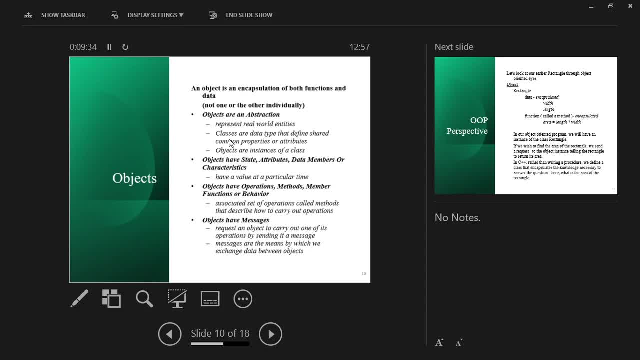 and then you use to create an object so then it refers that file and based upon that specification it creates an object and that object then exists in RAM so you will have 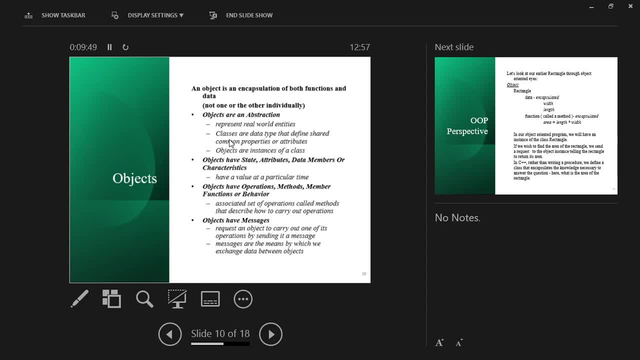 one class definition and based upon that class definition you can have tens of objects of that class ok like you can make 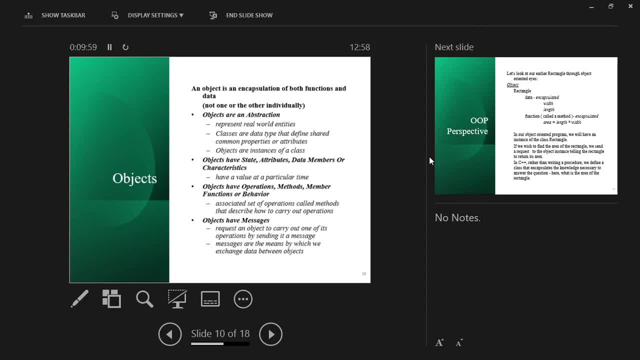 one map and 20 houses of that map on its basis ok 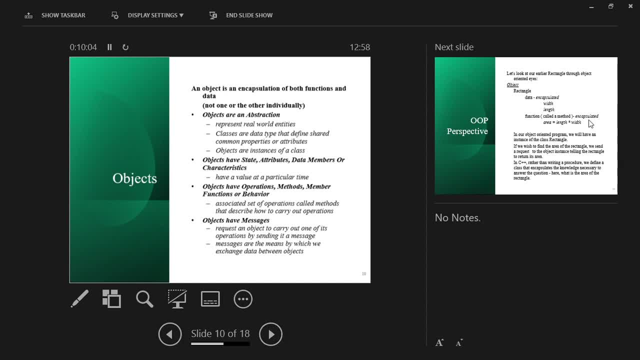 so remember these terms these terms are written here objects have state and attributes data numbers and characteristics here we give one more name which I have not written 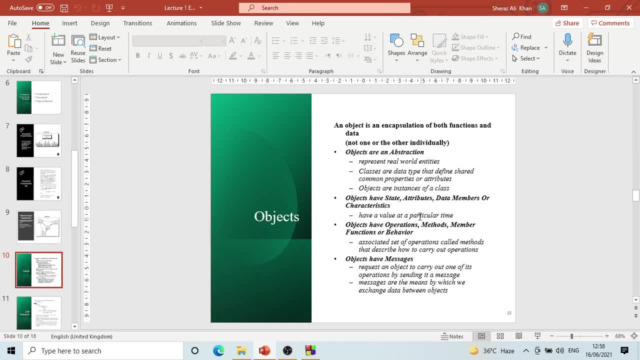 here properties ok objects have attributes state attributes data members and in fact instead of characteristics this is what we have 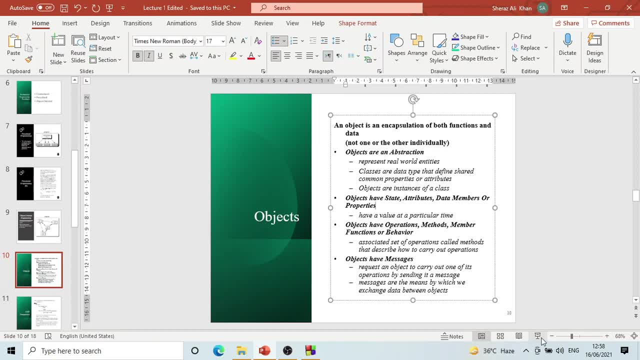 ok what does this mean that you have created my complex object it has two attributes real part and imaginary part 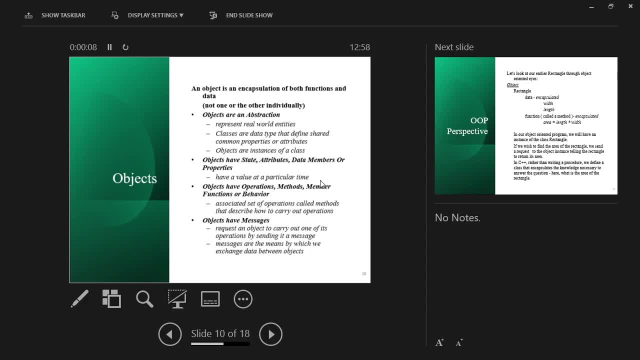 if you were to create an abstract air conditioner 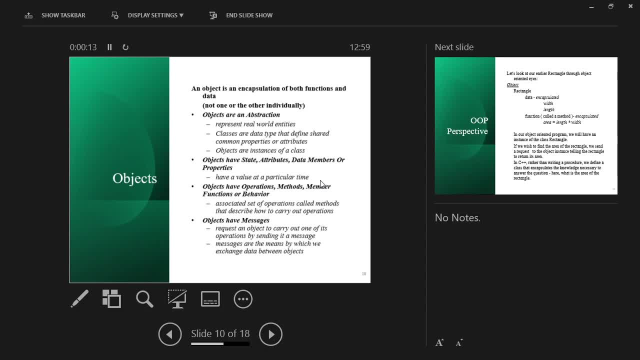 object for example then it has different attributes one it's tonnage or BTU value how much BTU heat can it extract 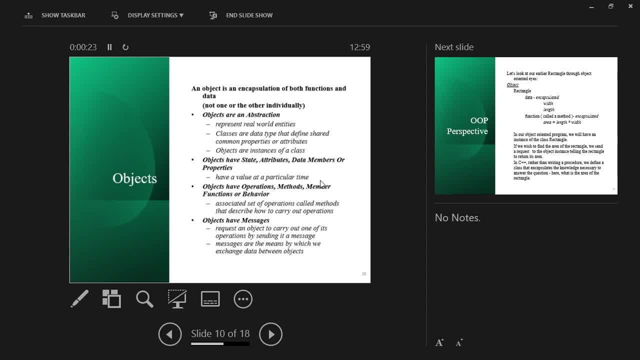 ok it's power rating its maximum or startup current 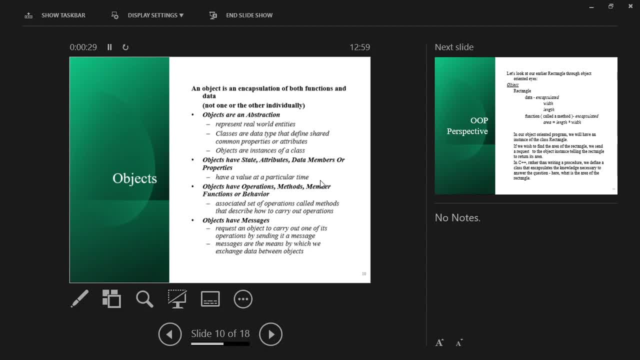 how much current ampere current in startup average current how much it does all its characteristics so 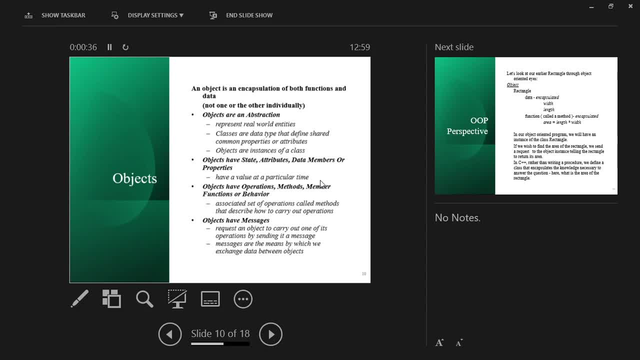 color different things can be for example if you have this multimedia projector so it can have different attributes 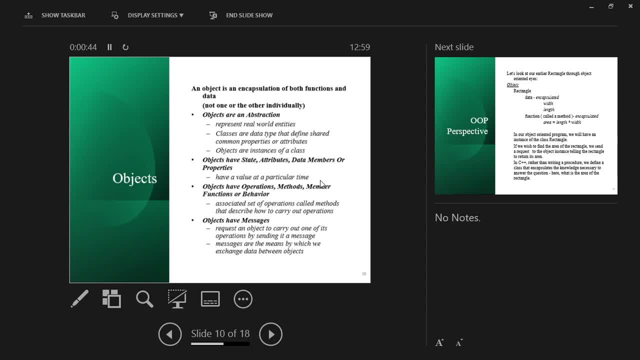 for example its resolution its make its length life its operation hours etc etc so you can have all these attributes it can have attributes it can have state it can have 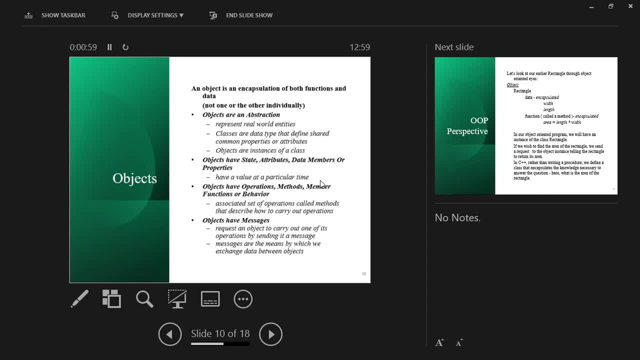 data members it can have properties so they are all different names but they mean one and the same thing 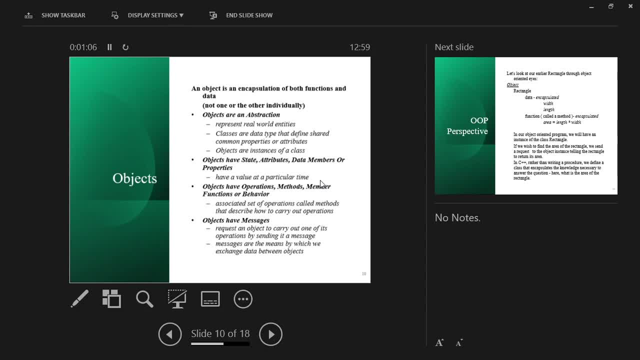 and to store them you declare variables to store them you declare variables so the variables of procedural programming in object oriented programming 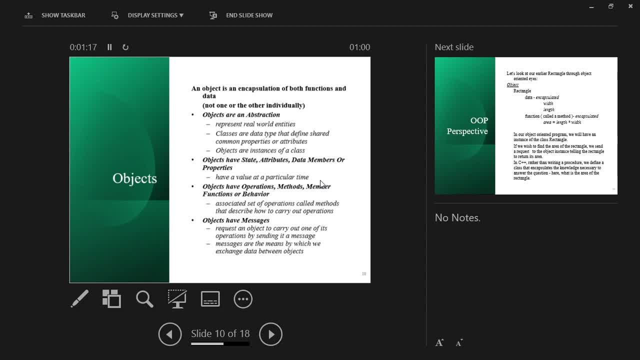 they become state they are used to store the state information or they are used to store attributes or properties 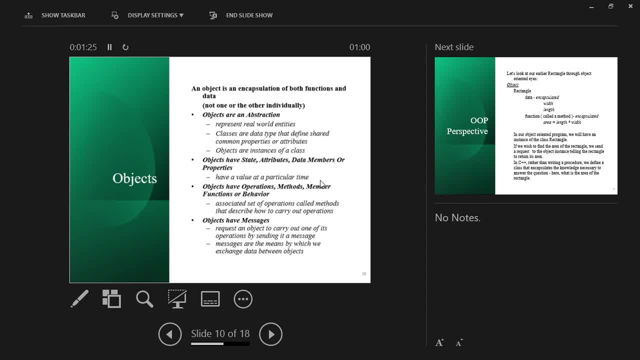 similarly objects have behavior behavior means you can turn on and off this air conditioner you can increase the fan speed decrease the fan speed increase the set temperature decrease the set temperature this is the behavior for this object similarly 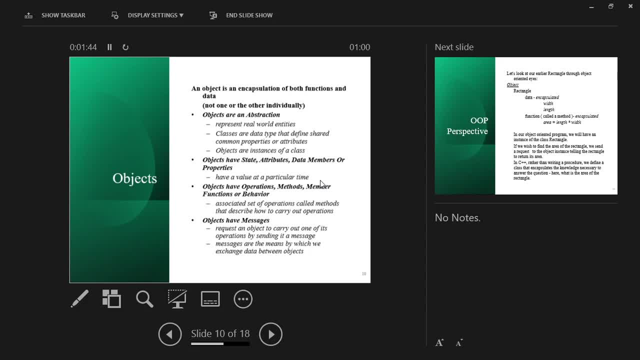 you can put it on swing both in vertical direction and horizontal direction this is its behavior it is a method by clicking a button either vertical swing or horizontal swing ok so you pass a message and it acts in that particular way ok 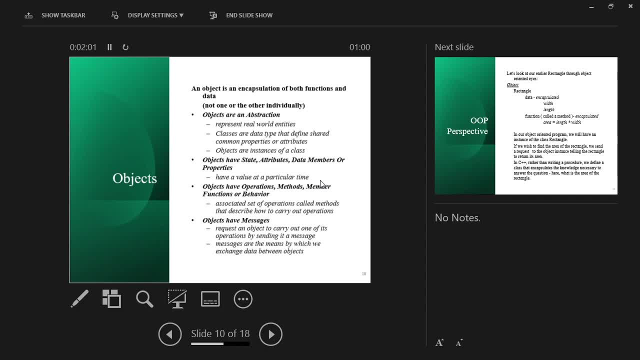 so objects have state or attributes or properties or data members and objects have behavior we also call behavior methods we also call behavior member functions 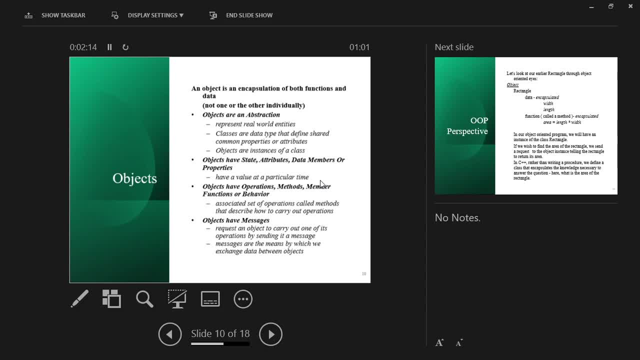 ok we also call behavior operations these are all different names now what is 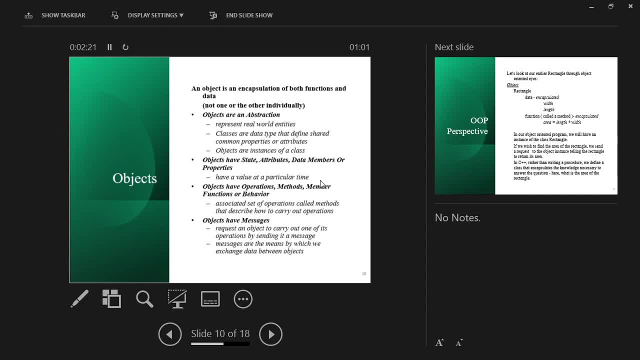 it it is basically a function that you write ok so I will demonstrate what it means so objects 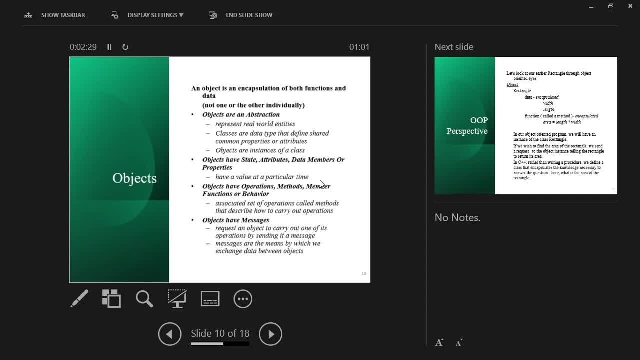 when two different objects when they are they want to access each other's facilities so they pass on messages messages means that one object calls another 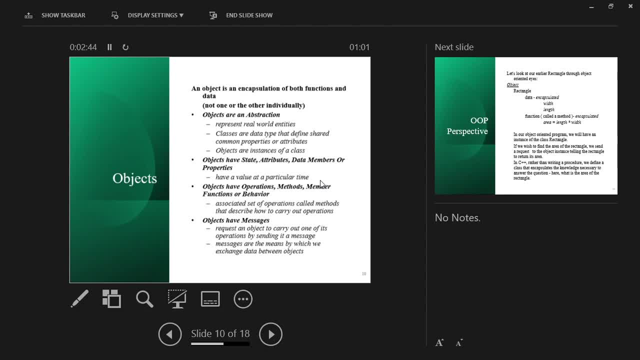 object we call that call passing of message ok this is just a term otherwise there is no such thing so let us solve that problem using this approach 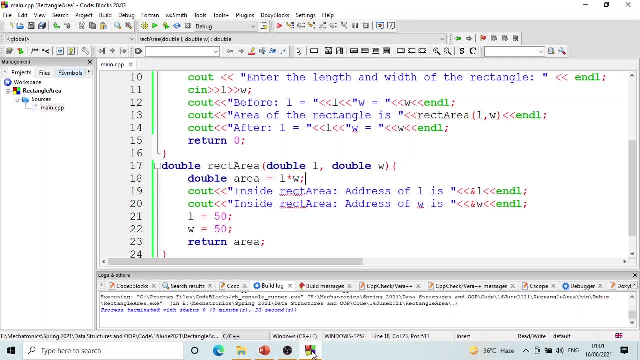 so now we want to solve the problem of finding out the area of a rectangle using the object oriented way ok how will we do that so again we demonstrated that how to do multi file programming ok 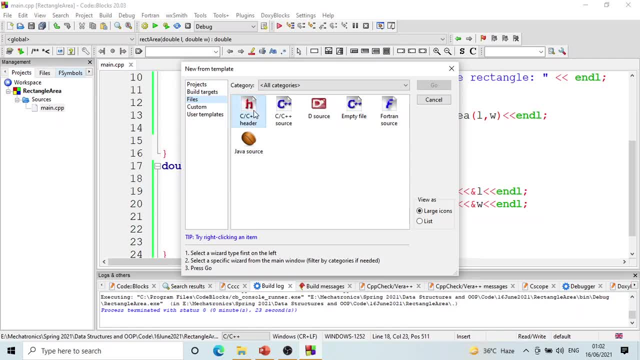 so let me add a header file first we will add a file in this project and in that header file yes ok 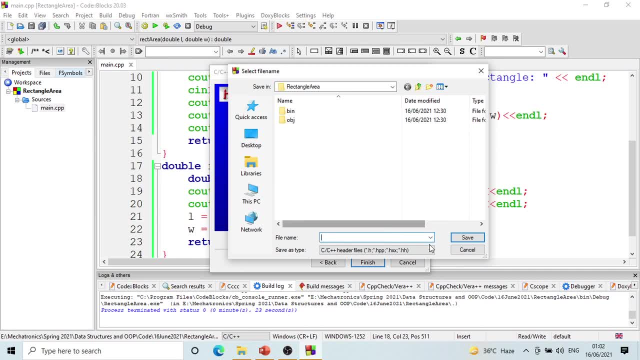 let us give a file name to it 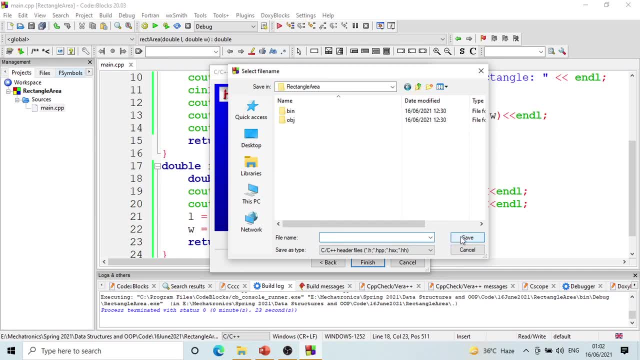 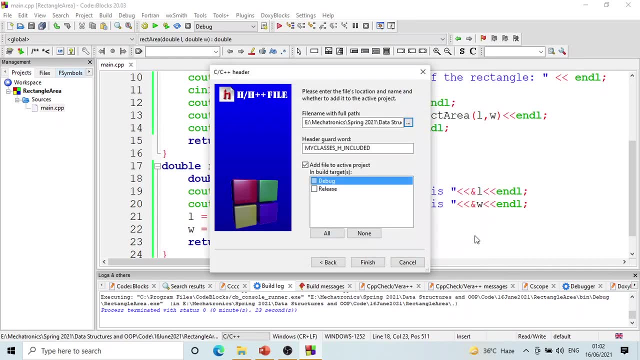 say my classes ok we will remember the name of my classes later ok so in the 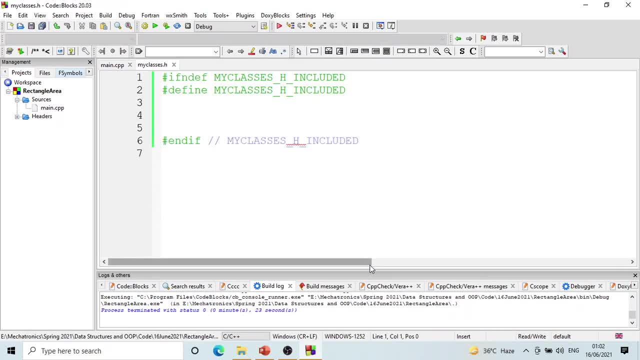 object oriented way we will find the area of a rectangle so for that we need to have a rectangle object a virtual rectangle object 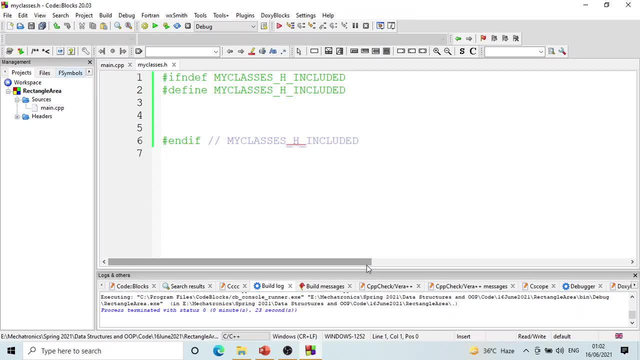 and we will ask that object to calculate its area there will be two attributes of a rectangle its length and its width and then we would invoke some method 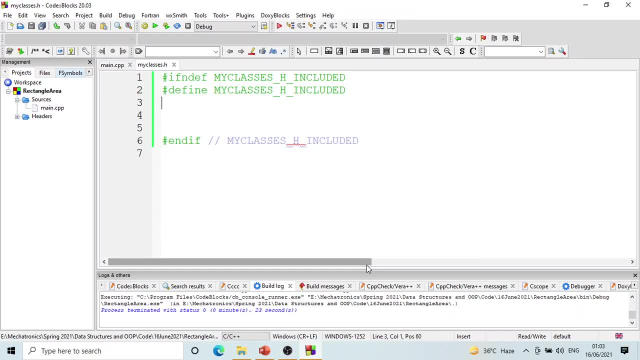 of the rectangle object and it will be a rectangle ok 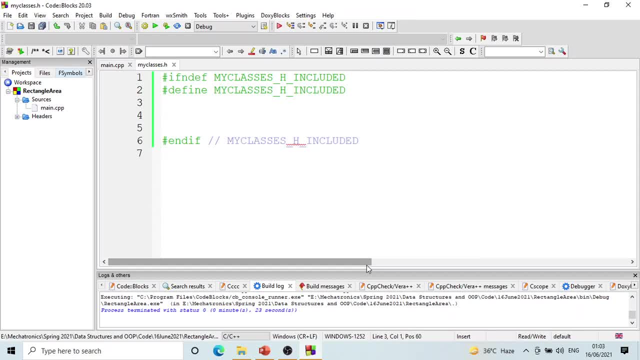 so first we have to write a class ok 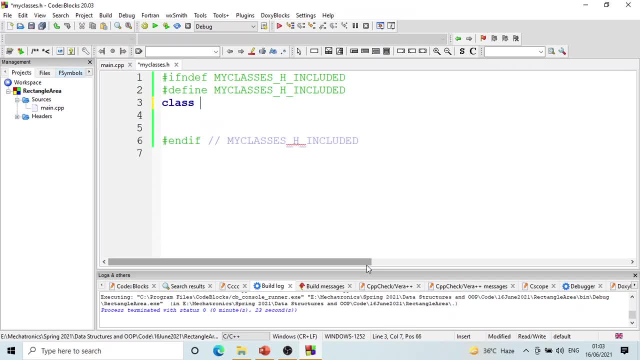 we have to write a class definition how to write a class definition so you have seen one demonstration so 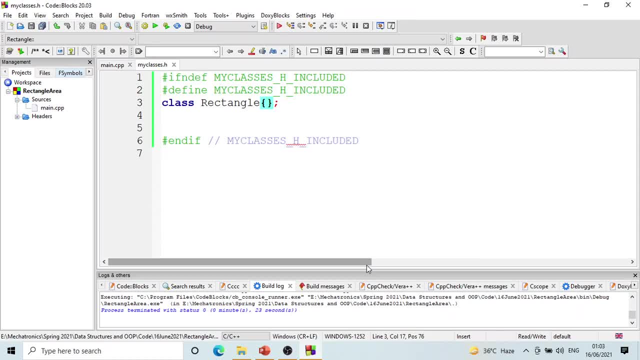 how do you write a class definition this is the simplest class it does not have any 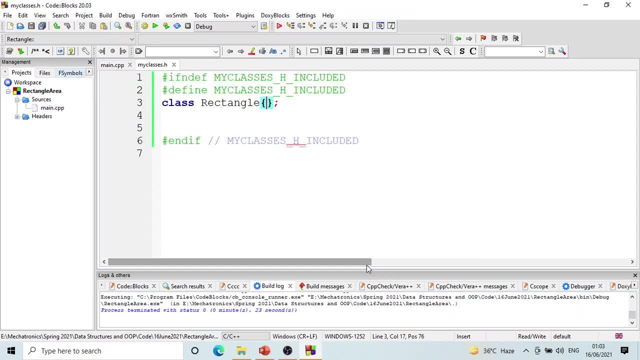 behavior any property but it is a useless class but technically from a technical point 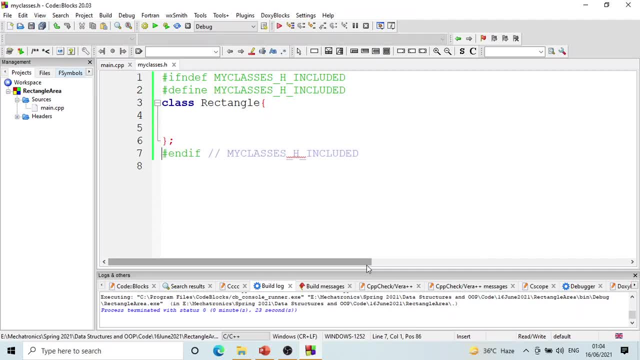 of view it is a simple two dimensional geometric figure it has two characteristics its length and its width ok 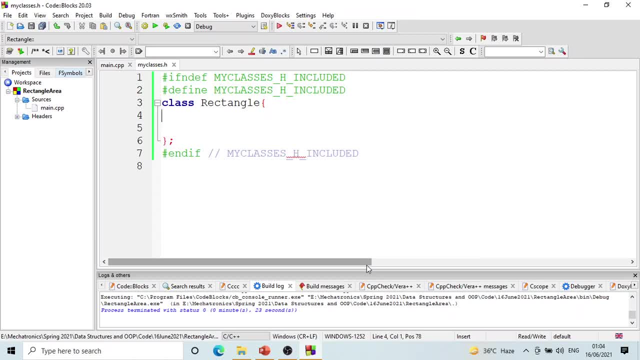 so I don't know whether we have discussed it or not have we discussed private or public ok 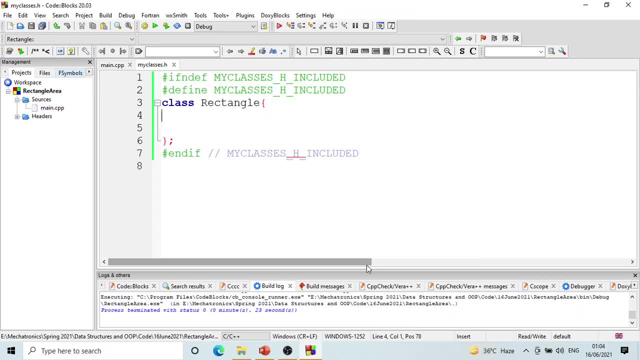 so usually any attributes 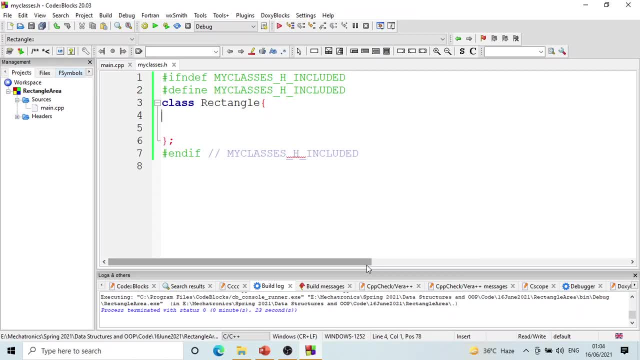 of those attributes are kept private ok what do you mean by that it means that you cannot change the 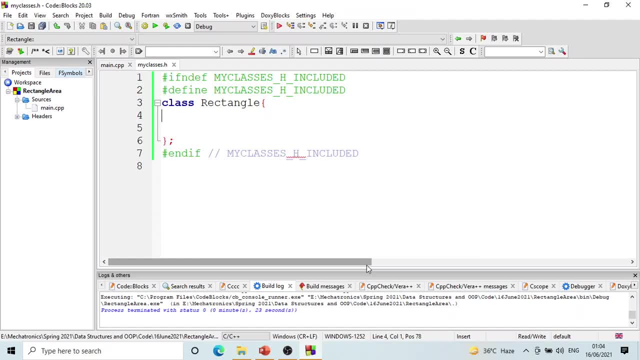 attributes or you cannot access those attributes directly the purpose of keeping attributes private is that you cannot 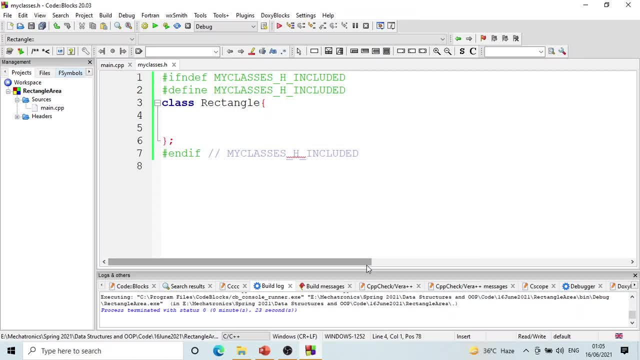 change the attributes and that is why you don't have any space to keep the attributes so 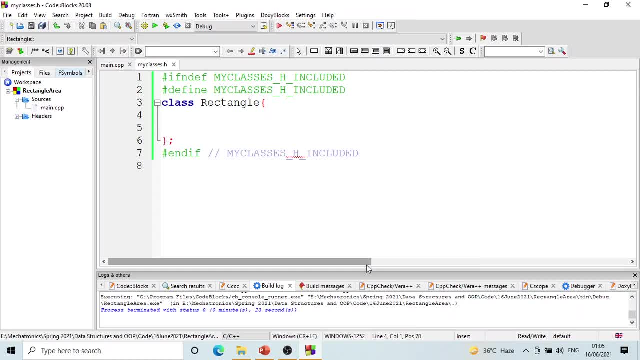 you cannot use any objects for your work and you cannot keep this in 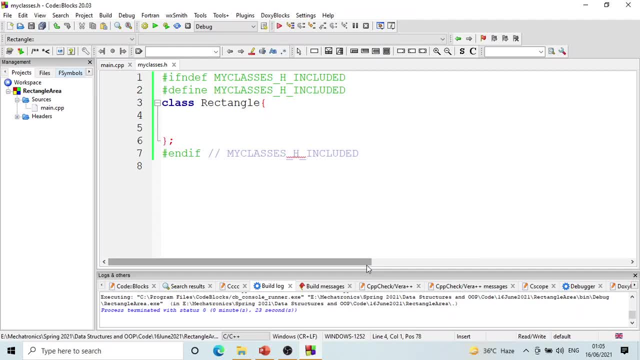 30 degree celsius is the maximum 30 ke upar go nahi jaega set temperature you cannot go beyond 30 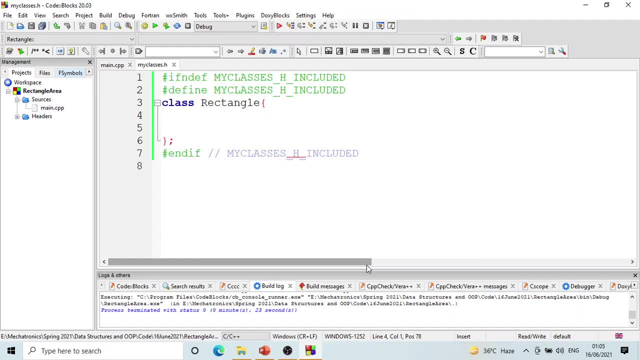 degree celsius say for example or minimum temperature 16 se niche nahi aapka for this 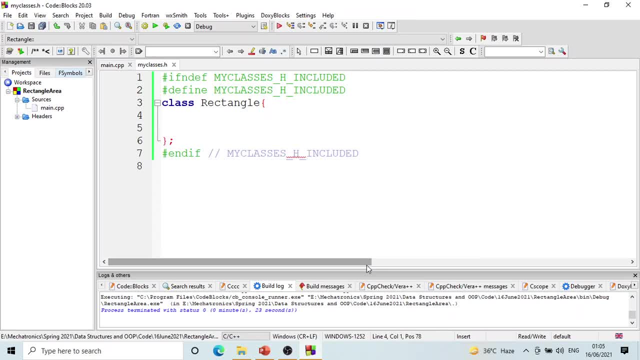 particular air conditioner so how is this possible it is possible ke aapko set temperature ko direct access nahi nahi gaya ki aap jaye aur waha pe jo bhi value punch in karne hai wo punch karne 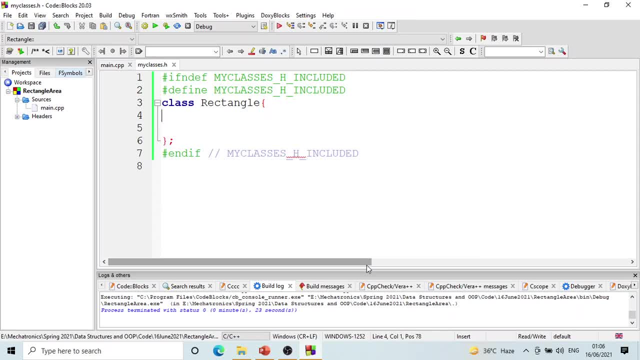 aur wo ho jaega aisa nahi you have been given a very restrictive interface aap button press 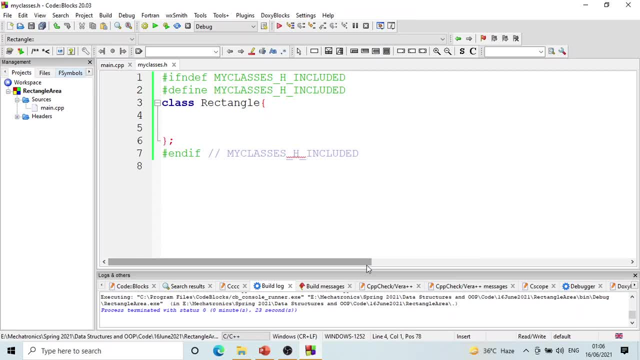 karte hain wo set temperature ko dekhta hai ke set temperature is par kya hai 16 hai aap usko 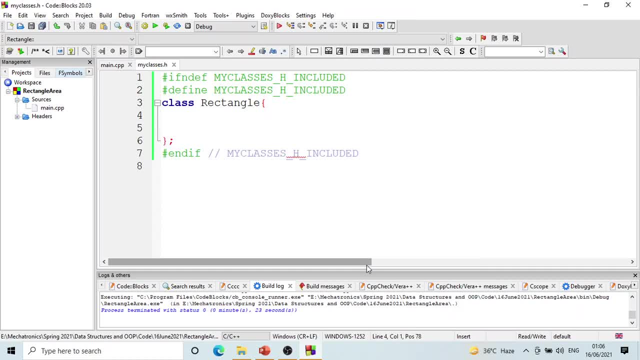 mardeet decrease karne ja rahe hain wo pe aapko decrease karne nahi dekha ke wo already 16 hai 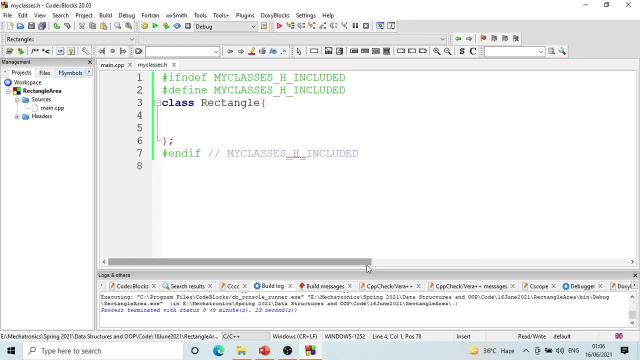 agar aapko direct access hoti then you could put any value in there chike so data numbers are 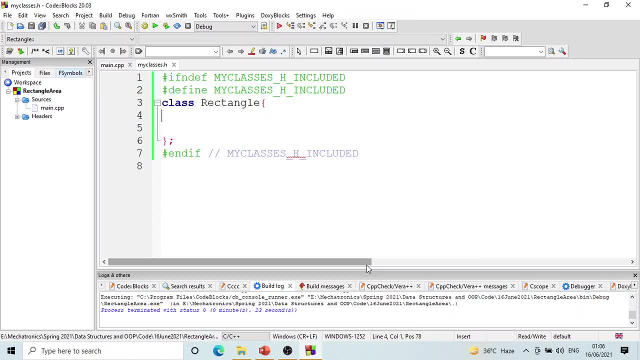 always kept private and there is a reason reason is ke you need to validate jab bhi wo data number 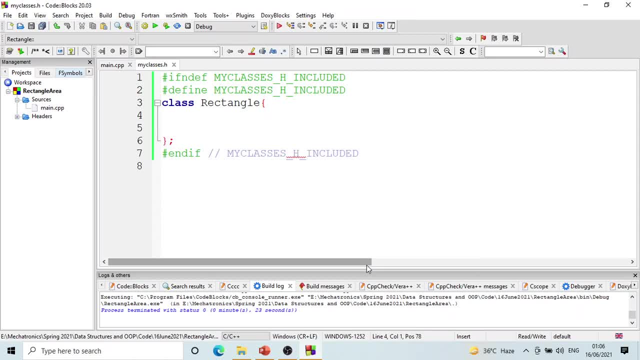 ki koi value set hogi aap us value ko set karne se pehle usko validate karna chahte hain is this 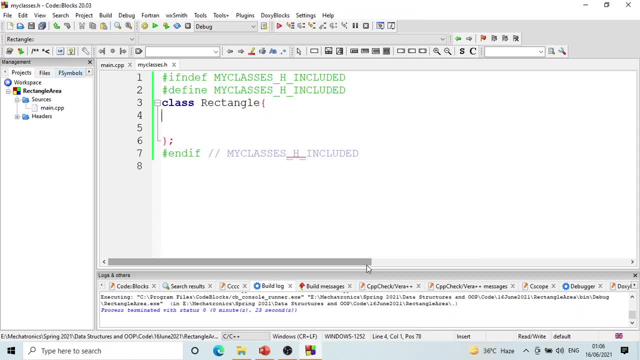 a correct value or not chike for example yaha students hain i have a database for students 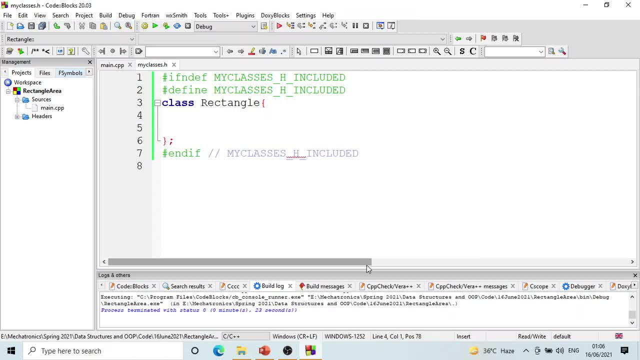 and mai unki date of birth unke baarame information store karna chahe ho and then we want to save 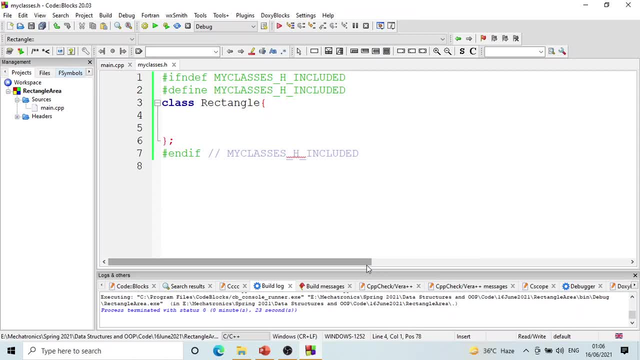 information about their date of birth aapko yeh ke date of birth ki chi ki 1600 enter karna 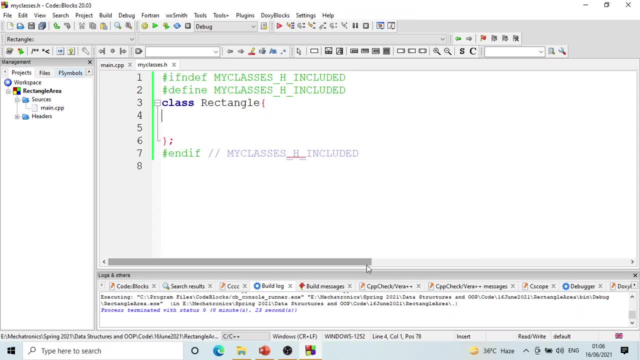 chahte ki yeh 30 june 1632 ko kaida hua hai so this is obviously incorrect university jo na wo 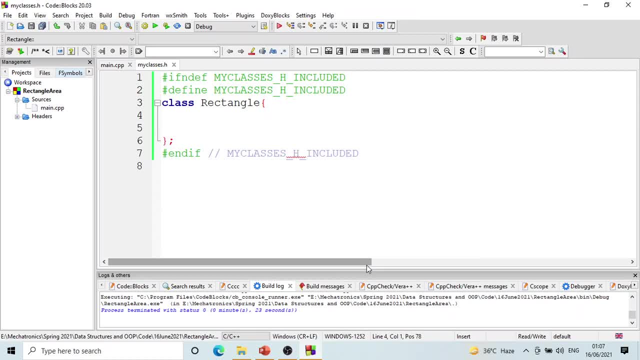 1982 mein bani thi say 1952 se college hai to maximum humaara cost 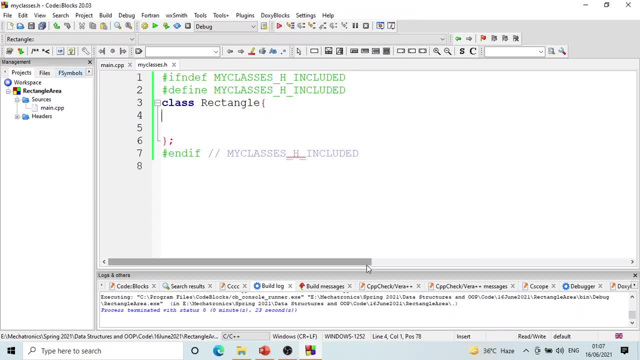 se purana jo banda aayega to wo 1900 sadi mein ho na chahiye 1800 karne aasakta usse pehle karne aasakta 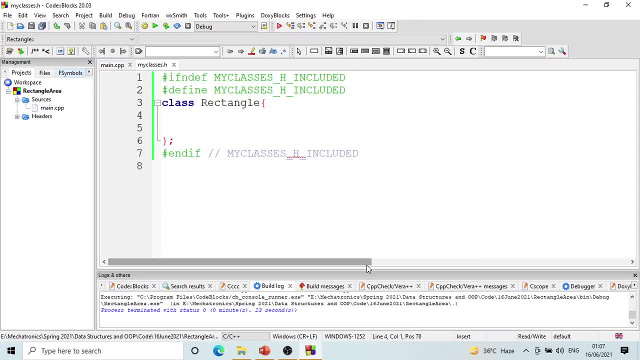 chike this is data validation this is a very important part of any software system yeh software 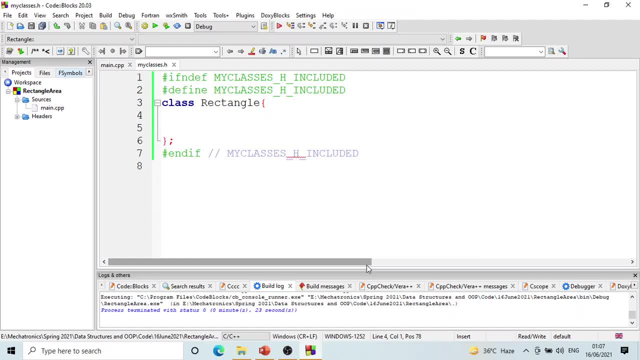 system agar koi data se store kar raha hai ya save kar raha hai it should validate that data ki aaya yeh value reasonable hai ya nahi hai chike so objects ke attributes ko private rakhne ka maksad hai ki you should be able to validate those attributes chike aacha to hum pehle attributes define karte hain but attributes ko hum explicitly private declare karte hain ki yeh private hain 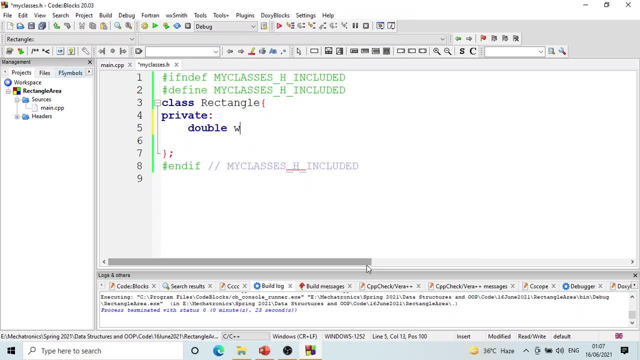 do attributes hai rectangle object ke one is width and the other is length yeh iske attributes hote chike if you remember humne iske liye wo functions rakhe the chike get width get length set width set length get function set function 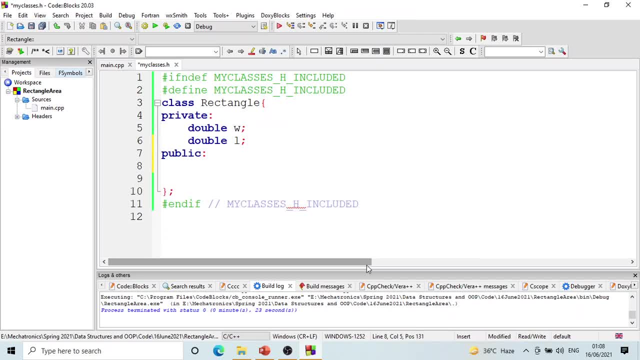 attribute to humne private rakh liya aap bahir se usko koi access nahi karsakta lekin aapne usko change to karna hai na chike so usko change karna aur read karne ke liye you have to define separate function so one is say double get width 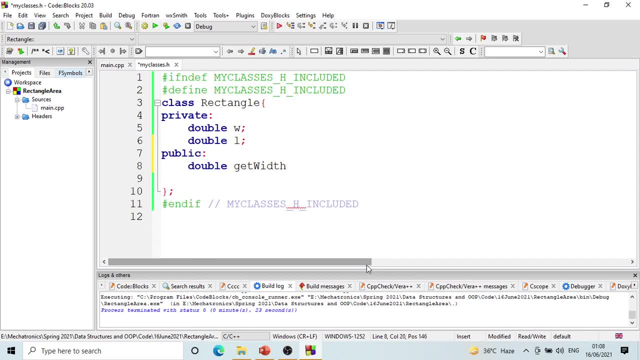 chike aacha yeh kya karega this would read the width value return w main yeh code yahi pe likh raha hu chike isme usme nahi kar raha hai similarly get length so this would be return l aacha void set length so isko ek double value milegi chike 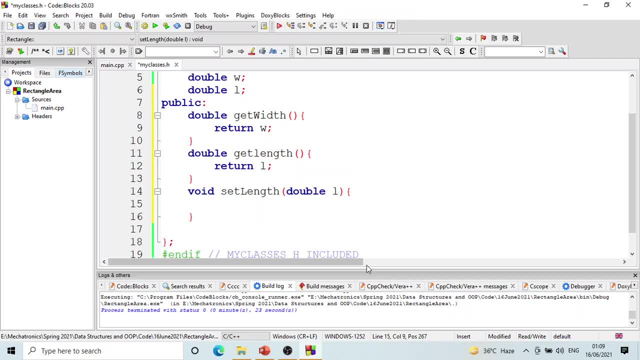 aacha now rectangle can not have negative length chike so this is the validation that you need a rectangle cannot have negative length length is always positive width is always positive so here you can put a check chike if 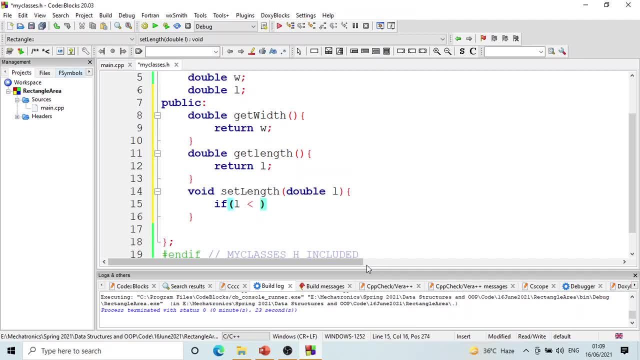 l is less than aacha isko thoda sa change kere dete hain length if length is less than zero sorry 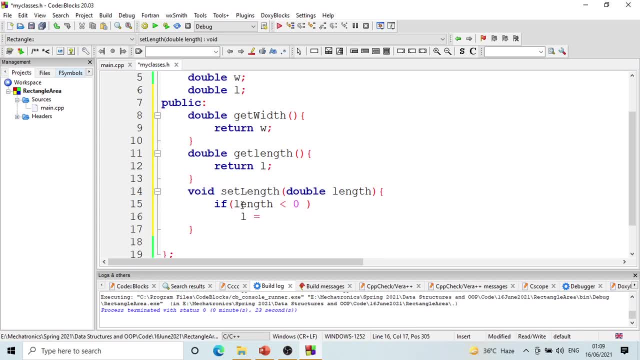 so l should be equal to aacha minus length 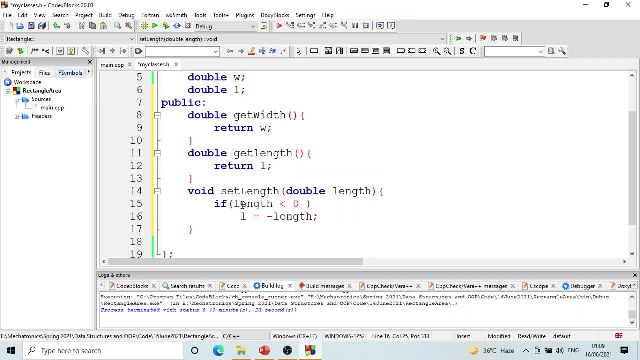 chike yaa isko khatam kardein phir uske liye hume wo maths library import karna hogi chike let us keep it this way else l is equal to length chike and similarly we will do this we will write the same code for 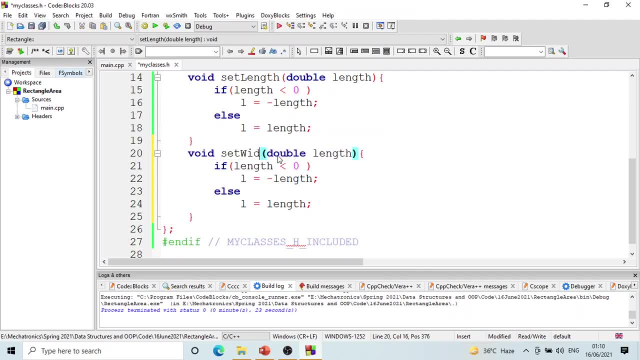 width as well set width width width so 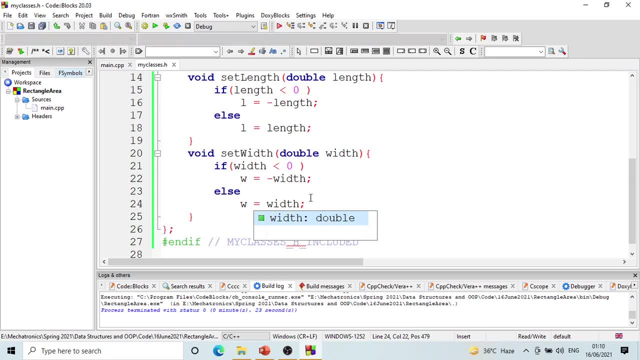 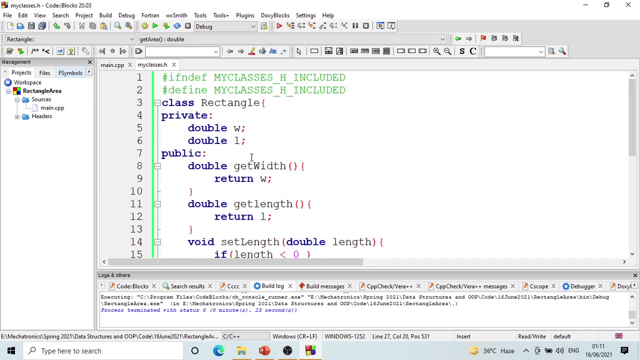 okay finally the problem was we wanted to find the area okay so how to do that double get area okay and here we would say return L multiplied by W okay here we can also provide the constructor function and sector function because the mountain Anna take it so constructor function is a special function which is used to initialize the values the data members of a class ticket so you class could be the members and by default they 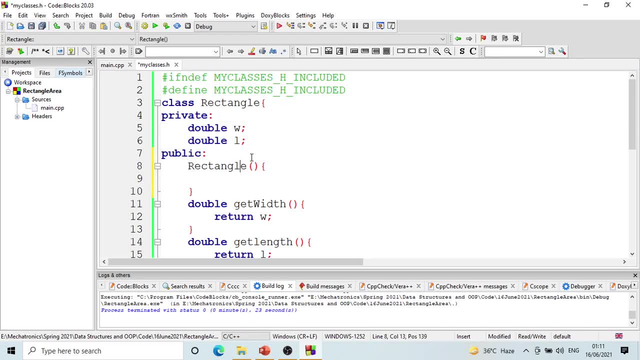 will have garbage values okay so if you want to initialize them these values to yeah pick the sector provider so this that is this is an overloaded constructor yeah premise to do value 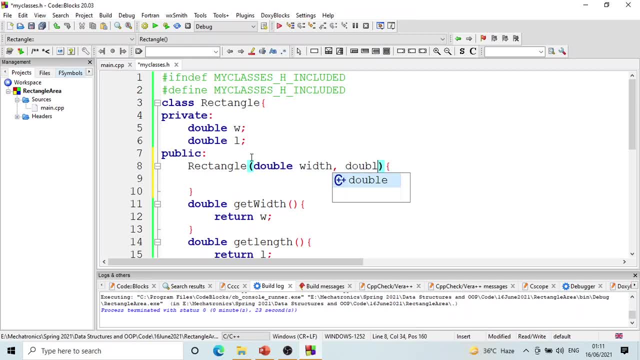 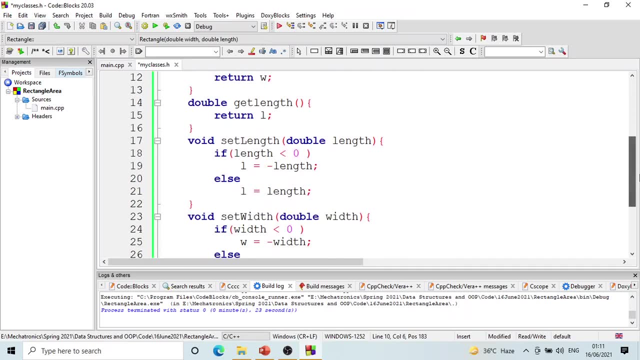 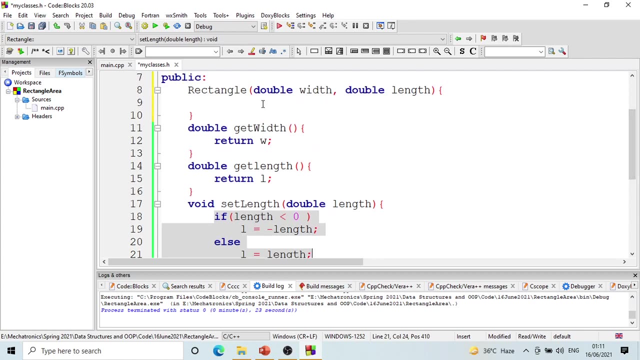 data and double weight and double length okay or yeah I think you don't know towards them copy paste card with them yeah in fact I'm here come to let a set wait here okay okay okay Professor for 40 benut eg the this is basically used to initialize 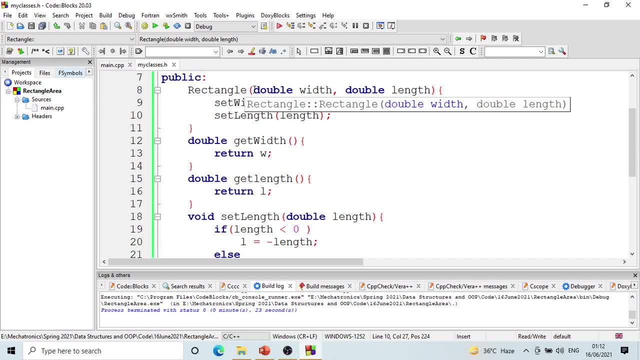 the length and width attributes of the rectangle at the time of creation oh yeah yeah validation 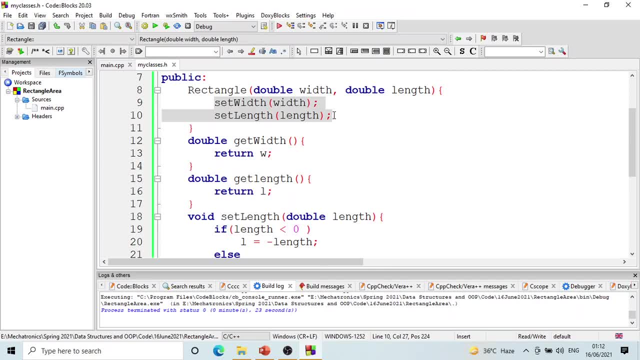 so we are reusing that code so you can call in functions so we have created our rectangle class 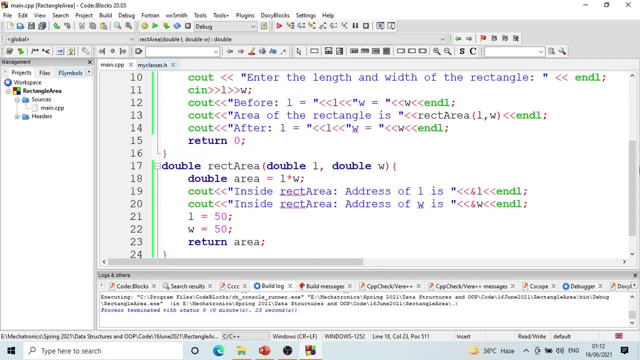 now how to use this so here we have to include this 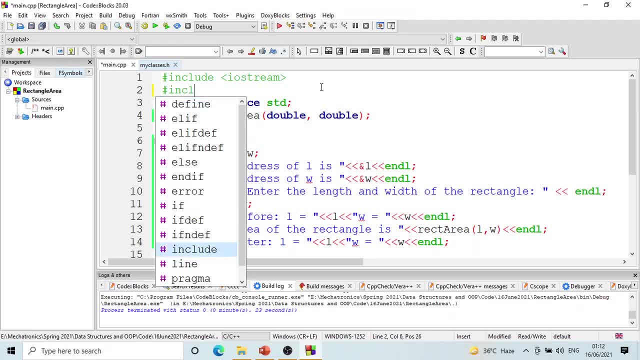 header file my classes ok 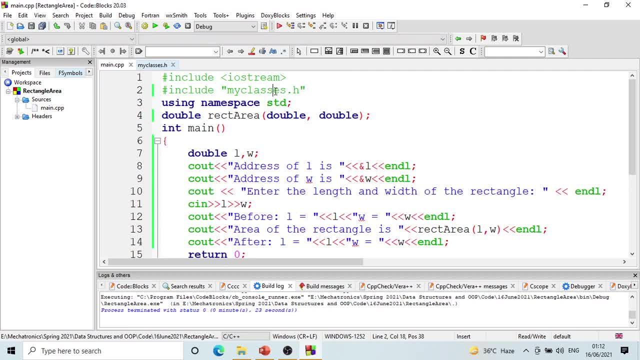 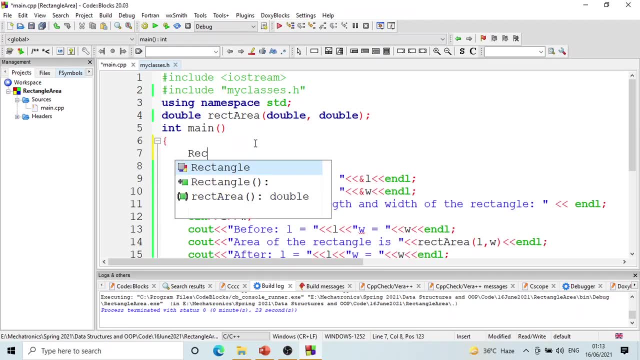 so we have included our header file and now we can create a rectangle object you can say rectangle r1 and you can give initial values say for example 10 or its length say for example 25 ok 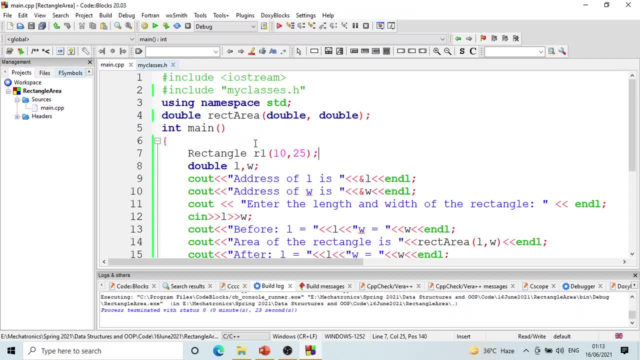 whose width is 10 cm or meters or whatever and whose length is 25 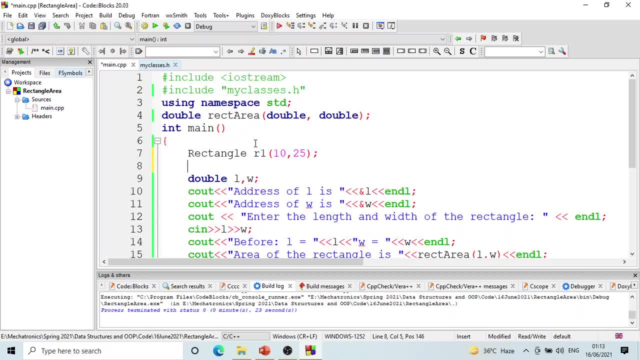 now we want to find out its area so we send a message to rectangle object r1 that please return our area ok 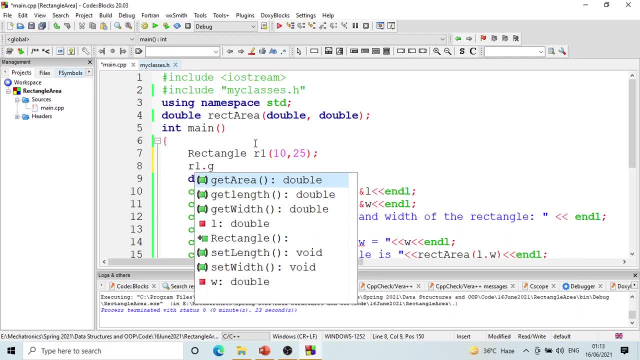 how do we send that message we say r1.getarea ok 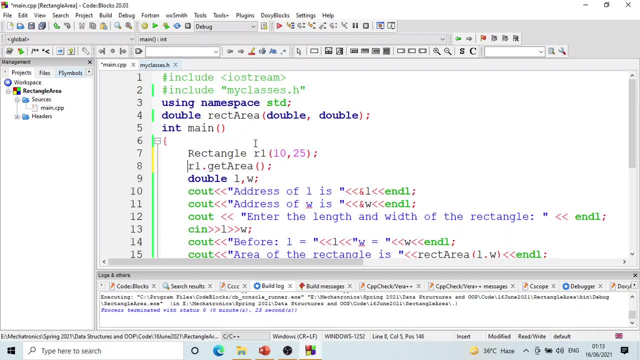 so that's it and we print this cout 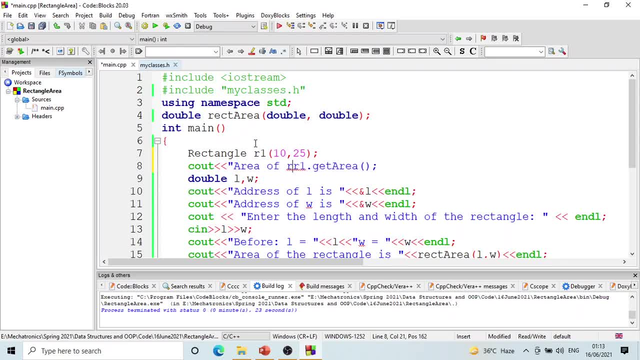 ok area of r1 rectangle r1 is 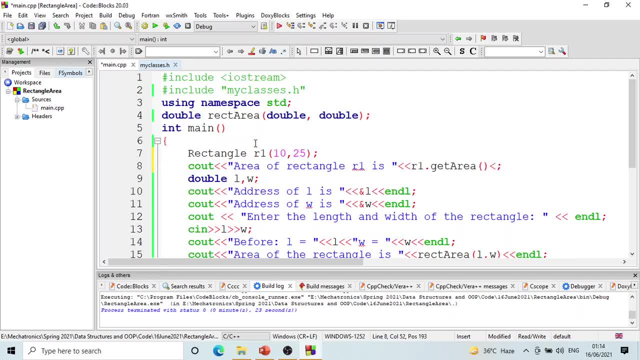 ok r1.getarea and then see now there is a difference of approach there is a difference between the two approaches here 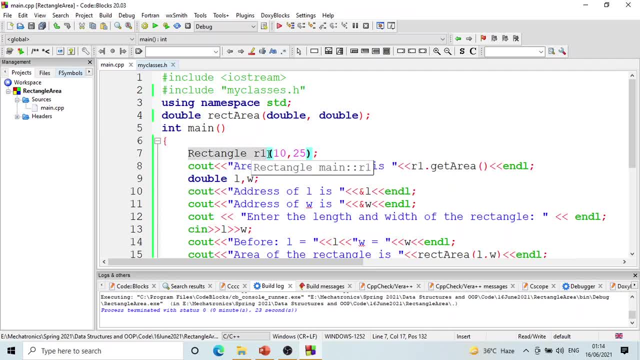 you have created a separate entity its activity is different from the previous one here you have created a separate entity you have defined its attributes you have provided the initial value of those attributes and then you call a member function of that entity which accesses those attributes 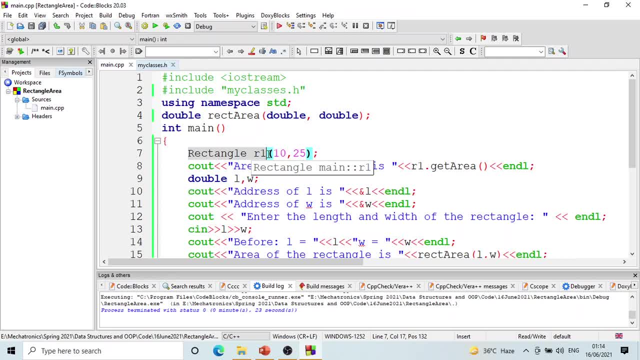 and gives you a value ok 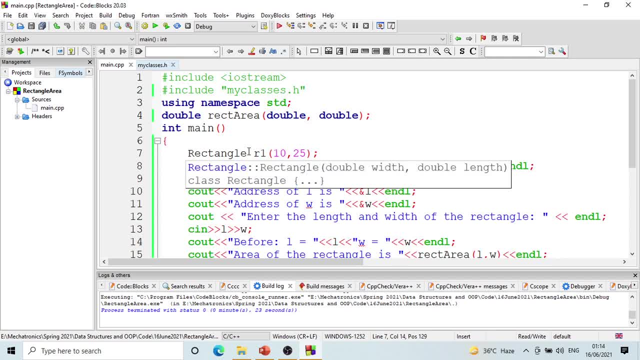 this is how we solve problems in the object oriented programming approach those functions or data 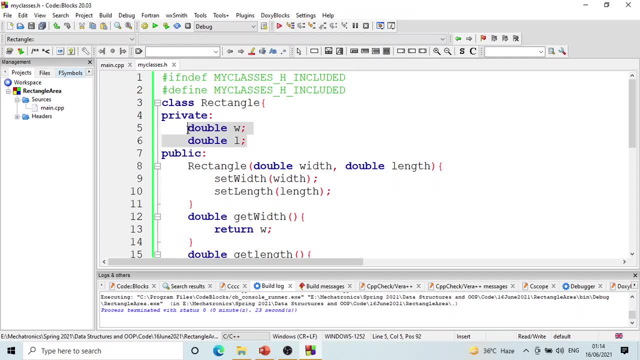 on which those functions have to operate we package the two together 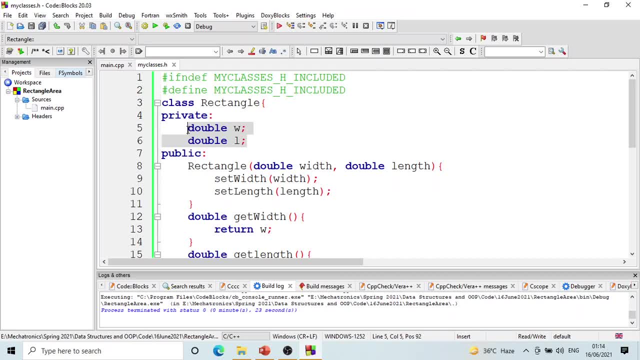 ok this is called encapsulation this is encapsulation this is the data or the attributes or the data members 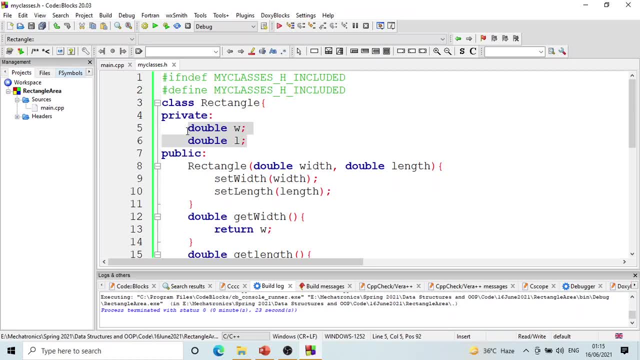 or the properties or the state of the rectangle object and these are the functions which can access this state 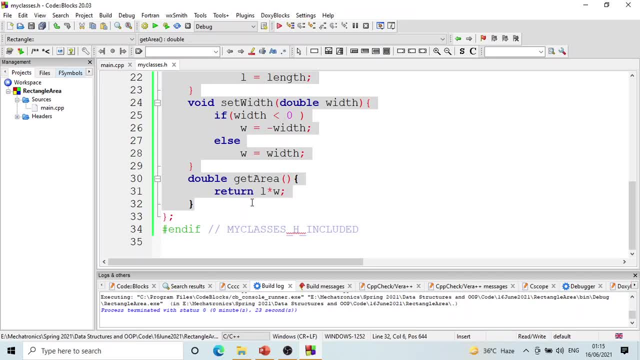 they are all together in one package in one class 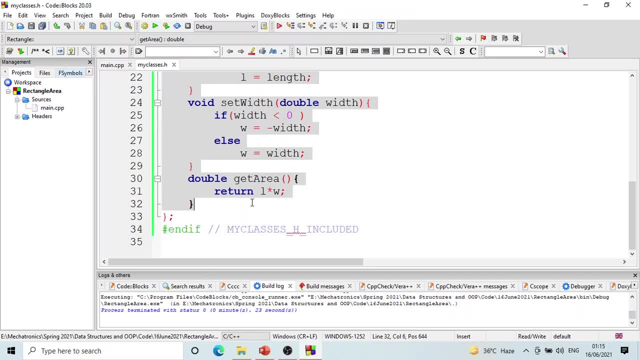 ok so this is what object oriented programming is all about 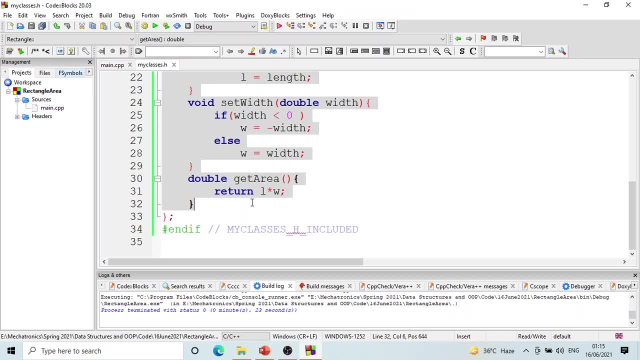 so whenever you need to solve a problem using the object oriented programming way you have to think in terms of objects creating objects or what will be the attributes of an object what will be the methods and in the main program 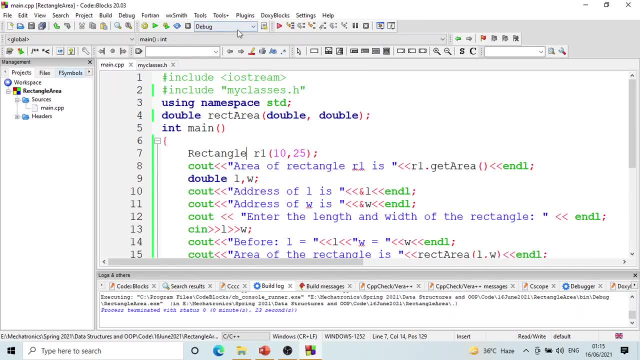 you will need to create objects of that class and then use those objects to solve that problem 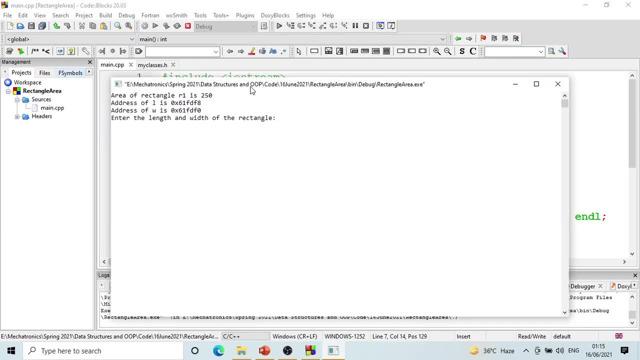 so area of rectangle R1 is 250 ok then that second program will run 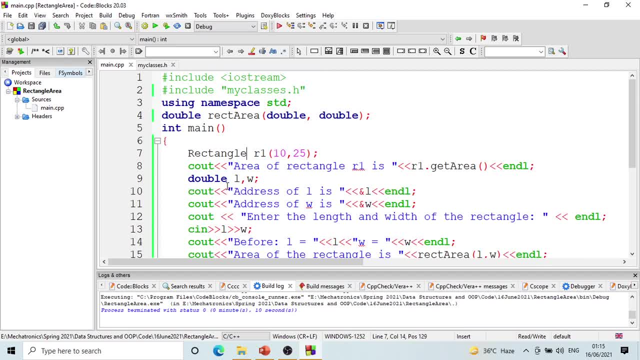 so did you feel any difference between the two methods one has more code than the other ok 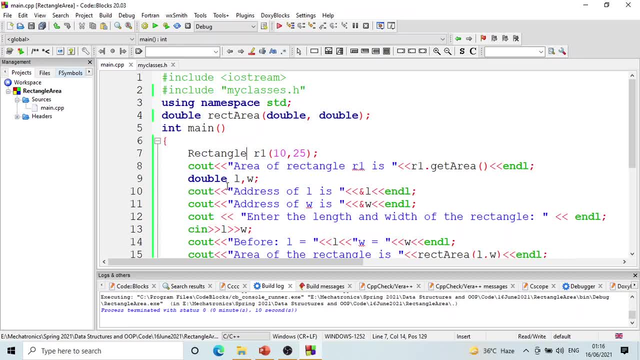 one difference is clear in object oriented programming you will need to write initially you will need to write a little bit more code 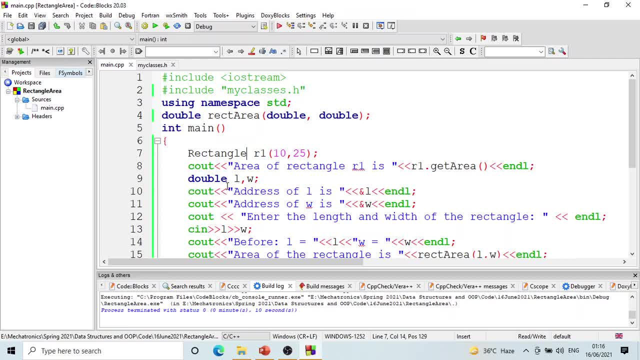 but once that is done they are easier to maintain to maintain them to debug them 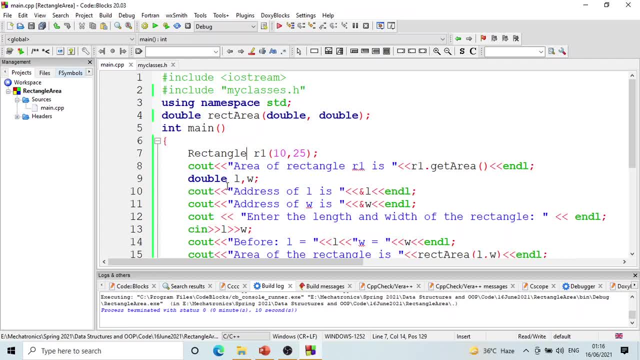 relatively it is easier from do not look at just these two very simple functions 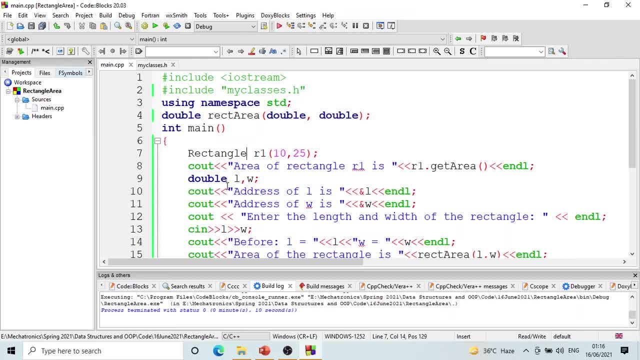 this is a very simple code but if the size of the project grows 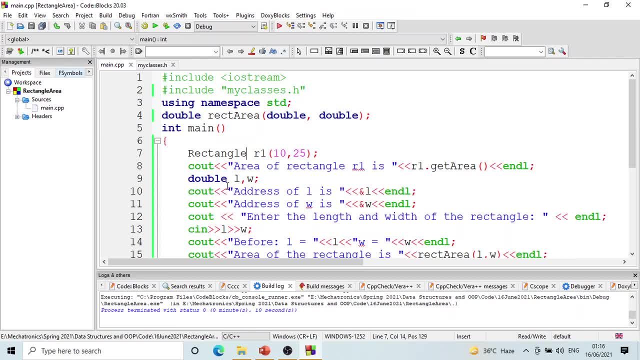 then you will like personally I haven't worked on such project I have never worked on such a big project 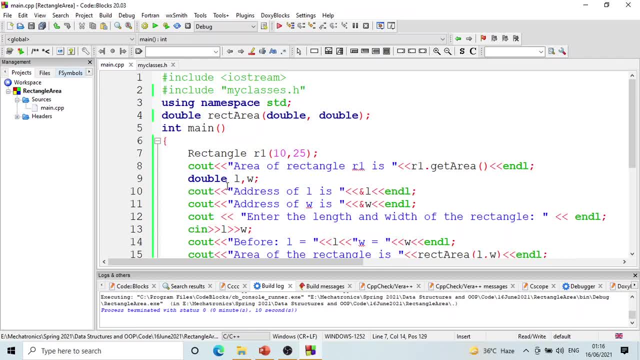 but if the project gets bigger then you can feel the pinch of procedural programming 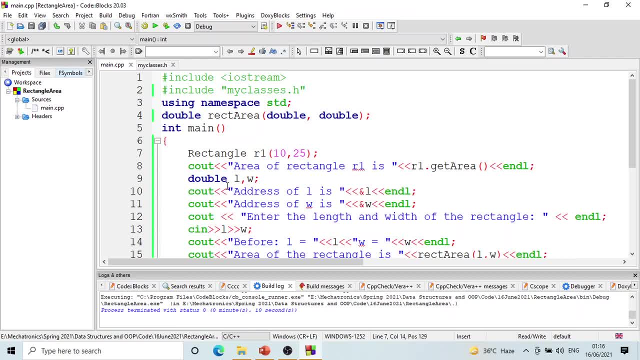 if you are not able to control it properly then there will be some problem this can be relatively easier for bigger projects ok 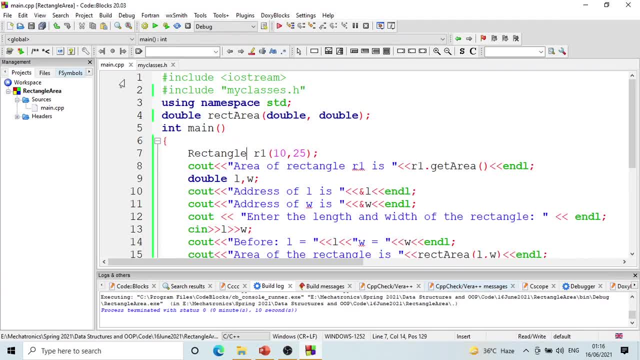 which one? this one I will upload it 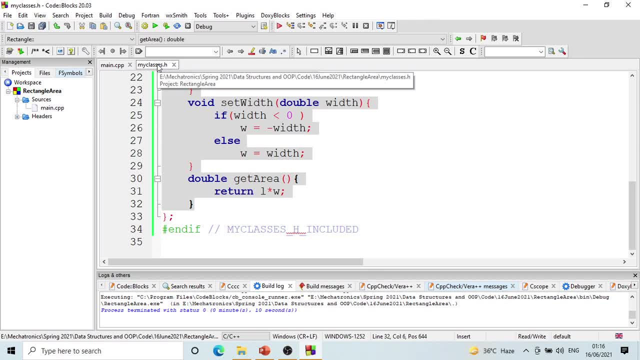 ok I will upload it ok I will upload it to Google Classroom ok ok ok 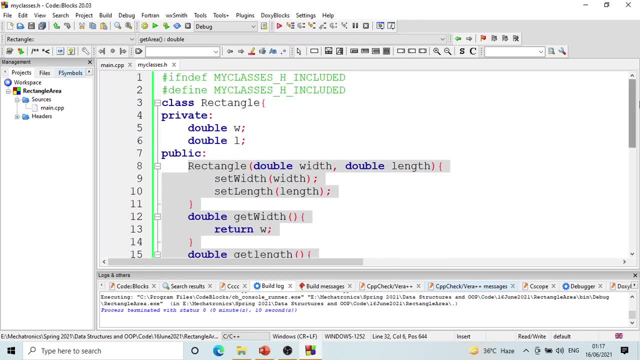 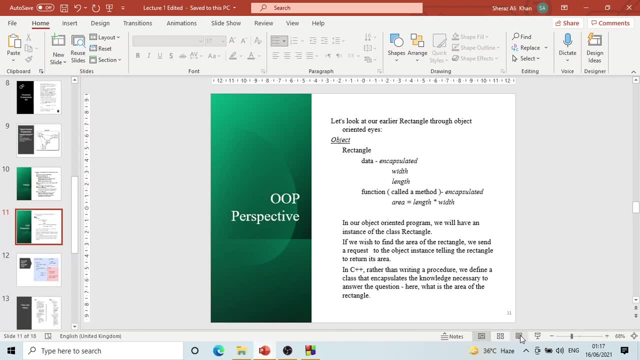 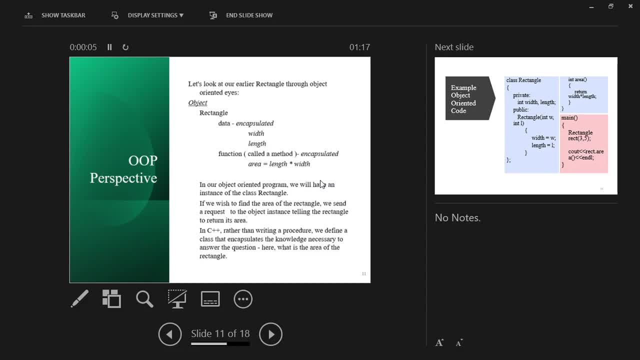 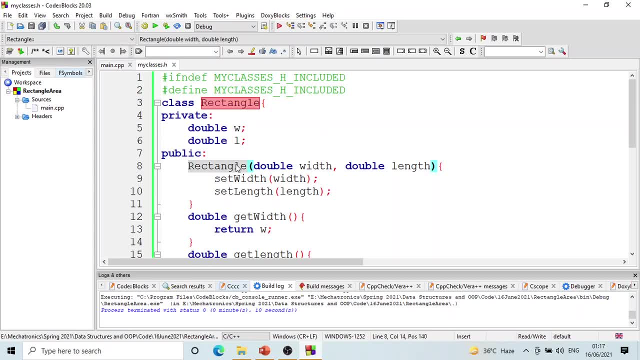 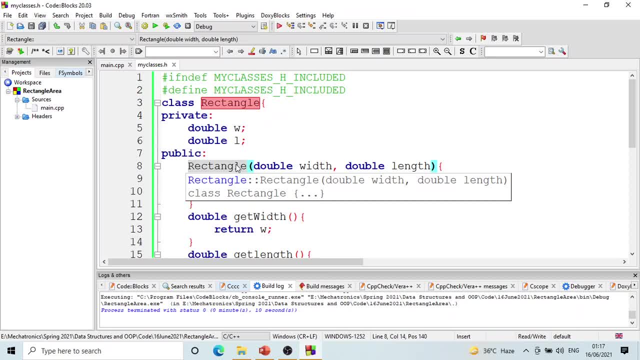 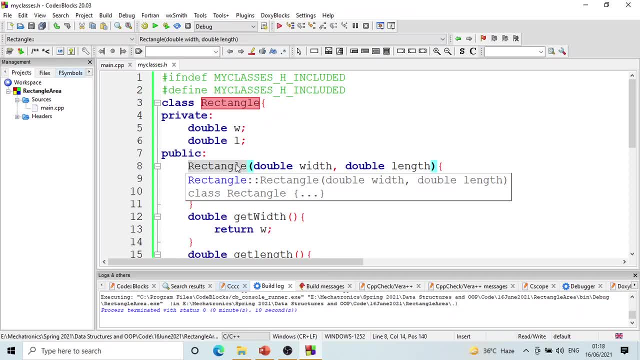 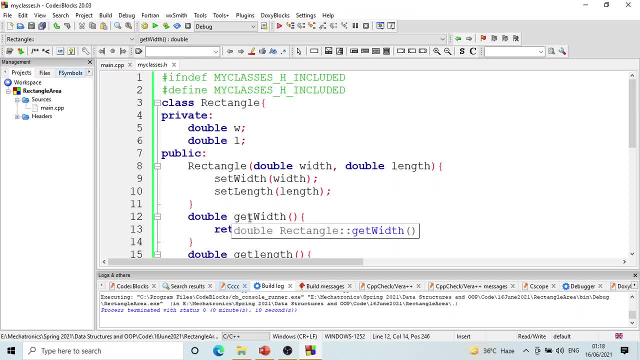 name will be one copy for all the objects of a class, whether it is one object or 1000 objects. But these data members have individual copies. Why do you write constructor function? 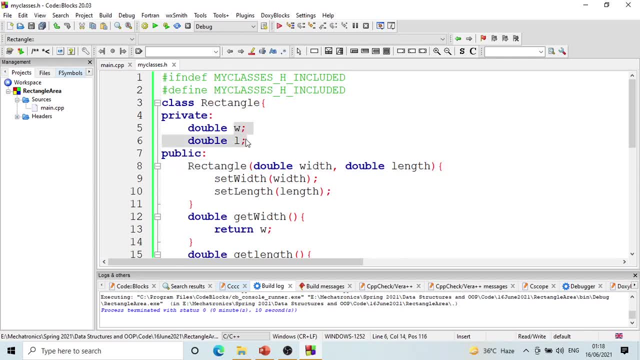 Because these data members by default they will have garbage values. So first of all you need to initialize them to proper value. Second, you might need to create classes in which you need to establish a connection to some database server or some web server or open some file before you can operate on that thing, on that whatever that problem is. So the requirement of every class can be different. This type of work which you have to do in the beginning, you have to open the file or make a connection with a file or a web server. For example, if you are using an app on your smartphone, so you usually connect every app that you use with some web server or database server. 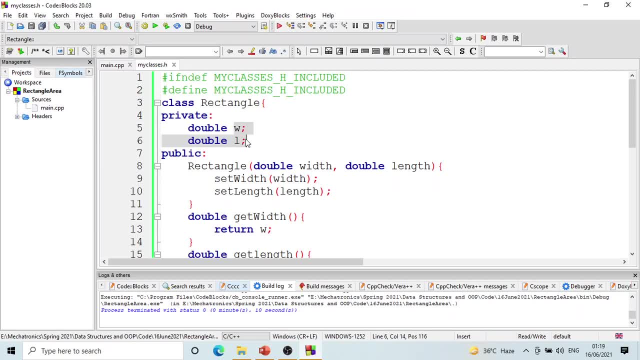 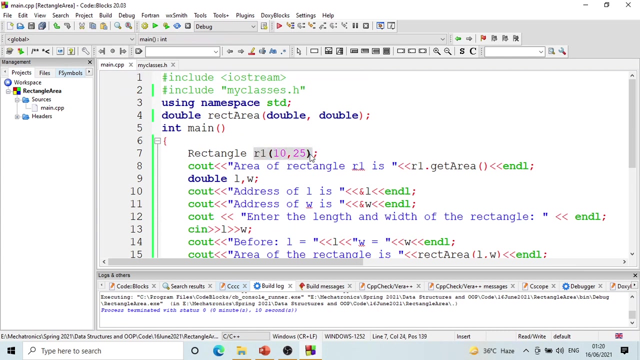 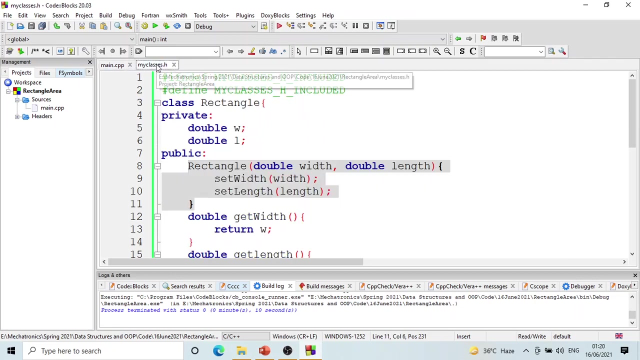 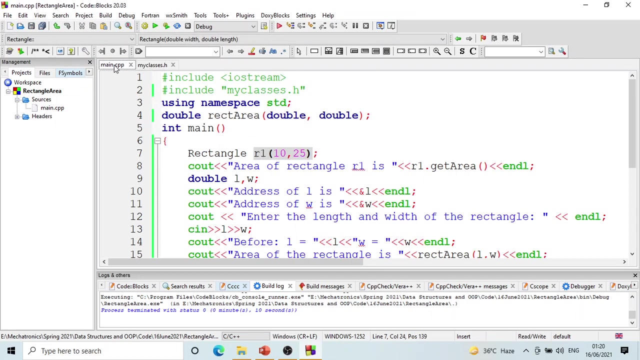 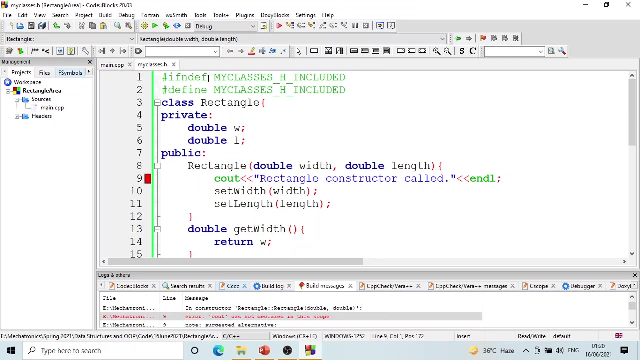 If you are using any app, for example, if you are using Jazz Cash app or Easy Paisa app, then it communicates with Telenor or Mobilink server. So when the app opens, then the work of establishing the connection should be done in the beginning. Then you should get the interface. The work of login should be done in the beginning. So after that, all the work which you need to get done with those things at the very beginning, you put all those things in the constructor function. So constructor function is the function that is called whenever an object is initiated. When you do this declaration, Rectangle R1 1025, the constructor function is automatically executed. If I write a line here, constructor function called, then you will see this line printed first. Before the calculation of area, you will see this output. Okay?ło We need to have bio stream. Okay.ło 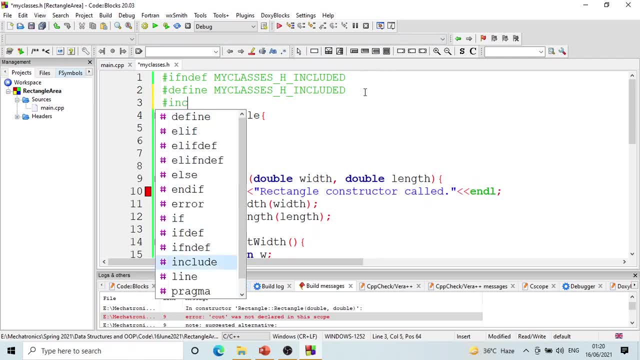 वीरप्यो प्यास प्यास दिये दियो that there's going to be a delays. चरई जोटे ज़ोटे दोधै जाड़ में शुभ दिखाई and we need to use namespace 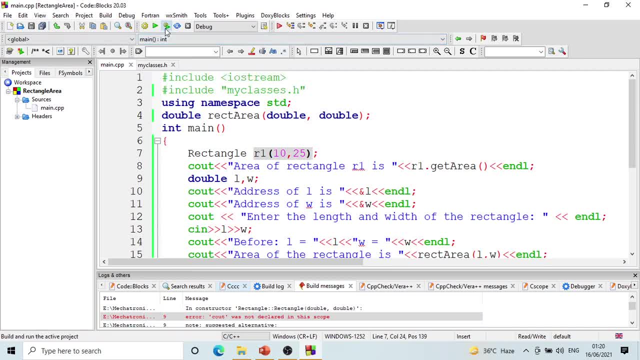 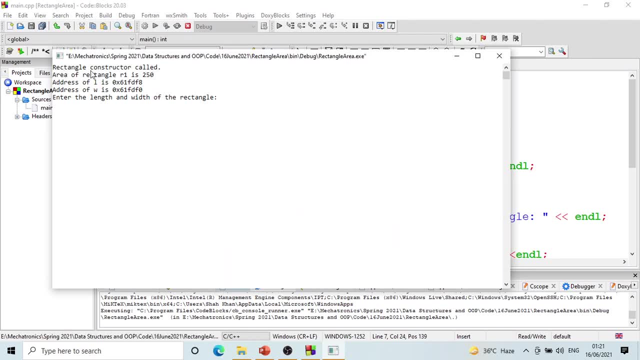 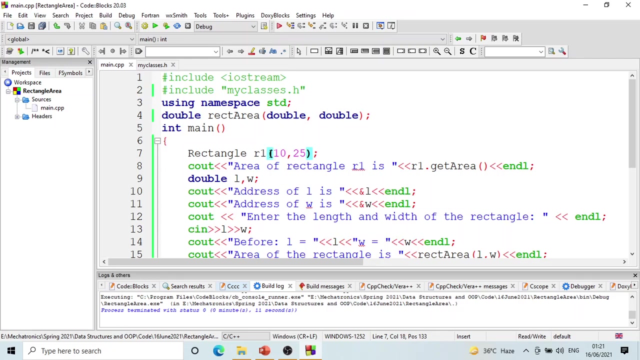 ok ok now when you will see this the first line that is printed is called rectangle constructor the first function that will execute will be the constructor of rectangle class here you are declaring the object of rectangle class and here you are implicitly telling that the constructor is overloaded which is expecting two values, execute that so that the state of the rectangle object is initialized its attributes have initial values why do we write constructor function? in order to initialize the attributes of an object 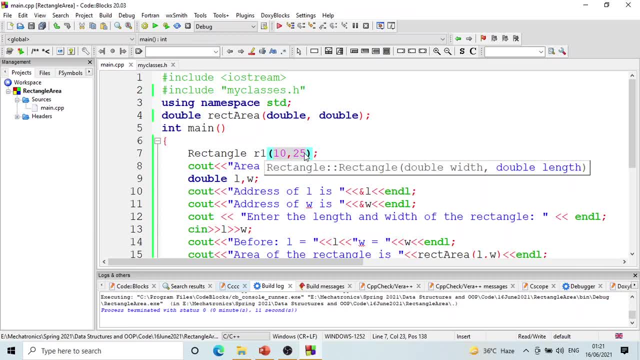 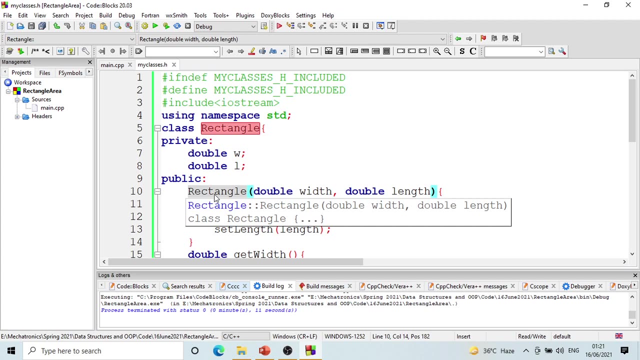 at the time of creation of the object we write constructor function how do we write it? the name of constructor function and the name of class will be the same and then you can give an argument in parenthesis and then the rest will be like a normal function opening curly base and closing curly base so you should know what is the purpose of constructor and how to create one 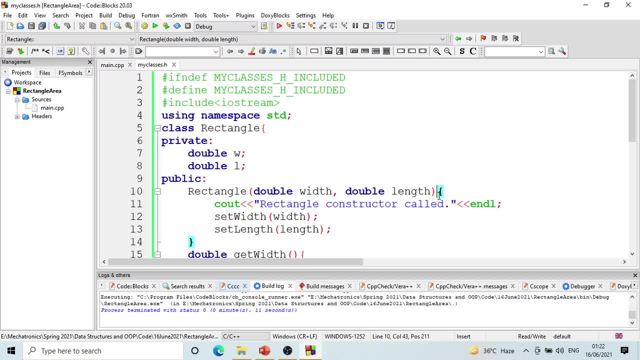 the purpose is that we need to initialize the attributes of an object whenever an object is created the way you create this constructor is this is how you create it 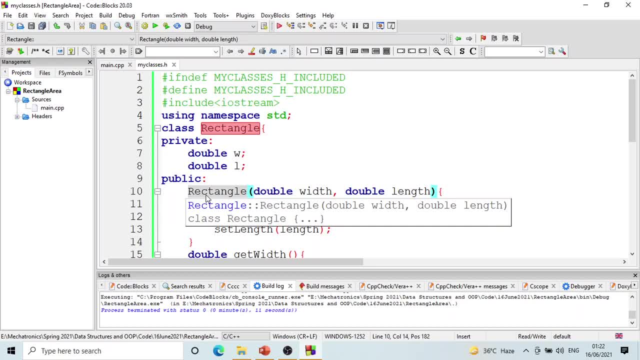 get function set get function set it is necessary that these functions are there if you want to read then it is necessary 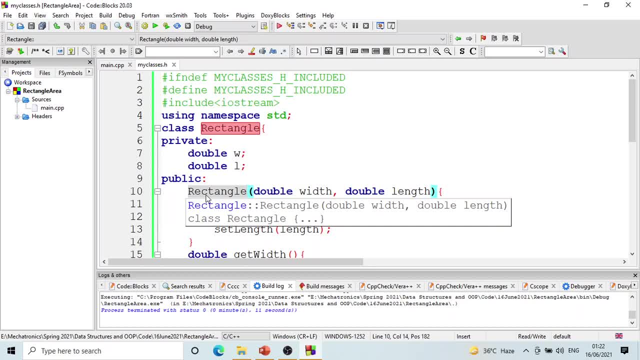 that what is the width of this constructor what is the length if you want to change the length and width 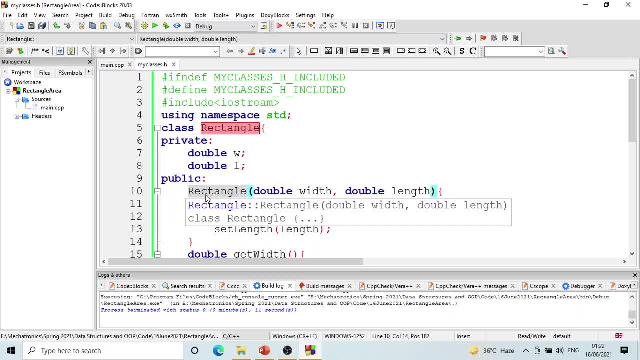 then you will also want to have that what is the minimum condition? the minimum condition is that the length it should be 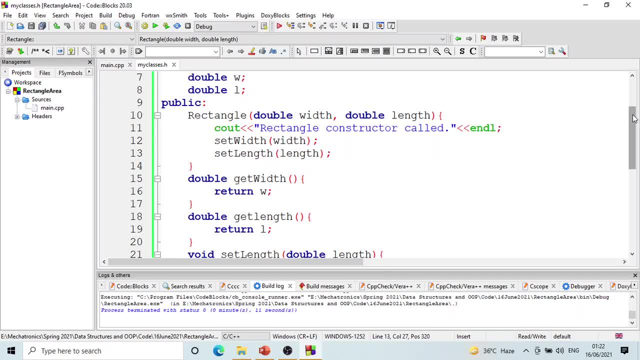 positive value it depends on the application in some applications it cannot be just any positive value for example the length of the table can't be 2000 meters 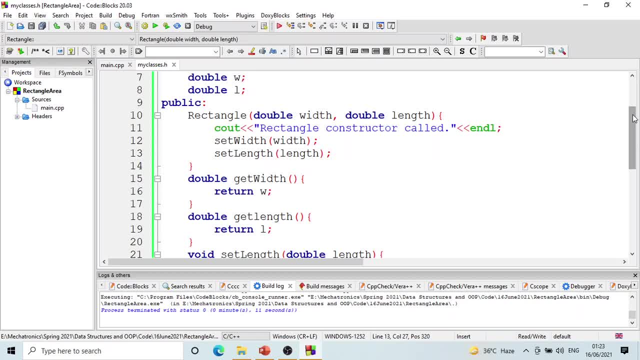 or 3000 meters it should be reasonable so that depends upon your application area or if you have a room and you want to place an object in the room then the length and width of that object it should not exceed the length and width of the room so restrictions will come from the application and then you might need to modify your code the advantage of this is that instead of modifying the whole code you only modify the rectangle class whereas in procedural programming you need to modify the whole code 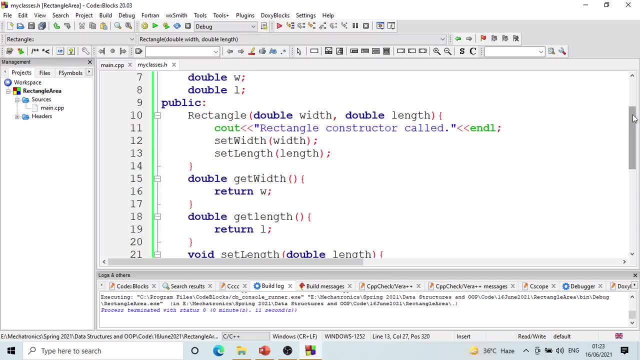 you need to modify the locations from where you are sending the values or whatever is happening ok 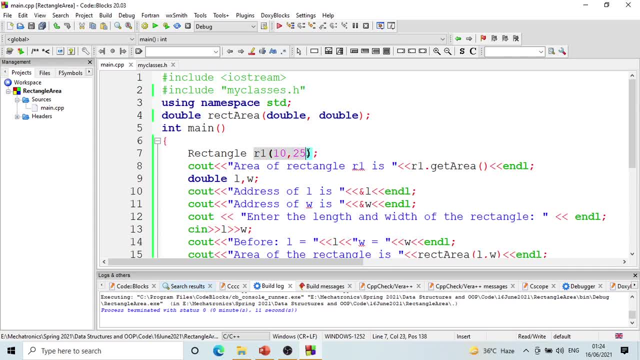 right now we have one constructor function we have only one constructor function which is this one 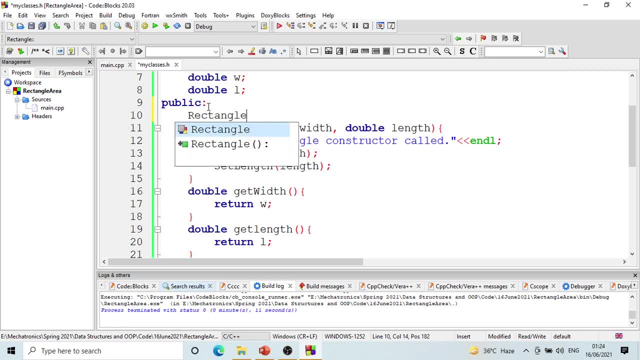 say for example we can have this default constructor as well default constructor does not get any arguments 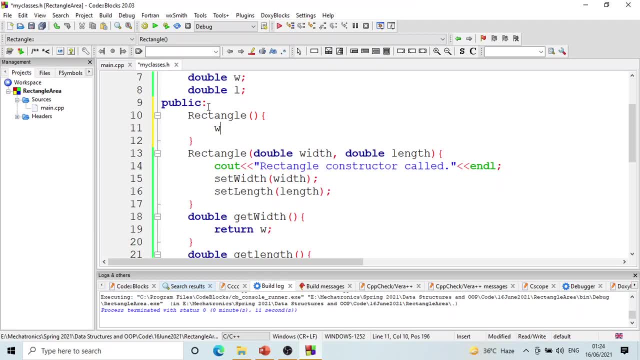 so you understand that then you create a unit square in fact length is also one and width is also one 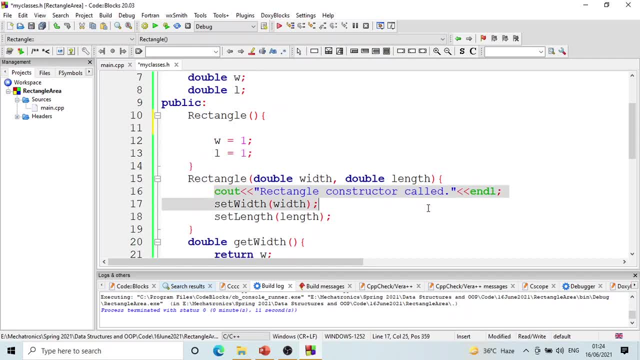 ok we will write a message here this is a default constructor 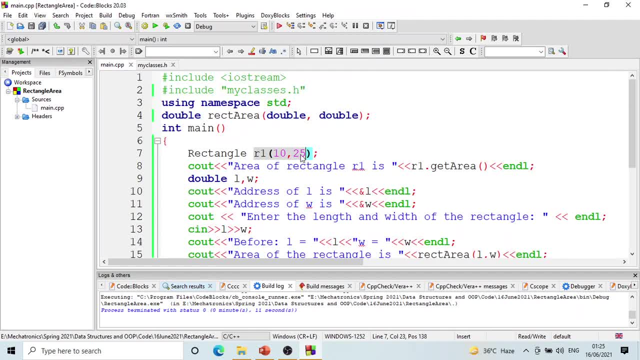 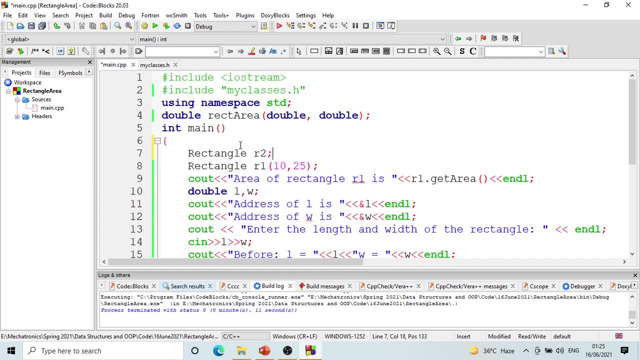 ok please don't talk white white see if I create this object rectangle r2 r2 and here I do not provide any arguments ok 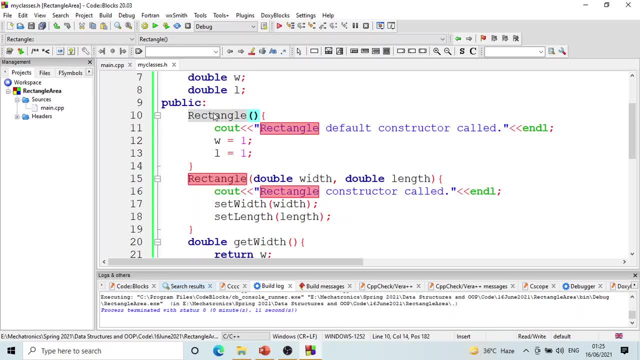 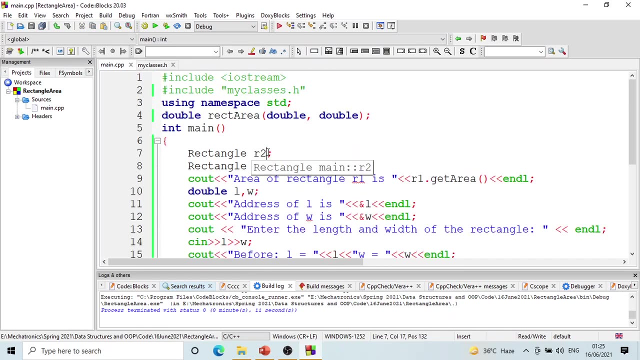 that means that I am invoking this constructor the default constructor which does not get any input arguments then this constructor will be called ok so you are implicitly determining which constructor is going to be executed implicitly just by providing arguments here or not you are determining which one will be executed ok so you can see that what will happen in this case 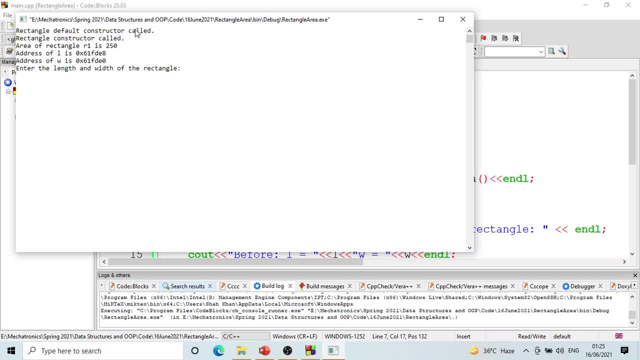 so rectangle default constructor called first that statement will be executed then this other constructor of rectangle 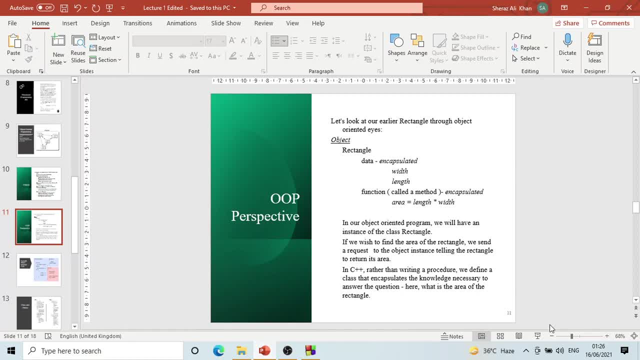 understood ok pardon me please let's go through these slides 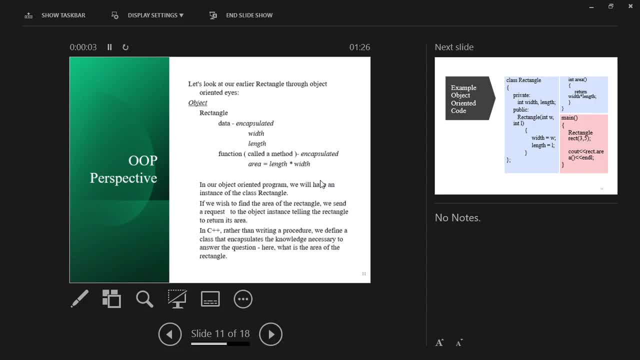 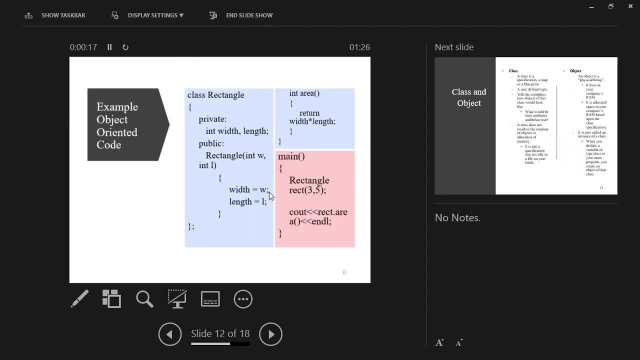 most of the thing that is in these slides we have already talked about it and demonstrated it ok so we have solved this problem using the object oriented programming way we have talked about encapsulation or constructor and all these things this is not the complete code but 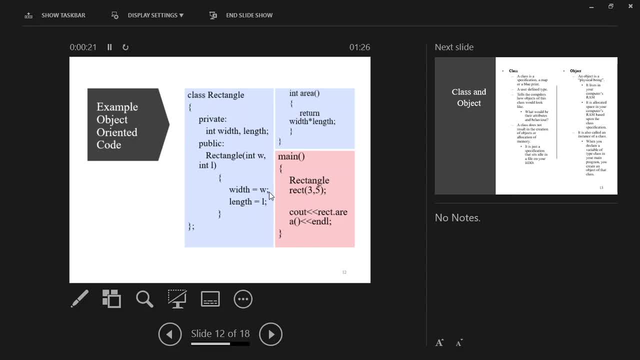 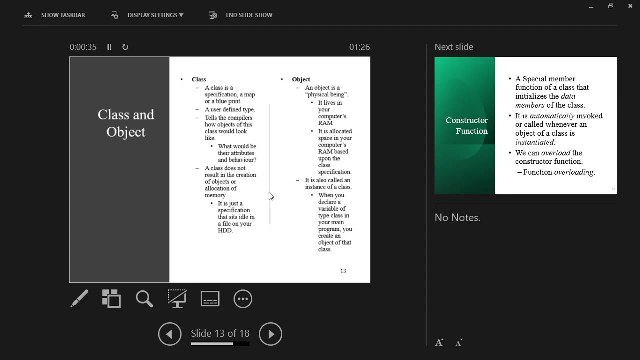 part of the code ok which you solve through object oriented method this is a little different but it is nevertheless you get that idea ok while talking about the while talking about this example we talked about a class and an object ok we talked about that that class and object these are two different things you don't have to confuse this ok so a class is basically a specification or a map or a blueprint 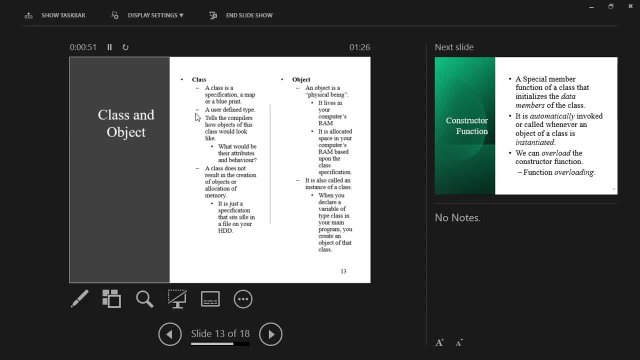 it determines that what will be the attributes of the objects of this class and what will be their behavior ok when you create actual variables on the basis of that class create actual object then it gets allocated in ram we call that particular thing as an object it becomes the object of that class so you should go through it a class is a specification a map or this it is also a user defined type we use classes to define 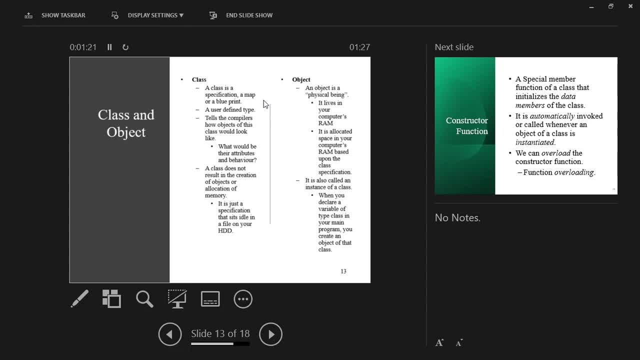 new data types my complex is done fraction is done rectangle is done so we can have other data types as well so these are new types that we can create using classes ok what does a class do a class tells the compiler it is basically a specification that how objects of this class would be created how will the objects of this class be created what will be their attributes what will be their behavior that is what it does 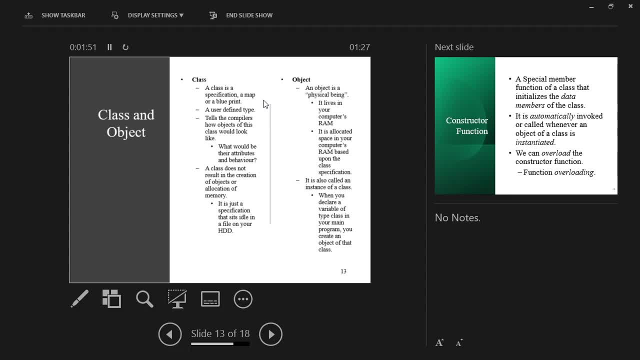 a class does not result in the creation of objects or allocation of memory when you write a class no objects are created no memories are located ok that is a simple definition 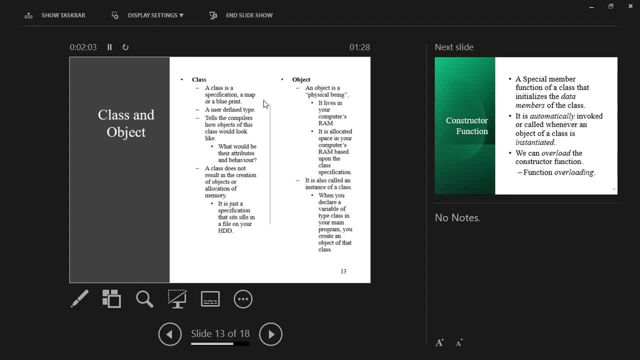 like if you make a map then automatically it doesn't become a house ok so if you make a map then you have to make a house so similarly when you define a class 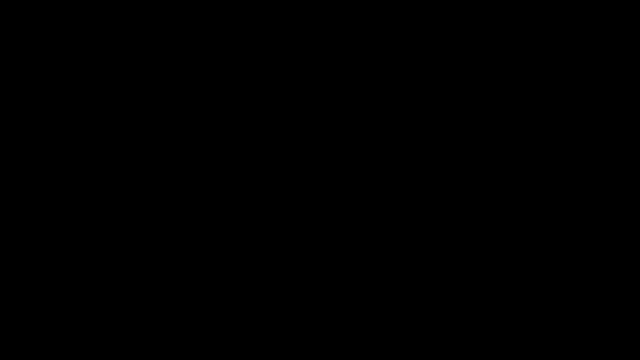 you have to instantiate objects of that class how do they do it this is how you do it in the main program this is how 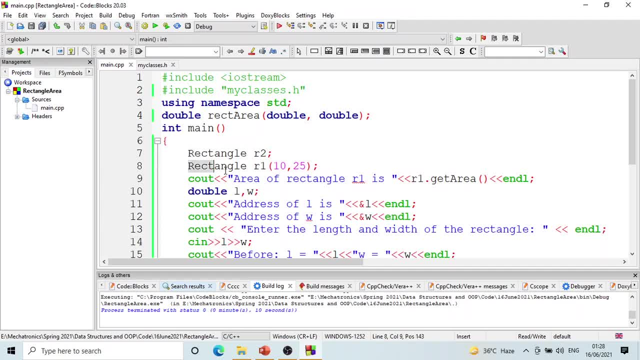 we instantiate objects of a class ok this is how we instantiate objects of a class 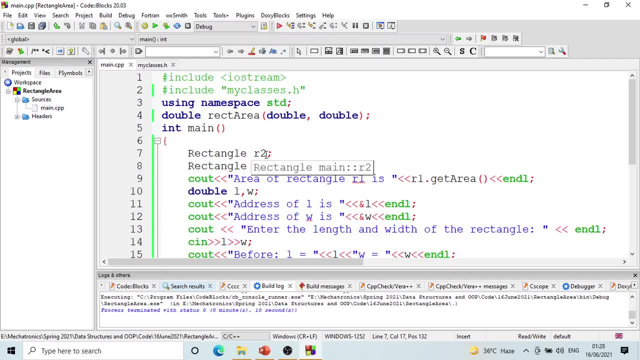 now we are creating objects R1 and R2 these are physical objects 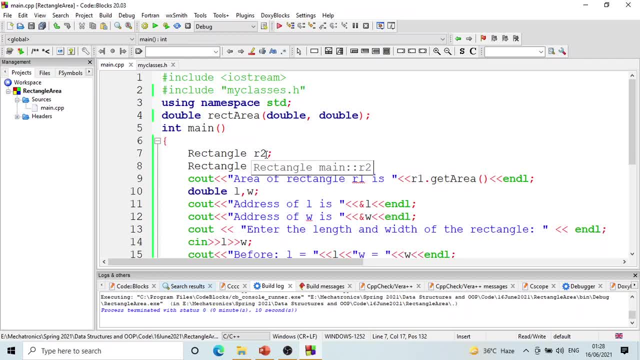 that reside in the random access memory of this laptop this definition it is 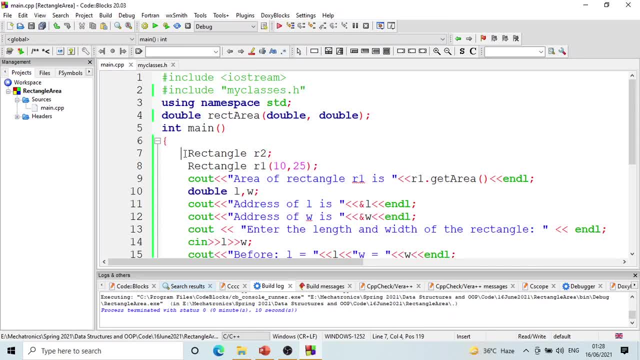 it doesn't do anything if we don't do this 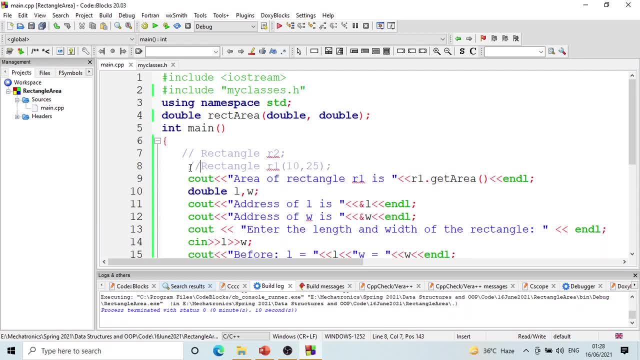 I will comment out these two things so 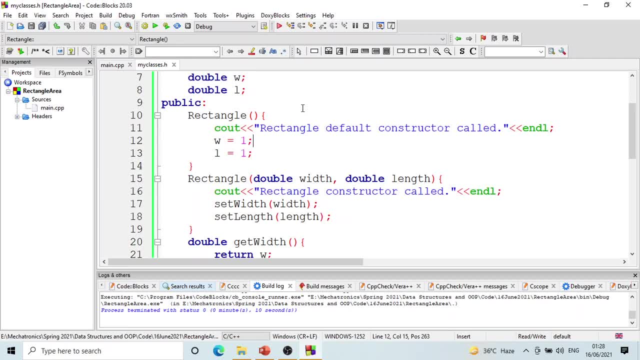 then this definition compiler will not use it for any purpose 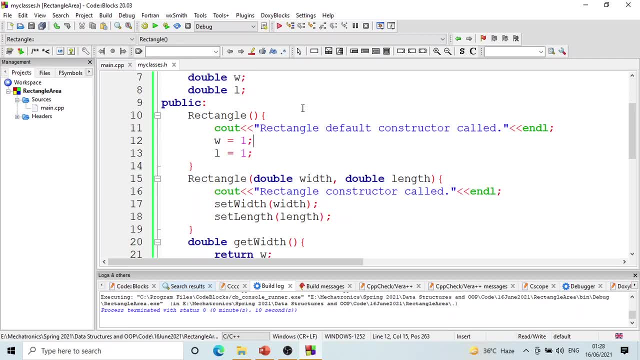 it is available but it is not being used to create anything physically 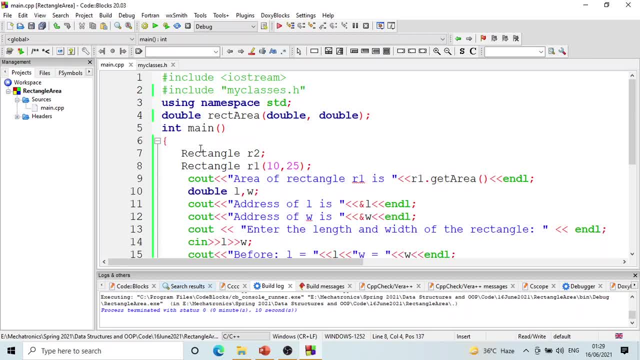 now we will talk about R2 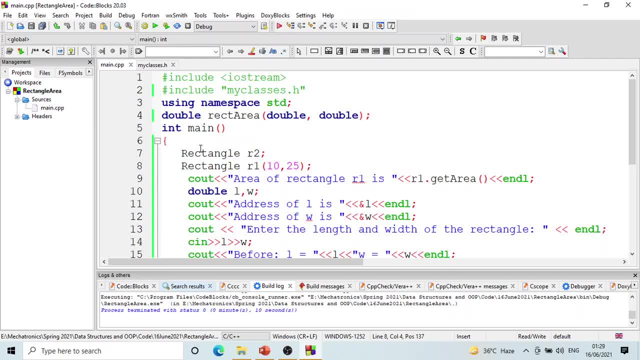 R2 and R1 R2 is not related to R function R2 and R1 R2 and R1 how do they take values 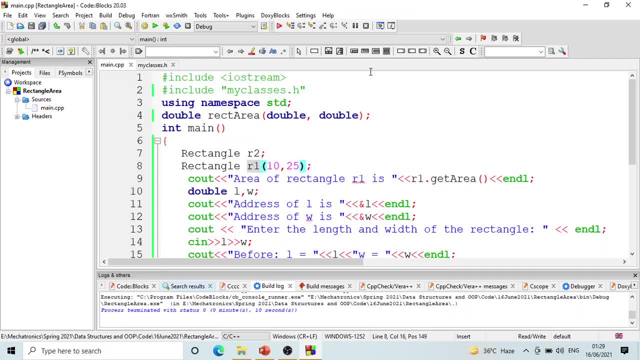 R1 is an object what what why why please 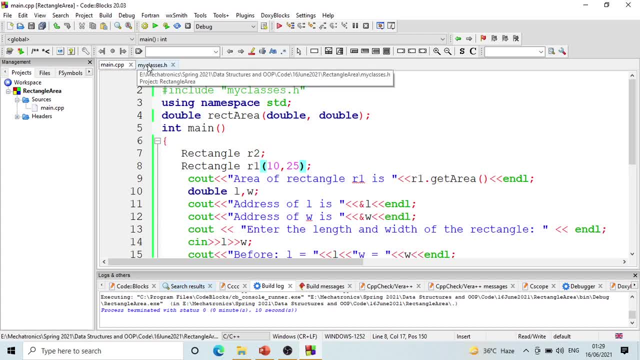 R1 R1 is a is a separate function R1 is an object 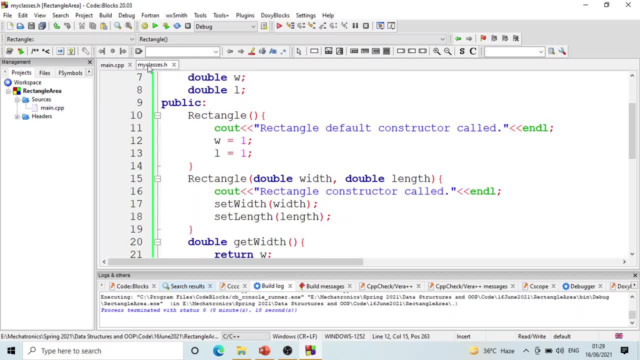 R is an object of type rectangle and these two attributes of rectangle class are width and length How these two are linked to rectangle object? 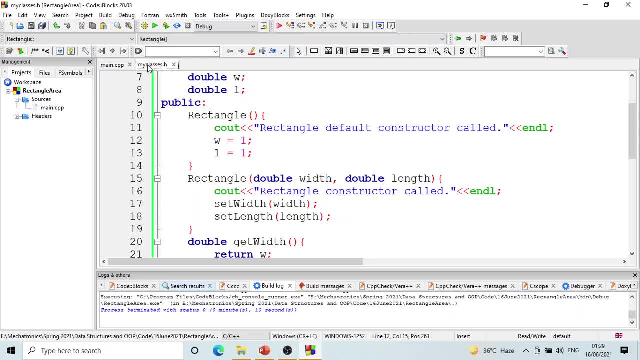 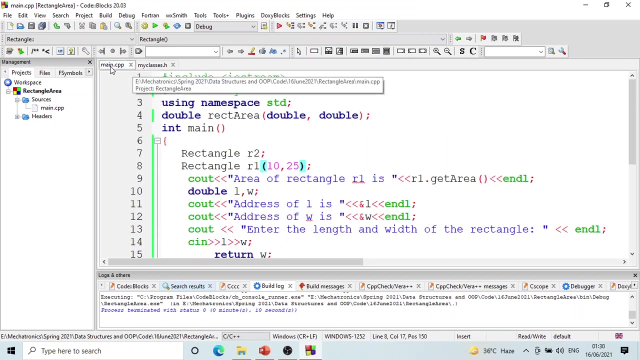 R is created on the basis of the rectangle class Your compiler reads the rectangle class and creates R1 and R2 object Basically it sees which attributes are there One is W and the other is L It reserves space for both the attributes in the RAM This work is done by your compiler This work of linking R1 and rectangle class is done by your compiler 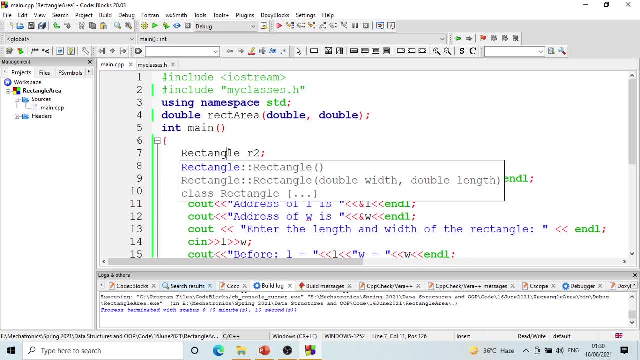 When you say rectangle R2 You are telling your compiler that R2 is an object of rectangle class So it sees rectangle class It goes to myclasses.h header file And there it sees rectangle class Rectangle class has two attributes width and length So it reserves space for them And then it has member functions It loads those member functions into the random access memory Then when you say in your main program R2.getArea So it calls getArea function And these two attributes of R2 These two attributes W and length It passes them How does it pass them? 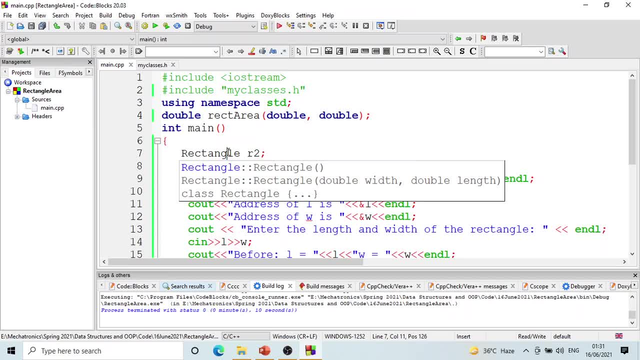 We will learn about it in a future lab session But this linkage 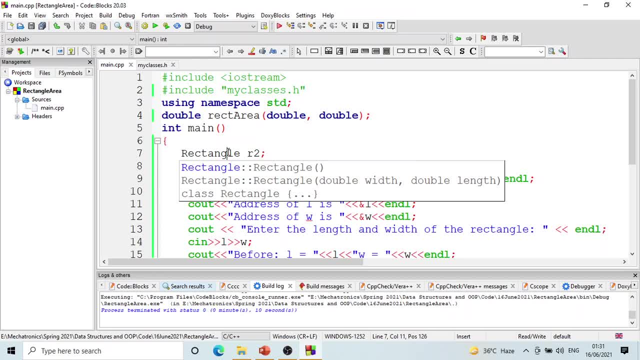 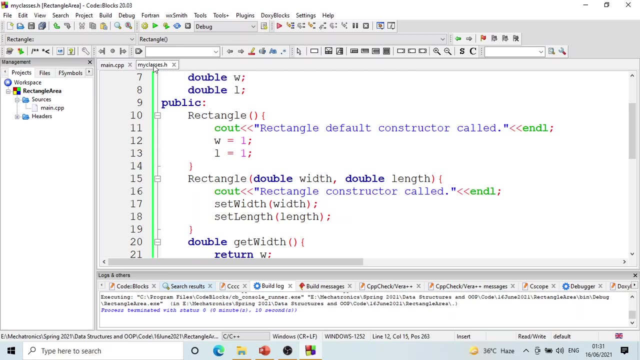 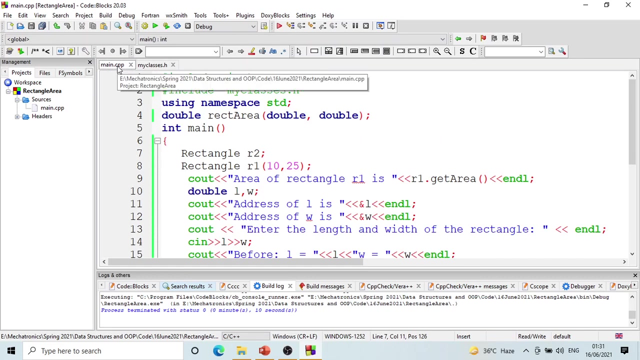 This is already initialized R2 is an object of rectangle class And the attributes of R2 W and L By default they are assigned values of 1 and 1 Because when we declared R2 We did not give any initial values to it We gave initial values to R1 Of 10 and 25 So the attributes of R2 Are initialized from 10 and 25 By calling the appropriate constructor One second The material of this slide 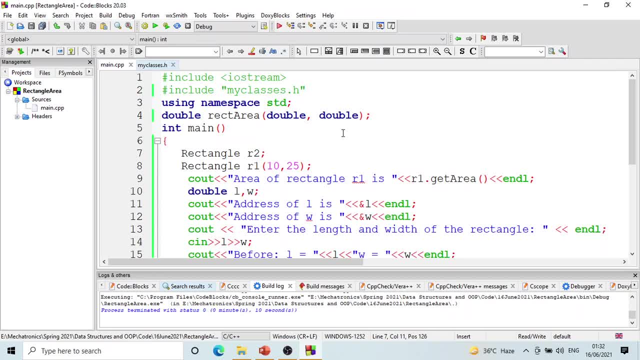 We have talked about it But I just want to go through it once Ok And then we are done Ok So we can do it quickly And then if you have any questions You can ask And those who want to leave They can leave Ok So let me do that quickly First let us see these slides So that those who are in a hurry 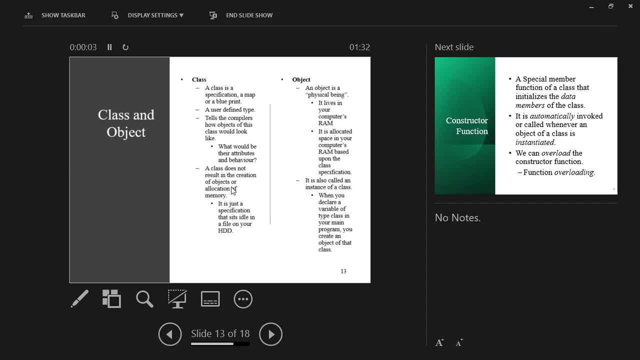 Ok So a class does not result in creation of objects Or allocation of memory Ok It is just a specification That sits on your drive An object is A physical being That means It resides in the random access memory It is allocated space Ok 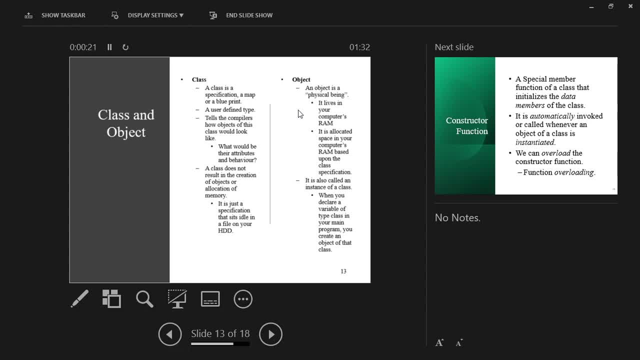 Based upon The class specification In that If it is told that It has 4 double data members 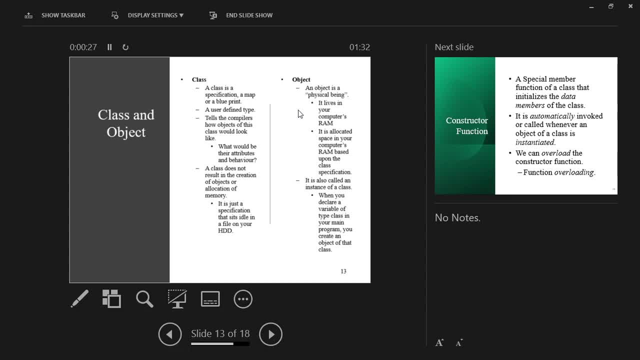 So it will be allocated 16 bytes space If there are 2 double data members Sorry For 4 37 data bytes memory will be allocated 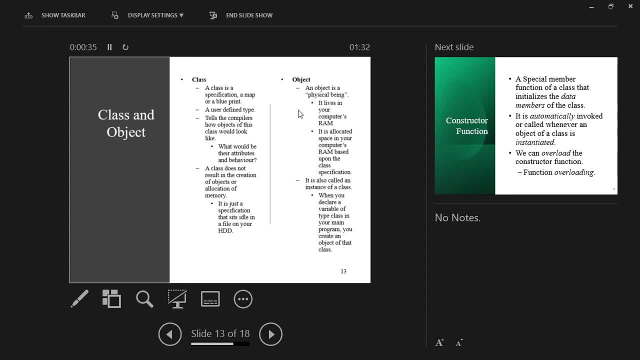 If there are 2 double data members So 16 bytes memory will be assigned Ok An object is also called An instance of a class 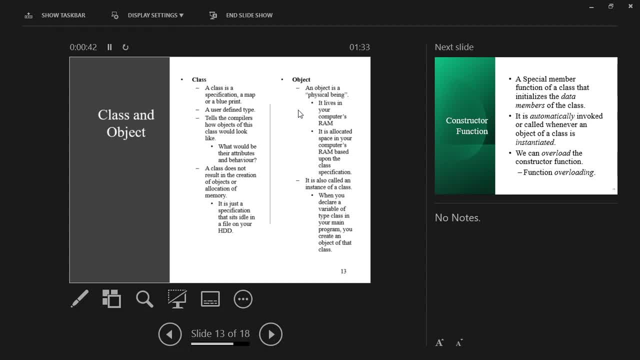 Now this is a term The objects which we declared R1 and R2 They are called Objects of The rectangle class Or instances of Rectangle class 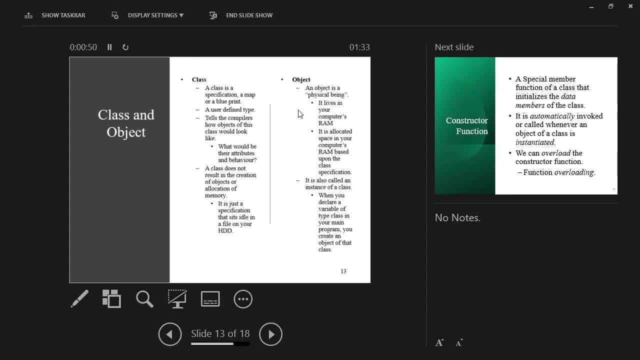 Ok Similarly In this context We also talked about The constructor function Ok So the same thing 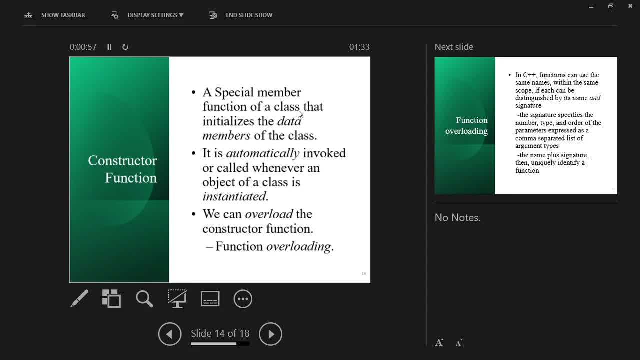 That we said That constructor is A special member function Of a class And its purpose is To initiate The data members Of the class Or attributes Of the class Ok 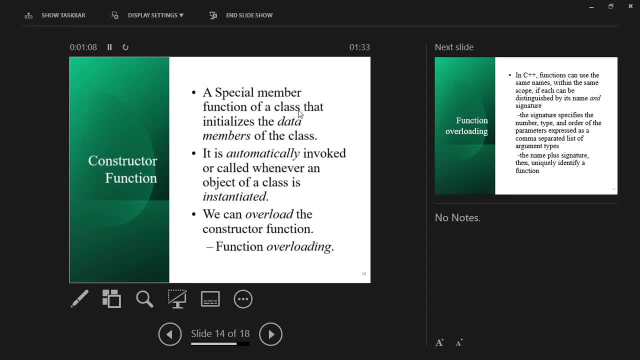 By initializing them Ok This is Invoked automatically When you create an object 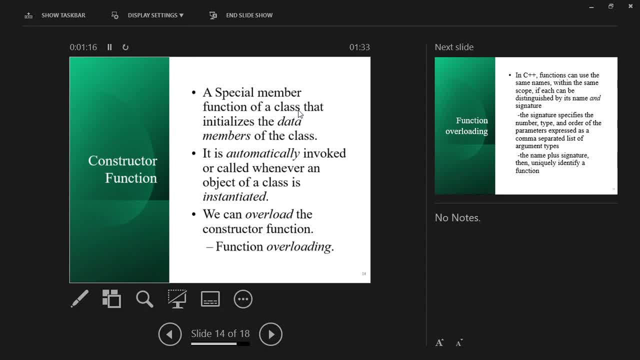 Whenever you say Rectangle R2 And we did not provide Any arguments Then the default constructor Was invoked When we said Rectangle R1 And gave it 2 values Then the overloaded constructor 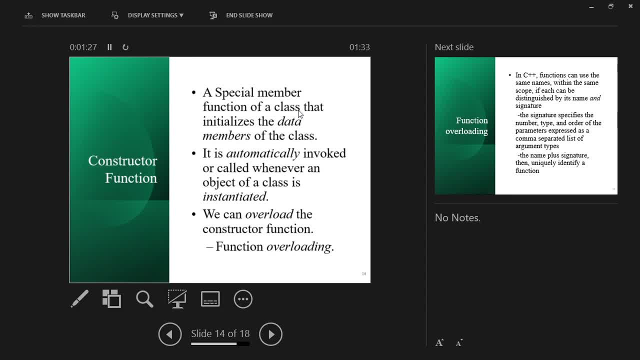 Was automatically called You did not call That function explicitly So whenever you 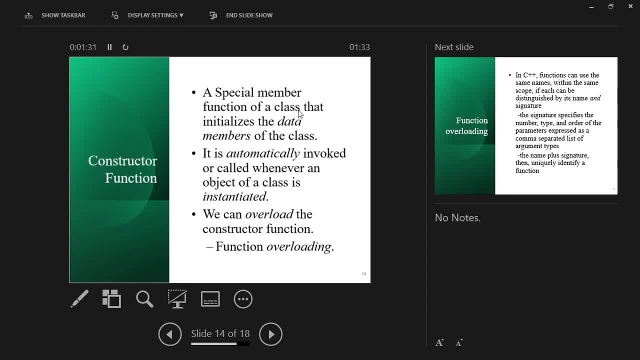 Influentialize an object The constructor function Appropriate constructor function 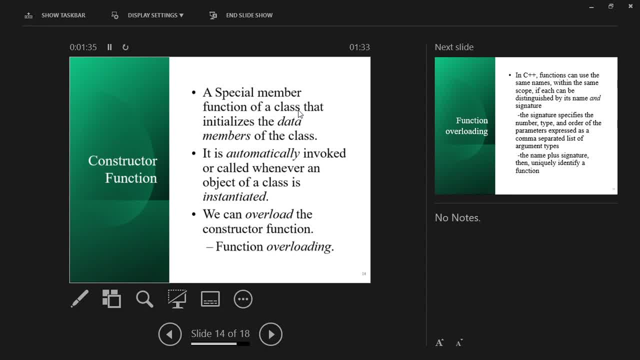 Would be invoked And And Constructor functions Can be Overloaded Ok 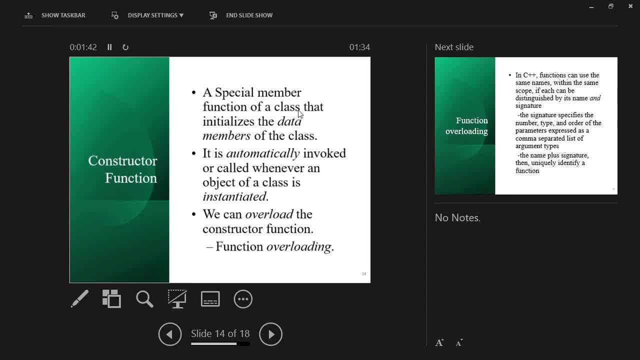 So function overloaded Overloading I hope you know The different functions Of the same name 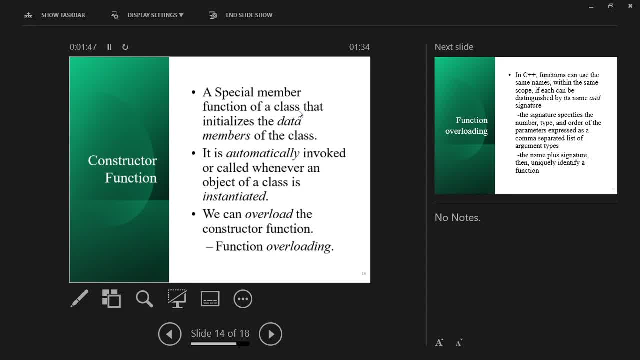 What is the difference That Their number And type of arguments Are different Ok 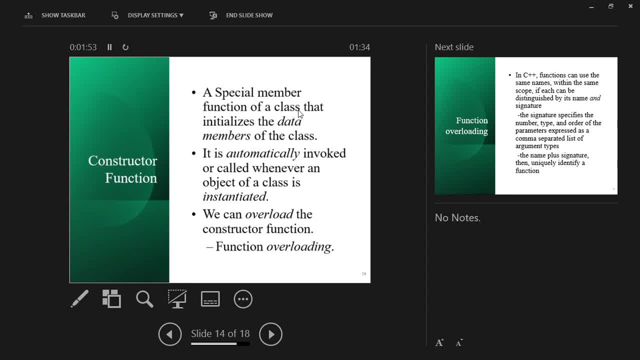 So here We have created Two constructor functions The names of both Were the same Constructor functions Of the same rectangle class One Was not taking Any input argument The other Was taking Two arguments So this is Function overloading 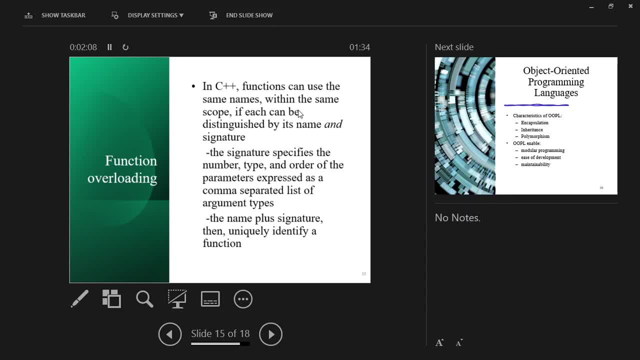 This is what is written Here Function overloading What is function overloading 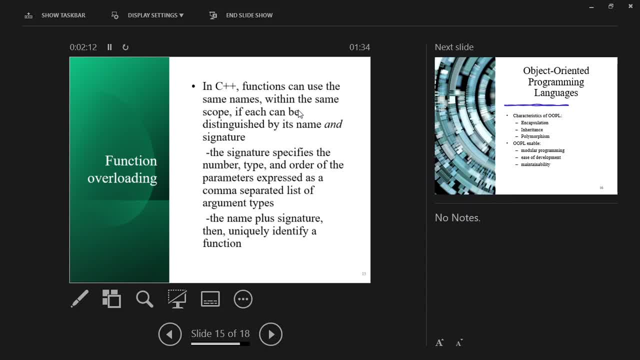 And Like What should be How can we Overload function 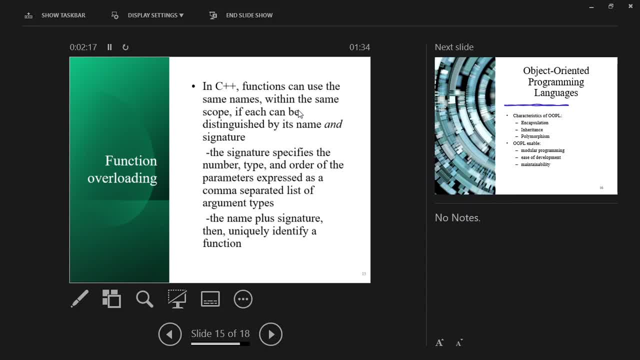 Functions What is the difference What should be The difference between Two functions 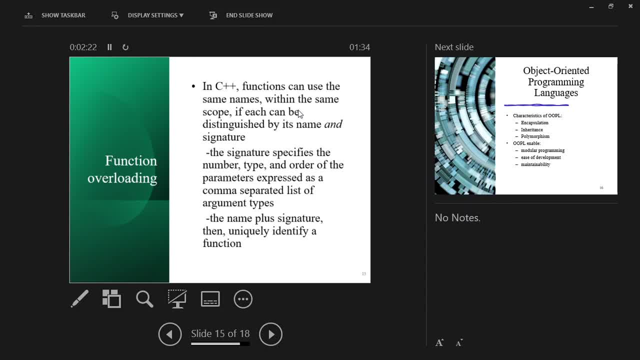 If you want to Overload them So they can have The same name But the number And type of arguments Should be Different Ok Now 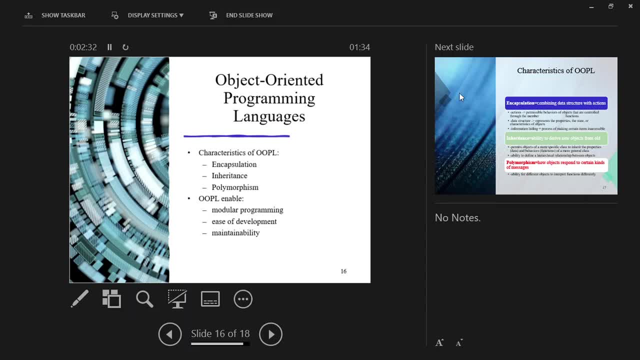 In the future Lecture Like These These things In detail Object oriented Programming Languages Have some Characteristics The first Characteristics We learnt about In this class That is Data encapsulation What does that mean That data And the functions That operate On that data You put them Or package them Together In one Class Ok This is called Data encapsulation Inheritance Attributes and behavior From another class So inheritance Is a very useful Mechanism of Extending code 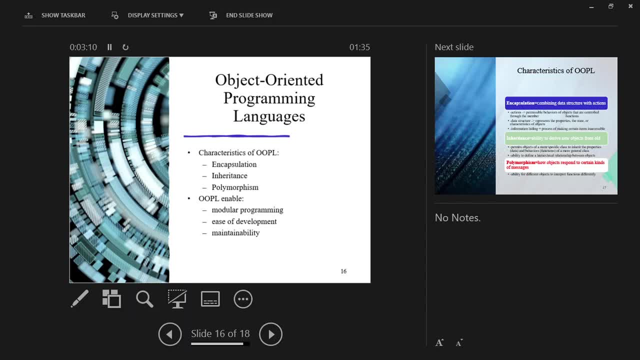 If you Have already A code Given to you You have to Extend it Ok So you can do it Very easily Through inheritance Normally In normal life You can also see that For example If you have a manual car You say I want to do it Automatic So you have The full structure All you do That you put 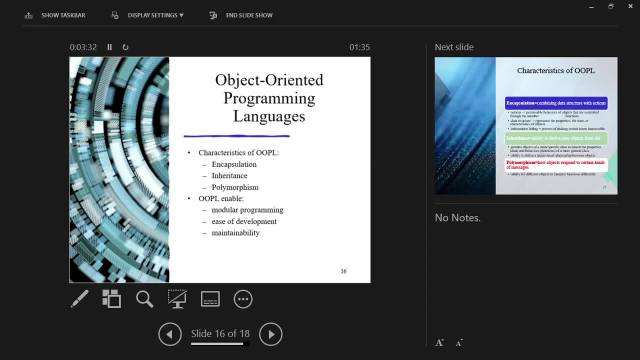 Automatic So you can Extend it And create A more specific Class Or more Extensive Class So inheritance Is a mechanism In which You take general Classes And make specific 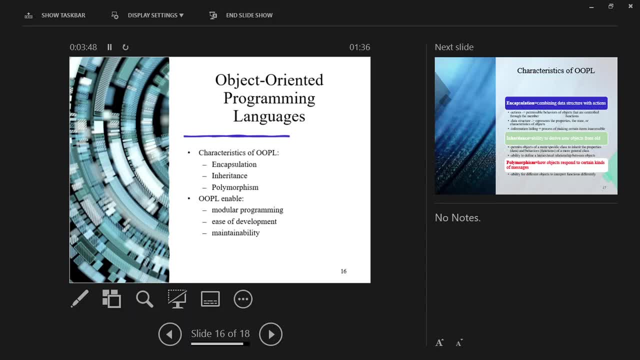 Classes Or extend Existing Classes Extend Their functionality Polymorphism Is As the name Reveals Polymorphism 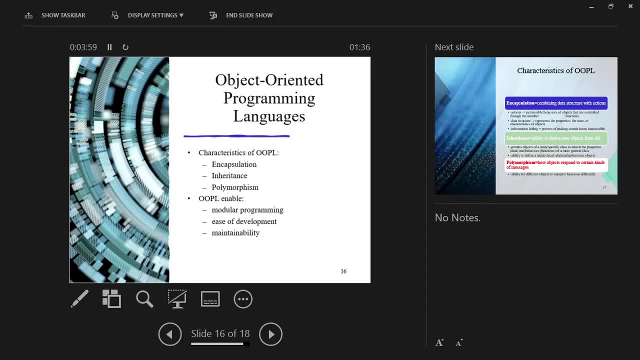 Poly Means Many You can use One One 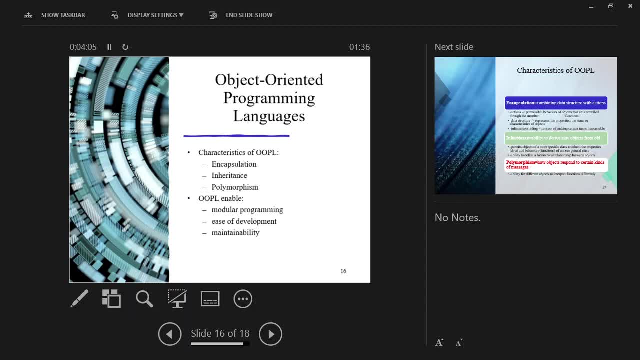 Variable To access Different Objects Ok Different types Of objects You can call 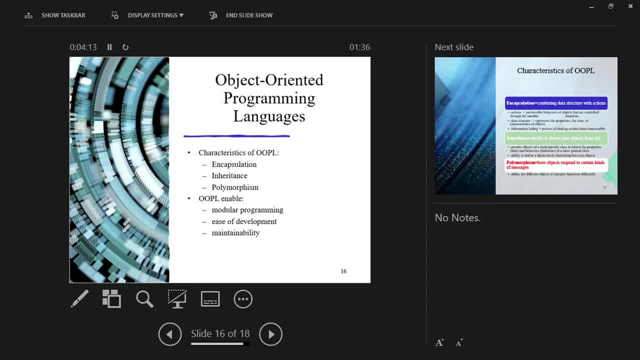 Different types Of objects Or different Methods With one 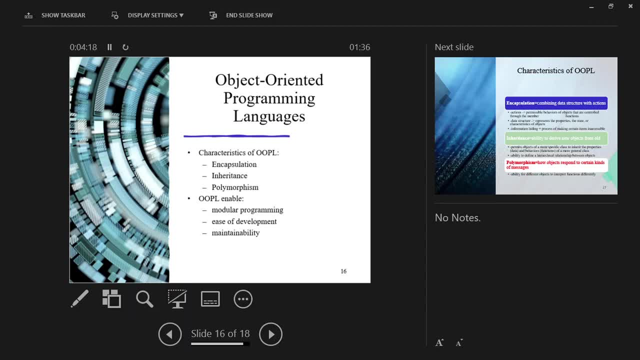 Variable In what Situations Is its Utility 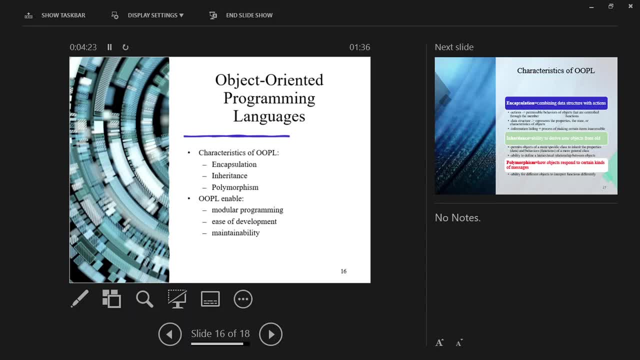 For example If you are Playing a Game On your Smartphone And you Get a Game Then you 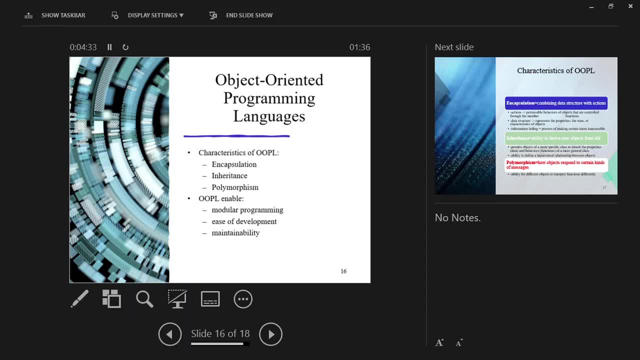 Return to The game And then you Start the Game When the Game Pauses All the Objects Of the Game Stop At Their 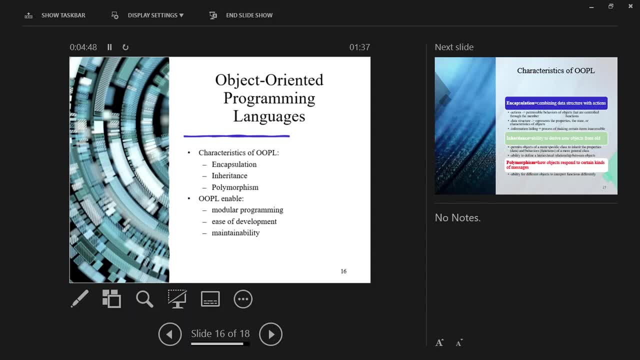 Place That means How The Programmer Will Do This Work The Programmer Has To Call So 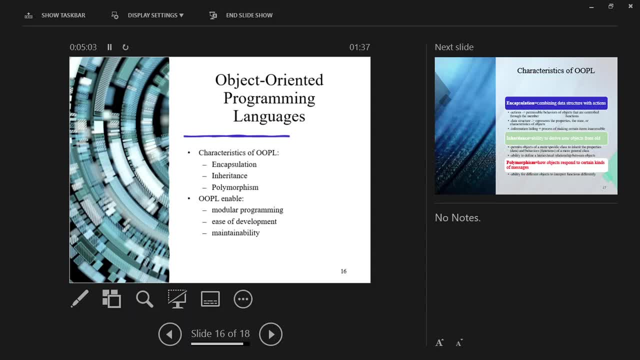 This is A very Good Example But Polymorphism Helps You In Those Situations Where You Want To 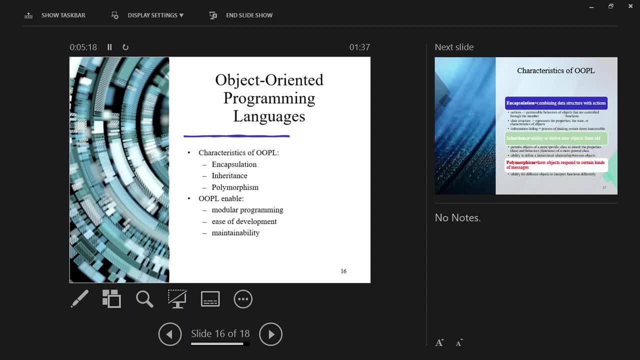 Control Many Objects With One Variable So There Polymorphism Helps You Learn And You Learn 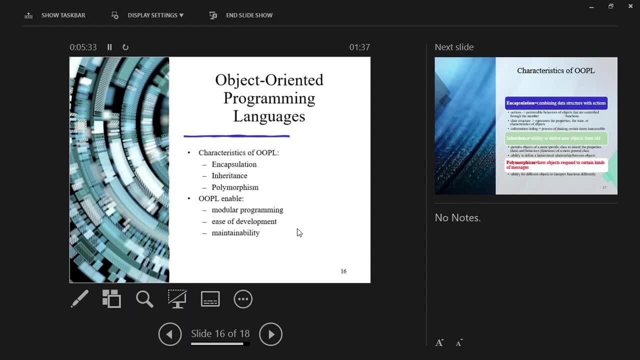 To Implement As Well And OOP Has Major Advantages Again We Are Towards The End 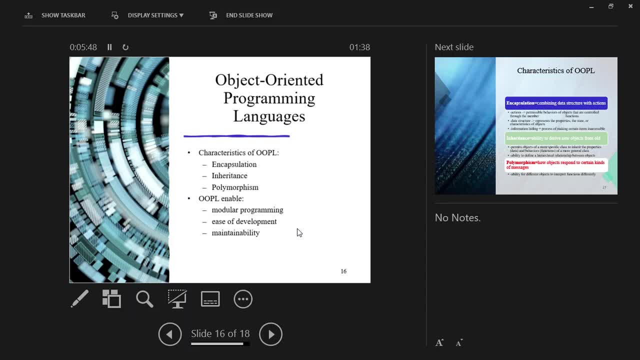 Of This Lecture OOP Enables Modular Programming So Your Program Is Fixing A Module If 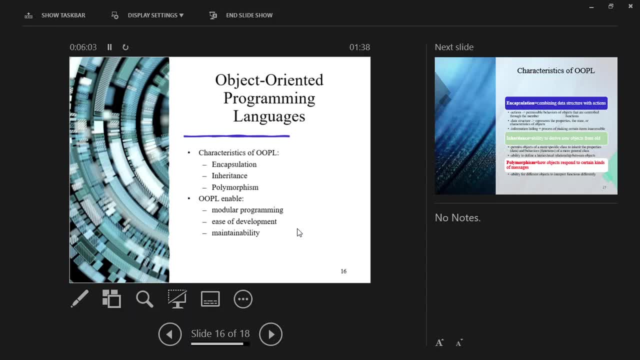 A Module Is Having A Problem Fixing It Becomes Very Easy So You Only Have 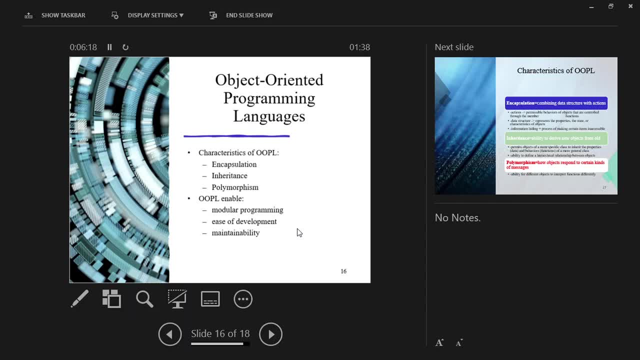 To Look At That Module And Its Behavior It Can Maintain The Code If There 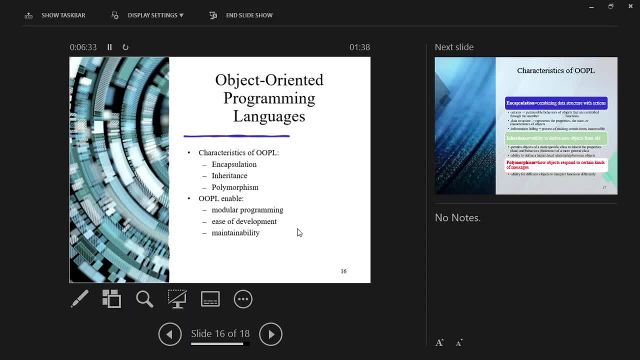 Are Bugs Bugs Can Be Removed Code Can Be Advanced So That Is Basically Somebody 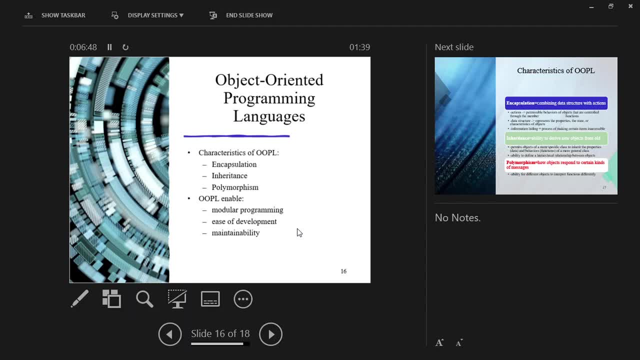 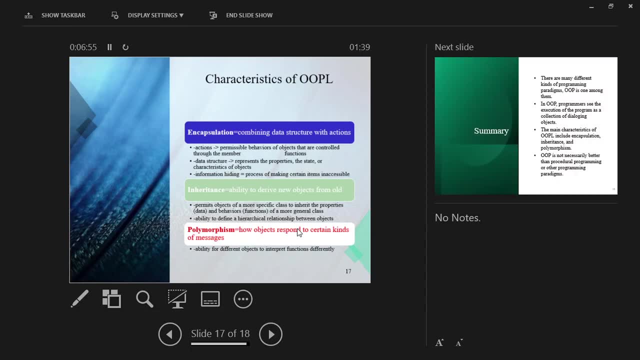 Is Maintaining That Code Removing The Bugs And So We Have Talked About This Encapsulation Inheritance Polymorphism 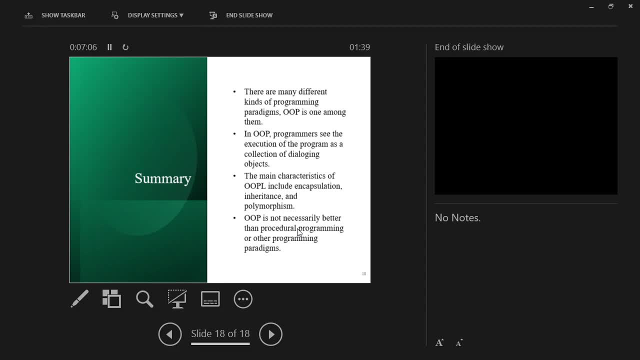 And This Is The Summary Of This Lecture There Are Different Ways 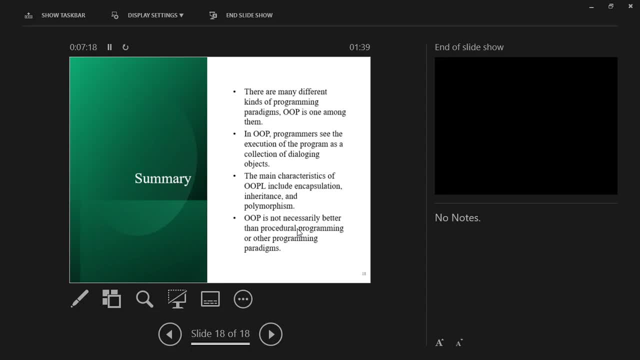 Of Doing Programming Each Way Has Its Unstructured Programming So One Thing That We May 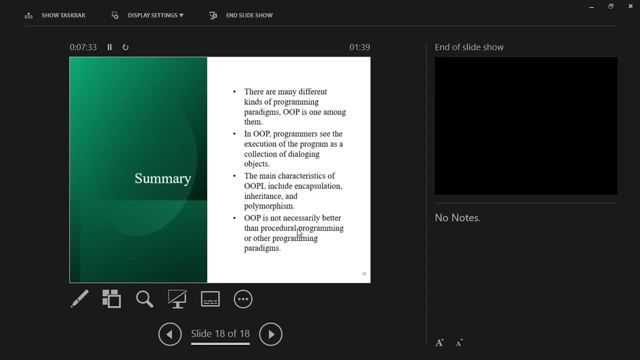 Say We May Be Able To Say Definitively Is That Structured Programming Is Better Than 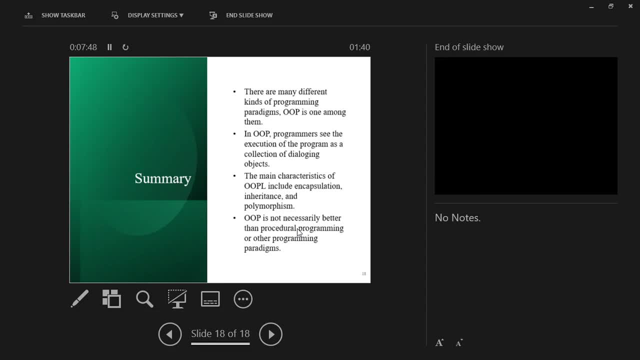 Unstructured Programming You Cannot Go That You Can Solve Big Problems More Complicated Problems With 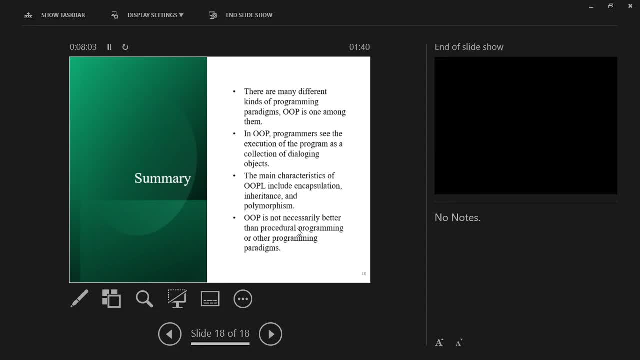 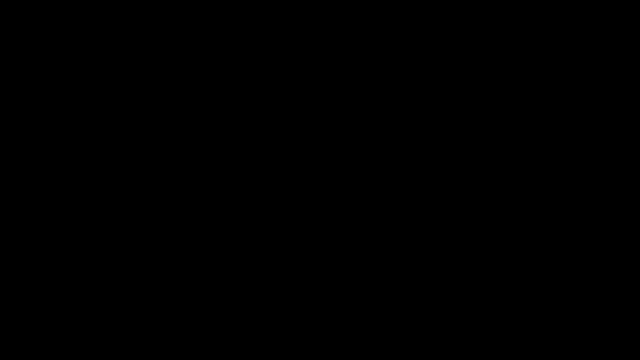 Relative Ease So We Have Talked About These Things You Can Also Go Through It Now If You Have Any Questions